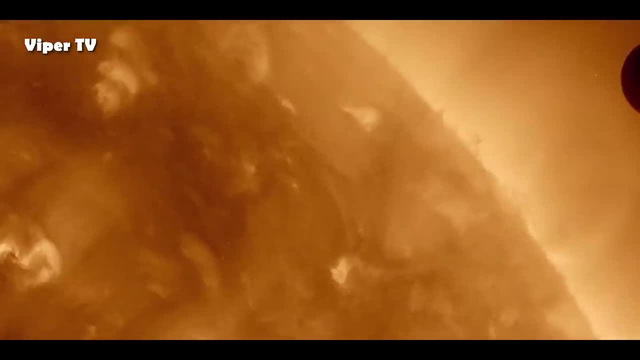 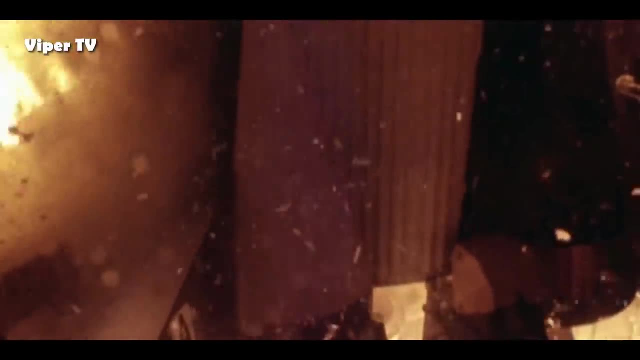 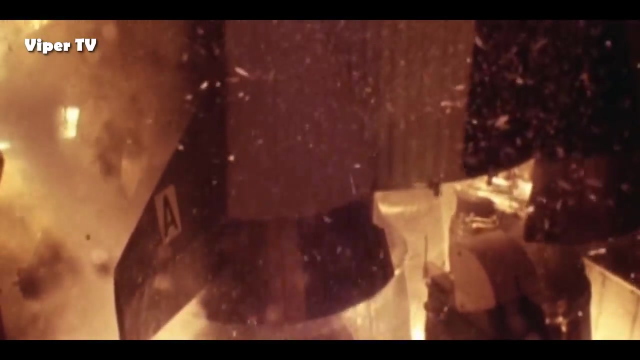 Venera, which attempted to explore the atmosphere and surface of Venus directly for the first time. The initial launches of the Venera program failed before they had even left Earth's orbit, but within a couple of years the program began to slowly see some success. Venera 1. was successfully launched on the 12th of February 1961.. Designed as a flyby mission, it is thought to have passed within 100,000 kilometers of Venus When the Probe came into play. the Venera 3 was used as a power satellite to measure Earth's 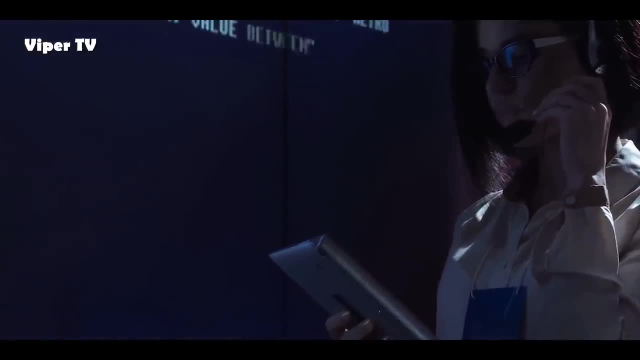 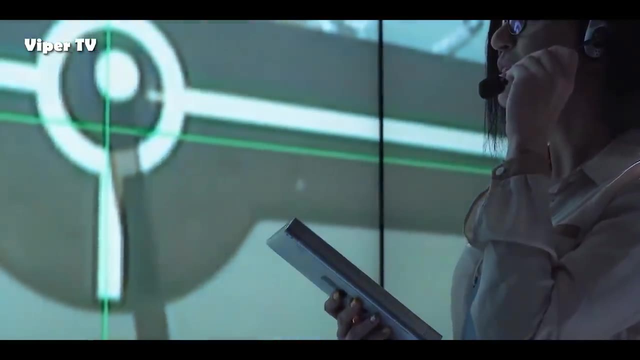 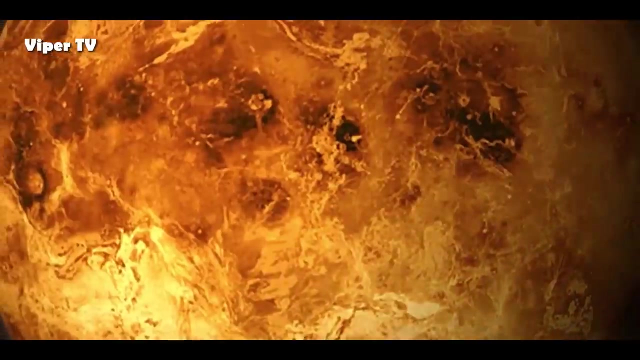 movement, But a total telemetry failure on the craft meant that no data was returned to Earth. As far as we know, Venera 1 is still in orbit around the Sun to this day. Venera 3 attempted to go a step further and was designed to enter the Venusian atmosphere to take the 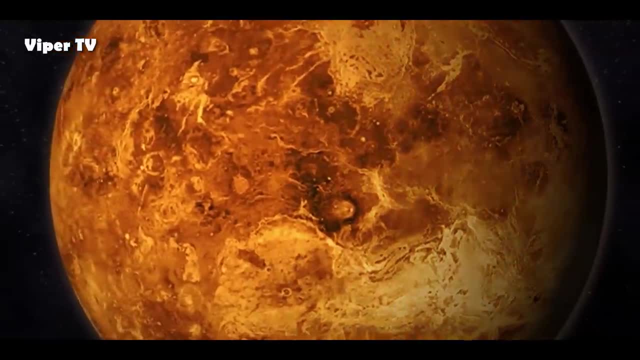 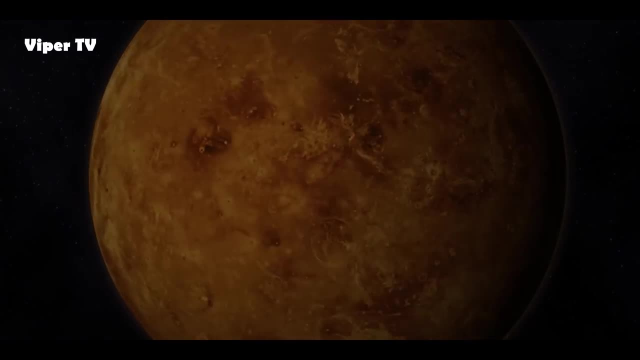 first direct measurements. However, on crossing the atmospheric boundary, the probe's systems failed and no data was returned as it plummeted towards the ground. All that was left for the historic position as the first human-built object to crash into another planet's surface. 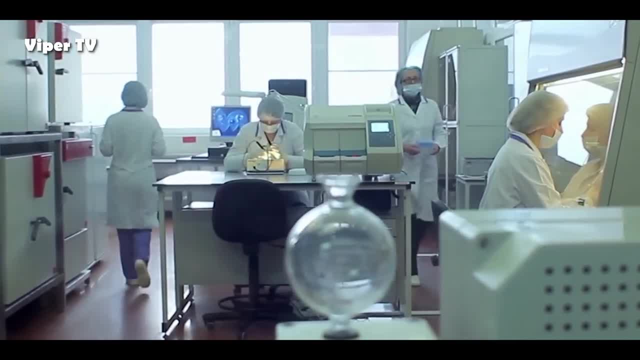 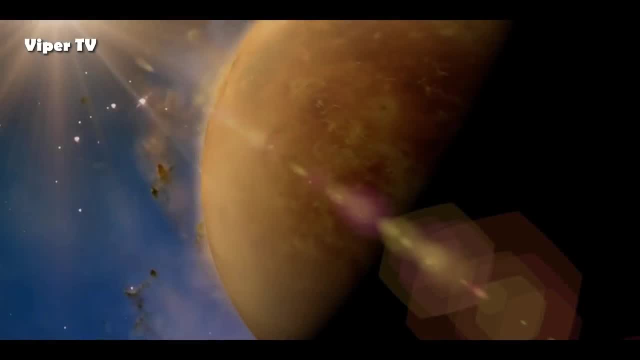 Nobel Prize-winning chemist Svante Arrhenius was one of the most renowned scientists to fuel the mythology of what lurked behind Venus's cover. Like many of the scientists of his era, Arrhenius let his curiosity wander into many different realms, including astronomy. 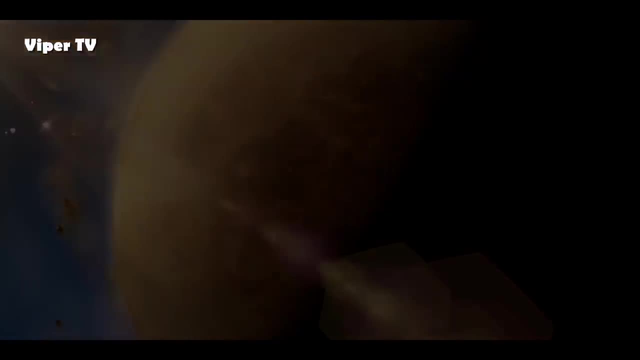 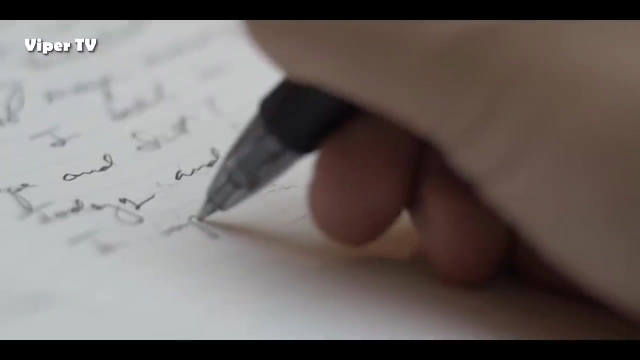 and he hypothesized at length about the Venusian environment. Assuming the clouds of Venus were composed of water, he wrote in his book The Destinies of the Stars that a very great part of the surface of Venus is no doubt covered with swamps, creating an environment not unlike 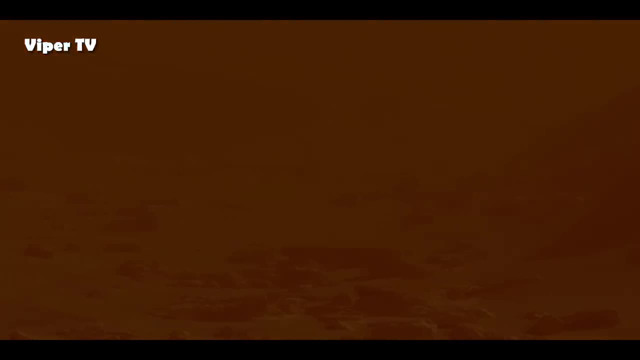 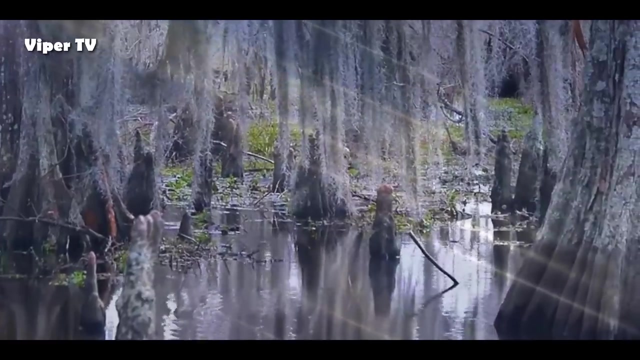 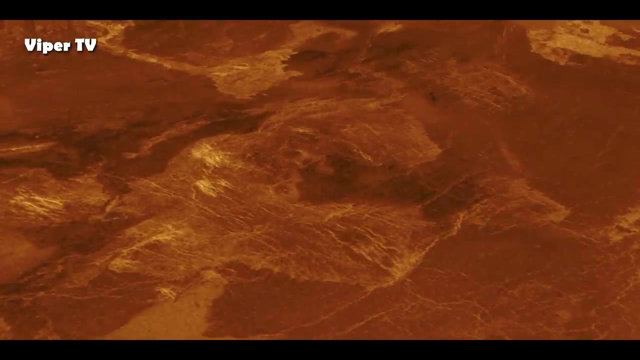 the tropical rainforests found here on Earth. Expanding on this picture, he suggested that the complete cloud cover of the planet created a uniformity, totally unlike the extremes of weather that define different parts of the Earth. In Arrhenius's imagination, this stable 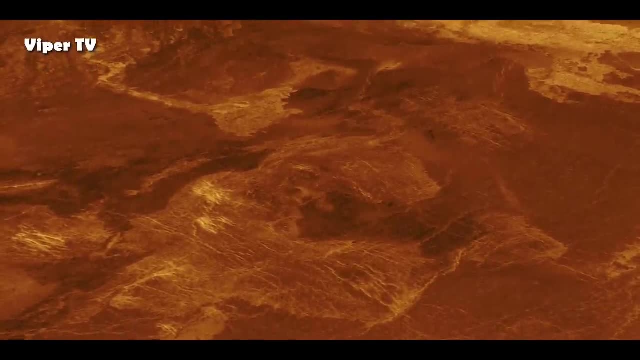 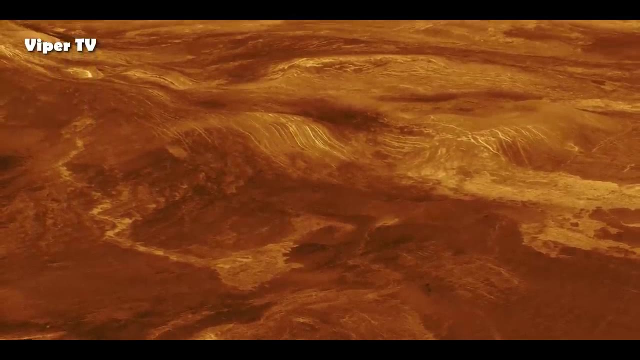 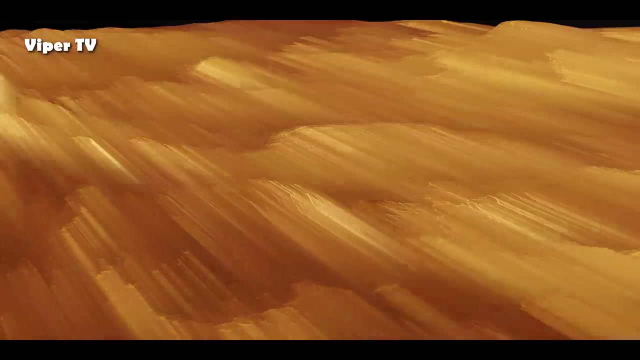 environment with a consistently uniform climate all over the planet, meant that any life on Venus lived without the evolutionary pressures of changing environments that drive natural selection here on Earth, leaving Venus in an evolutionary limbo akin to the Carboniferous Period. Describing: 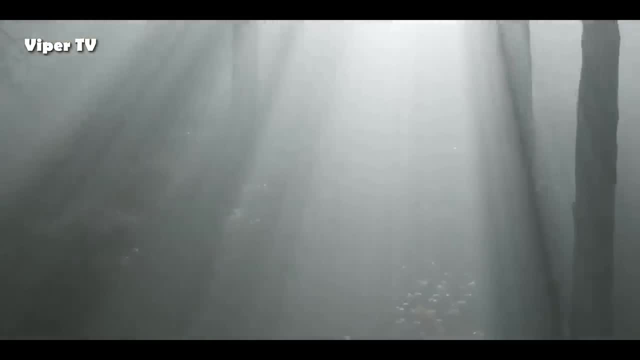 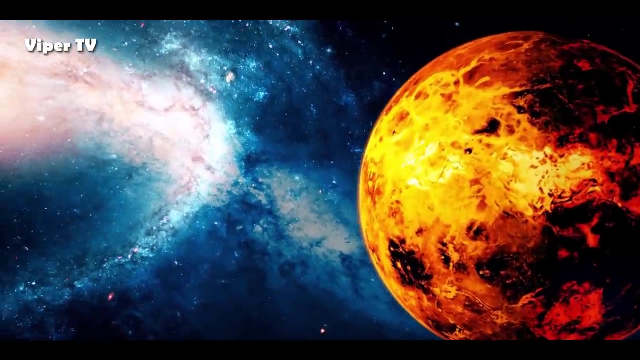 a world full of prehistoric swamps and dark forests. Arrhenius created the perfect canvas for science fiction writers of the time to conjure up a menagerie of curious life forms lurking beneath the clouds- clouds. Today, Arrhenius is far less known for his fertile imaginings on the wildlife of Venus. 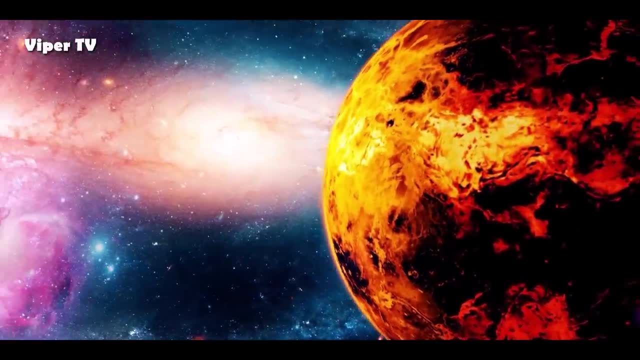 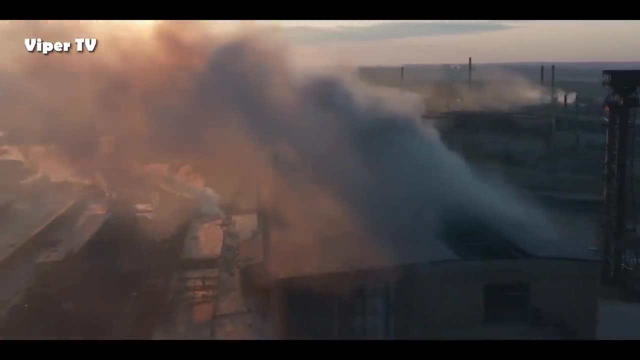 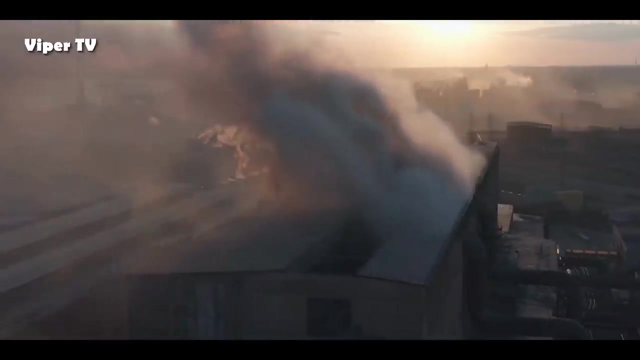 than he is for his work on the climate of Earth. In 1896,, he was the first scientist to use basic principles of chemistry to demonstrate the impact that the atmosphere can have, in particular levels of carbon dioxide, on the surface temperature, a process that was called the Arrhenius effect. 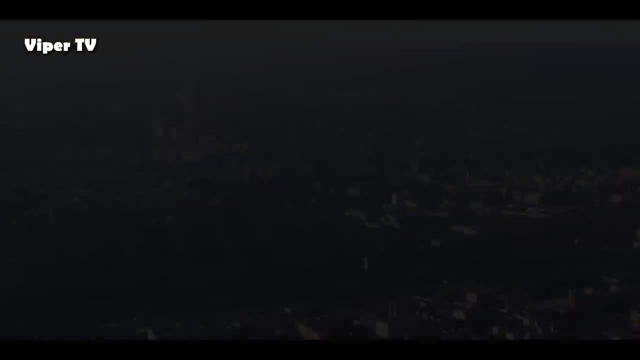 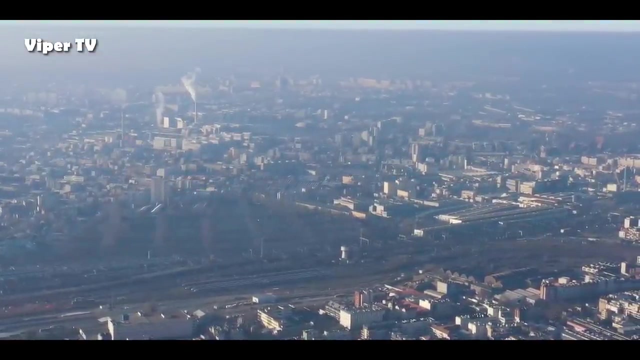 but is now known as the greenhouse effect, an effect that would not only have profound consequences for our understanding of our impact on our own planet, but would also be vital in explaining the true nature of Venus beneath the clouds. The Mariner 10 mission had enabled. 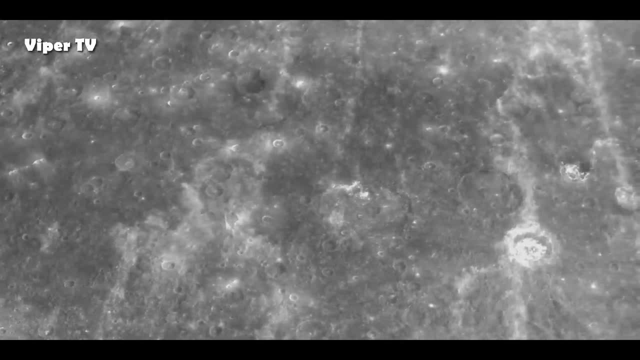 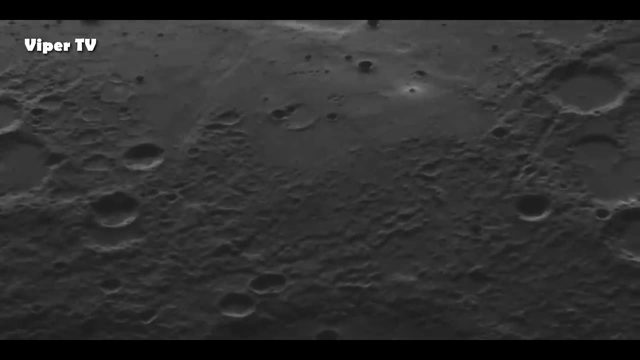 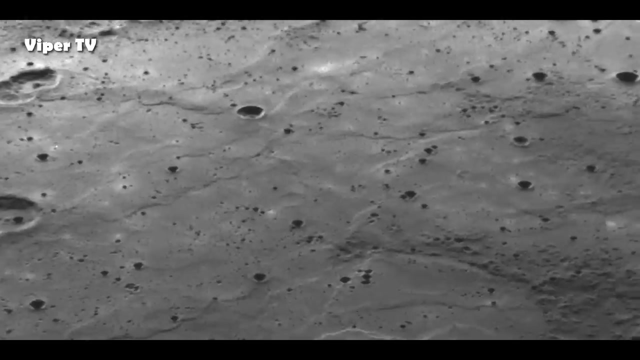 scientists to see about half of the planet. so the first real glimpses into the terrain of Mercury came from the flybys of MESSENGER. As planetary scientist Nancy Chabot explains, before MESSENGER we had only seen 45% of the planet and we saw some stuff during the flybys. 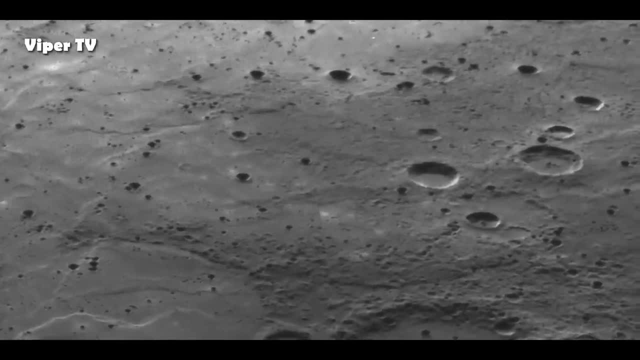 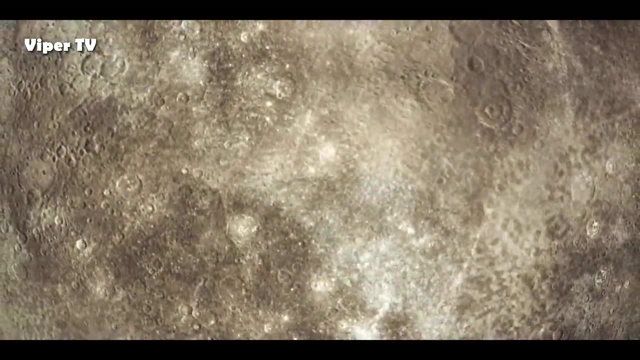 before we went to Earth, But after orbiting the planet. we've now mapped 100% of the planet and seen nearly everywhere. There are some permanently shadowed regions which are still mysterious, but after mapping the full planet we have a good idea of what the surface looks like. 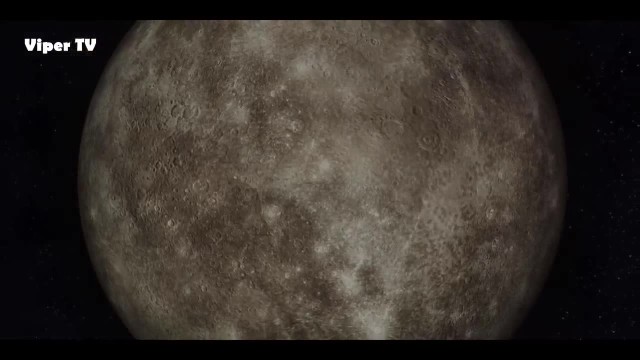 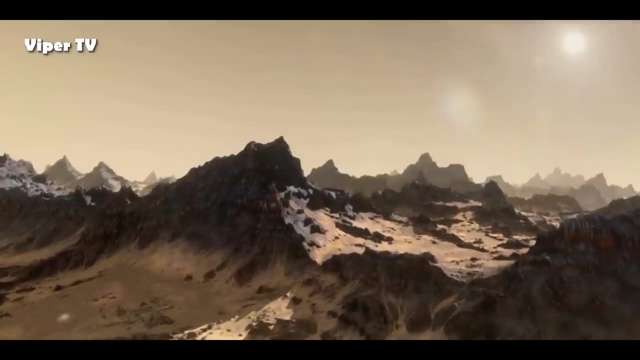 and craters are absolutely a dominant landform. This planet has been sitting there for billions of years and been hit over and over, and it hasn't had a lot of processes to destroy those craters. Amongst the thousands of craters, there are a number of them, and they're all the same. 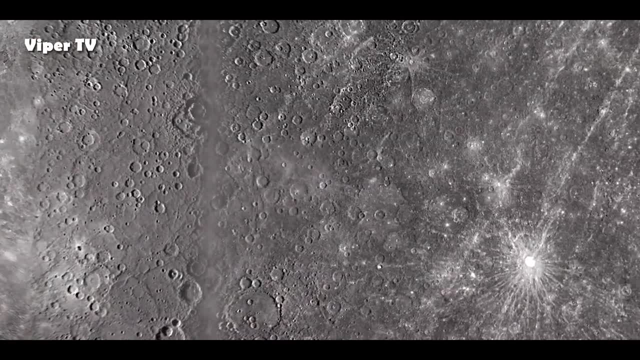 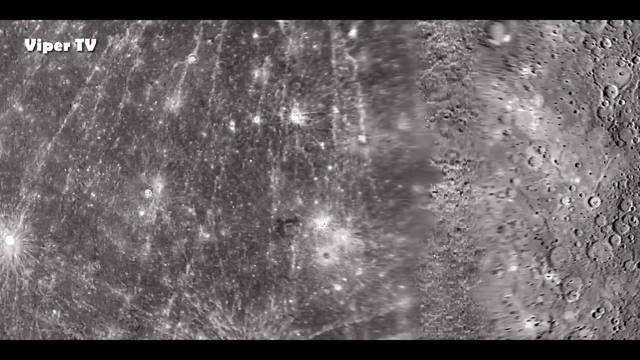 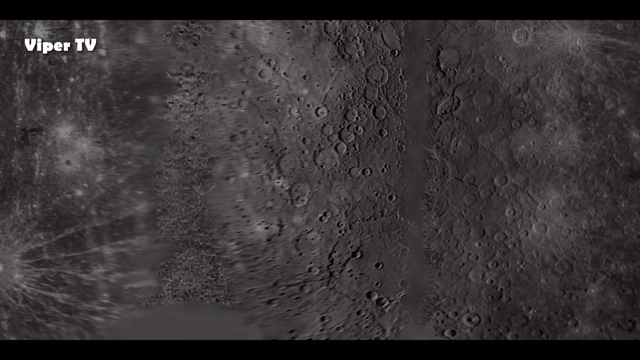 There are thousands upon thousands of craters on Mercury. The largest by far is Caloris Planitia, a lowland basin 1,525 kilometers in diameter that is thought to have formed in the early years of the solar system, around 3.9 billion years ago. It was first spotted as Mariner 10. 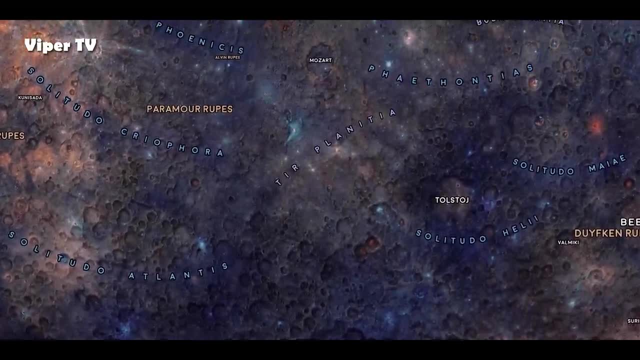 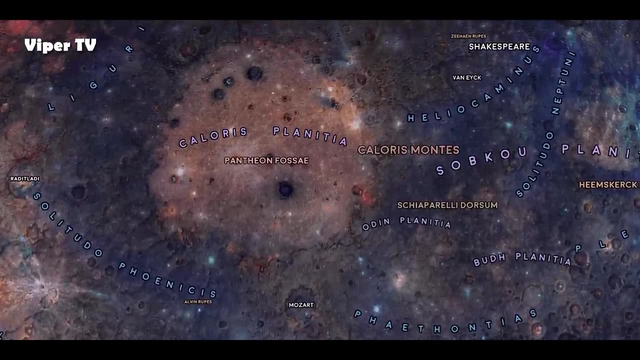 sped past in 1974, but due to the trajectory and timing of the craft, only half of it was lit. so the full character of this crater remained a mystery for another 30 years, until MESSENGER could photograph it in all of its glory. 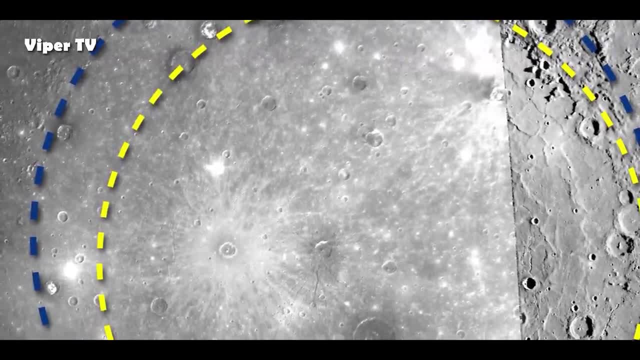 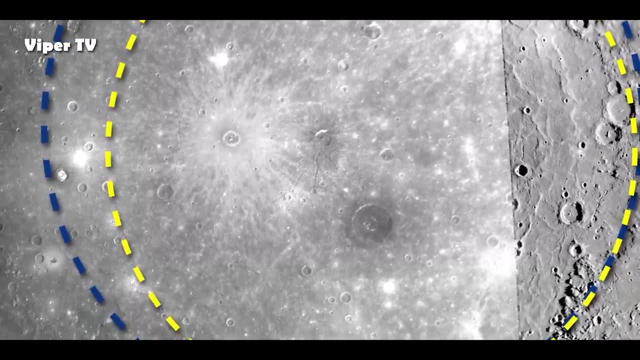 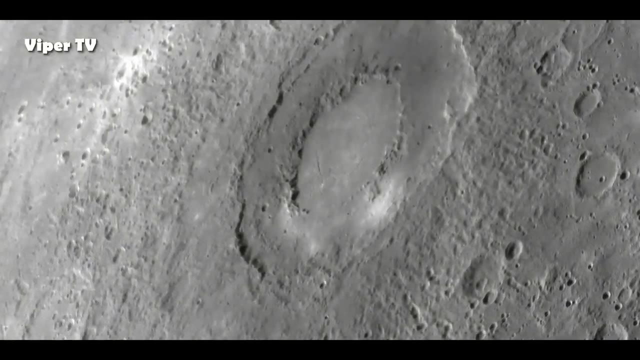 Taking one of its very first photos, MESSENGER revealed Caloris to be bigger than had been previously estimated, encircled by a range of mountains rising two kilometers from the Mercurian surface, whose peaks create a 1,000 kilometer boundary around the lava plains within. 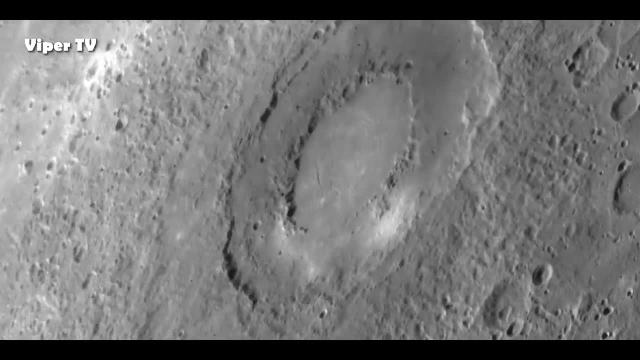 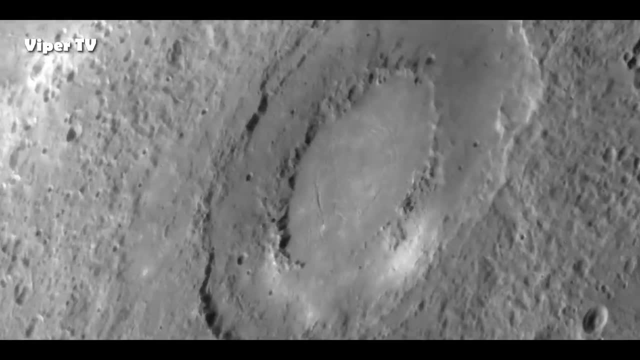 On the other side of the mountains. the vast amount of material that was lifted from the planet's surface at the moment of impact was found to be. a large amount of material that was lifted at the moment of impact formed a series of concentric rings around the basin, stretching. 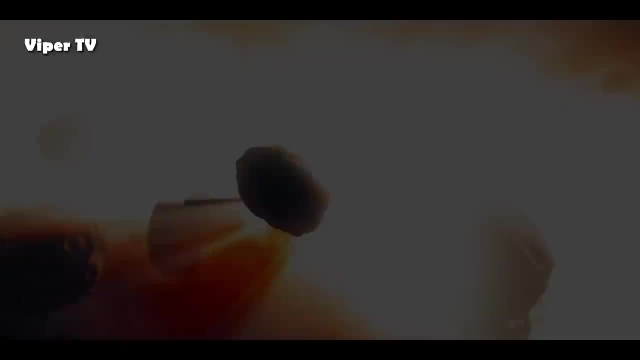 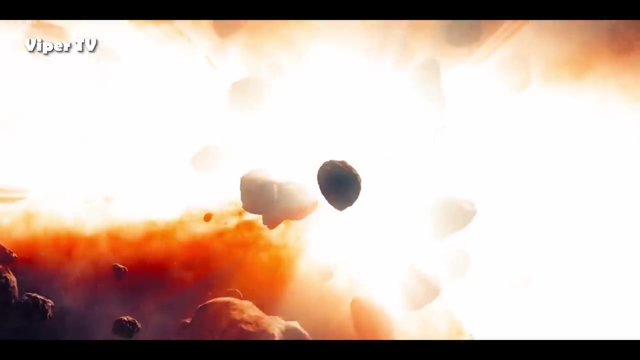 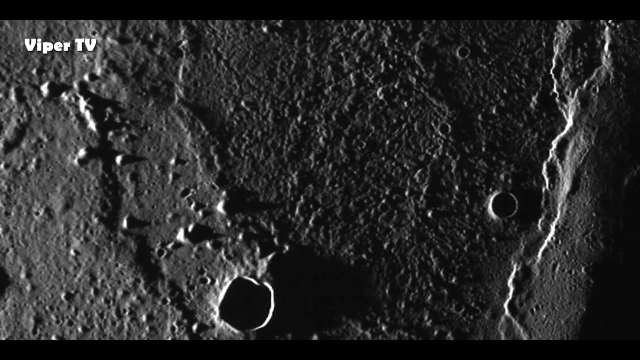 over 1,000 kilometers from its edge. The collision that created Caloris hit Mercury with such force that it also had more global consequences. MESSENGER photographed in great detail an area named in the not particularly scientific vernacular the Weird Terrain, a region at 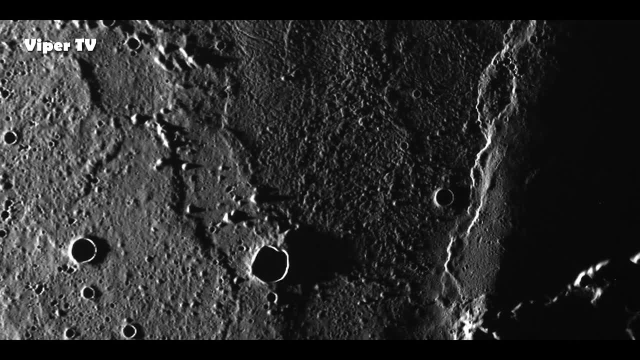 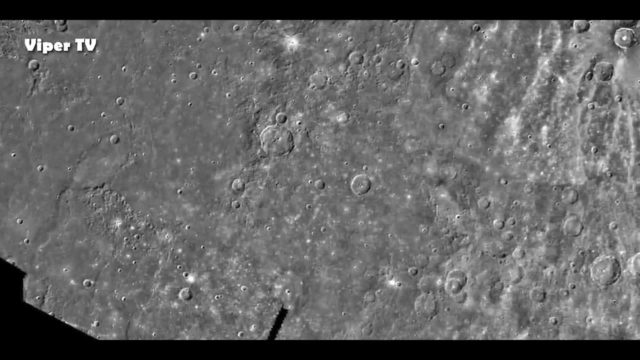 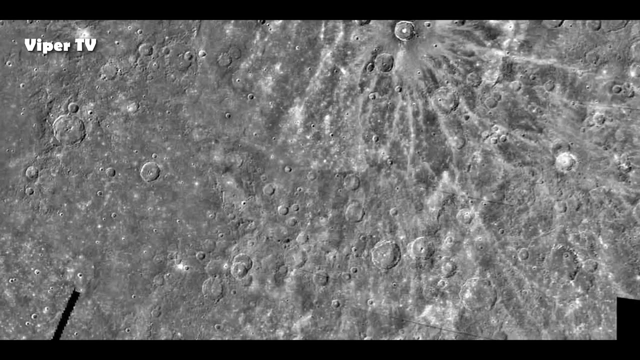 the planet's diametrically opposite point, the antipode. This area of strange geological formations, distinct from the rest of the surrounding terrain, was likely created by the seismic shock wave of the Caloris impact reverberating through the whole of the planet. 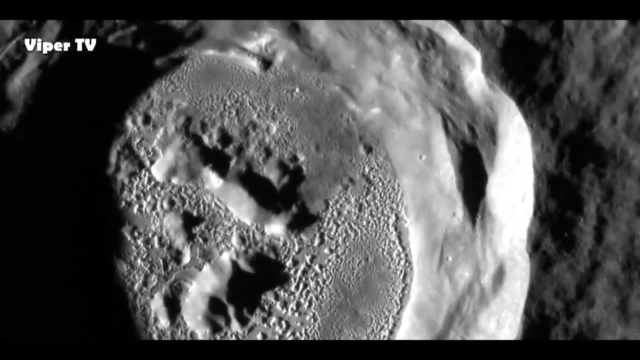 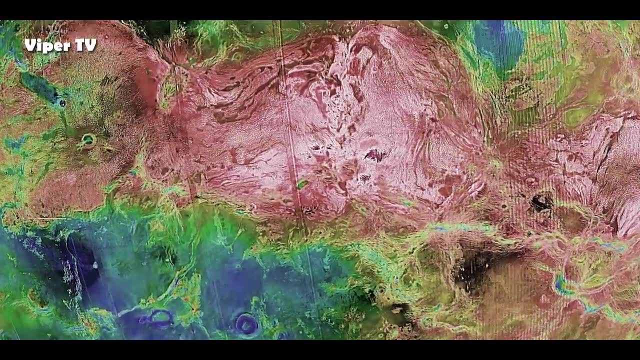 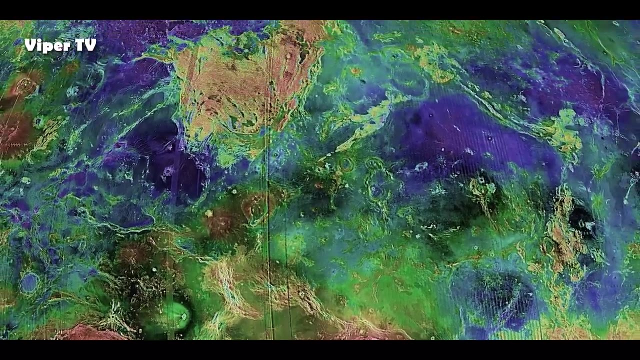 Right up until the end of its mission in 2015,, MESSENGER continued to uncover many of Mercury's secrets, including a few very particular surprises. Using a combination of photography, spectroscopy and laser topography, MESSENGER revealed tantalizing evidence that even this close to the sun, 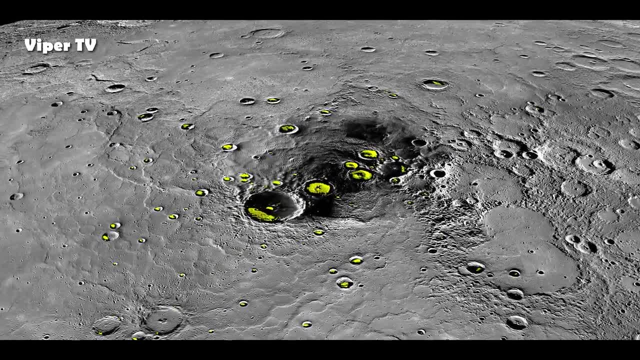 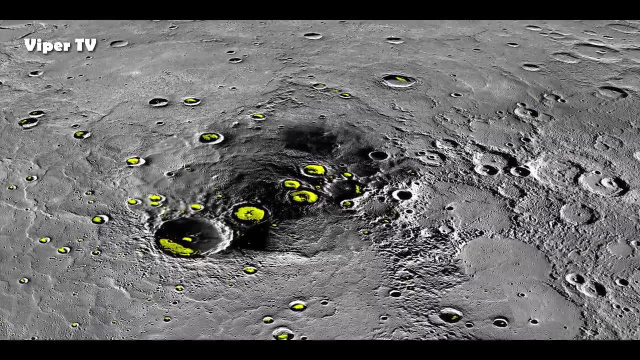 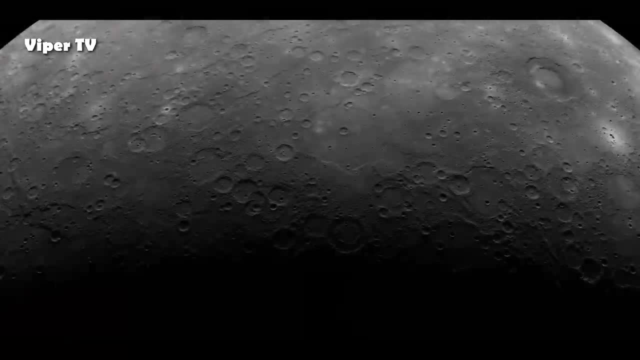 water- ice- can exist on the surface of a planet. Even though the sun blasts much of Mercury's surface, the tilt of its rotational axis is almost zero, So there are craters and features around the planet's poles that never see direct sunlight. Combined with the lack of atmosphere, 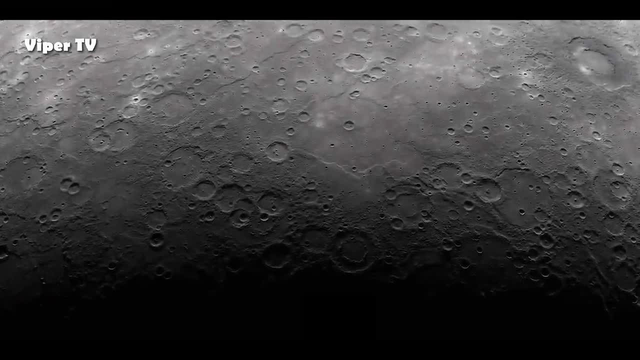 these regions are forever exposed to the freezing temperatures of space. J votes for the earth as the world's largestélite and the world's largest solar planet with freezing temperatures of space, And it's in this environment that MESSENGER was able to. 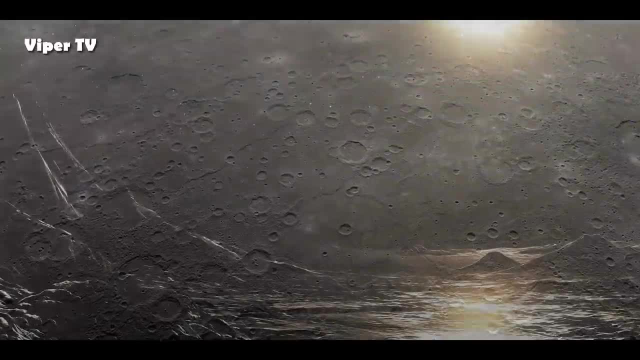 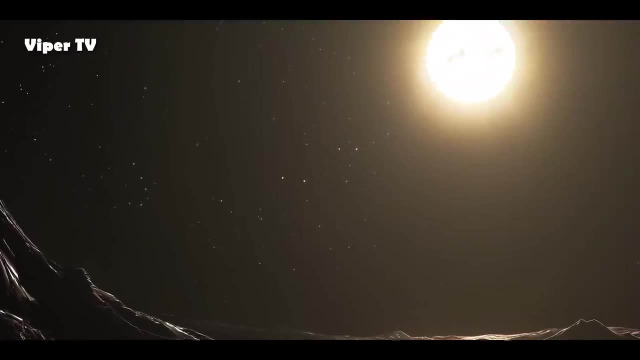 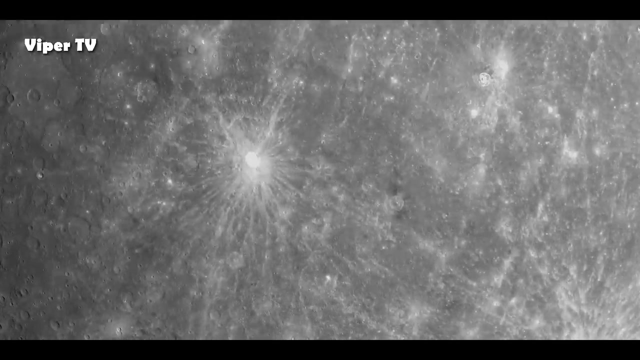 record the clear signature of water ice. Here, in the eternal night of a polar crater, it's cold enough for ice to survive for millions of years, just meters away from the savage ferocity of the Sun's light. However, MESSENGER's most startling discovery 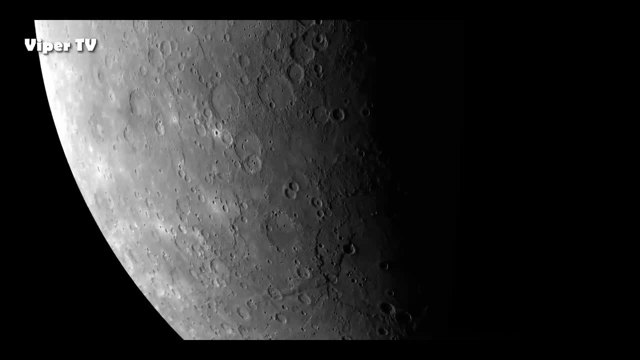 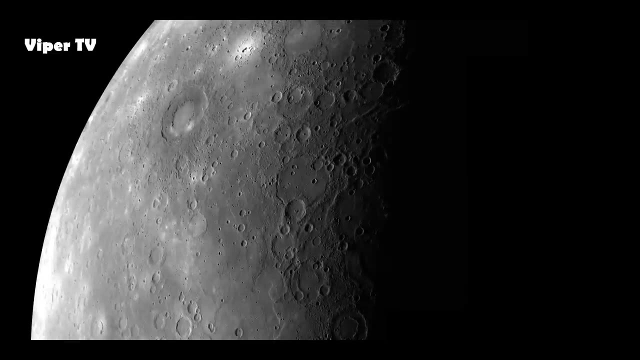 was still to come. The mission objectives had been developed to explore the deep history of Mercury and provide data to test against our theories of the formation and early life of the planet. MESSENGER was equipped with a collection of spectrometers designed to 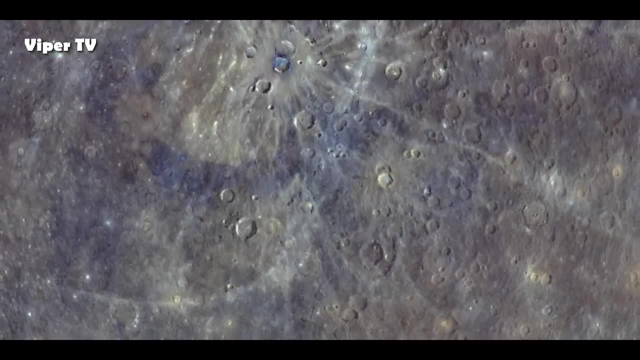 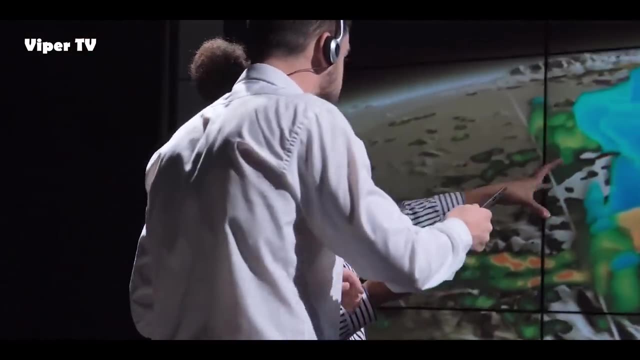 analyze the composition of Mercury at different depths. The MESSENGER team had worked on a detailed set of predictions outlining the chemistry of the planet, But as the spacecraft began to sniff at the Mercurian surface, it soon became clear that our assumptions had 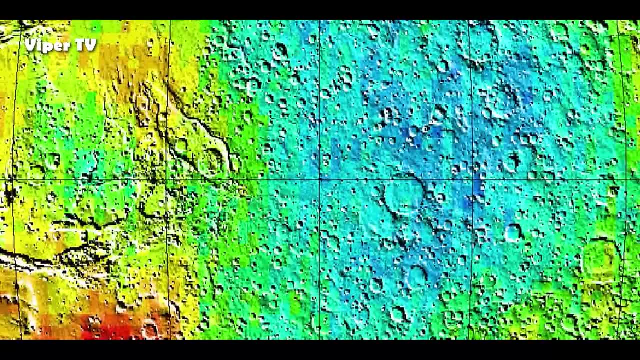 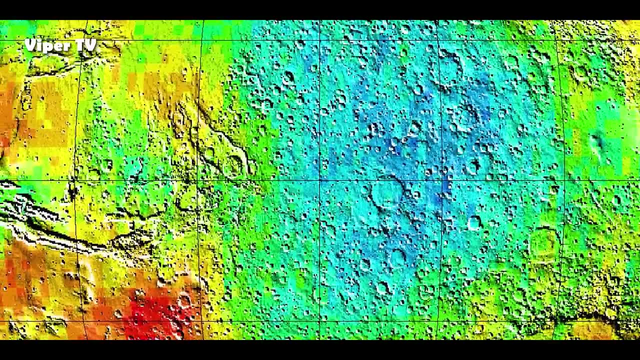 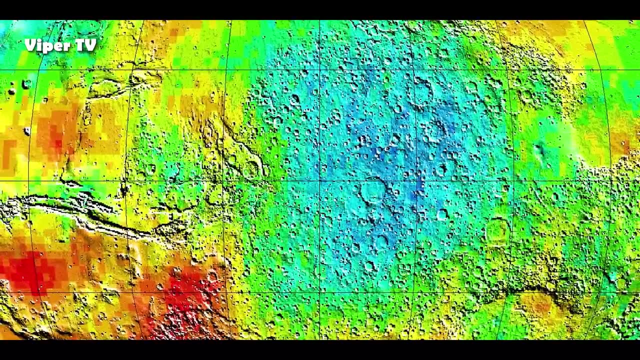 not been quite right. As the gamma-ray and X-ray spectrometers analyzed the elements on Mercury's surface, they began to measure the unexpected characteristic signature of a number of elements such as Phosphorus, Potassium and Sulfur, at much higher levels than they were expecting. 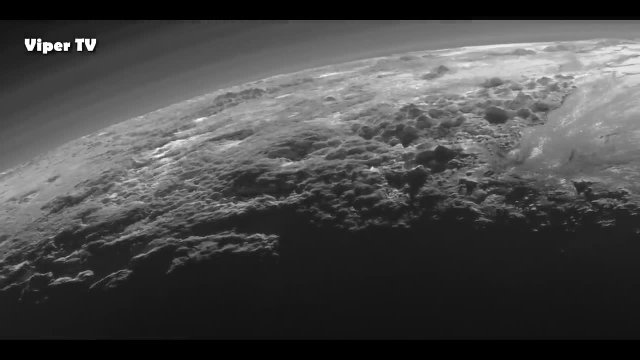 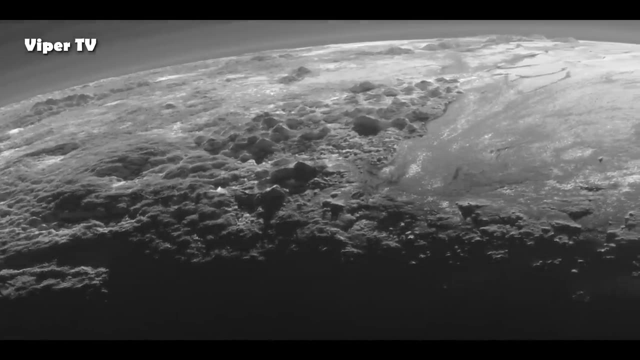 Up to this point, the working hypothesis had been that, during the formation of Mercury and all the rocky planets, as the rock condensed and combined to form the planet, the heavier elements, like ice and the rocks of the Earth would become more and more dense, But the 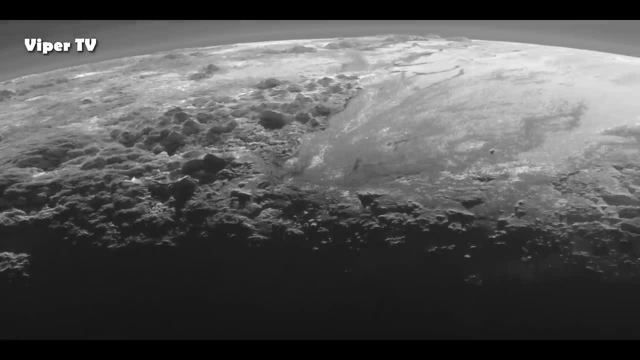 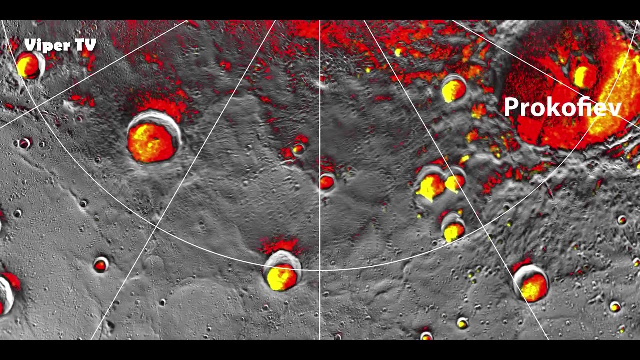 iron would sink towards the centre, forming the bulk of the core, while the lighter elements, such as phosphorus and sulphur, would remain near the surface. These more volatile elements would then be expected to be stripped away from the surface, particularly on a planet. 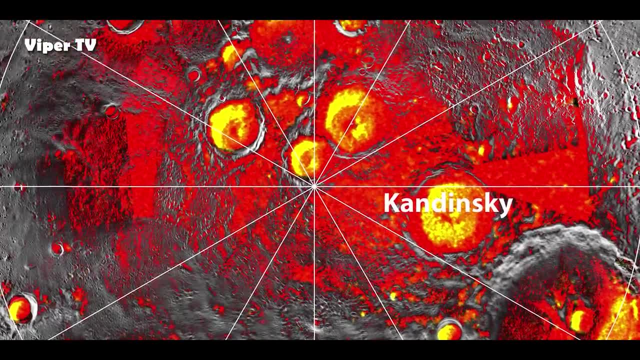 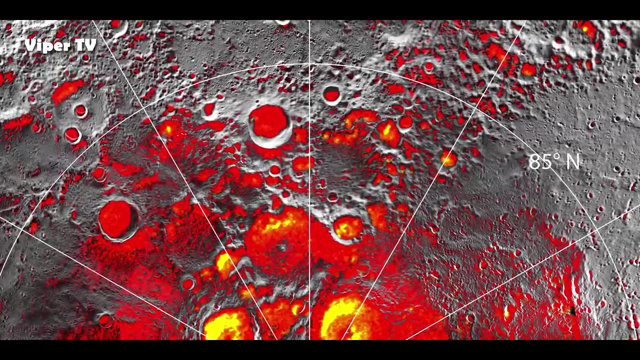 like Mercury, which is so close to the Sun. And yet the messenger data confirmed high levels of potassium and sulphur was detected at ten times the abundance of the element on Earth or the Moon. Both are volatile elements easily vaporised, and when this close to the 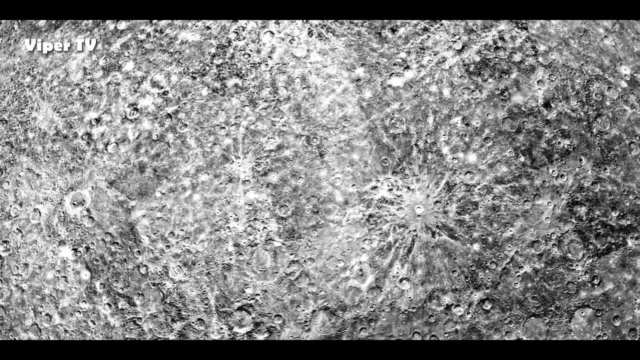 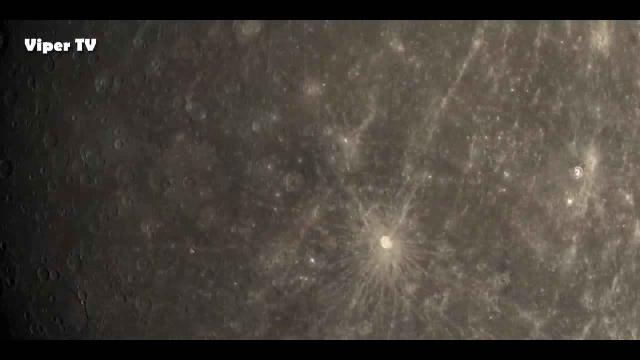 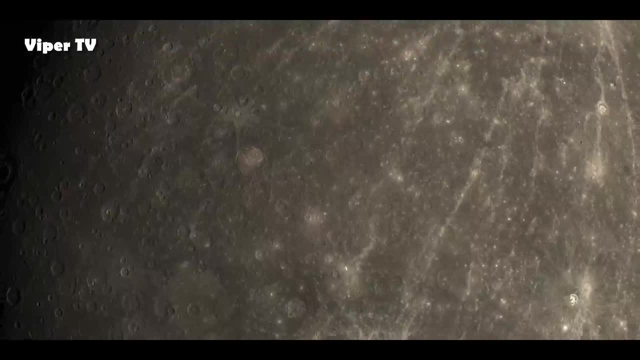 Sun. they simply should not have survived the planet's birth. On top of that, the messenger data confirmed what we had long suspected about the structure of Mercury: that it is the densest of all the planets, with a massive iron core making up 75% of the planet's radius. 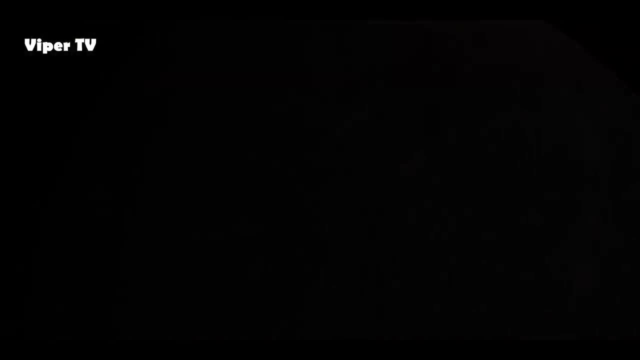 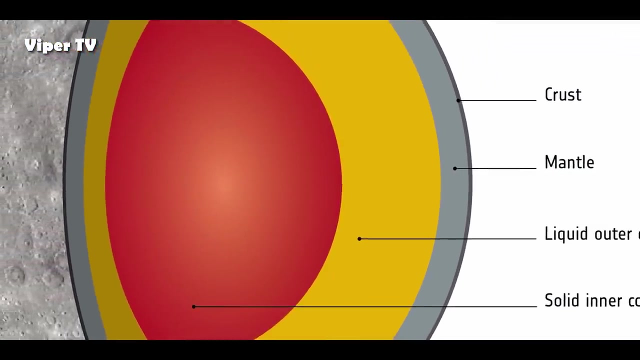 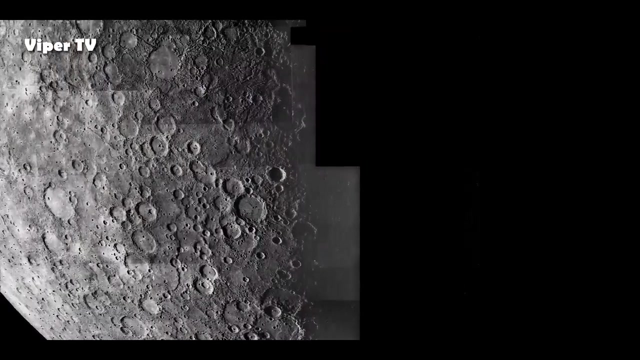 compared to just over 50% here on Earth. The core creates a strange lopsided magnetic field, indicating that the internal dynamics of the planet are different to anything we have seen before. All of this adds up to making Mercury something of a mystery, as nothing quite accords The eccentric orbit, the abundance 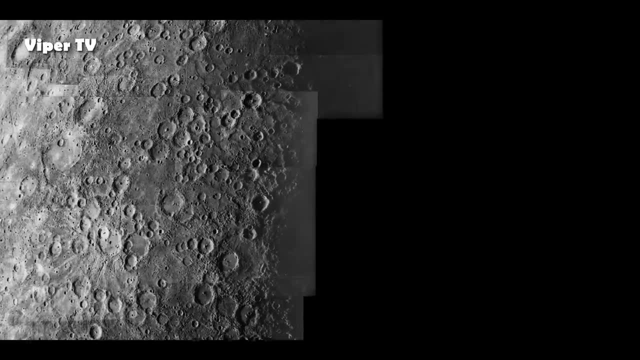 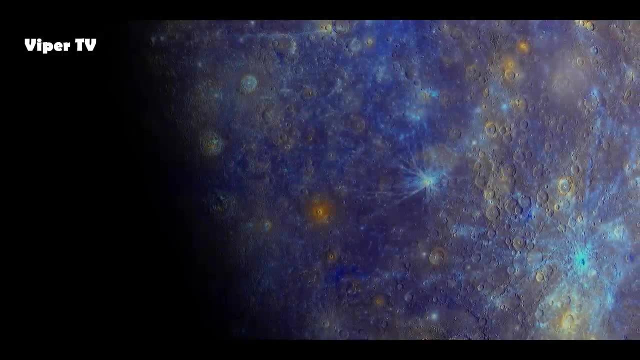 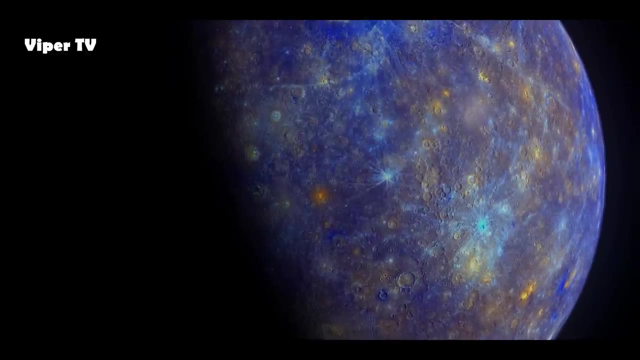 of volatile elements on the surface and the oversized iron core all point to the planet having a history far more complex than was first imagined, And the only explanation for this is that Mercury was not born in its current sun-scorched position. It has long been, supposedly. 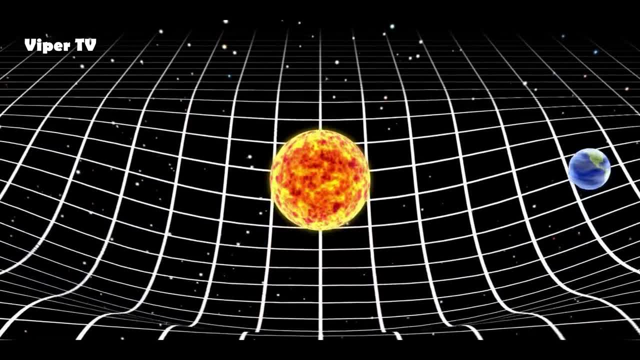 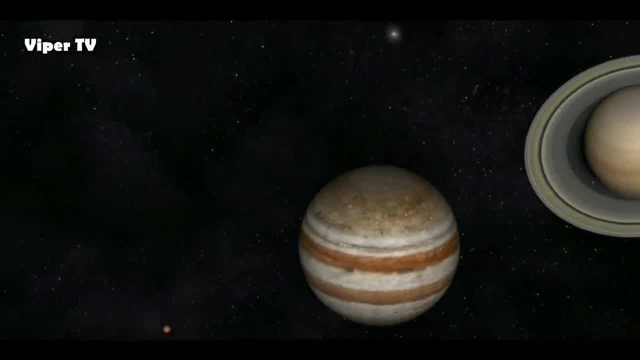 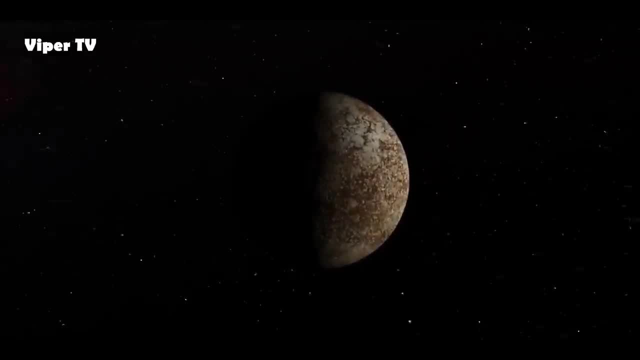 known that the orbits of the planets are eternal, stable loops that sustain the structure of the solar system in an endless rhythm, But everything we are learning now suggests that this is far from the whole story. Mercury, like all four of the rocky siblings, was formed. 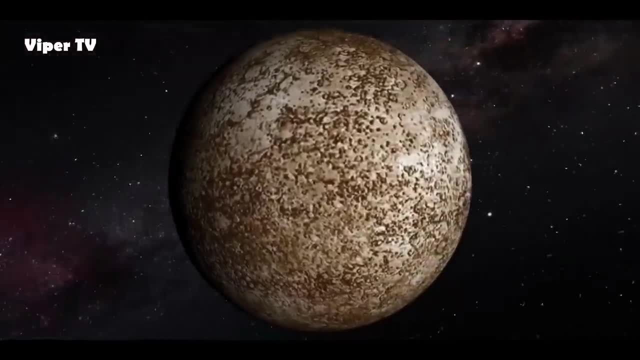 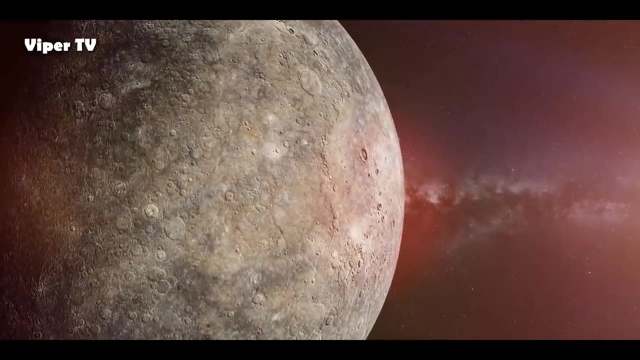 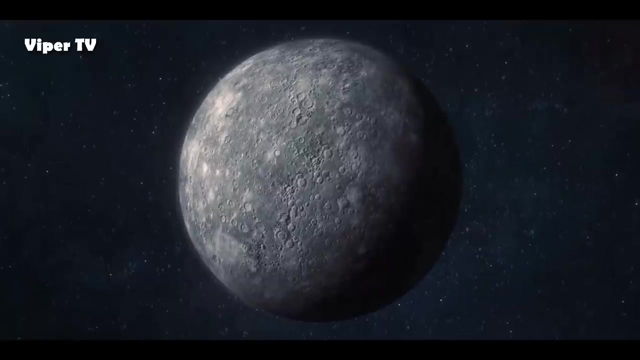 out of molten rock. A few million years later, as the young planet began to cool its crust, solidified and its journey around the sun transformed from being part of a swirling cloud into a clearly defined passage, an orbit. The path the infant Mercury travelled, however, was most probably far removed from the course. 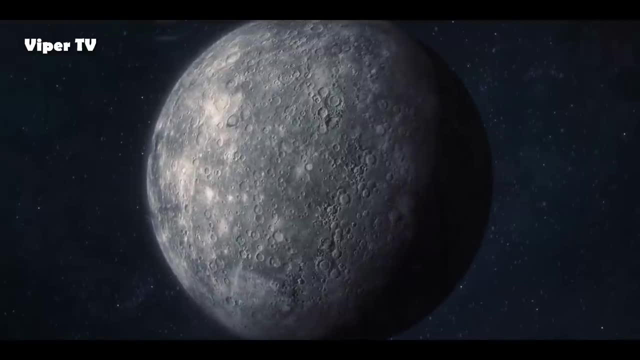 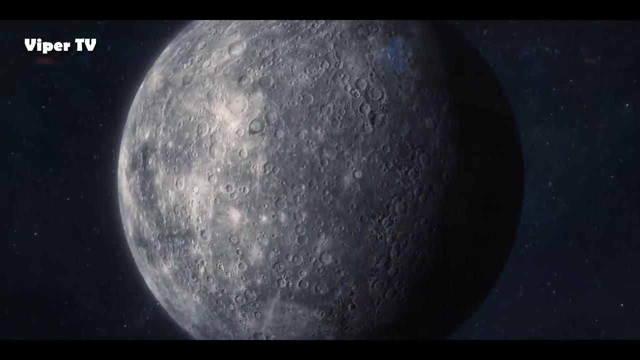 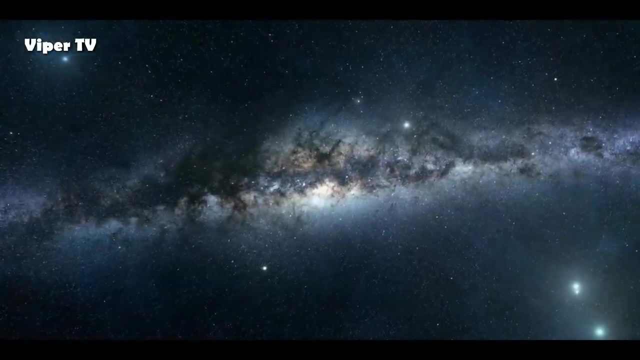 it now holds. The young Mercury was born not as the closest planet to the sun, but at a much greater distance. The Earth's orbit was far beyond the orbit of Venus, beyond Earth, perhaps even beyond Mars. This was a planet that came into being in the mildest region of the solar system. 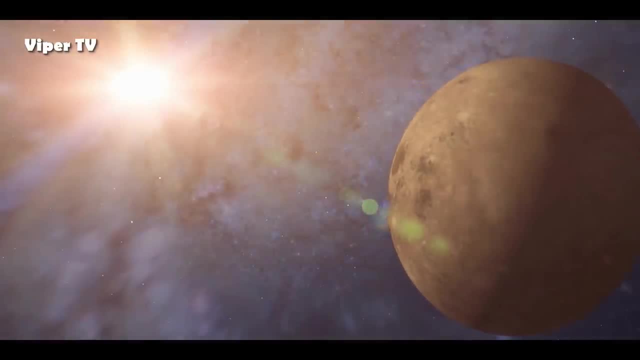 It was far enough away from the sun to allow volatile elements like sulphur, potassium and phosphorus to be folded into its first rocks without being vaporised away by the heat of the sun, But maybe near enough for its surface to be warmed, perhaps even just the right. 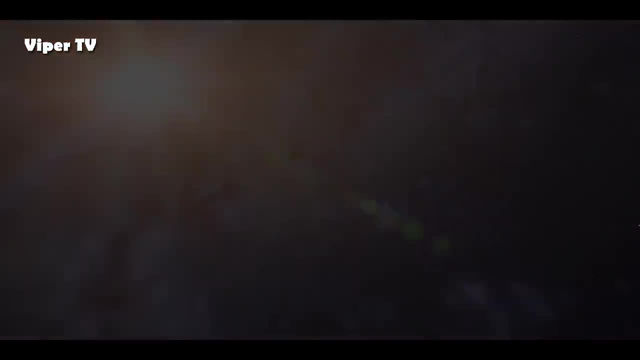 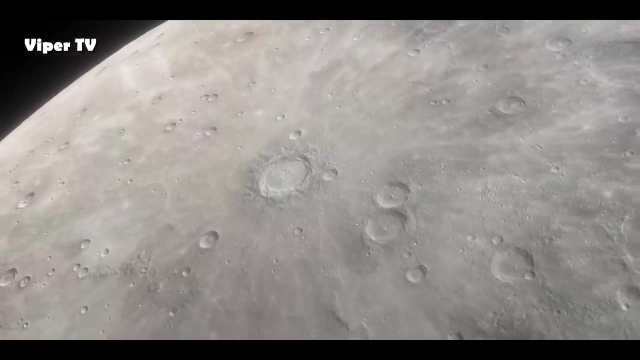 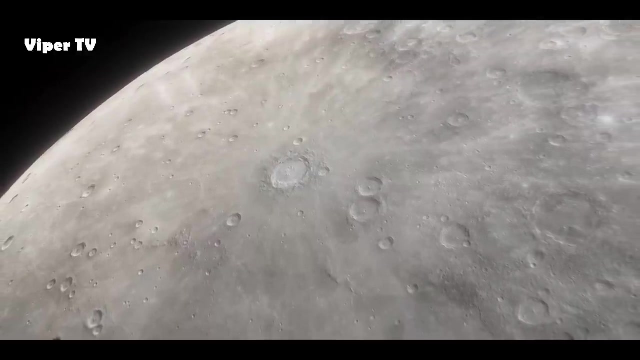 right amount for liquid water to settle on its surface. this may well have been a planet big enough to hold an atmosphere, a watery world upon which all the ingredients of life could well have existed. mercury, it seems, really did have its own moment in the Sun. but these hopeful beginnings were not to last. 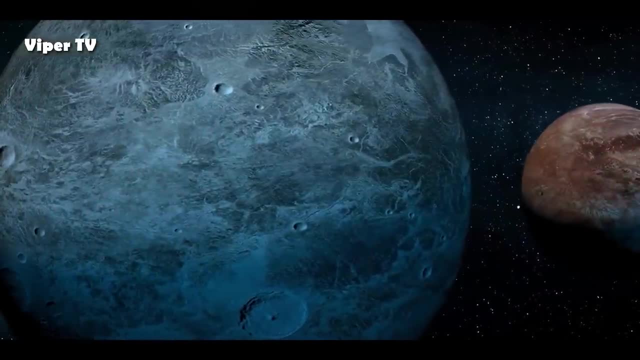 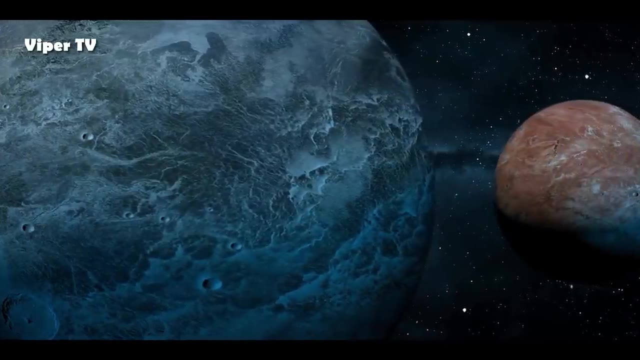 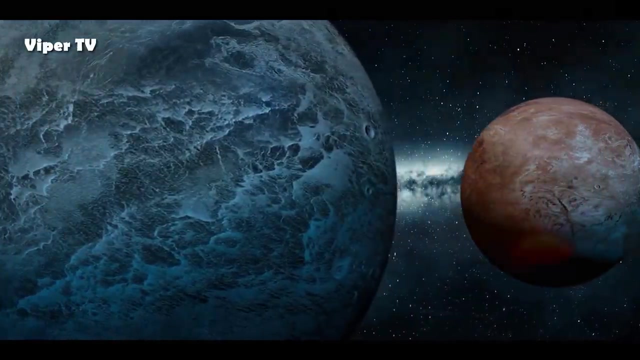 today, it's hard to imagine the planets in any orbit other than our night sky. they feel eternal, permanent, and so it's natural to think of the solar system as a piece of celestial clockwork, a mechanism running with perpetual and unchanging precision, marking out the passage of time in time frames that we 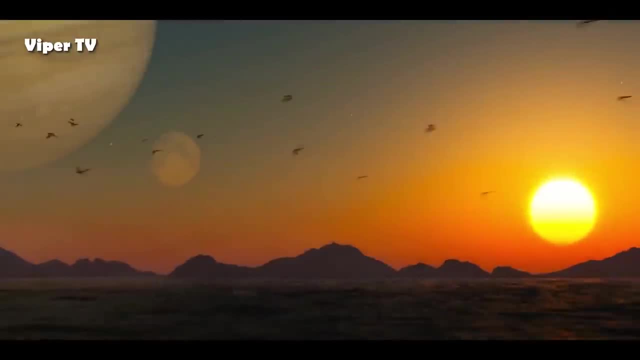 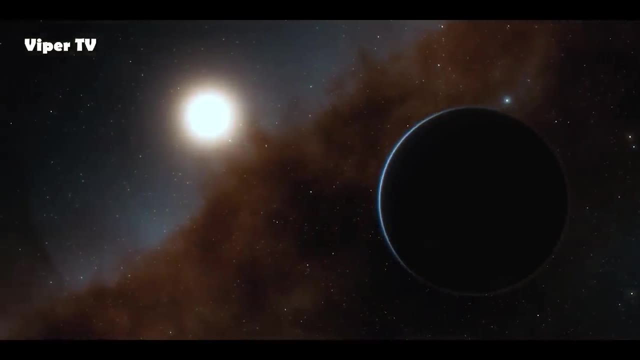 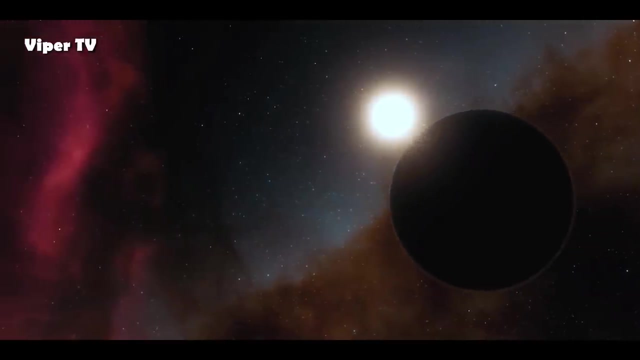 can comprehend days, weeks, months and years. the motion and trajectory of the planets is just that clockwork. we use these markers to plot out the 24 hours of a day, 365 days of a year, and the lunar cycle is, of course, intimately linked to our months beyond. 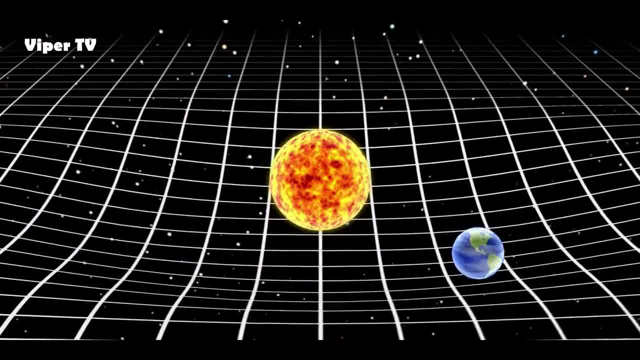 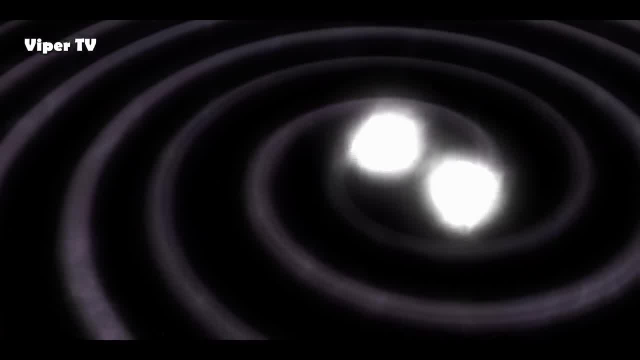 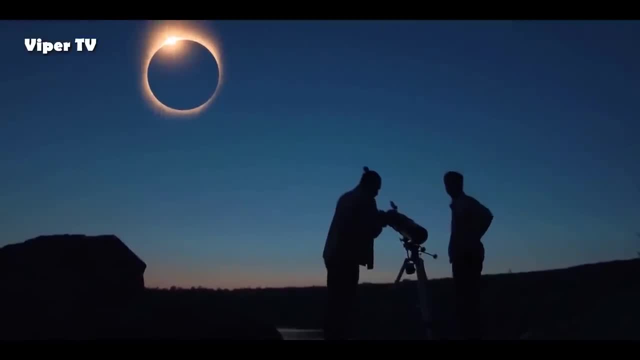 that Newton's laws of universal gravitation, first described in 1687, allow us to this day to plot out the trajectories of all the heavenly bodies far into the future and back into the distant past. this predictability of motion is what allows us to plot great astronomical. 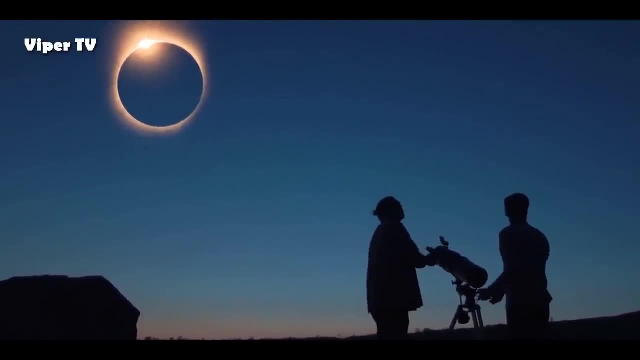 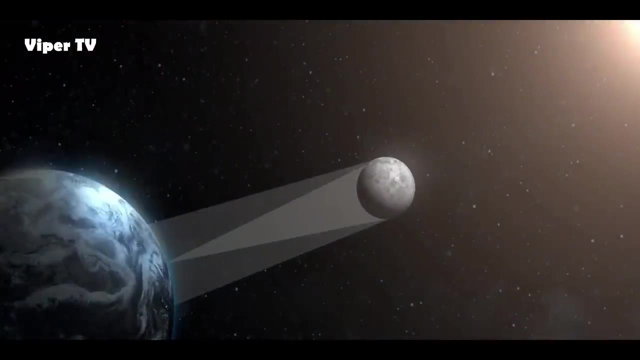 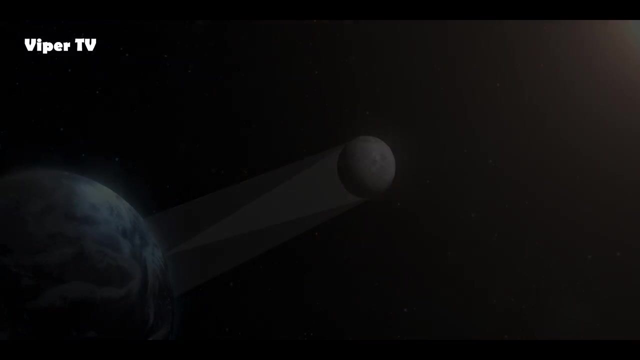 events such as eclipses and transits far into the future. for example, we can predict that on the 14th of September 2099 the Sun, Moon and Earth will be in precise alignment to create the final total solar eclipse of the 21st century across North America. but 100 years ahead or behind us is 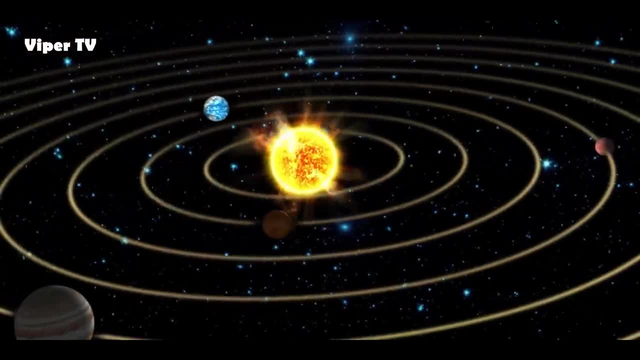 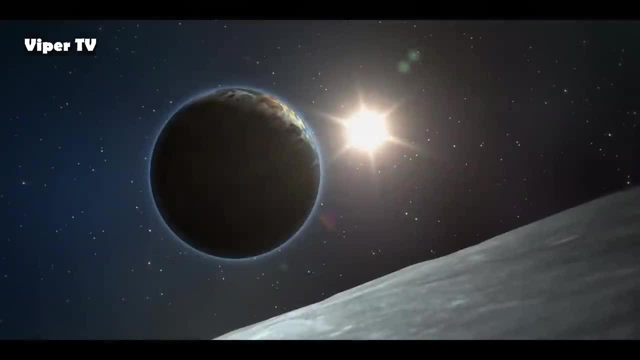 nothing more than a proverbial blink. in terms of the life of the solar system and over longer durations, the clockwork becomes a lot less reliable. if there was only one planet orbiting one star, for example, if Mercury was the orphan child of the solar system, we would be able to. 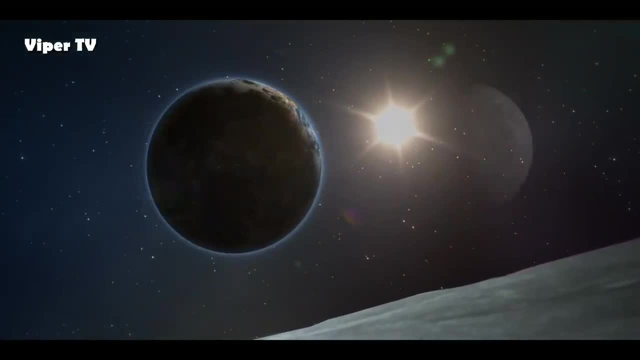 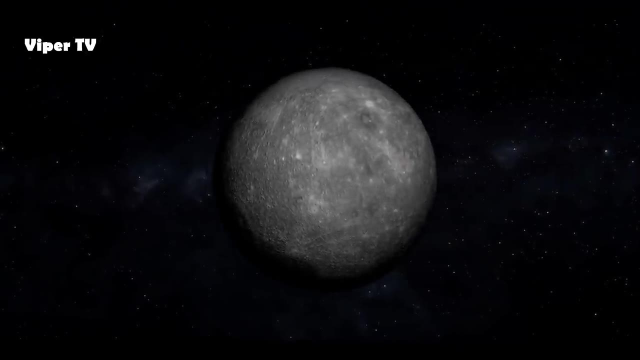 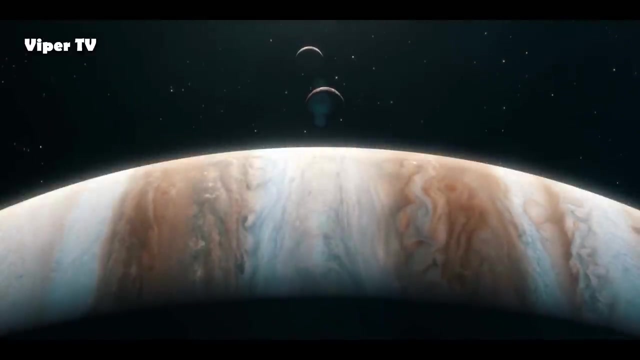 calculate precisely the gravitational force between Mercury and the Sun and to plot Mercury's orbit around the Sun with essentially infinite precision. but add one more planet into our rather vacant imaginary solar system. let's say we make it Jupiter. so there is now a gravitational force between all. 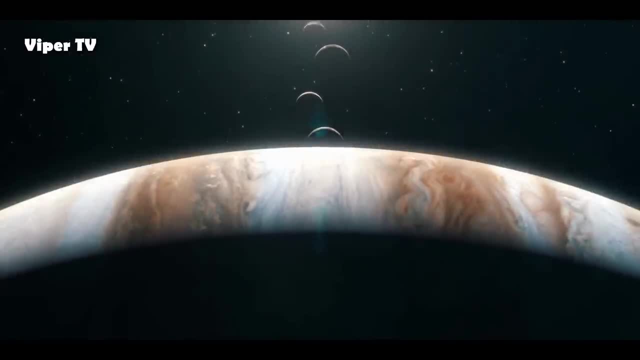 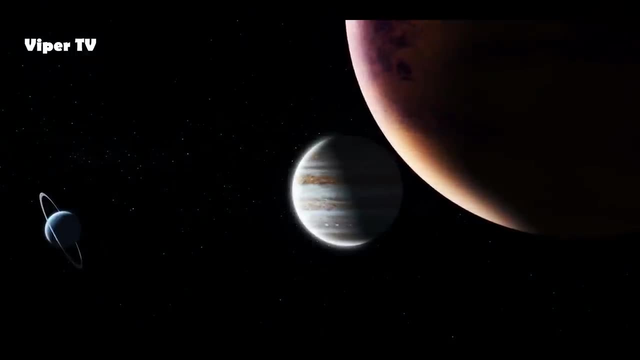 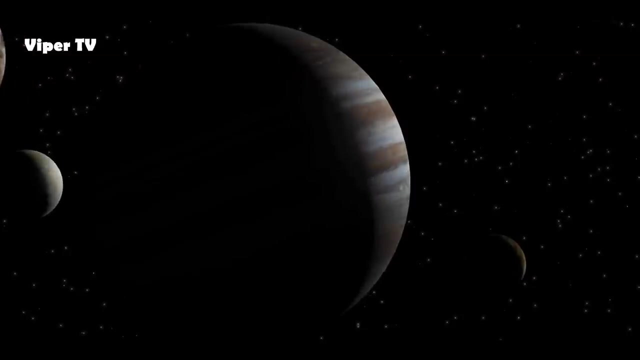 three objects- the Sun, Mercury and Jupiter- and it's no longer possible to calculate exactly where they're all going to be in the future or where they were at some point in the past. when there are more than two objects in play at any one time, you have what physicists call a chaotic system. it 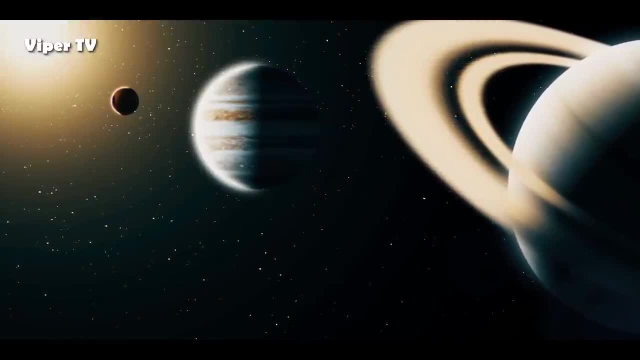 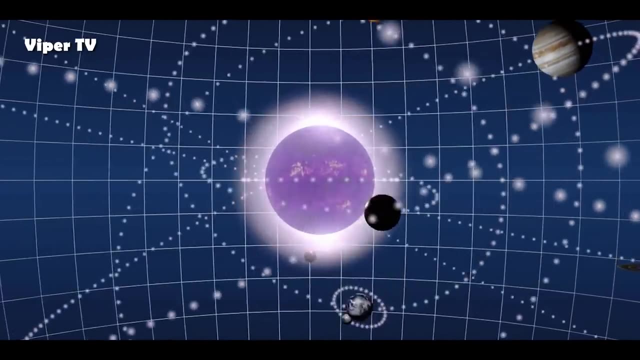 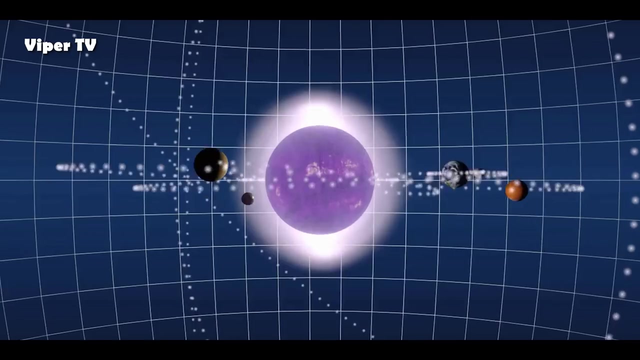 means the planets can push and pull one another, moving entire orbits in ways we simply cannot predict. so the further we look back in time, the less certain we are of the position of any of the planets. our mathematics fails, so instead we have to rely on circumstantial evidence. 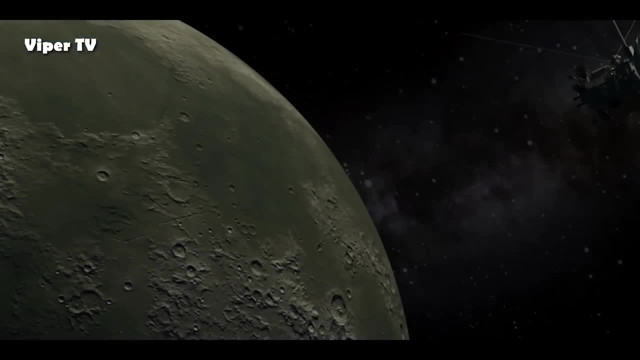 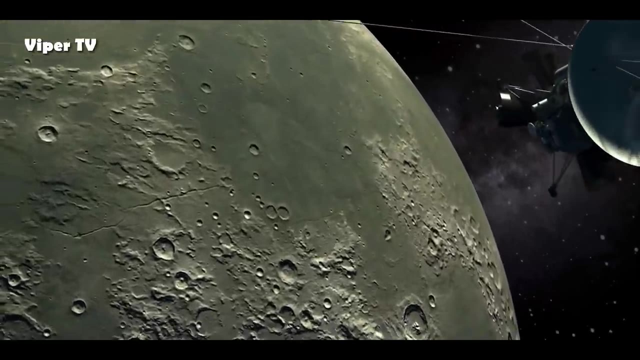 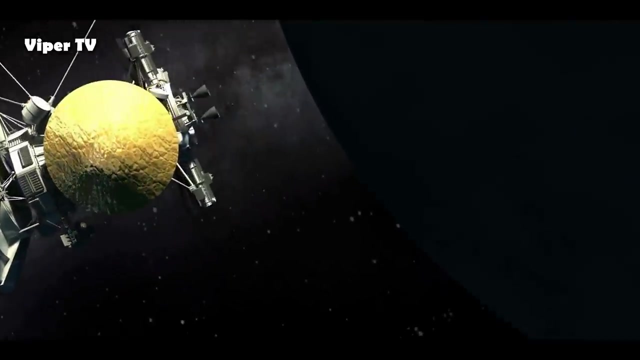 to piece together a picture of the past. in the case of Mercury, it's the evidence from messenger detailing the levels of volatile elements like potassium and sulfur that enable us to begin to understand the early life of the planet and infer that Mercury must have begun life further out in the solar system. 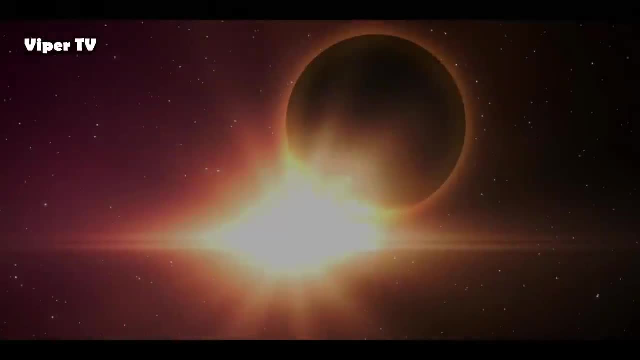 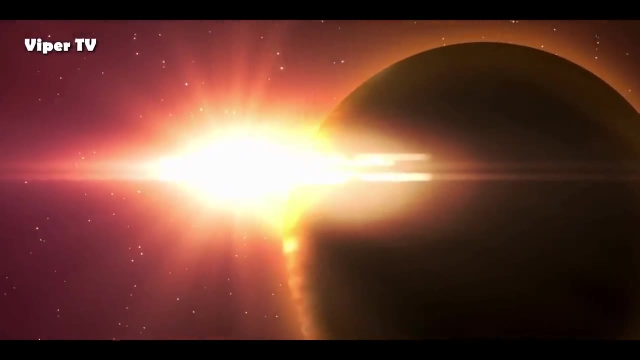 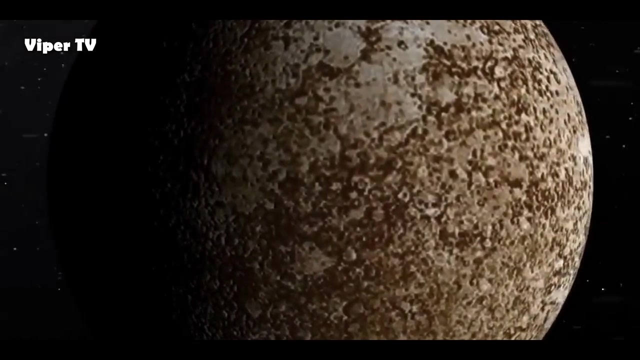 than it finds itself today. so what happened next? how did a planet that began its life in the sweet spot of the solar system end up in the scorching interior? the answer lies in the other clue messenger confirmed for us: Mercury's massive iron core. relative to its size, mercury has the most massive. 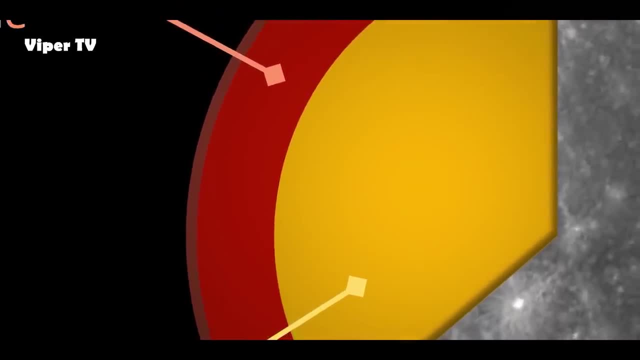 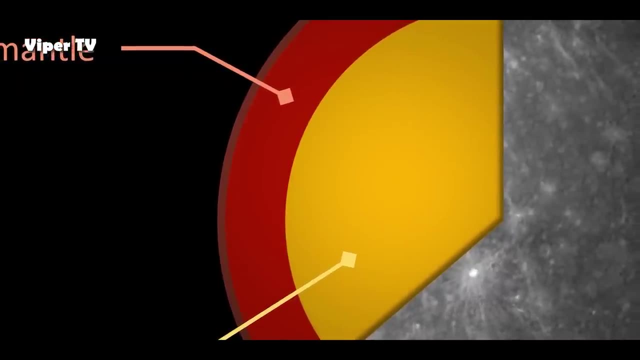 core of any of the rocky planets. seventy-five percent of its diameter and almost half of its mass is molten iron, compared to around just a fifth of the mass of the earth. we suspected the oddity of mercury's composition for well over a hundred and fifty years. 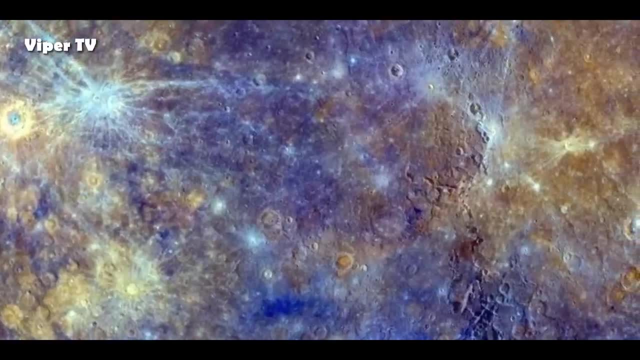 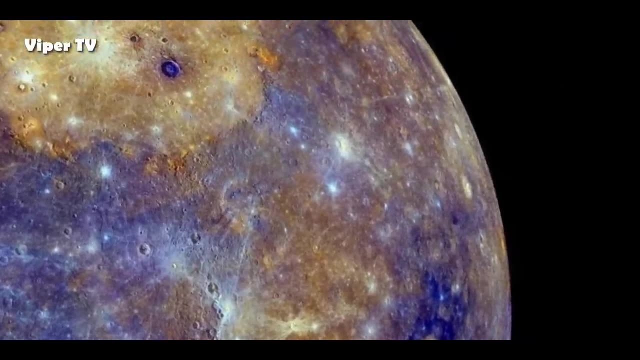 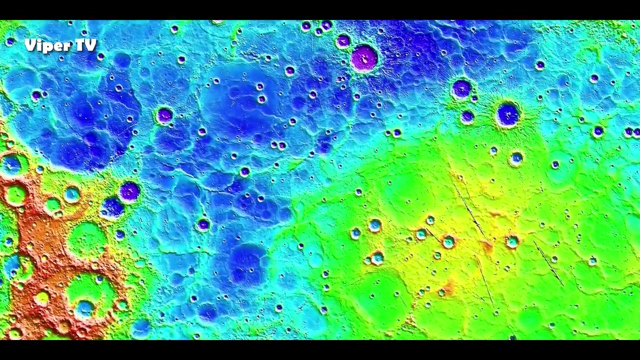 and that's because of some brilliant deduction by a German astronomer called Johan Franz anchor, who determined the mass of mercury by measuring the gravitational effect it had on a passing comet, a comet that we now call, unsurprisingly, comet anchor. with an approximation of the planet's mass, we 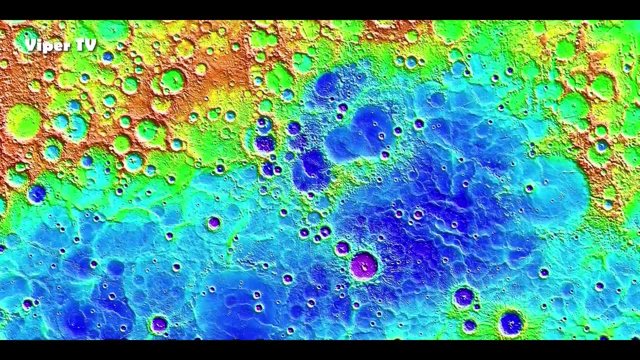 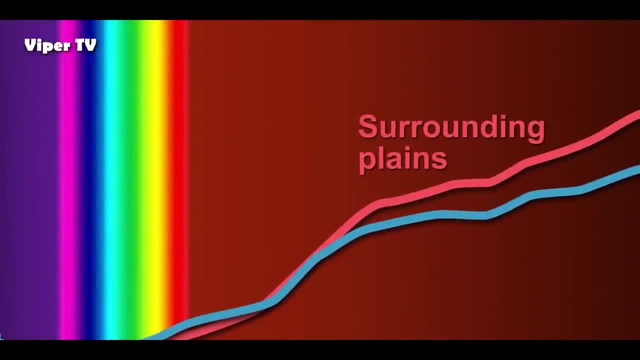 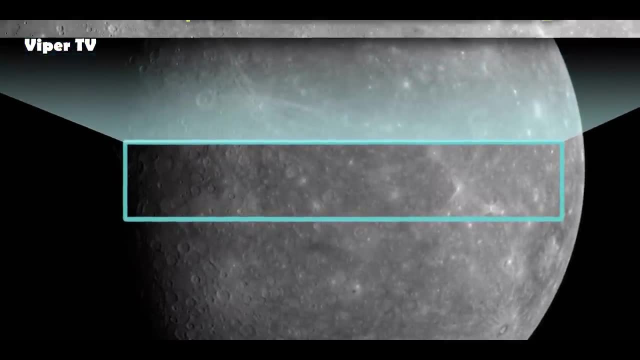 are able to calculate the density of the planet and with that calculation approximate its composition. so we've known for some time that mercury is odd, but only with the arrival of messenger did we begin to reveal just how odd the smallest planet actually is. by accurately measuring mercury's magnetic 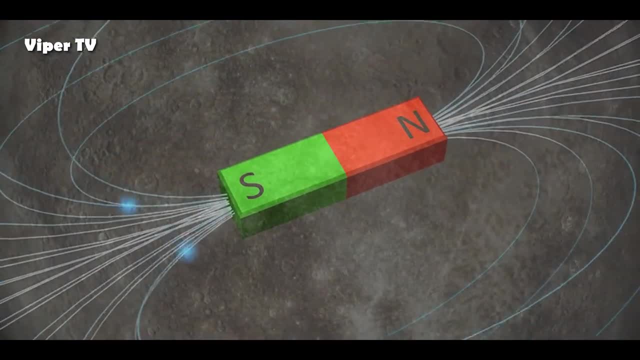 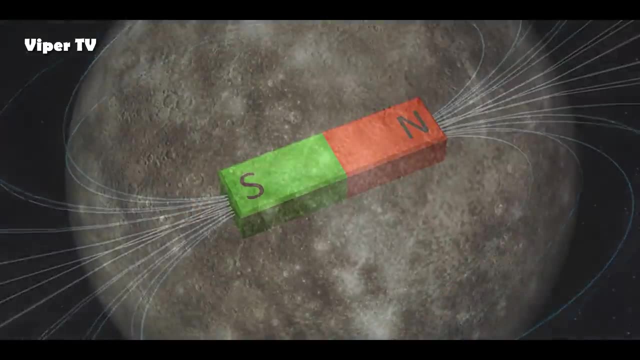 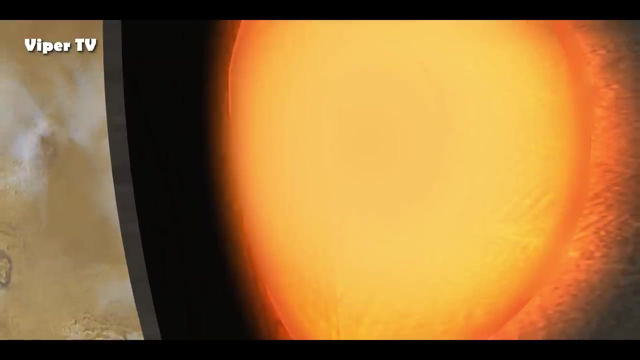 field, we've been able to confirm that, far from being a geologically dead planet, mercury has a dynamic magnetic field driven by an internal force, indicating that the core is at least partially liquid. this goes against the conventional thinking of planetary dynamics, because we would expect a planet as small as mercury to have lost its magnitude. 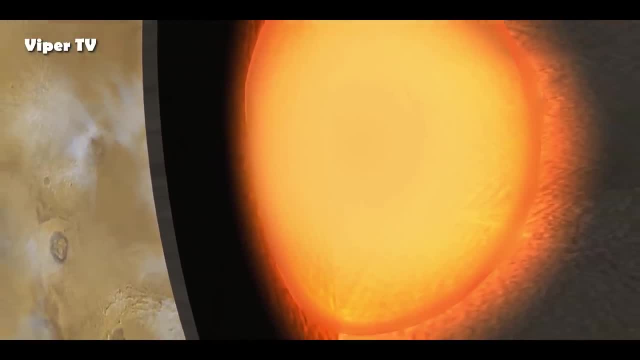 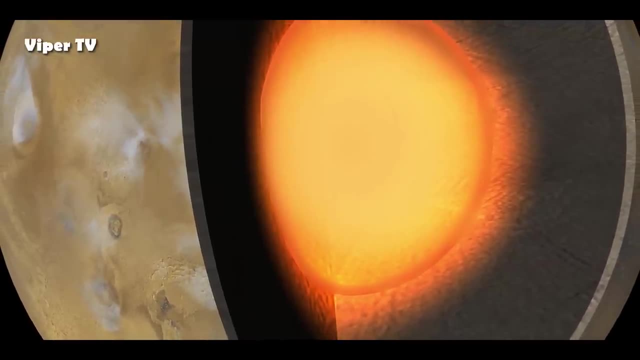 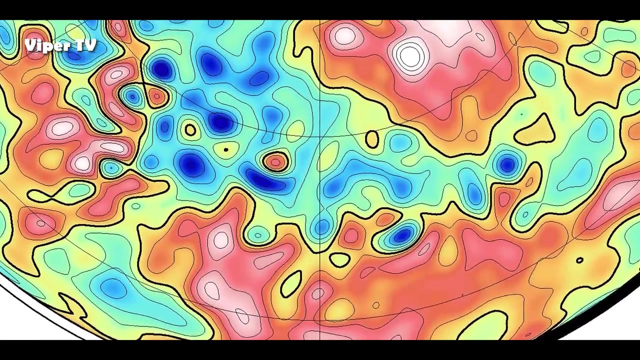 lost its internal heat long ago, Just as Mars lost its heat because of its size. we would have expected the core of Mercury to have cooled and solidified, but MESSENGER's data proved otherwise By combining precise measurements of Mercury's gravity field with the extraordinary mapping. 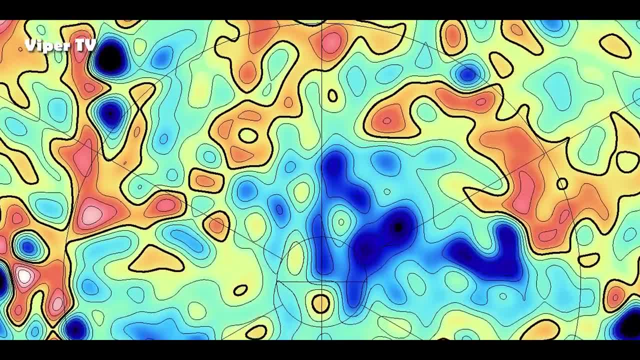 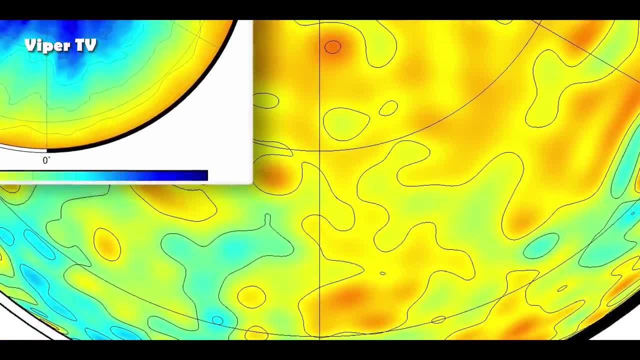 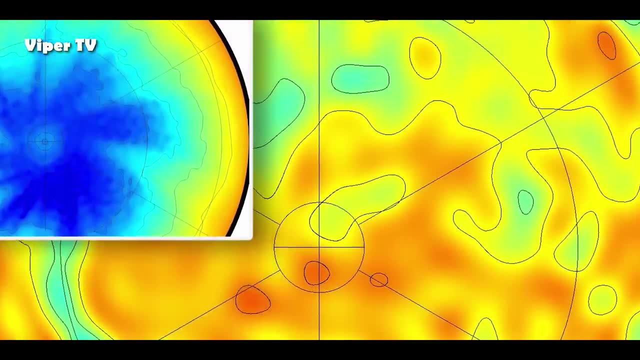 of its surface, MESSENGER found that Mercury's structure is unique in the solar system. It appears to have a solid silicate crust and mantle above a solid layer of iron sulphide which surrounds a deeper liquid core layer, possibly with a solid inner core at the centre. 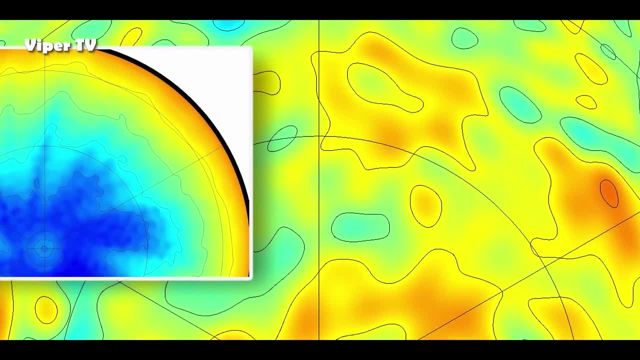 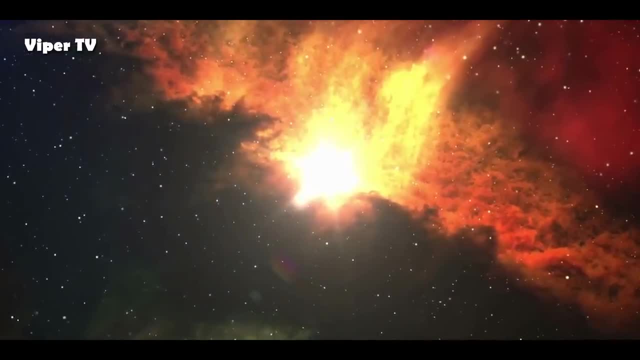 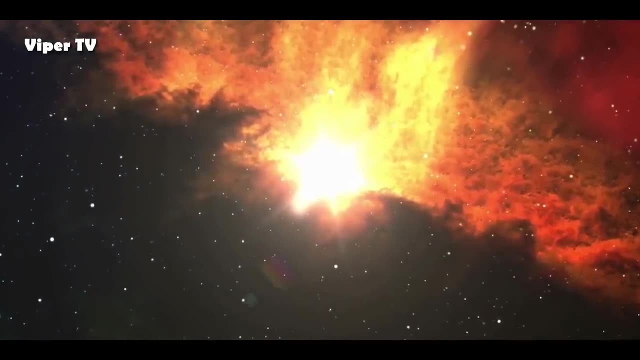 of the planet. This challenges all the theories about its formation. Four and a half billion years ago, we know that the inner solar system was in turmoil. In the middle of it all, the newly born Mercury found itself orbiting far out from today's 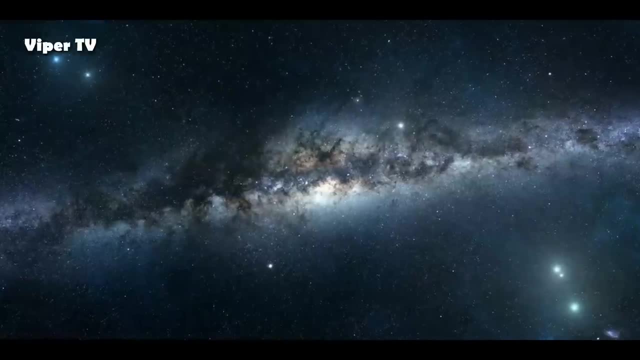 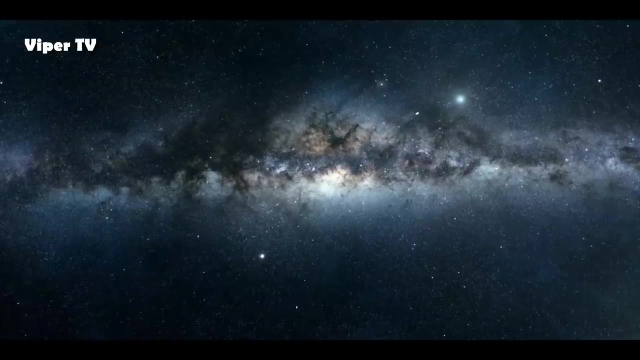 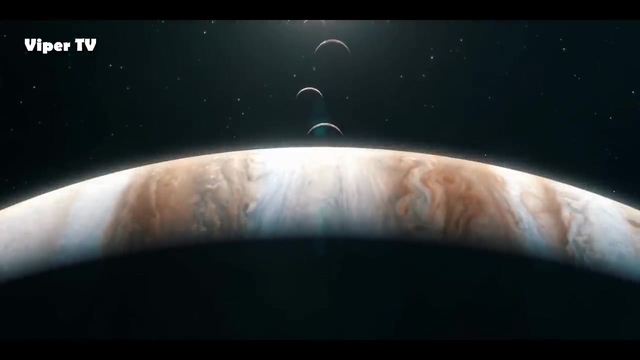 intimate proximity with the Sun, surrounded by rocky debris and scores of planetary embryos all jockeying for position. The young solar system was still a place where planets could live or die. But it wasn't just the rocky planets that found themselves disturbed. Jupiter, the largest and oldest of all the planets, was on the move. 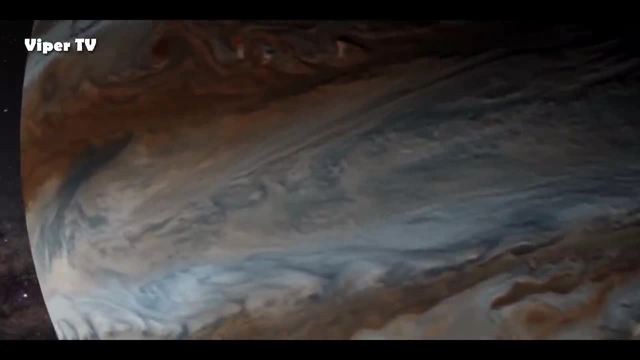 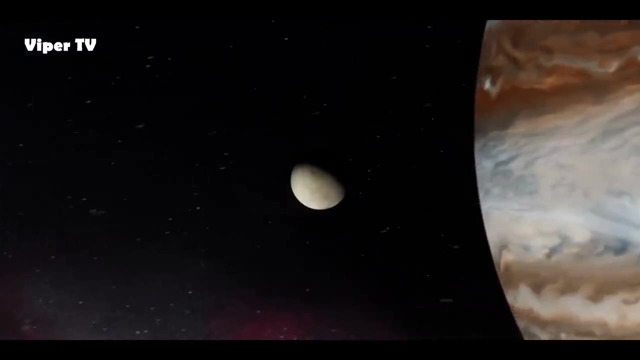 And when a planet of that size shifts its position, there are almost always casualties. But for now, all we need to know is that the ever-evolving MESSENGER system is still in the process. But what's more interesting is that the evidence suggests that the juvenile Mercury was kicked. 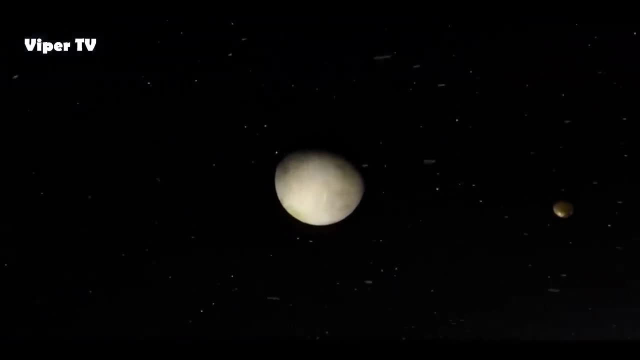 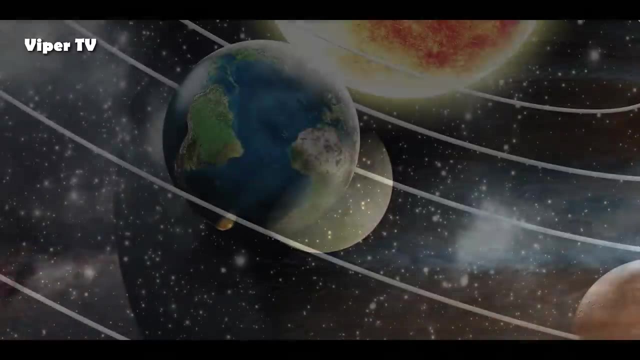 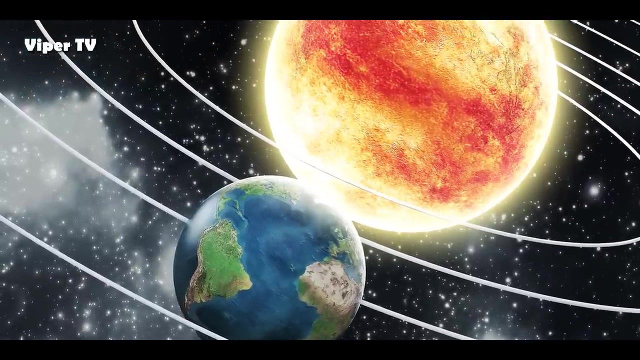 by the gravitational force of Jupiter on an inward trajectory, finding itself flung in towards the Sun and into the path of danger In the crowded orbits of the early solar system. such a change of course was fraught with danger, And all of the evidence indicated that this was the most violent and defining of turns. in Mercury's history. As the planet swerved inwards, it collided with a 9.7 trillionth of a second-largest planet into another embryonic world and shattered. Today we see the evidence of this ferocious collision in the strange structure of this tiny planet. 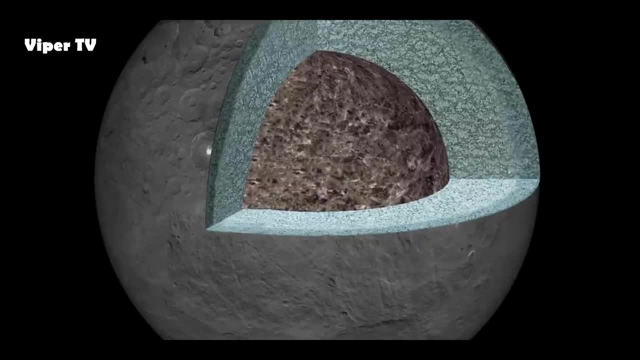 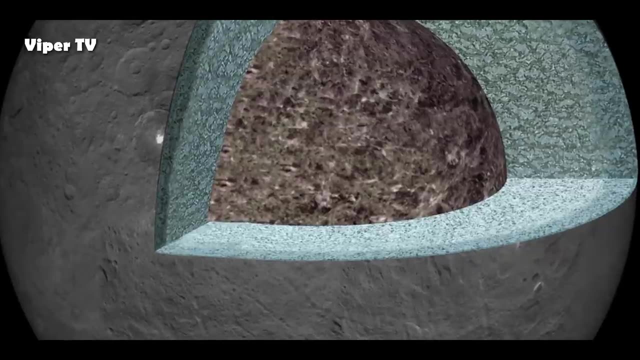 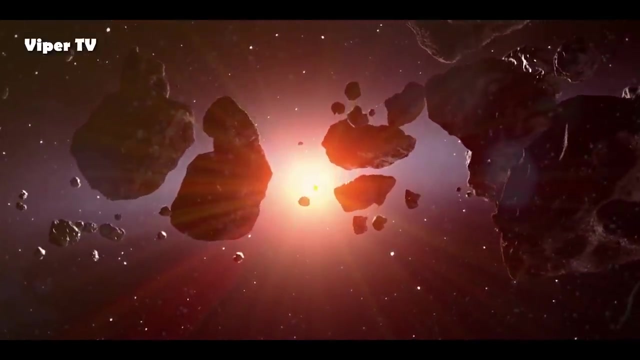 A giant core has been left behind The exposed interior of a planet that had much of its outer layer, its crust mantle, stripped away and lost to space in the aftermath of the collision. This collision not only transformed the physical characteristics of the planet, but also knocked Mercury further inwards. 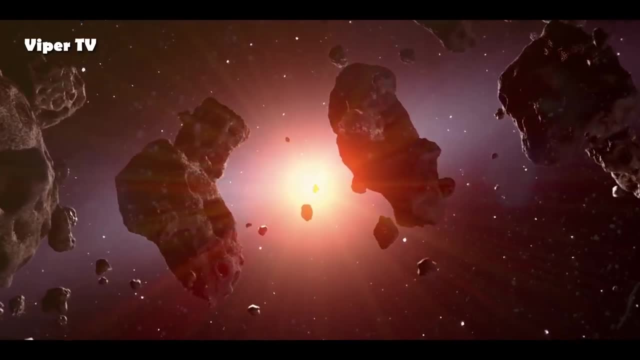 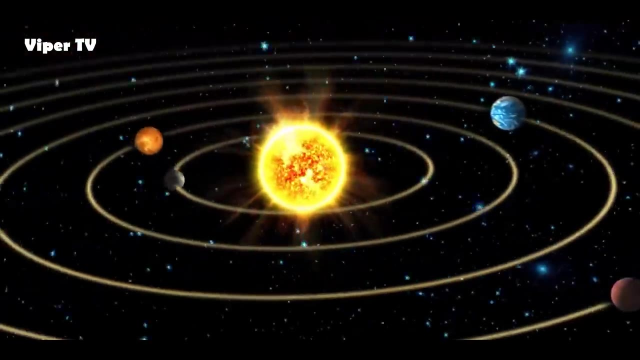 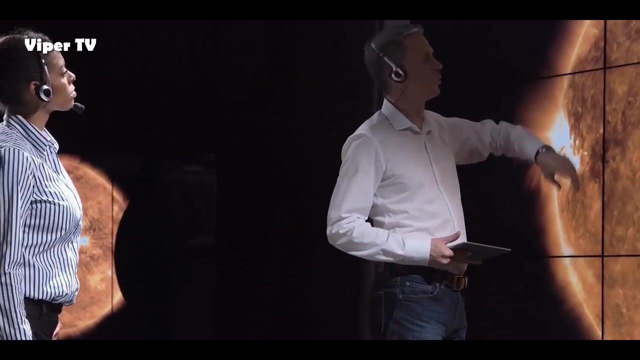 on a lopsided trajectory that we see reflected in the most elliptical orbit of all the planets. Although we cannot be certain of these events, it's a brilliant piece of scientific deduction. to use the evidence, we have to create a plausible scenario of events that happened unimaginably long ago. 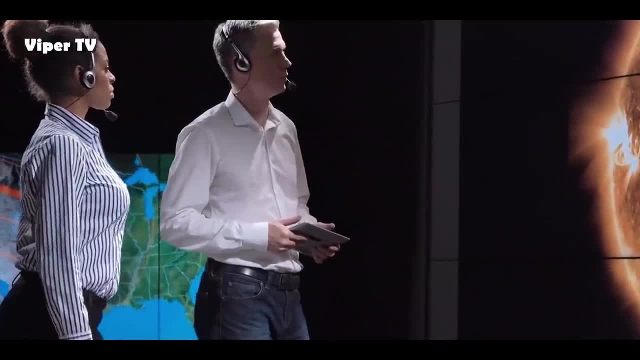 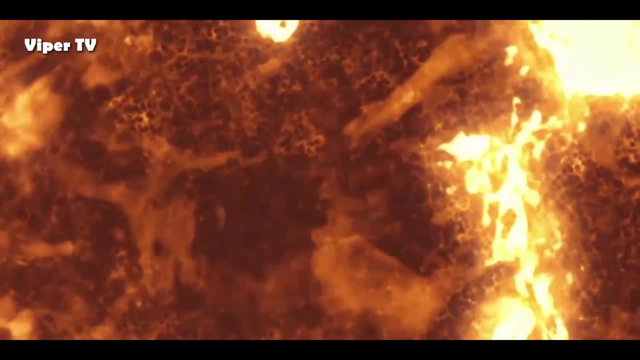 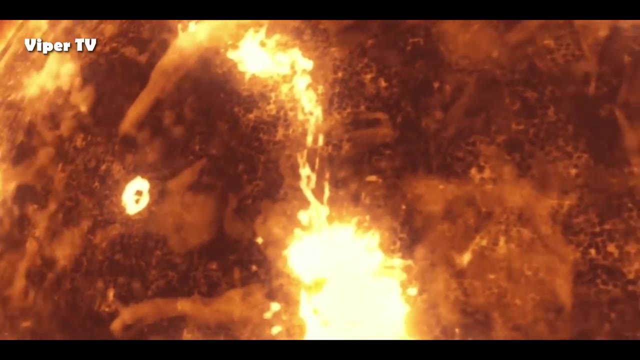 Events that drove the first rock from the Sun from a position full of potential to a place much too close to the Sun to support any form of life. An opportunity lost. After four years of observation and its brilliant discovery of Mercury's ancient past, MESSENGER finally ran out of fuel on 30 April 2015. 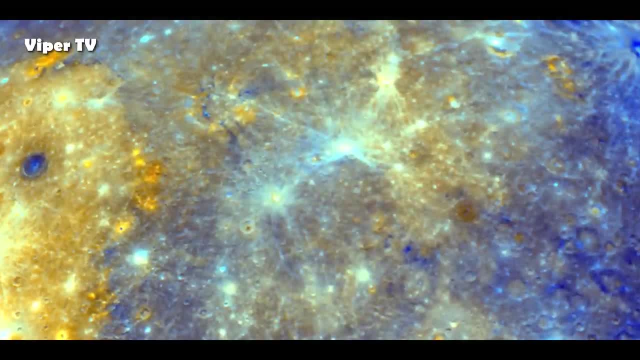 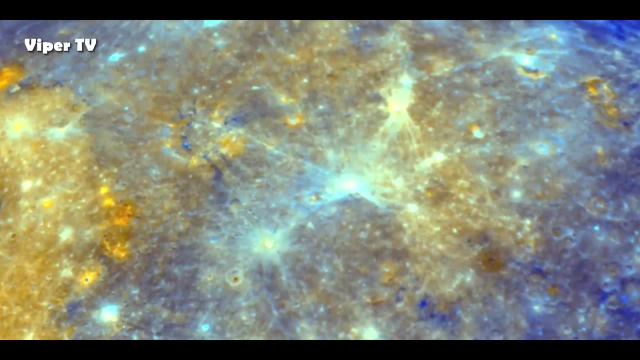 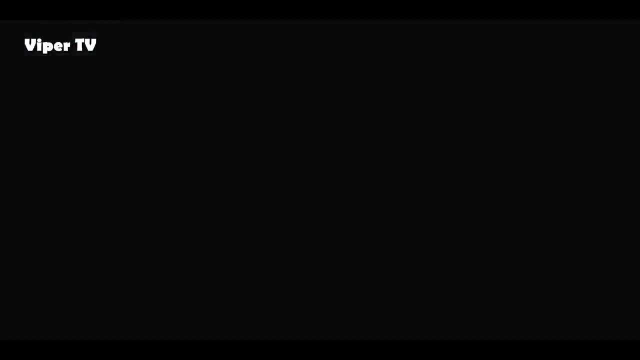 and added yet another crater to this tortured world that once held such promise. Shrouded in an unbroken blanket of cloud, the next rock from the Sun tells of a very different story. Over 50 million kilometres beyond Mercury lies a world that, at first sight, has the potential. 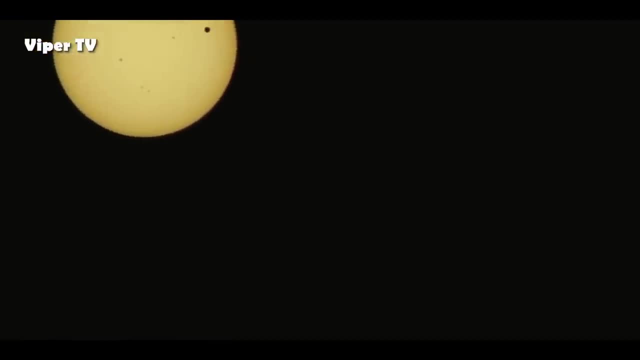 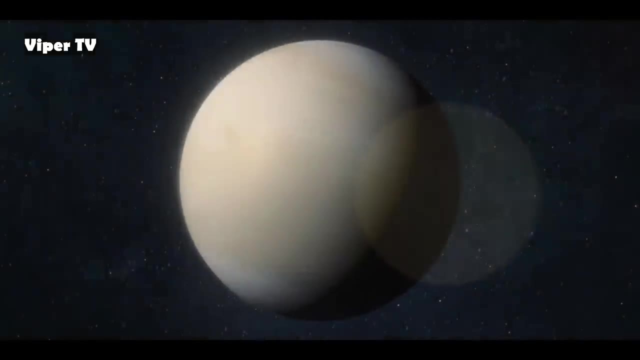 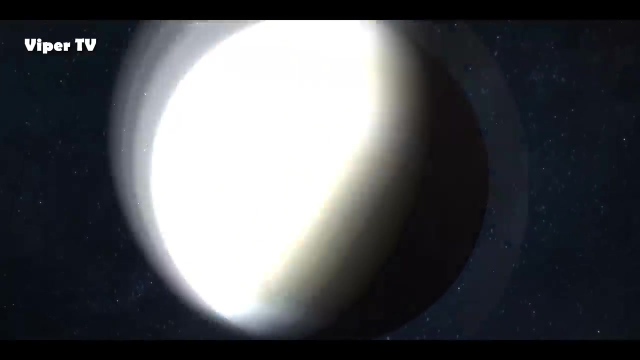 to be far more Earth-like than her scorched inner companion. Venus is perhaps the most mysterious of all the planets Lying on the inner edge of the so-called habitable zone. this is a planet that holds its secrets close. For centuries, it has teased us with its brightness. 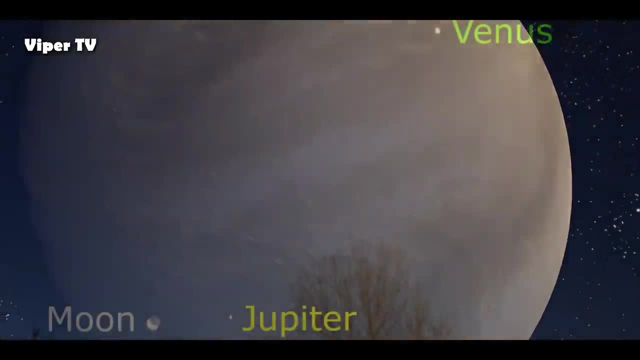 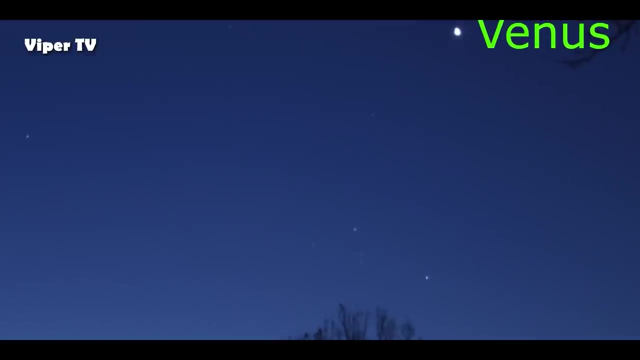 in the early morning and early evening sky. It's so bright because it's a large planet, about the same size as the Earth. It's not too far away from us either, and the clouds that shroud it are highly reflective, reflecting three-quarters of the light that hits them. 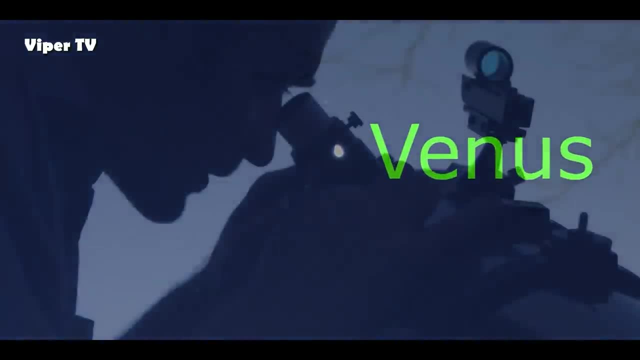 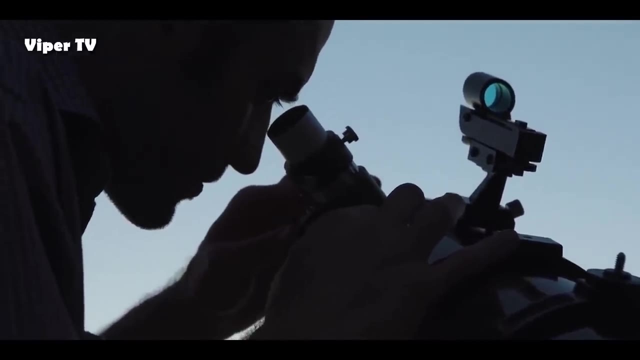 That's the frustrating but tantalising thing about Venus, because even when you look at it through a big telescope, it is featureless. You never see the surface, which means that until the 1950s, scientists could only speculate about what lay beneath. 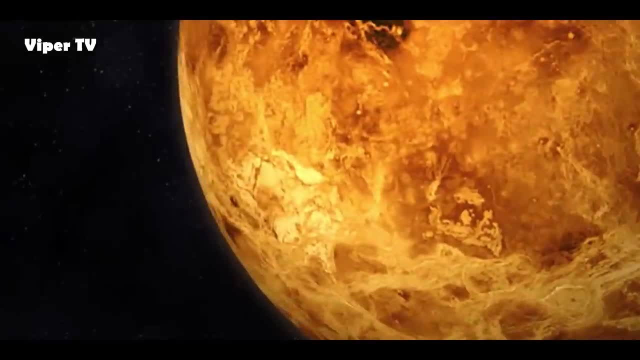 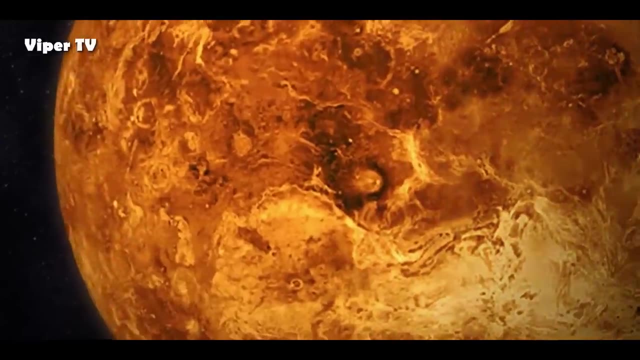 In the late 90s and early 20th centuries, many thought that beneath her clouds, Venus was hiding a mirror world to Earth, if not home to complex sentient life, then certainly hosting basic life forms. Faced with that impenetrable cloak, 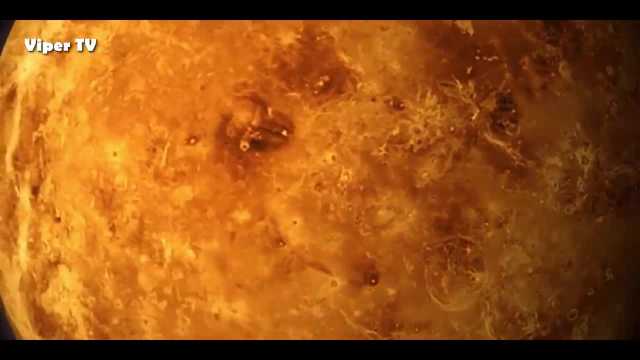 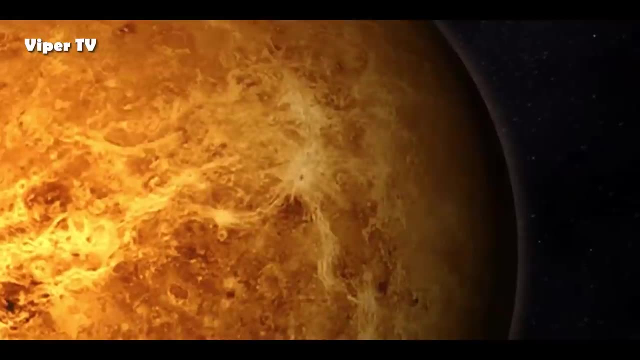 our collective imaginations fuelled the idea of a living, breathing world beneath the clouds, a shroud that meant for the first half of the 20th century. we lived convinced that we were far from alone in the solar system, As with almost all of our understanding of the planets. 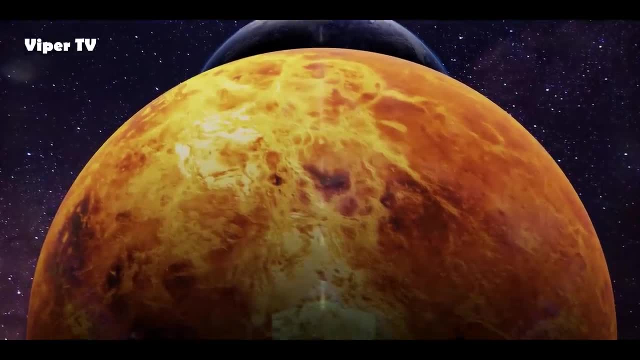 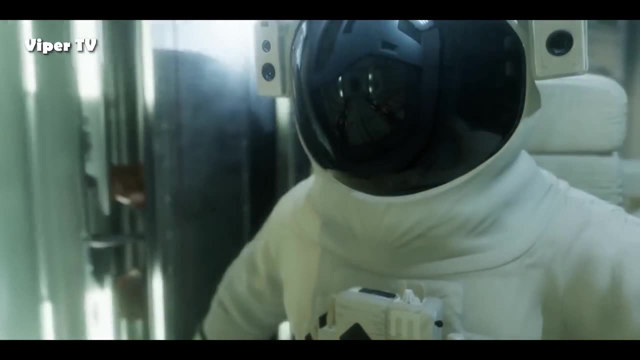 the evidence that built this picture has been accumulated through decades of exploration, starting with the Venera mission's first touchdown on the planet, to the pioneer Venus orbiter and to the more recent Magellan mission, which not only relayed extraordinary radar soundings, 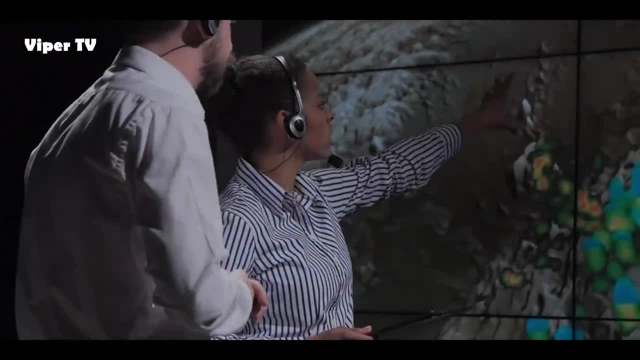 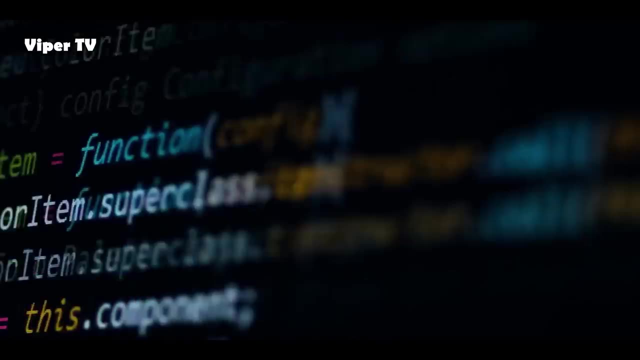 of the surface of Venus, but provided the first full topographical map of the planet, collated over a period of four years in orbit. Combining all this, all of the data that has been accumulated over decades of exploration, has allowed us to peer deep into the planet's past. 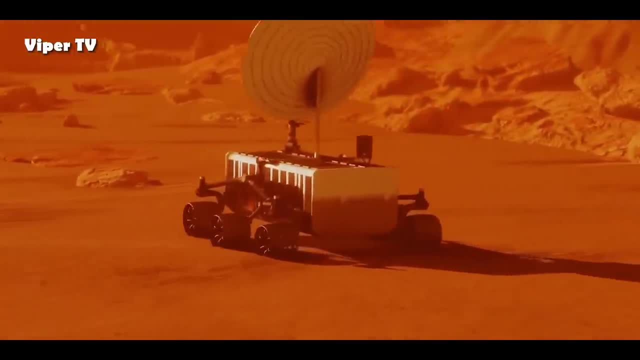 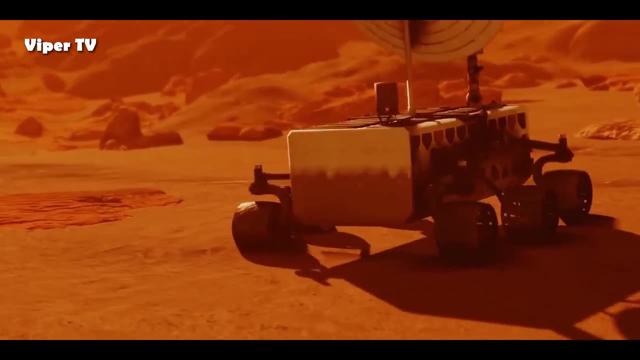 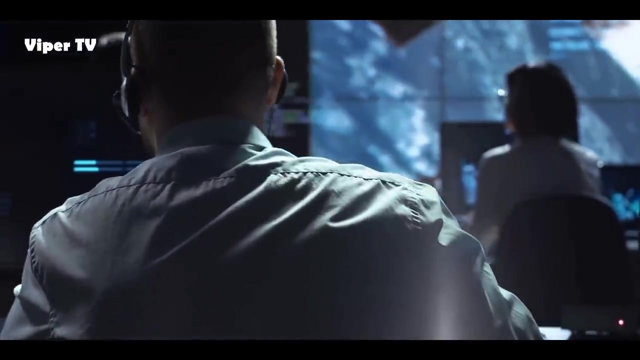 using the same tools that enable us to model the future of climate change here on Earth, to create climate models of Venus in the past, present and future. The results of this analysis, conducted most recently by a team from NASA's Goddard Institute for Space Studies, GIS. 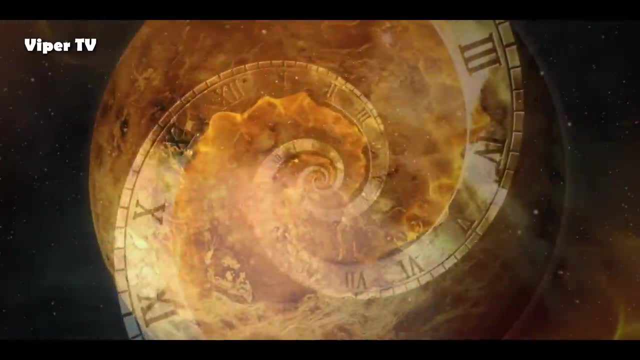 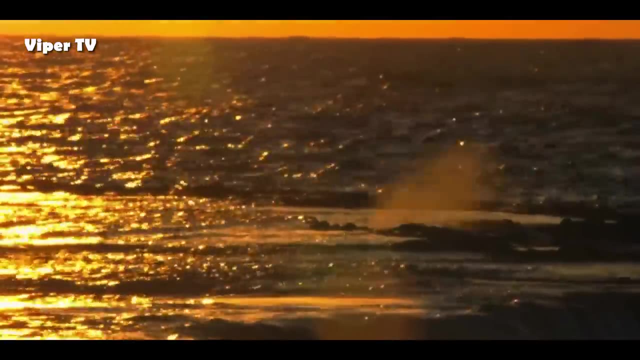 all point to the same conclusion: In the distant past, Venus was a planet covered in shallow primordial oceans. Some estimates suggest that this water world was far from fleeting, a blue planet just like our own that could have been sustained for around 2 billion years. 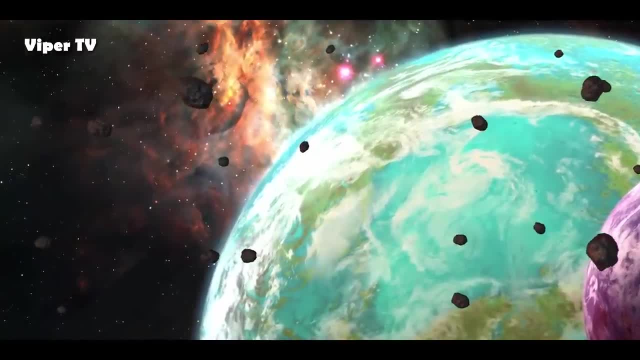 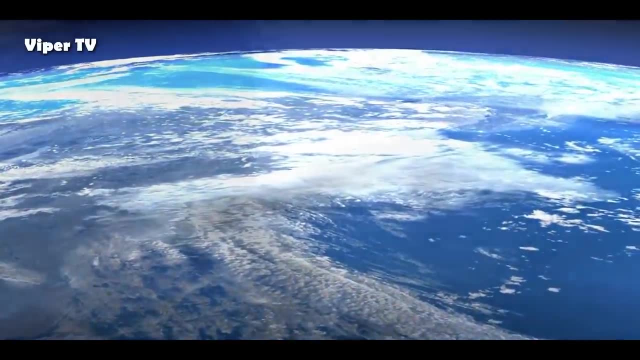 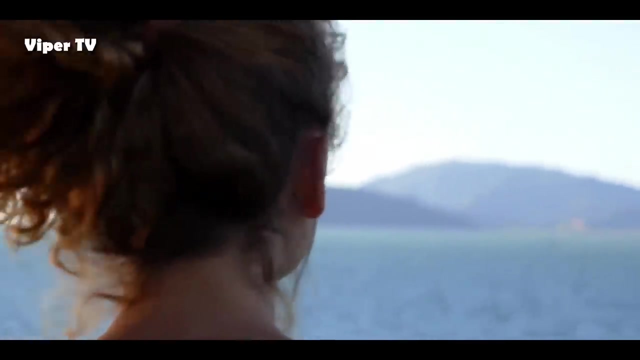 and perhaps only disappeared some 700 million years ago. It's a tantalising thought that such a similar world to our own existed for so long, with liquid water on its surface. We know life took hold quickly on our own blue planet, within half a billion years of the Earth being formed. 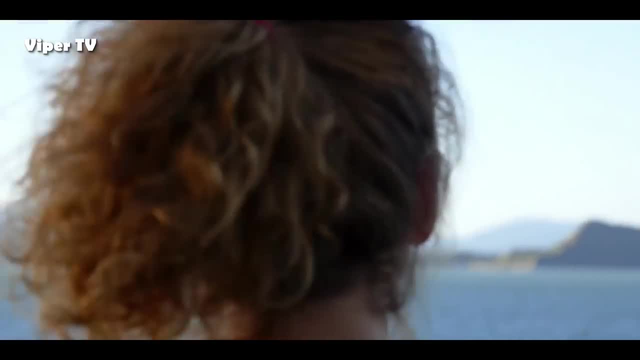 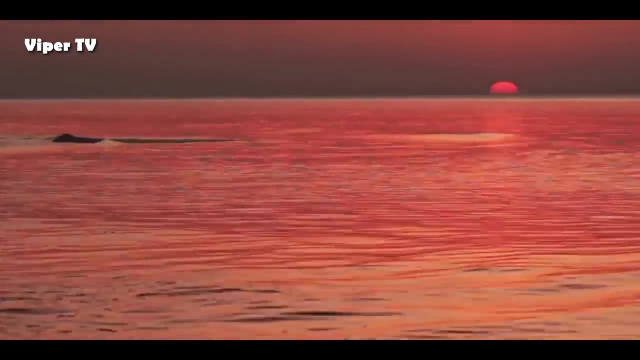 So there seems good reason to suspect that if Venus really was as wet as the models predict, it too could have sprung into life. Exactly what went on in the long-lost rivers and oceans of Venus is yet to be discovered, Hidden behind the clouds. 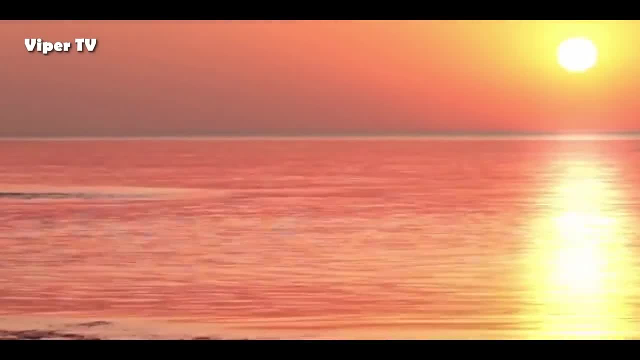 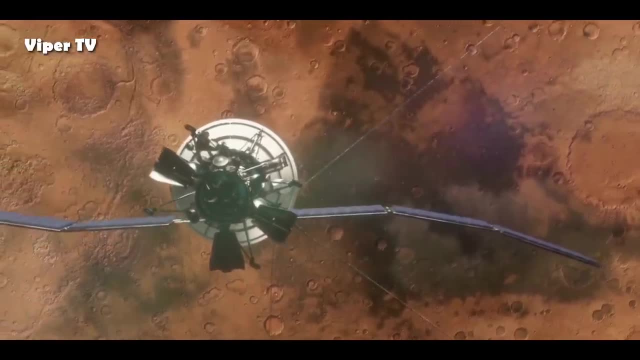 we have not yet been back to search for any signs that life ever took hold here. Our exploratory attentions have turned to Mars as a planet that not only has a fertile past, but is also a possible target for human colonisation in the future. 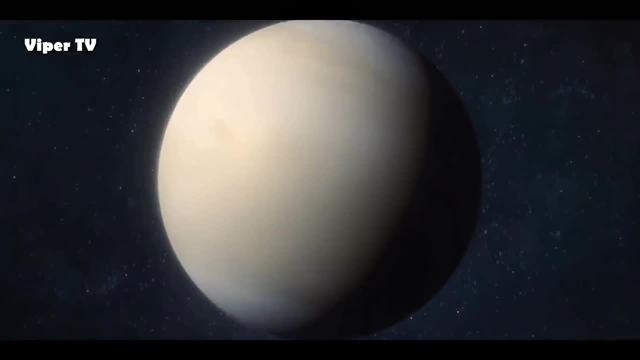 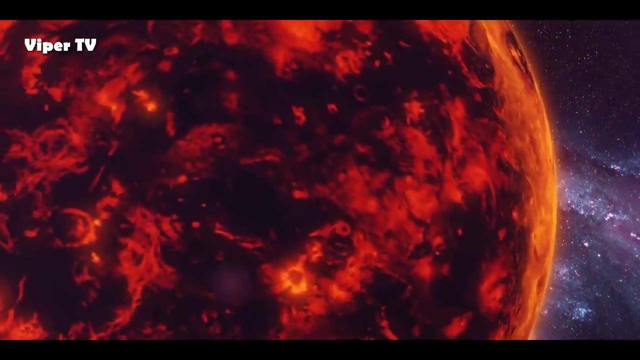 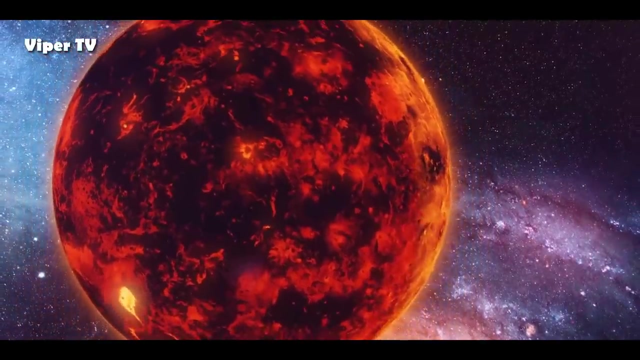 We know for certain that no life, at least no life we understand, could exist on Venus today, And perhaps even the evidence of any biology on that long-lost water world has long ago vanished under the oppressive heat, rampant volcanism and extreme pressures of the planet today. 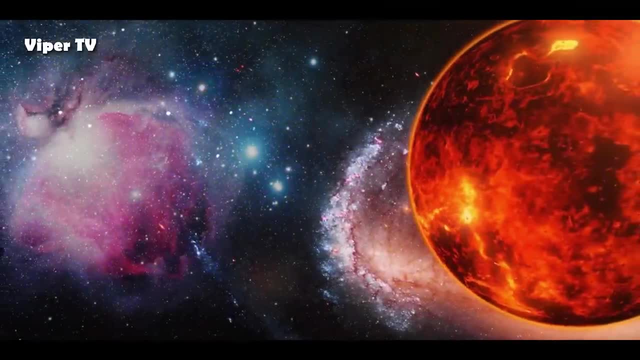 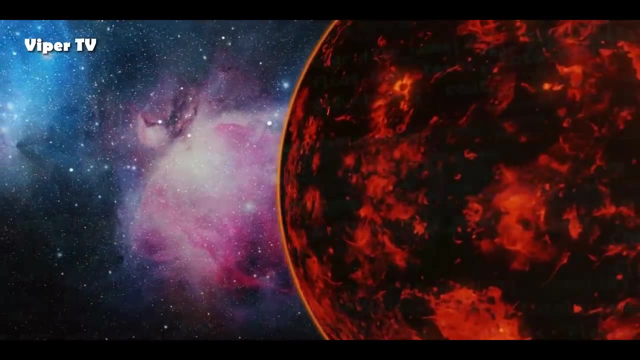 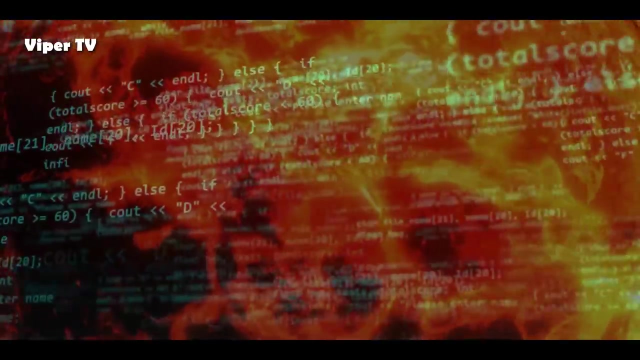 Despite multiple failures, the Soviets didn't give up And in October 1967, Venera 4 entered the atmosphere of Venus and sent back data supporting the Earth-based observations, revealing for the first time that the blanket of clouds surrounding Venus was made up of primarily carbon dioxide- 90 to 95%. 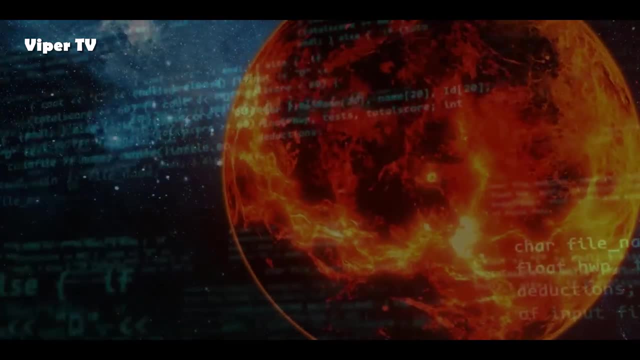 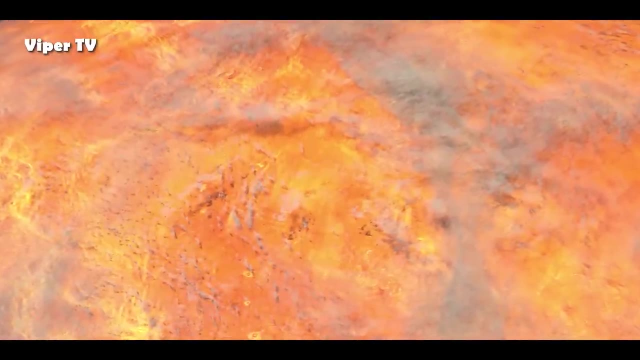 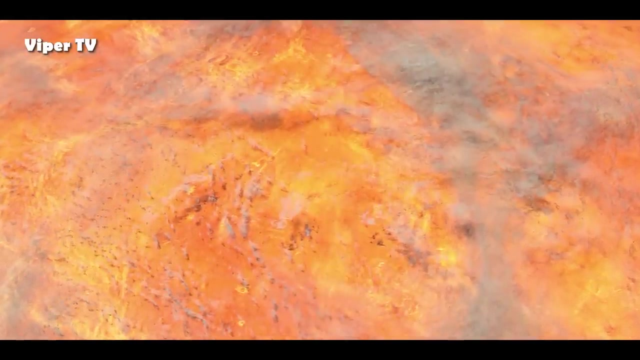 3% nitrogen and just trace amounts of oxygen and water vapour. Venera 4 confirmed beyond all doubt that this was no second Earth. As it descended through the thick clouds, the temperature rose to 262 degrees Celsius. The atmospheric pressure increased to 22 standard atmospheres. 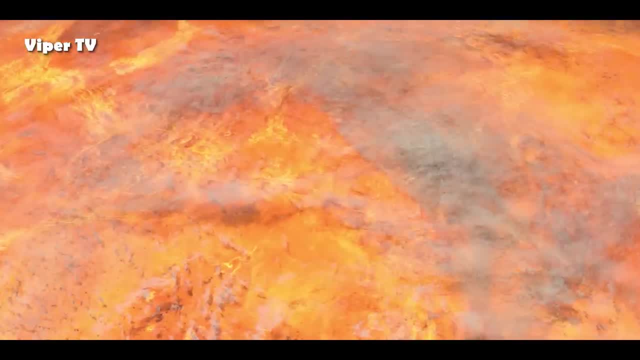 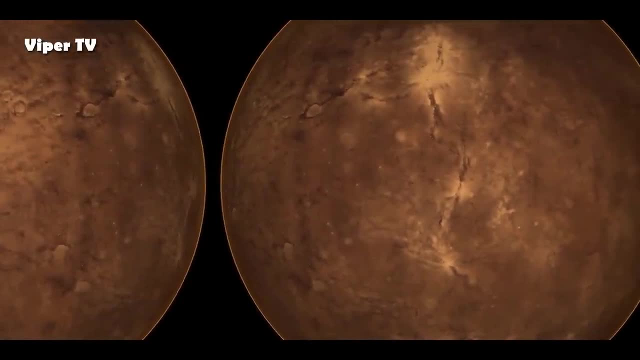 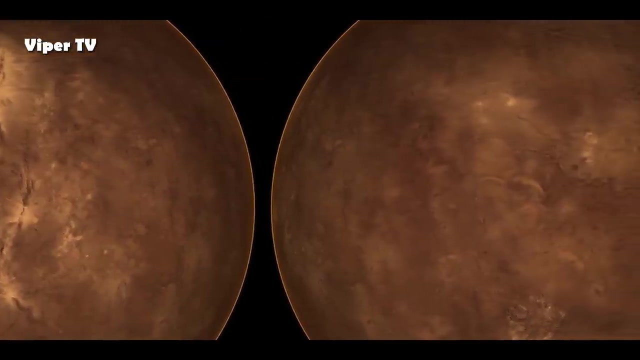 2,200 kPa, And this was still 26 kilometres above the surface. As Venera 4 parachuted its way down to the surface, it provided data to Earth while confirming its own imminent death. This was a spacecraft that was not designed to survive. 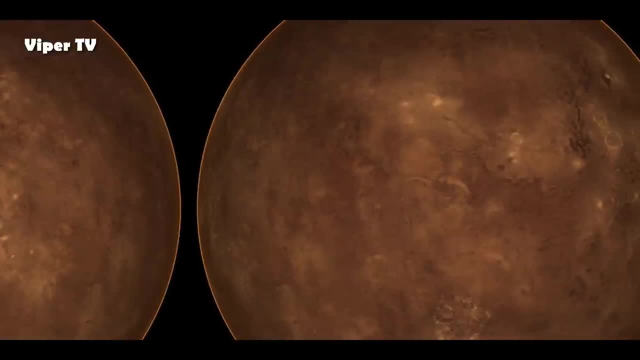 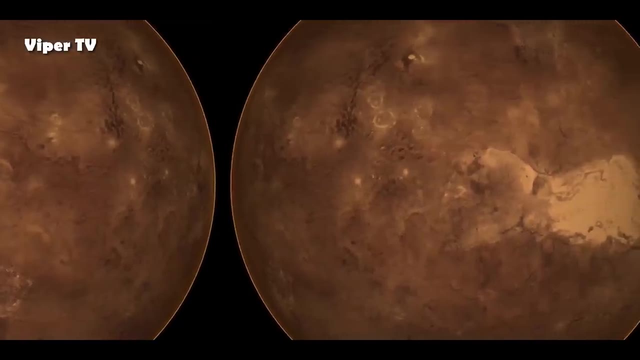 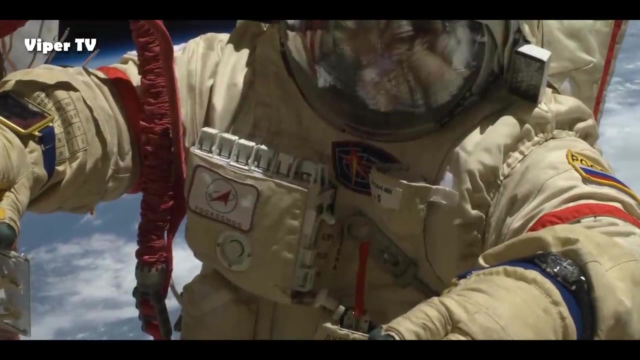 the intense pressures and temperatures it was measuring, Let alone the lack of the water landing it was designed for. The craft failed during the descent and was lost long before it reached the surface. Gradually, through the following missions, the Soviet scientists began to overcome. 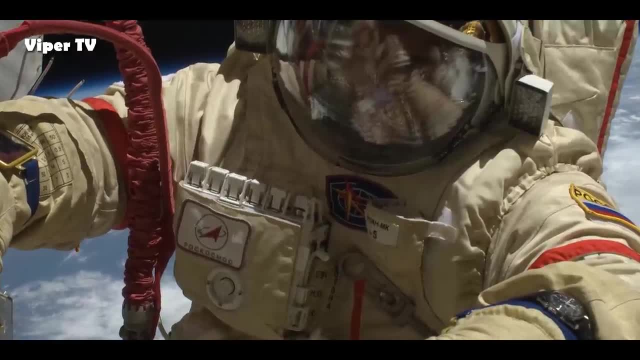 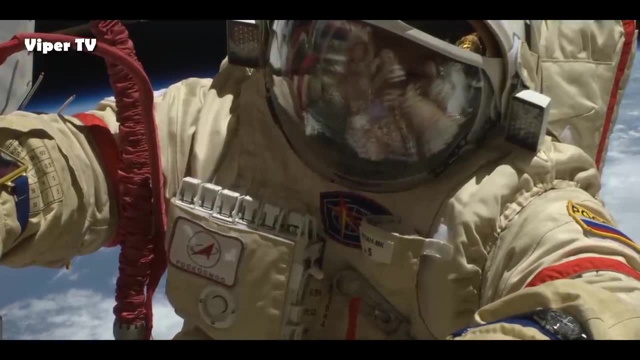 each and every challenge Venus put in front of them. Venera 7 was built to survive the most violent of landings And, even though its parachute failed, it made it to the surface intact in 1970, and was able to use its damaged antennae. 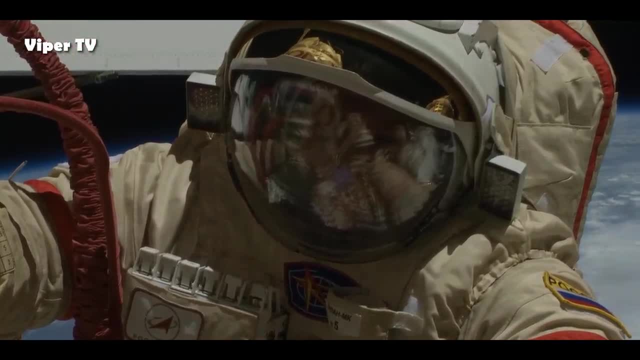 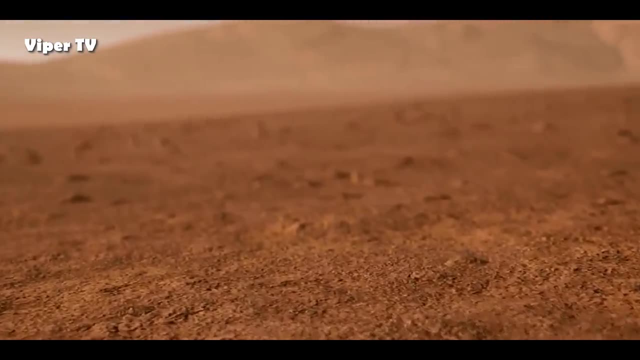 to transmit limited temperature data for 23 minutes. before it expired, Venera 9 not only made it to the surface and operated for 53 minutes in October 1975,, but was also the first craft to successfully deploy its camera on the ground. 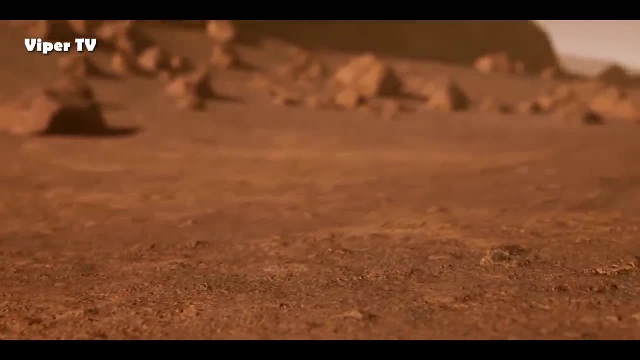 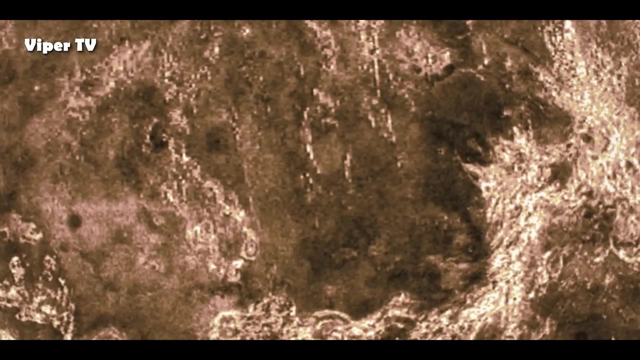 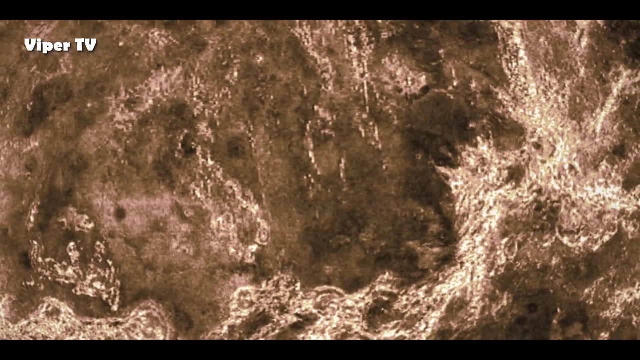 and transmit an image back to Earth In the first ever picture taken from the surface of another planet. the black and white fractured image revealed a rocky, desolate landscape, With measurements confirming it to be a blistering 485 degrees Celsius, with an atmospheric pressure of 90 ATM crushing down. 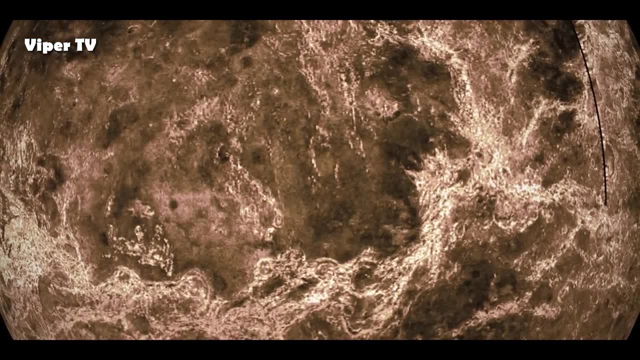 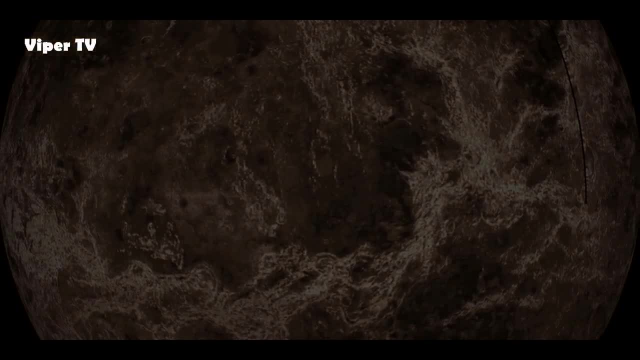 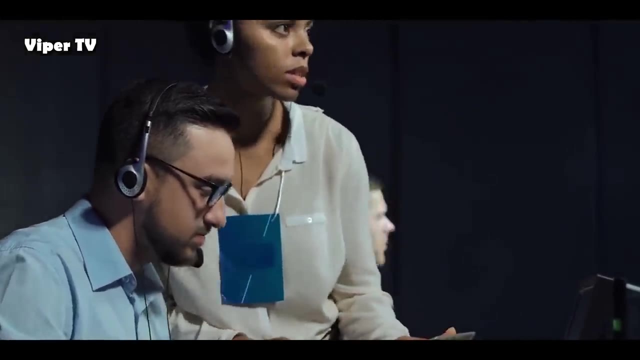 By the time Venera 13 launched on 30 October 1981, the ambition of the missions and the confidence in delivering data from the surface had been radically transformed. Venera 13 functioned for 127 minutes in recorded temperatures of 457 degrees Celsius. 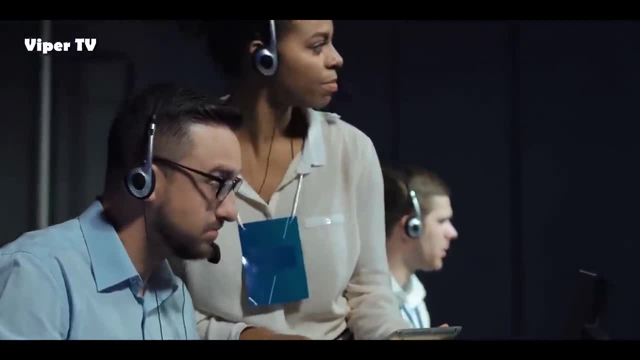 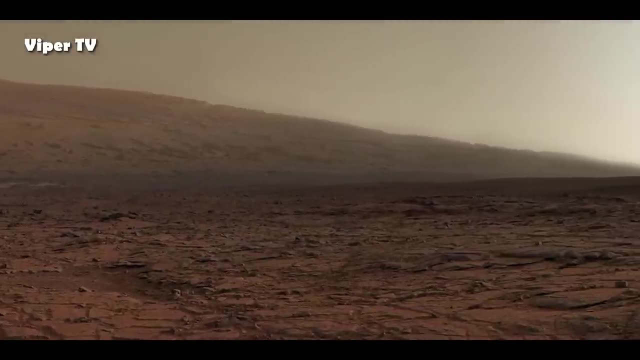 and a pressure of 89 Earth atmospheres. The probe's cameras deployed, taking the first colour image from the surface of Venus. Spring-loaded arms measured the compressibility of the soil, while a mechanical drill arm took a sample of the Venusian surface. 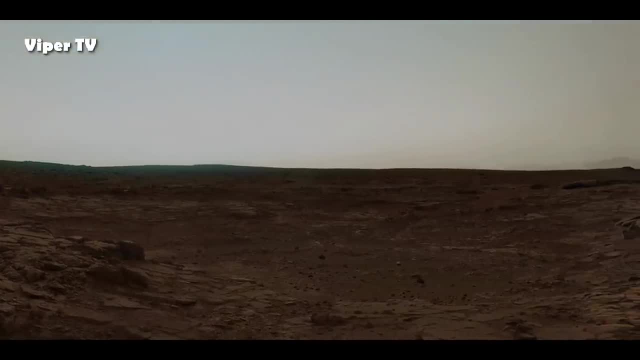 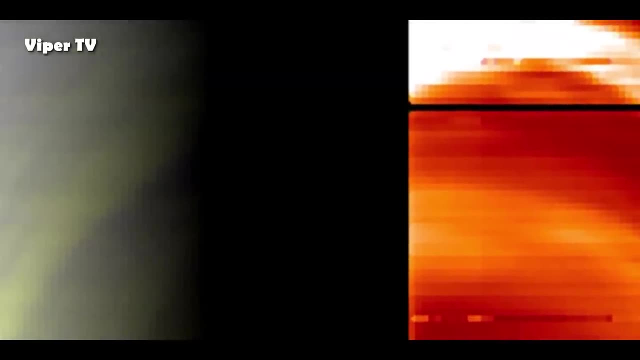 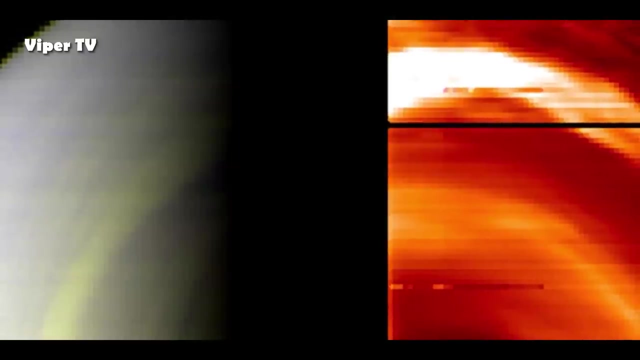 that was analysed by an onboard spectrometer. If that wasn't enough, onboard microphones were deployed to record the vicious winds that were assumed to be whipping the surface of Venus, the first ever recording of the sound of another planet As the Venera missions came to a close in 1983,. 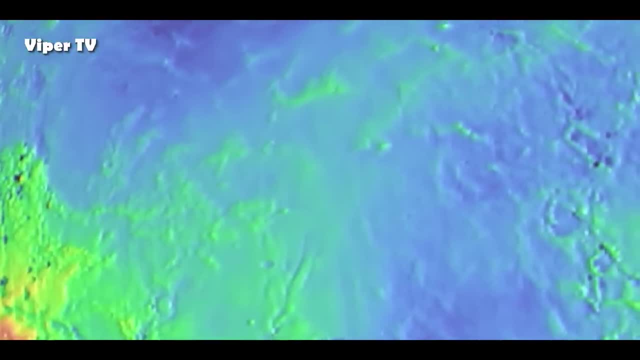 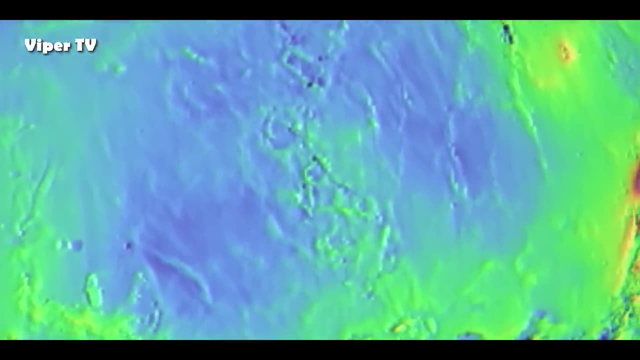 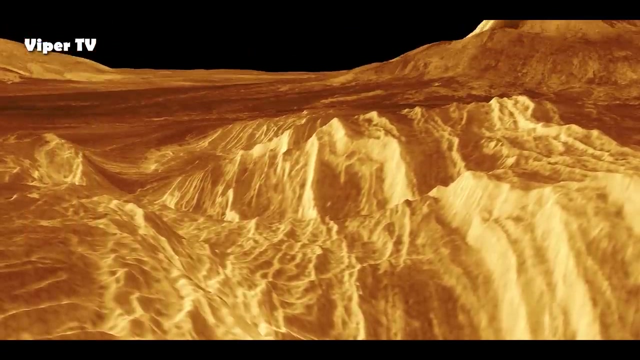 not even the smallest doubt remained of Venus's hostility. Far from the benign water world we had once imagined, the reality was that this was not a sister we recognised. In our search of the heavens for a place like home, we'd found a toxic, fiery hellscape. 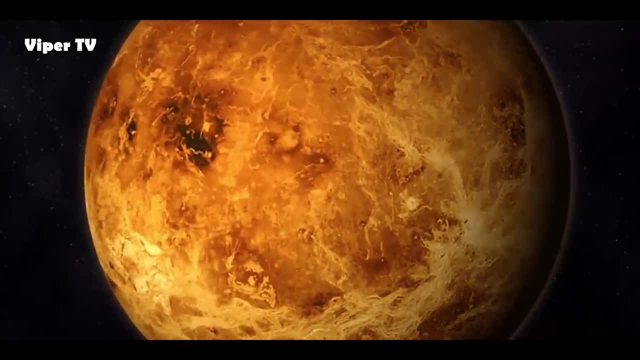 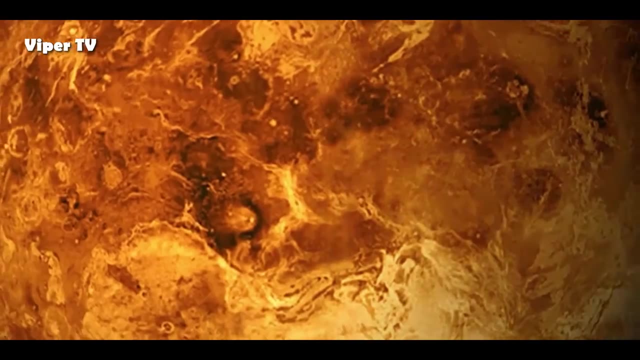 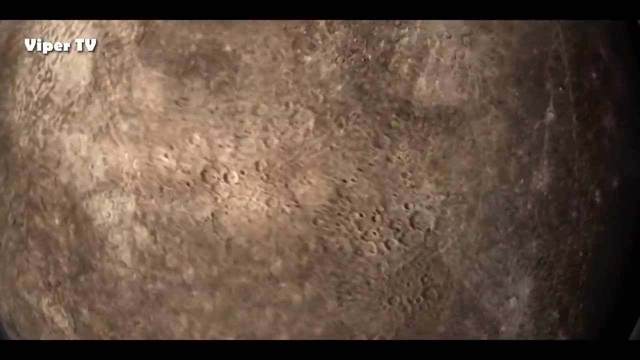 Venus is an enigmatic world, almost Earth-like in size, position and potential, and yet as far from paradise as it's possible to imagine. If Mercury's story is one of catastrophic orbital change and Earth's of balance and stability, the story of Venus is a tragedy. 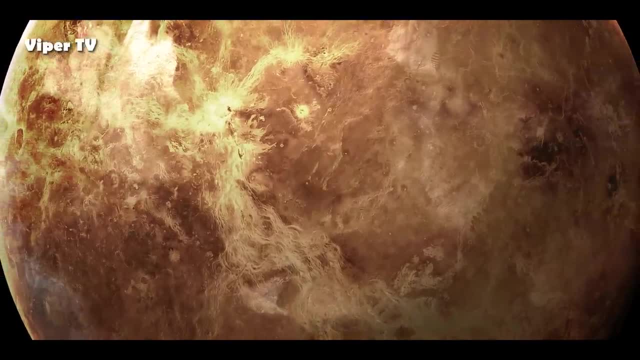 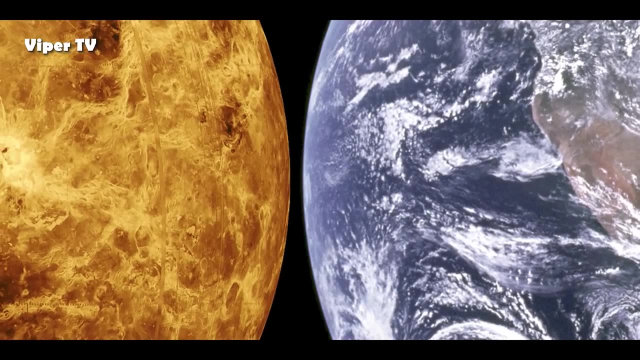 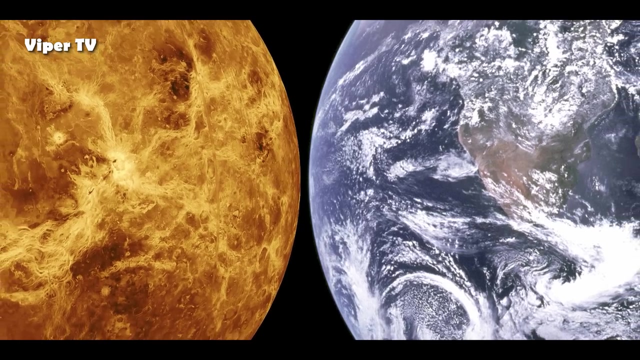 a tale of subtle yet relentless decline. So why did it all go wrong for Venus? Why did a world born with such similarities to the Earth take such a different path? To answer that, we need to look beyond the tortured planet we see today and go back to a time when Venus was a young, thriving planet. 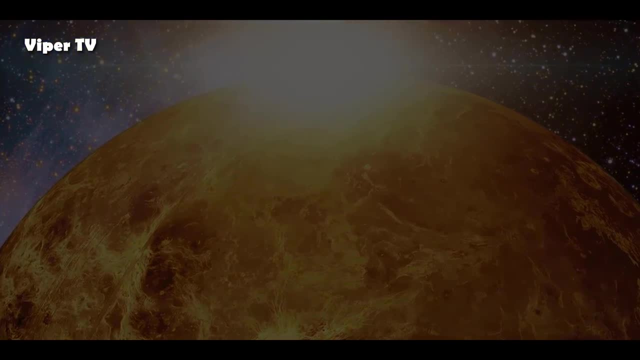 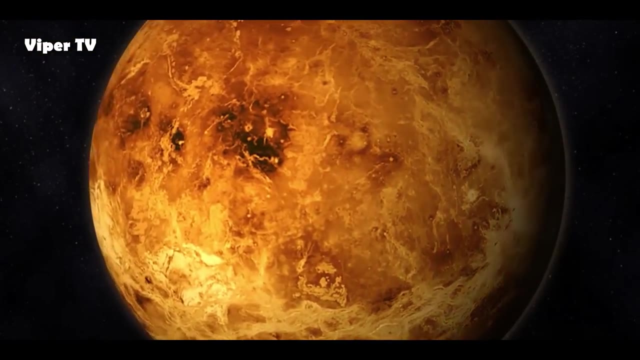 Four billion years ago, Venus was a familiar world, a world created from the same dust as the Earth, born just about the same size and settled in the same place as the Earth. A world just about the same size and settled into an orbit that seemed just far enough away. 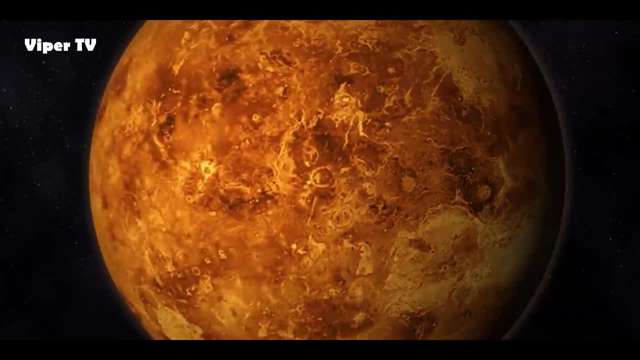 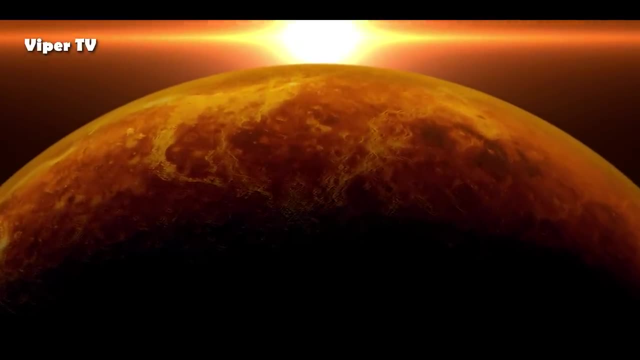 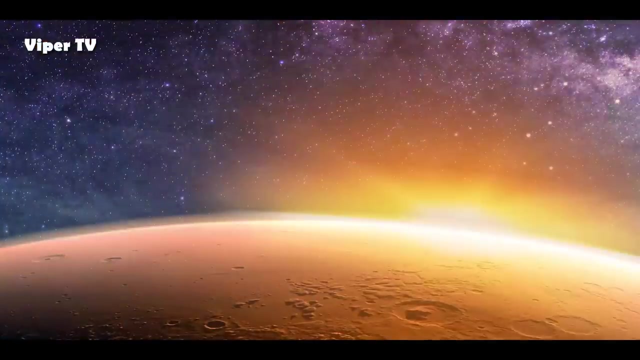 from the glare of the Sun to allow a precious process to begin to take hold. In almost every conceivable way, Venus's early life mirrored that of our own world. As its newly formed crust settled and cooled from the violent heat of its birth, an atmosphere began to grow around the young planet. 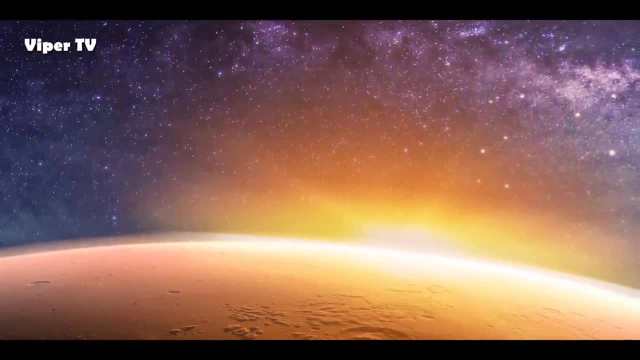 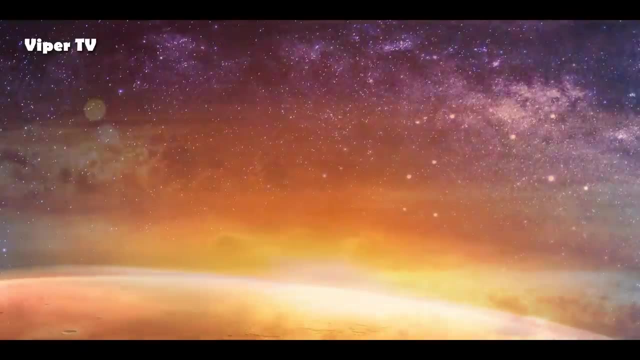 fed by gases bubbling up from the molten rock below its surface, as well as captured from the clouds of gas and dust it swept through on its orbit around the Sun, Clinging to the young Venus. this thin layer of gas would have certainly contained. 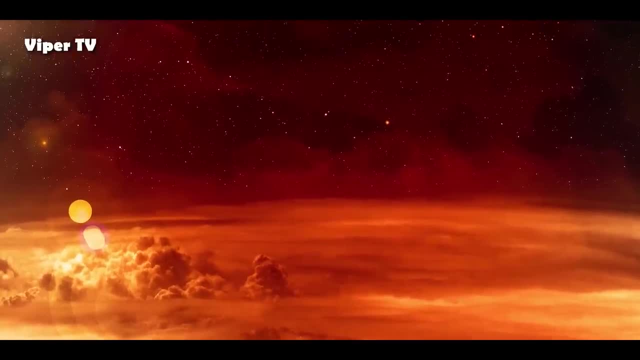 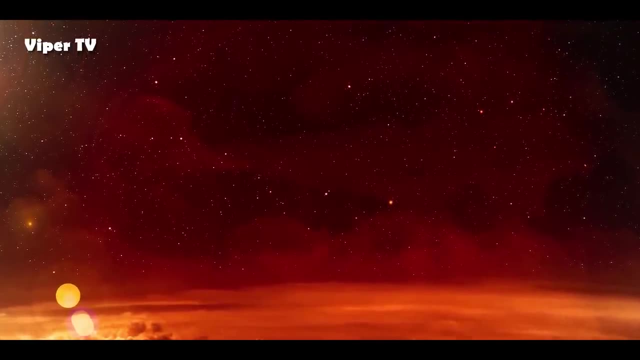 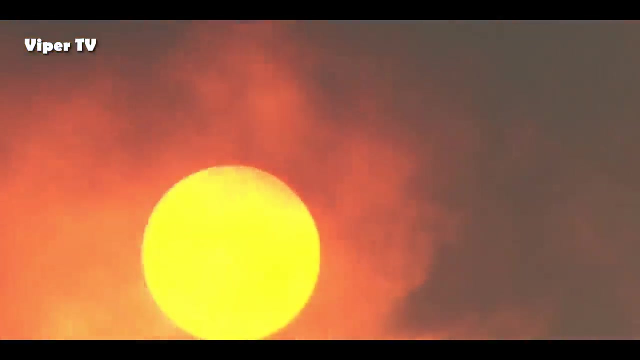 nitrogen oxygen and carbon dioxide. But, most intriguing of all, we are certain it would have also contained large amounts of water vapour High in the Venusian atmosphere. this water vapour eventually cooled enough to change state from vapour to liquid. 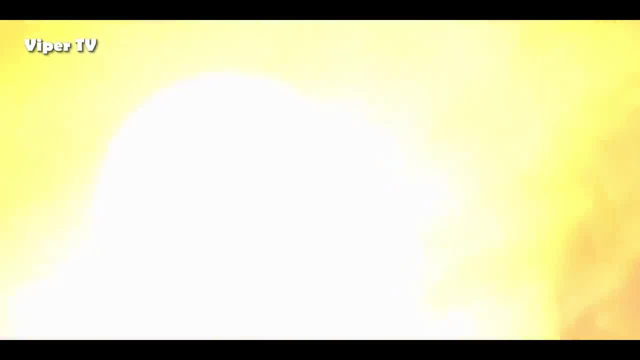 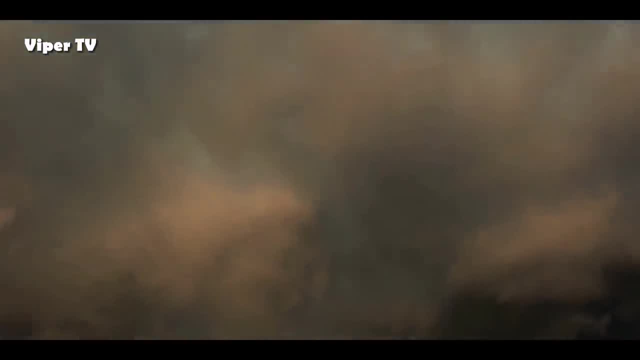 And with that transformation, a process began that perhaps for the first time on any of the planets would have seen the conditions become just right for droplets of liquid water to take shape and begin falling from the Venusian sky. These were the first rains of the solar system. 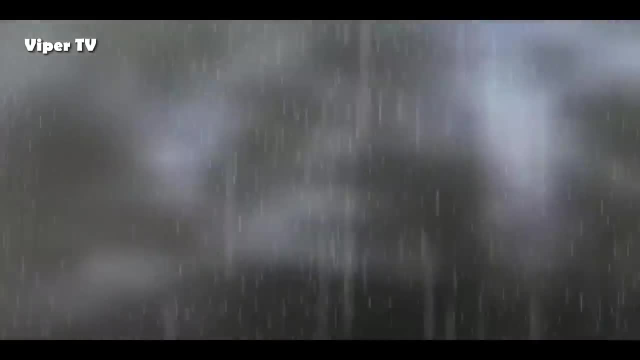 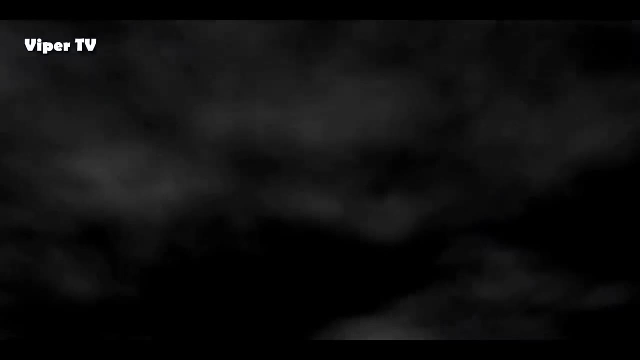 showering down onto the dry plains of Venus Gradually. these rains would have not just fallen but flooded the surface. Rivers would have flowed and shallow oceans taken hold of large swathes of the planet's surface- Venus, perhaps before even the Earth. 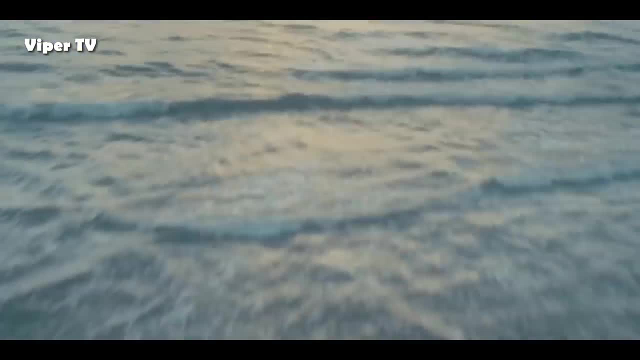 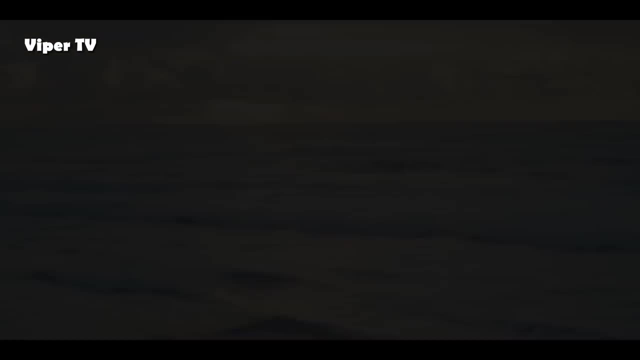 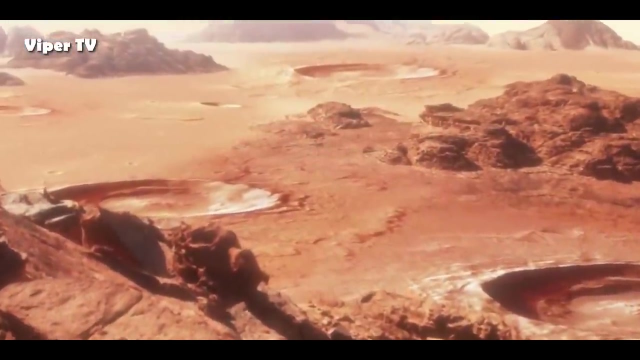 became a water world, a planet with skies full of clouds and a surface full of oceans, feeding the cycle of water around this young planet. How can we be certain this blue version of Venus existed, Unlike Mars, where we can see the evidence of its watery past? 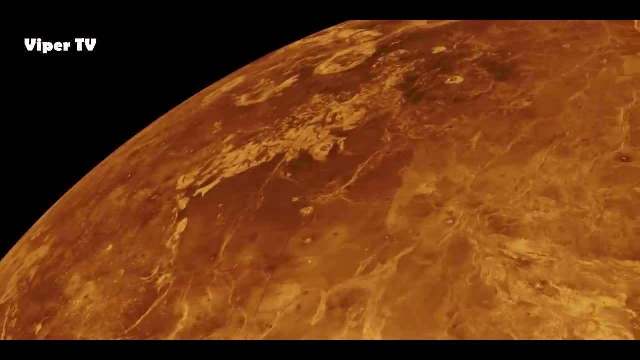 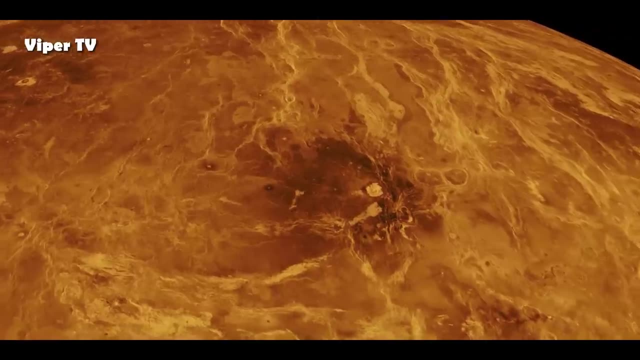 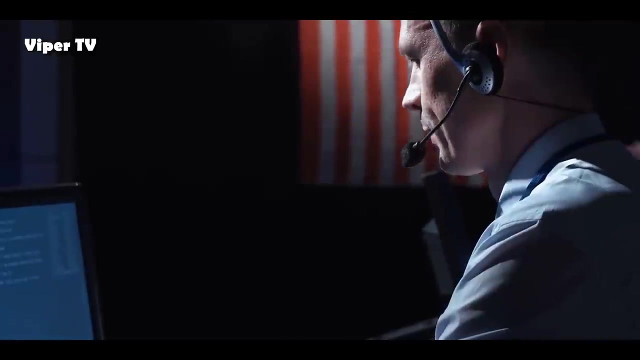 etched onto its surface. we have no such direct evidence of the presence of liquid water on the surface of Venus. The only physical evidence we have that suggests the planet's watery past comes from measurements taken by NASA's pioneer Venus spacecraft back in 1978.. 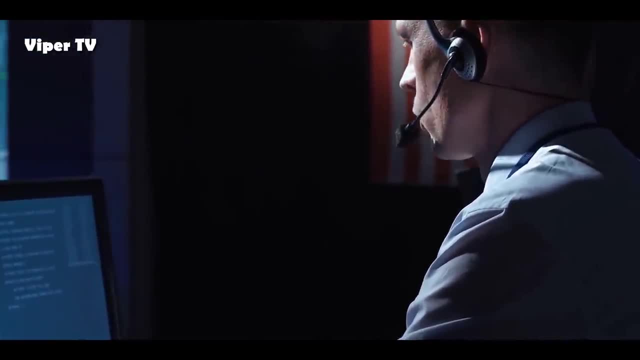 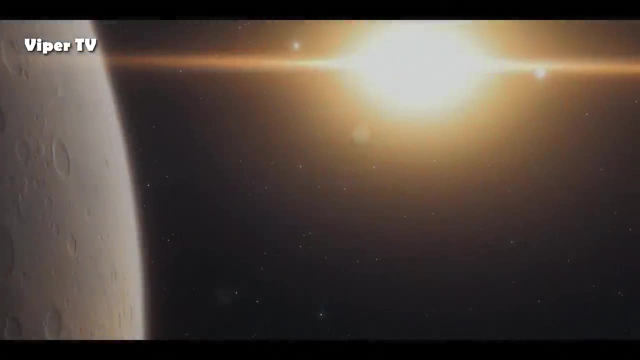 One of its most surprising discoveries revealed an unexpected amount of deuterium heavy water in the atmosphere. compared with hydrogen, This D-H ratio is far smaller on Venus than it is on Earth, And that's interesting because when the two planets formed, 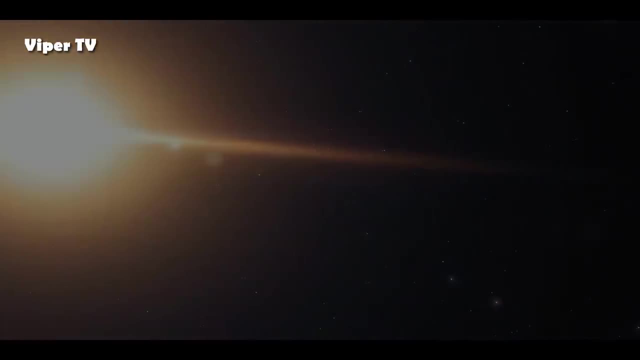 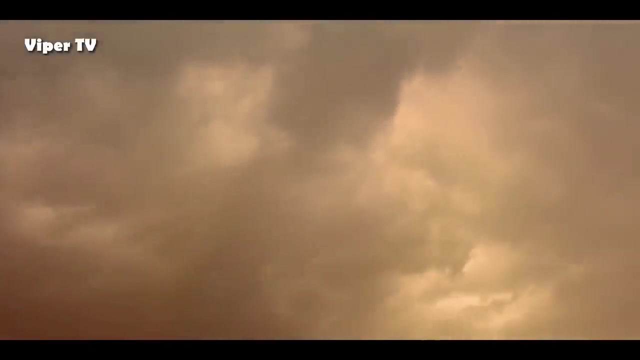 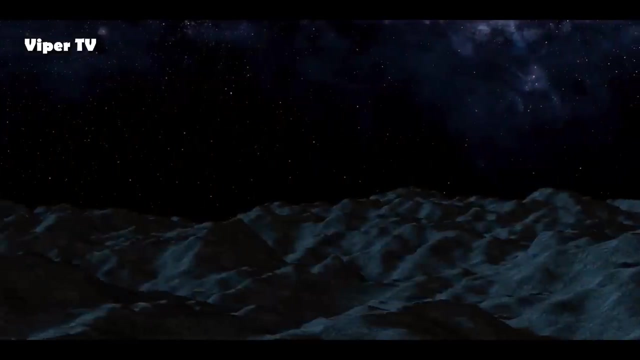 the ratio would have almost certainly been the same, Because hydrogen is far more easily lost from an atmosphere than deuterium. this smaller ratio suggests that Venus has lost a lot more water than the Earth over its lifetime: the signature of a long-lost primordial ocean. 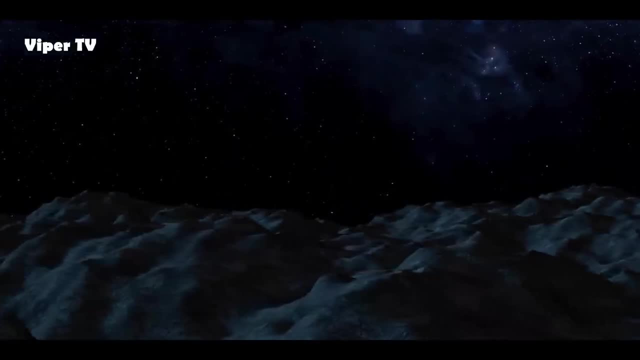 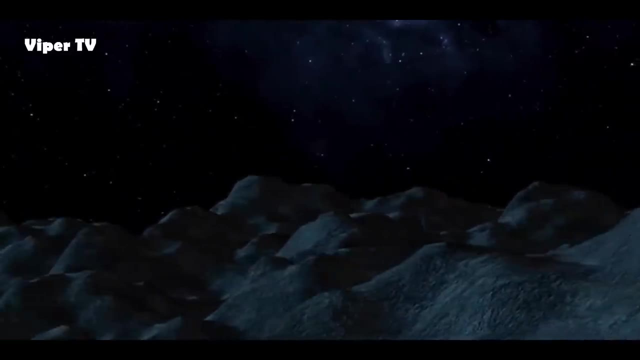 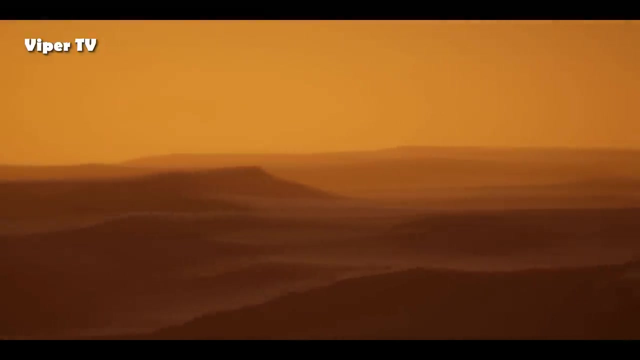 as cosmochemist Larry Knitler explains, Scientists believe that Venus once had a lot of water in its oceans, but lost it over time, and perhaps in oceans as recently as a billion years ago. The reason we can tell this is from the isotopic composition of hydrogen. 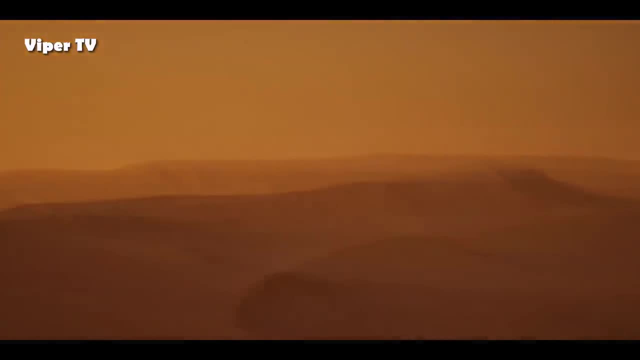 measured in its atmosphere by spacecraft. Now, hydrogen has two flavours of isotopes. Whereas most hydrogen atoms are just a single proton in the nucleus, some, a small fraction, are what we call deuterium, that have a proton and a neutron. 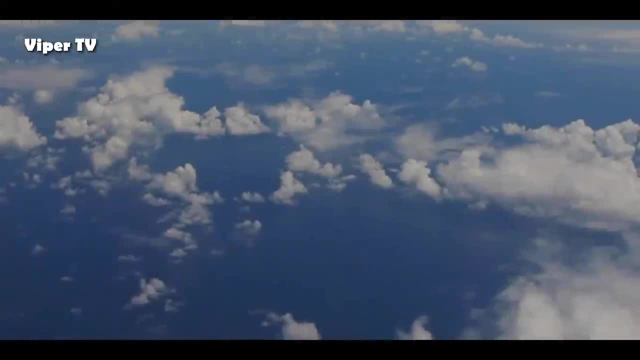 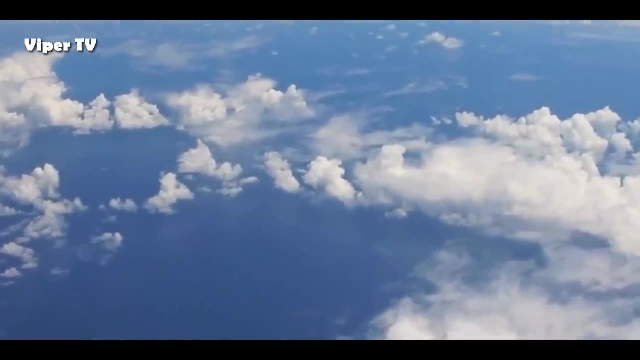 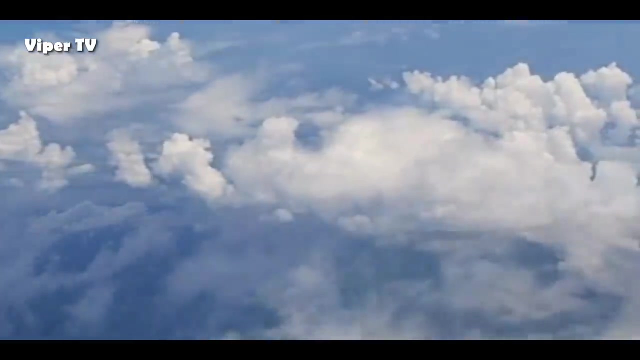 So they weigh twice as much as the regular hydrogen. What happens when you have evaporation of water from a planet or the atmosphere is that the water molecules that contain hydrogen are much lighter than the water molecules that contain deuterium, so they evaporate more easily and can be lost more easily. 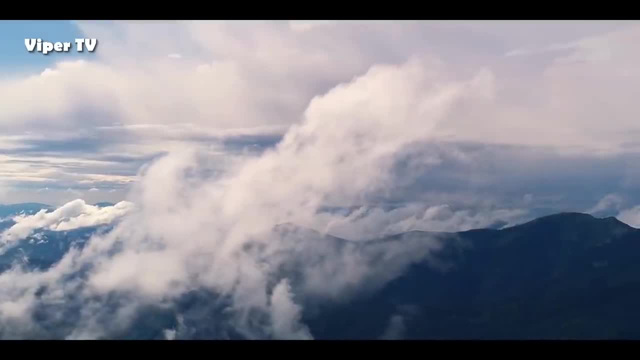 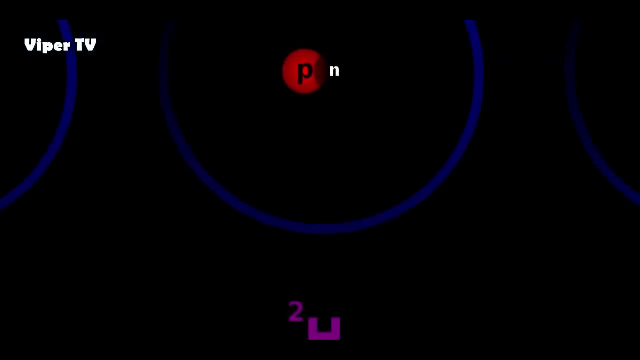 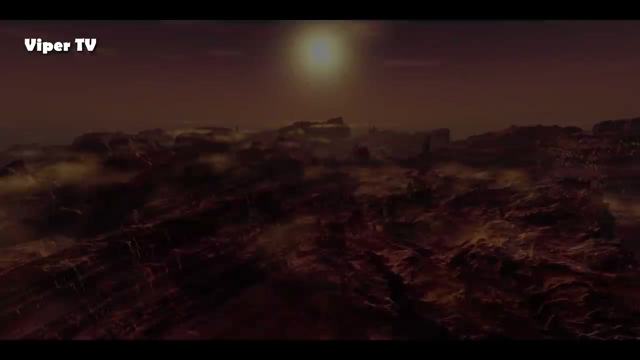 So over time, as you evaporate water, deuterium-bearing molecules stay behind relatively to the regular ones and you build up a deuterium-to-hydrogen ratio And by back-calculating from the measured ratio today, we can figure out how much water has been lost. 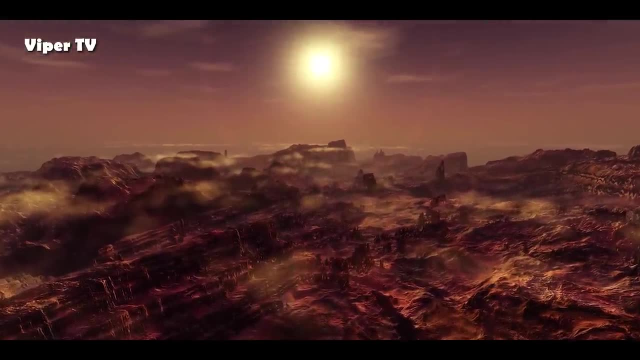 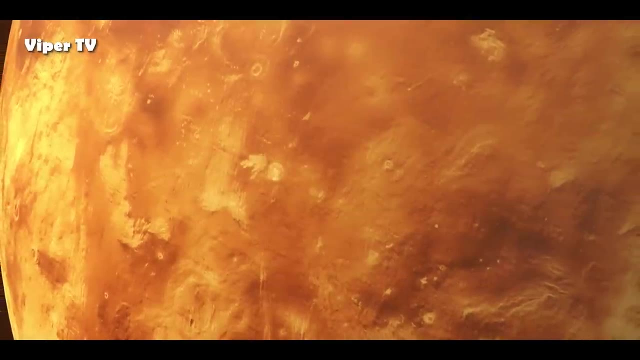 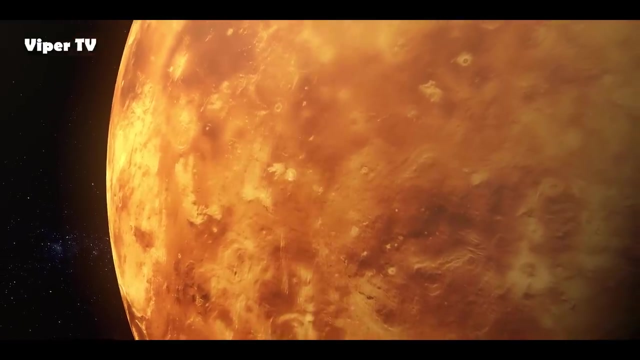 over the billions of years of evolution and on Venus. it's quite a lot. None of this is solid proof, but it does begin to point us in one direction, And, with no further exploration of the surface, we've had to rely on an accumulation of indirect evidence. 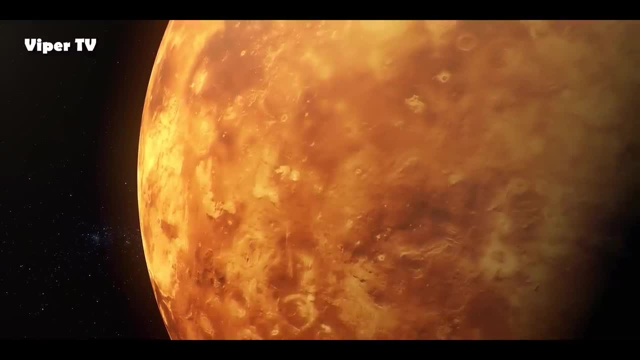 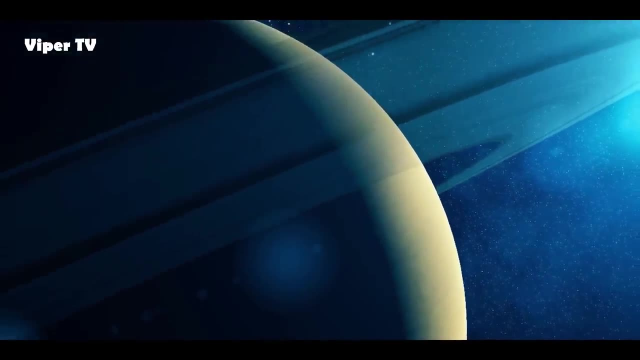 to begin to paint a more detailed picture of Venus's watery past. The next planet out, Saturn, also has its ever-growing family of moons. Amongst its collection of over 60 confirmed satellites are Titan, the only known moon with a dense atmosphere. 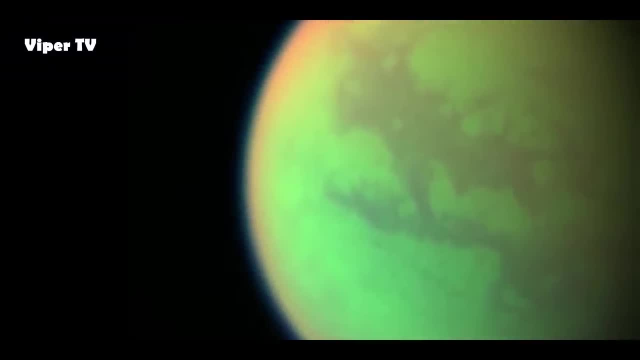 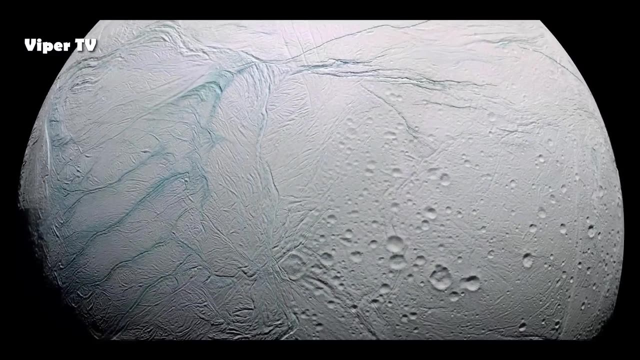 and liquid lakes on its surface, though they are primarily methane, not water, and Enceladus. a frozen ice moon, just like Europa, with a liquid ocean deep beneath its ice. Until we go back and explore further, we can't be certain what lies below. 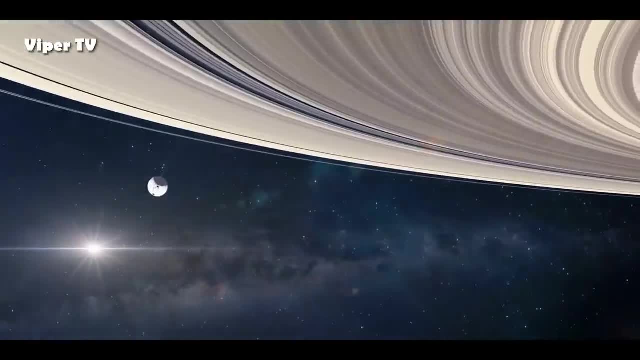 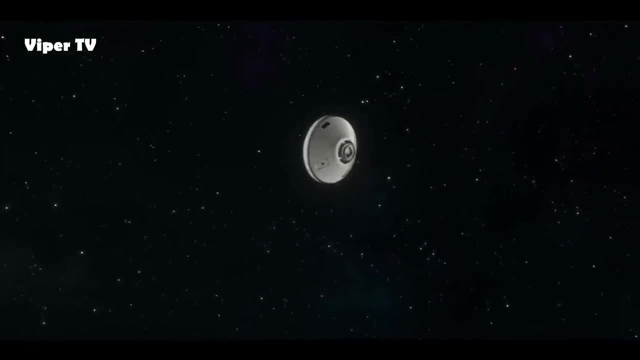 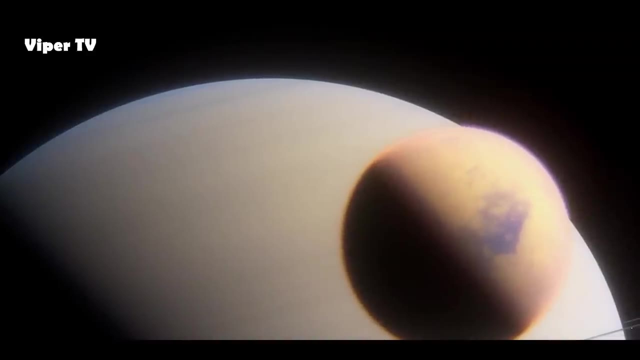 But the possibilities that the Cassini probe has so tantalisingly hinted at make it one of the most exciting places for us to visit within the next generation of interplanetary expeditions. All these ice worlds sitting dormant in the frozen reaches of the solar system. 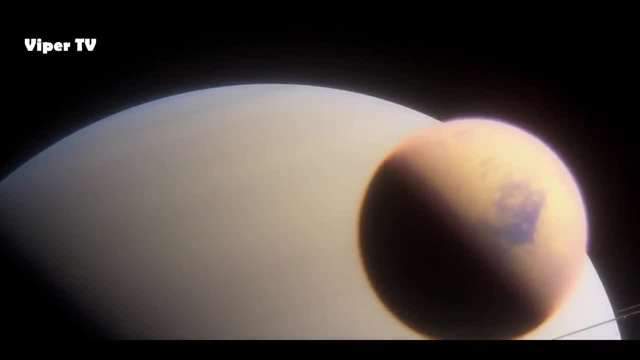 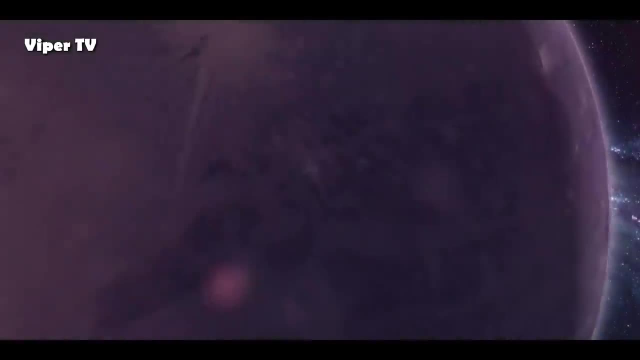 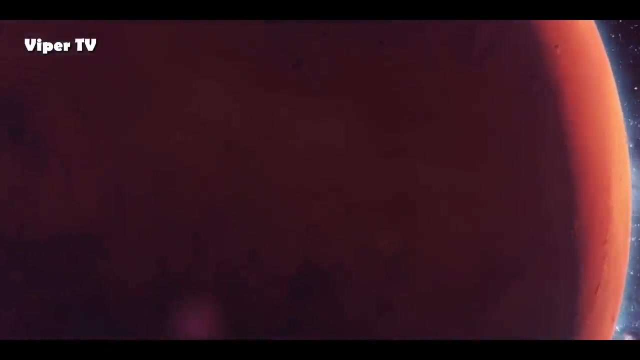 offer the promise of a very different future, one in which the rocky worlds of the inner solar system have been reduced to cinders and a new generation of worlds waits to be born. Ice worlds will become water worlds, warmed by the expanding sun. 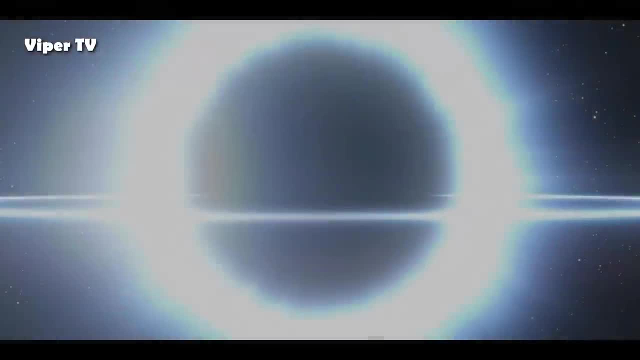 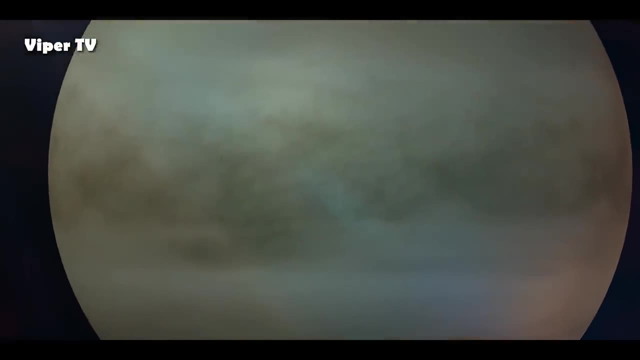 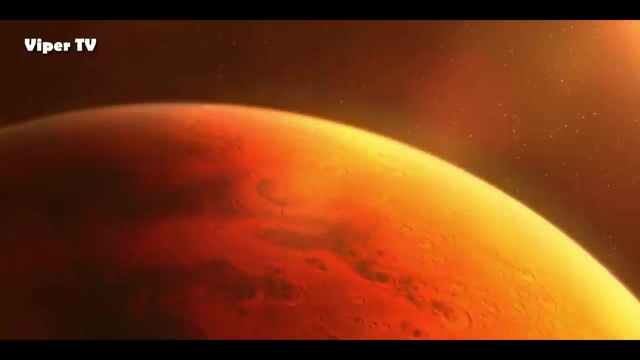 until our dying star ultimately collapses into a white dwarf. Today, Venus has the slowest rotation of any planet in the solar system, taking 243 Earth days to complete one rotation on its axis. This period is known as the sidereal day, which is different to a solar day. 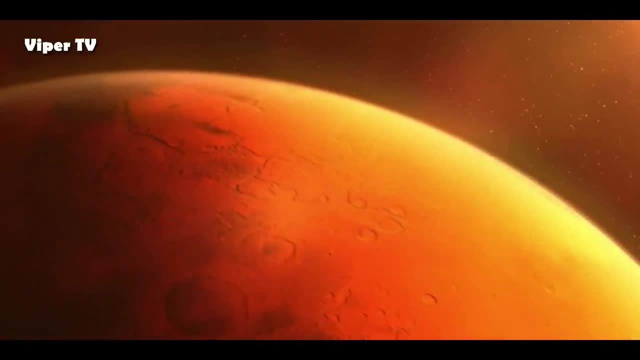 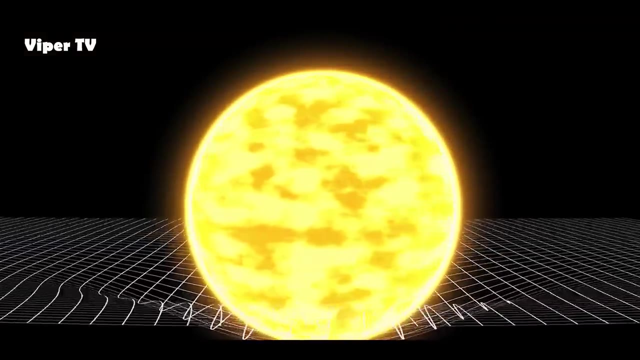 the time it takes for the sun to return to the same point in the sky On Earth. the sidereal day, at 23 hours 56 minutes and 4.1 seconds, is very close to the solar day, which lasts pretty much exactly 24 hours. 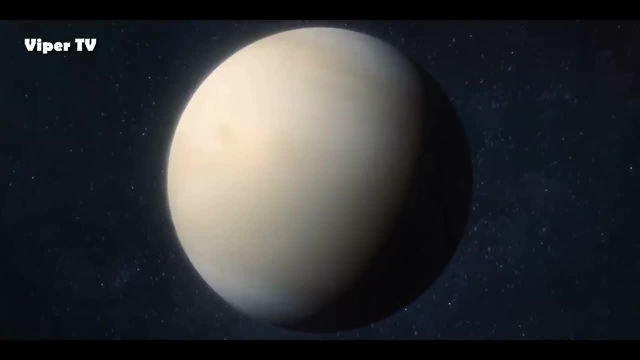 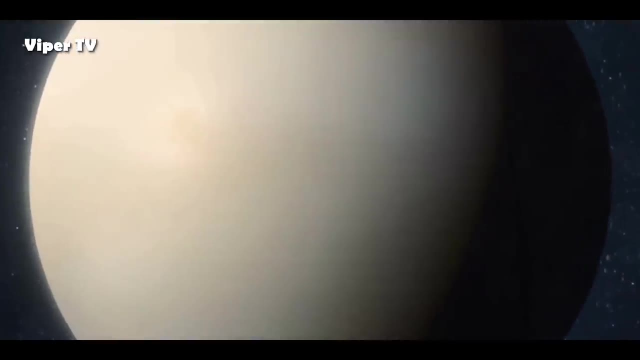 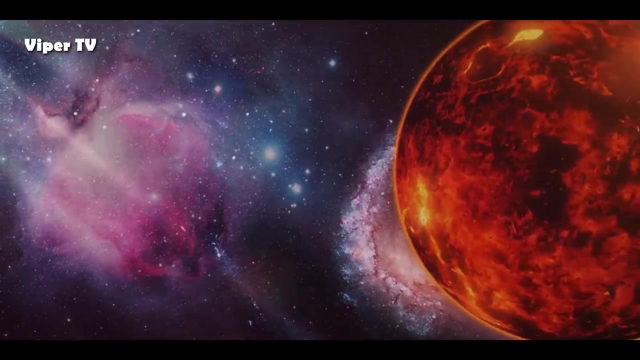 But on Venus the difference between these two periods is much greater. Even though the planet takes 243 days to rotate on its axis, when combined with its orbit, a solar day on Venus lasts for 116.75 Earth days. It means every day on Venus lasts almost four months on Earth. 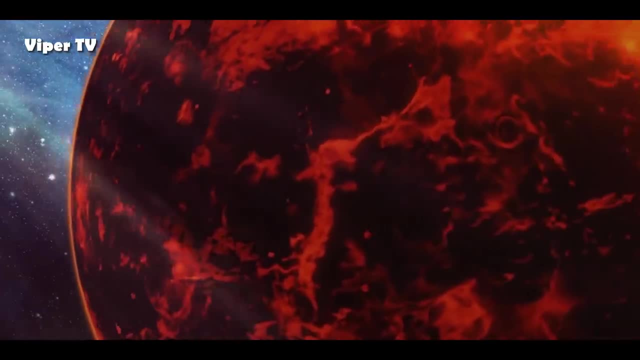 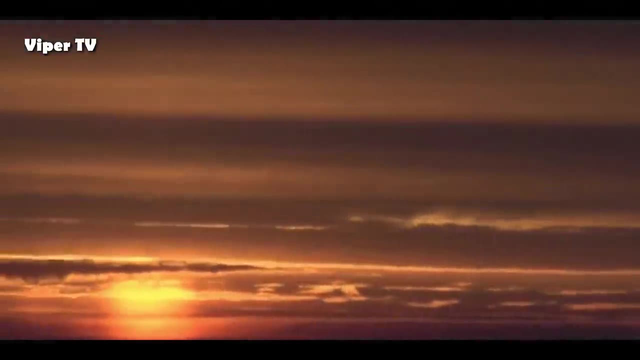 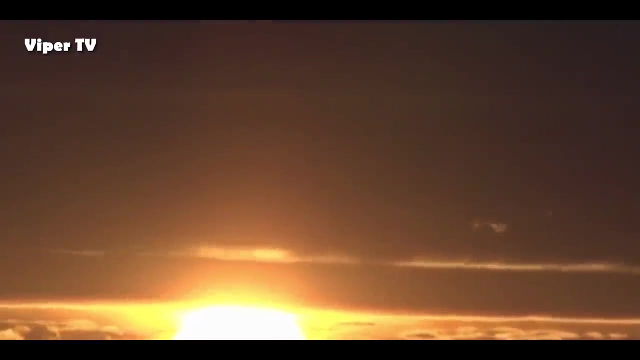 And not only that, but Venus also rotates from east to west, one of only two planets to do so, along with Uranus. So across this toxic world, a sunrise would last literally for days as it inches across the sky. This slow progression of the sun in the Venusian sky. 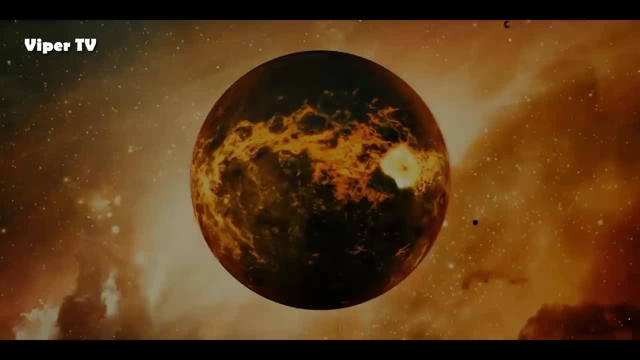 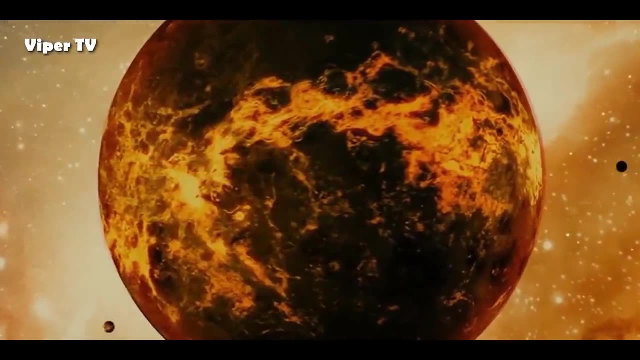 due to the planet's creeping rotation has raised many questions about how, in the past, the planet would have been heated and how the climate would have been affected by such a different rotation compared with the Earth's. Today, the climate of Venus is what is known as isothermal. 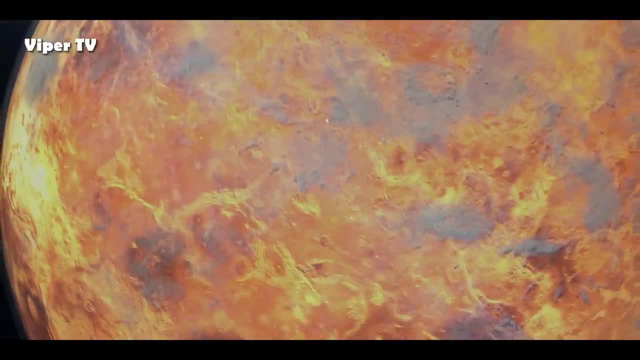 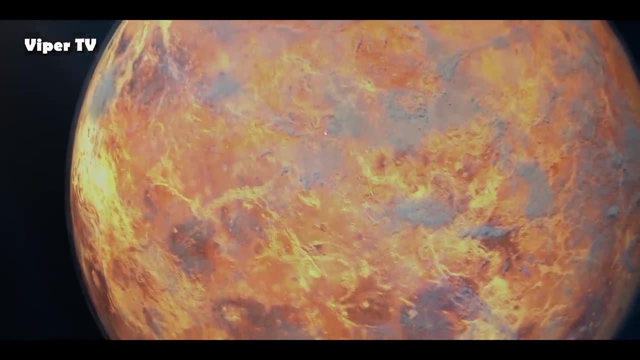 There is a constant temperature between the day and night sides and between the equator and the poles. This is because the thick atmosphere naturally acts like a blanket dissipating the heat of the sun, so that the only real variation in temperature on the Venusian surface 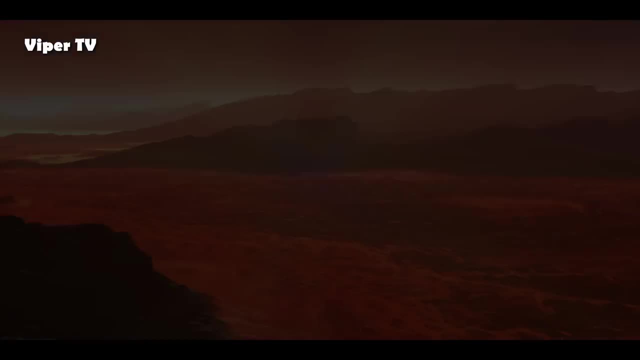 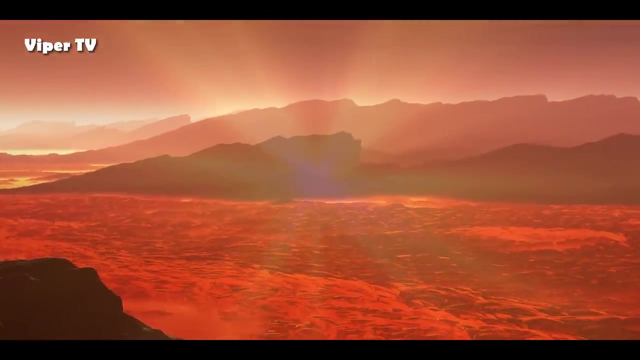 occurs due to differences in altitude. In its past, however, this may have been very different, with a more Earth-like atmosphere, so the sun would have been beating down on the planet's surface for days on end. To make things even more complex, 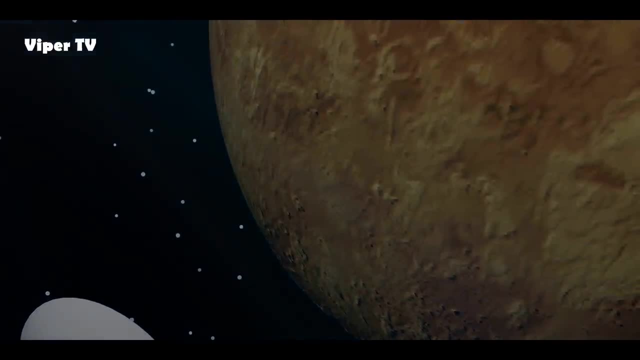 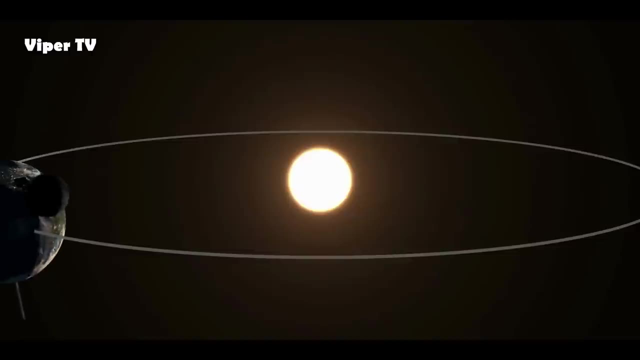 we know, the spin of a planet is intimately linked to its climate, and we've got strong evidence to suggest that how fast a planet spins is directly related to its chance of habitability. Until very recently, it was assumed that the slow rotation of Venus 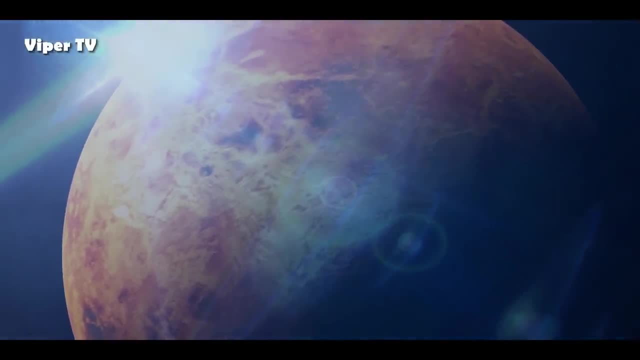 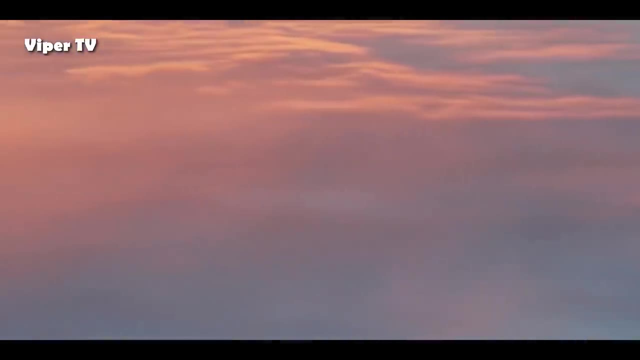 must have been caused by the presence of a thick atmosphere early on in its history that, in effect, acted as a brake on the planet's spin. However, recent studies now suggest that the planet could have had a thin atmosphere like that of modern Earth and still have ended up with its slow rotation. 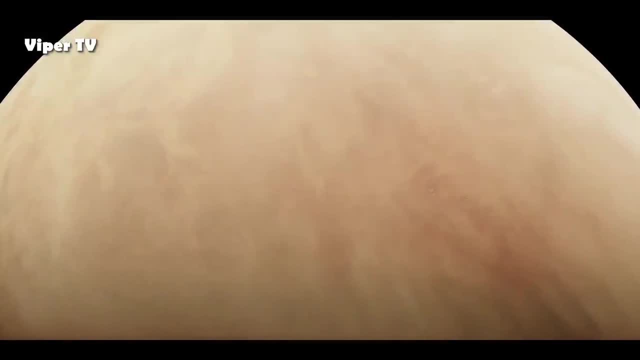 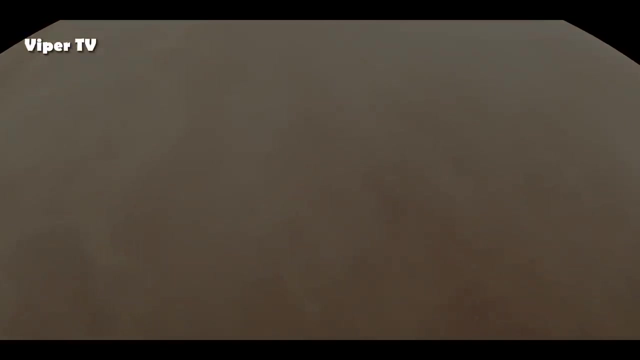 Gradually, as we start to build a picture of ancient Venus, we begin to see beyond the cloud cover of today, through to an ancient planet with an Earth-like atmosphere and a day lasting over 200 Earth days as the sun beat down on the ocean-covered surface. 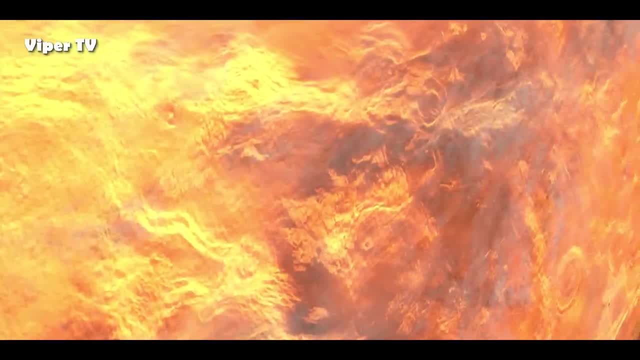 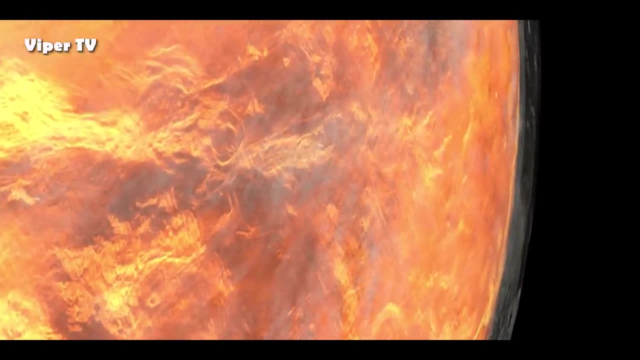 To make sense of the climate of this Earth-like Venus, the team at the Goddard Institute needed to make another tweak- or postulation to be more precise- to the model, With the sun hitting the one side of the surface for so much longer than on the Earth. 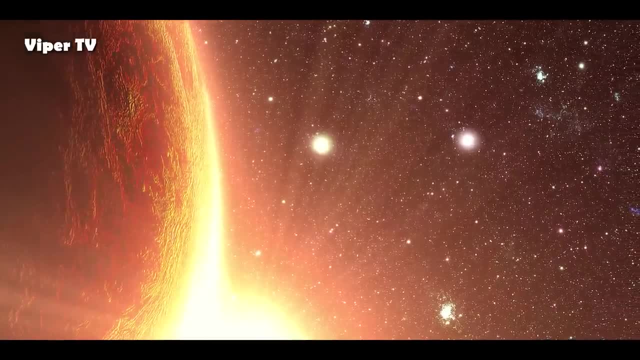 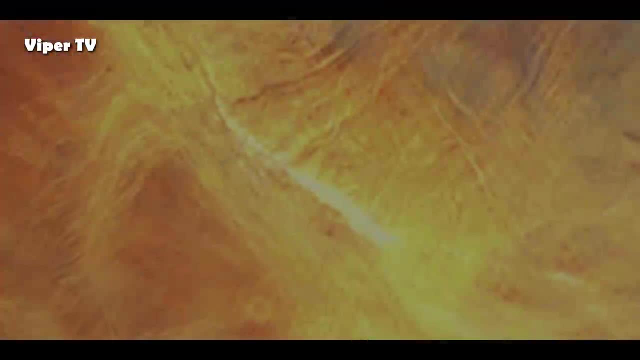 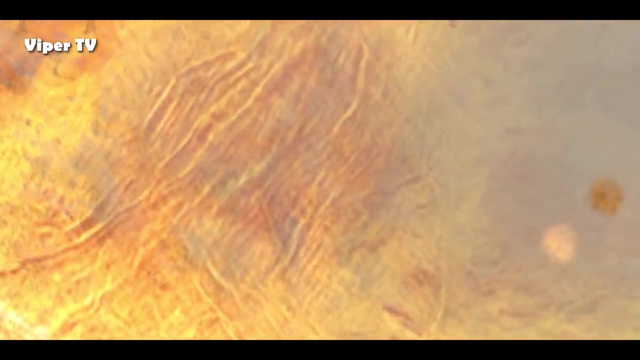 the evaporation rate of the oceans would be far greater and potentially incompatible with the water world we suspect existed. But by simply adjusting the amount of dry land on the surface of Venus, especially in the tropics, the effect is dramatic, With a higher percentage of land. 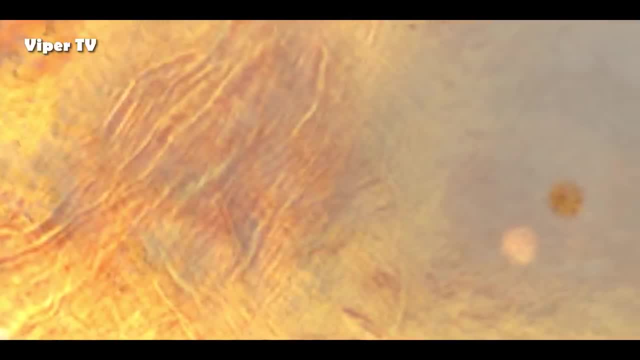 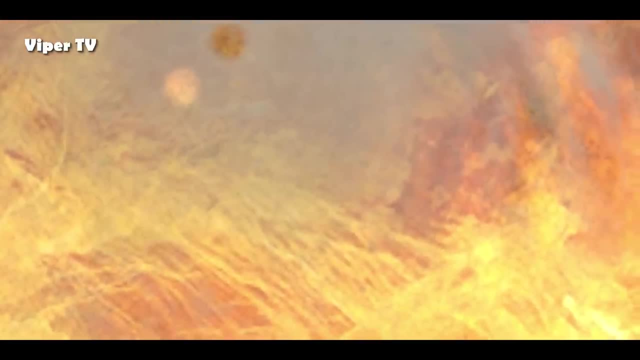 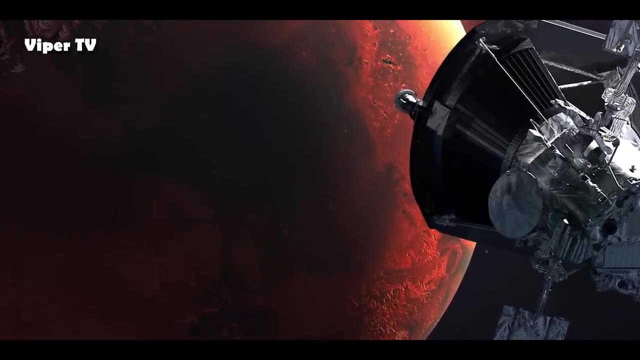 the models suggest that even the slow rotation would not dry out the planet and it could have held onto enough water to be ripe for supporting the emergence of life. By combining all of this data, the GIS team have painted our most up-to-date picture of early Venus. 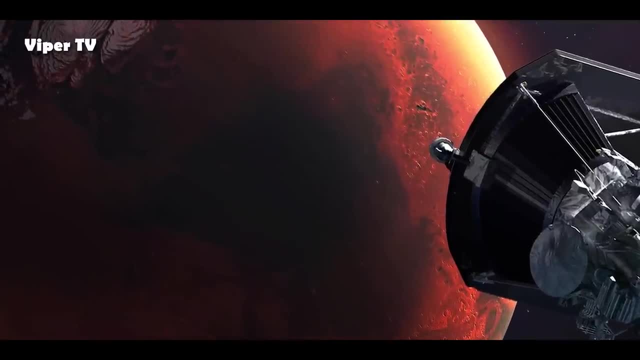 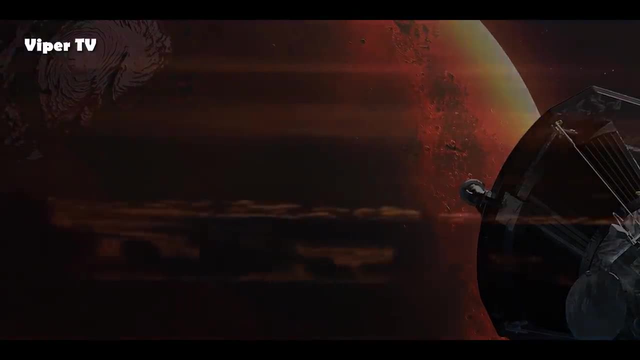 And it's a beguiling image Within the infant solar system. it is a planet the size of Earth with similar atmosphere to the one we see today. On Venus, days lasted for months as the sun arced slowly across the sky from west to east. 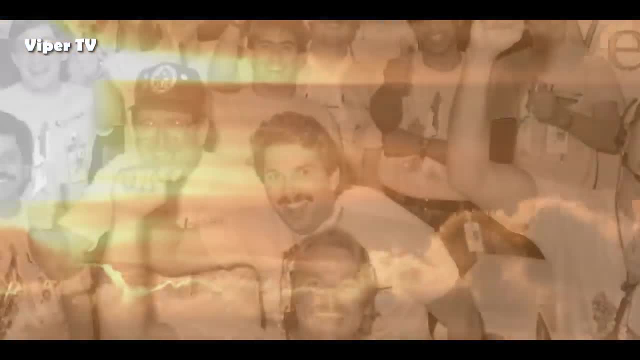 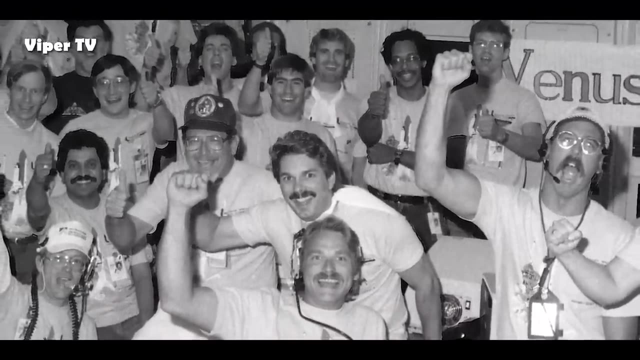 rising and setting over a vast ocean. Finally, the data from radar measurements taken by NASA's Magellan mission in the 1990s was used to paint the last brushstrokes of this long-lost world, Filling in the lowlands with water. 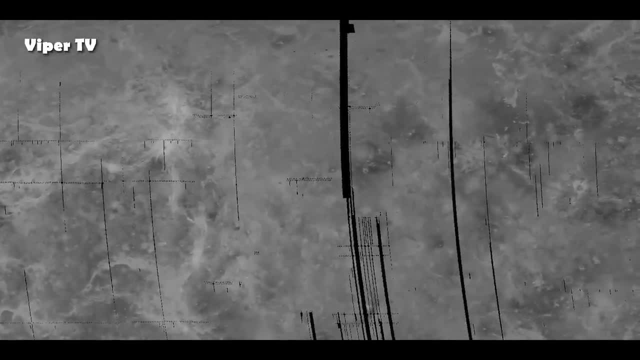 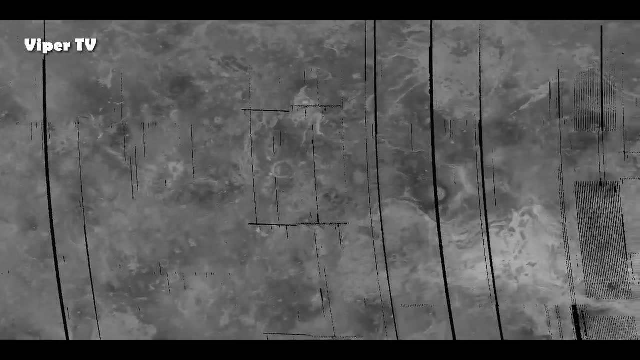 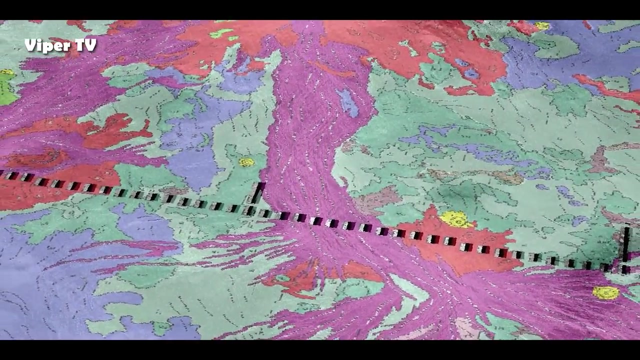 the topography of this ancient world emerges, with the highlands exposed as the Venusian continents. It all points to the possibility that Venus could have been the first habitable world in our solar system. So what changed? To find out, we need to look not just at the planet in isolation. 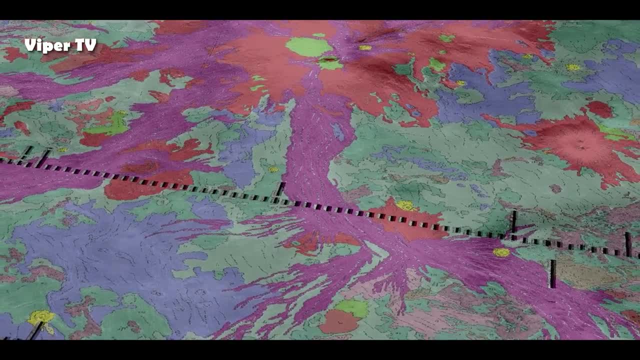 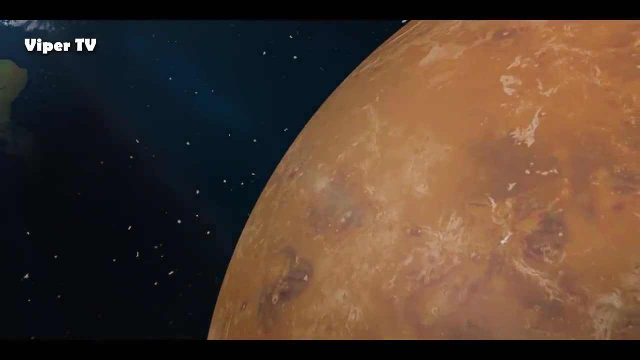 but also at the star around which it orbits. No planet lives out its life in isolation. Venus, like all the planets, is not just part of a configuration of planets and moons, asteroids and comets, but is also part of a solar system. 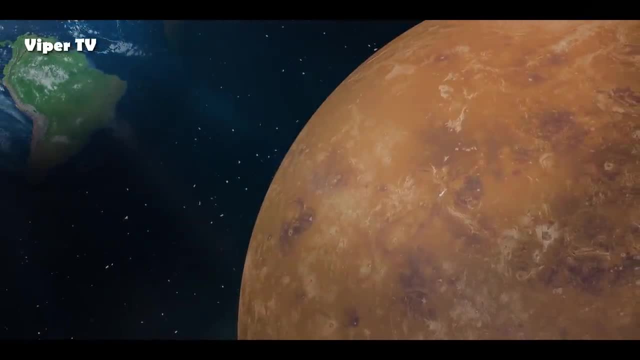 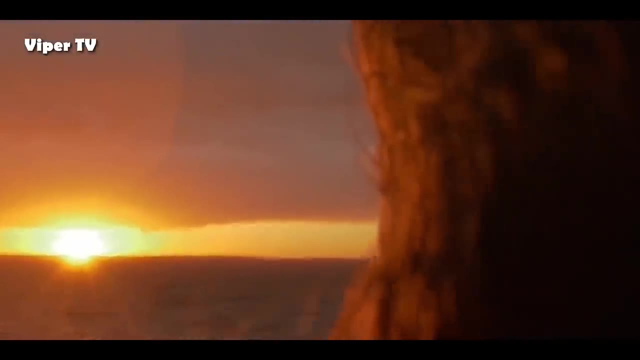 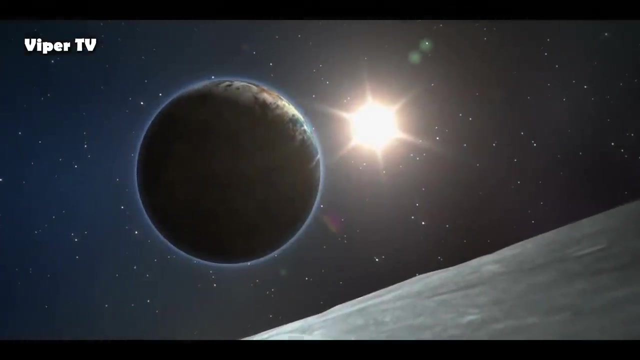 a system that is driven more than anything else by the star at its centre. Today, the sun burns bright in our skies, bathing our planet in just enough starlight to keep the oceans from freezing, but not too much to boil them away. Earth lies in the sweet spot we call the Goldilocks zone. 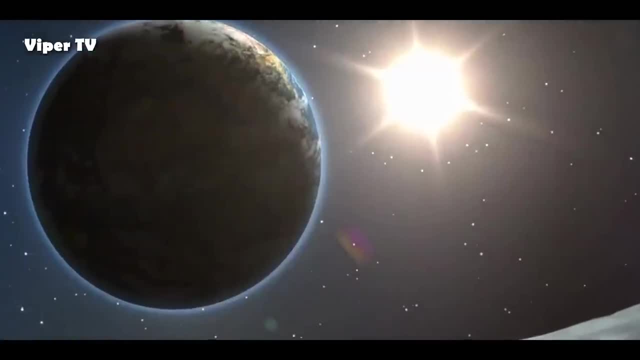 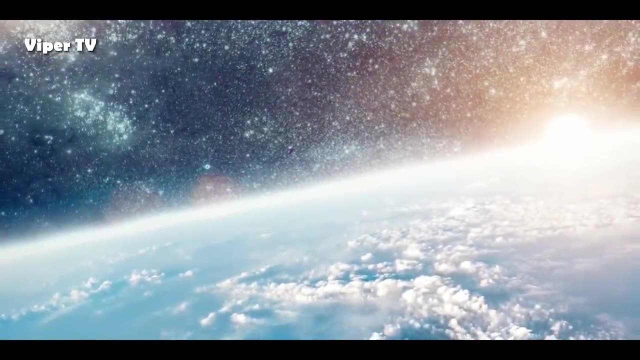 but, as we have already seen in this chapter, nothing in the solar system is forever, and what we see today is not what we will see tomorrow, nor what we would have seen yesterday. As our sun gets older, it's gradually burning, hotter and hotter. 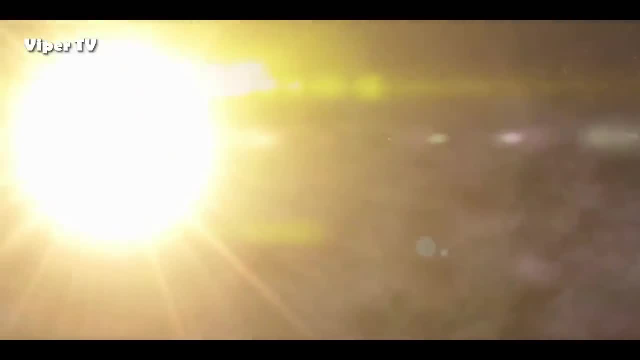 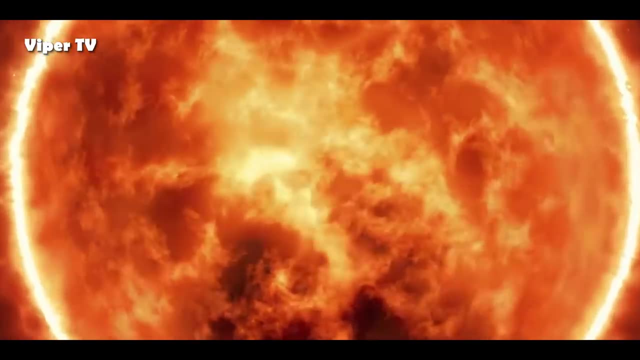 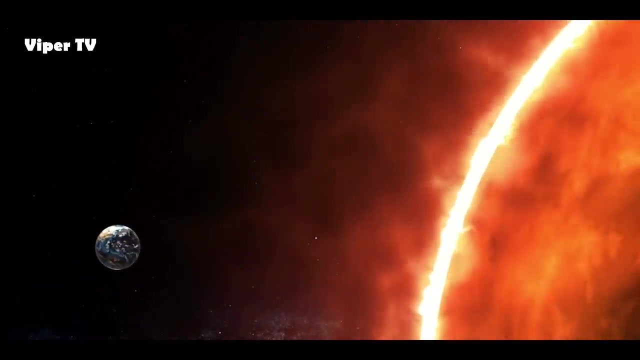 This is because, as it ages, the process of nuclear fusion- the fusion of hydrogen into mainly helium- gradually leads to an increase in the amount of helium in its core. This rise in helium causes the sun's core to contract, which in turn allows the whole star to shrink in on itself. 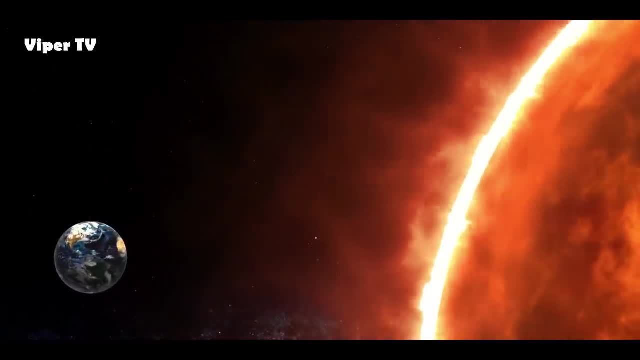 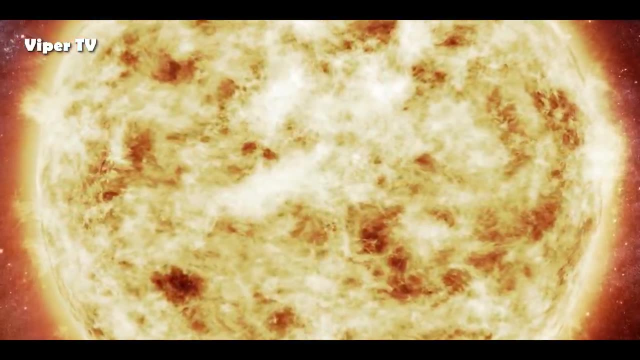 creating an increased pressure. that results in a rise in the rate of fusion, and so the energy output of the sun goes up. If tomorrow the sun is burning hotter than today, it of course makes sense that in the early days of the solar system. 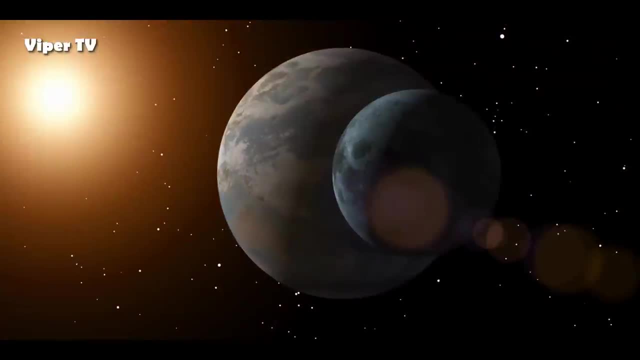 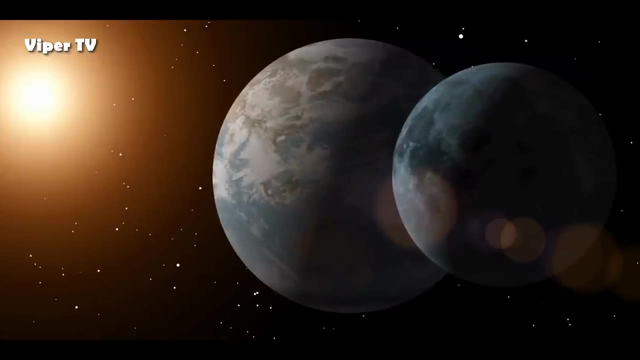 our sun burned far less brightly. It's a life cycle that is common to all main sequence stars. the category of star that includes our sun and, as the most common type of star in the universe, we've been able to study this life cycle in intimate detail. 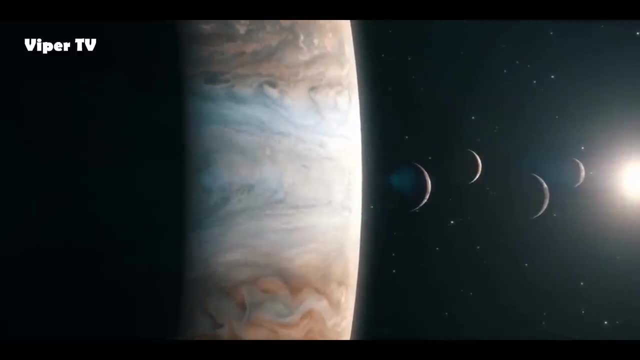 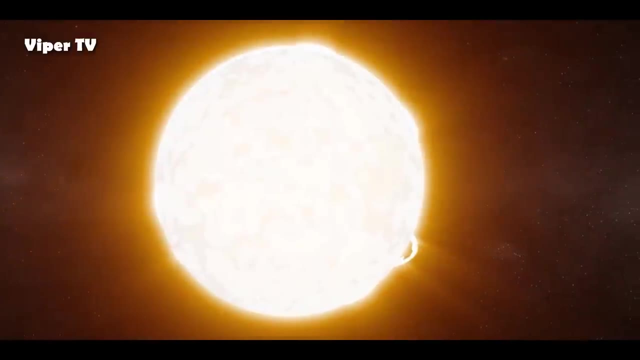 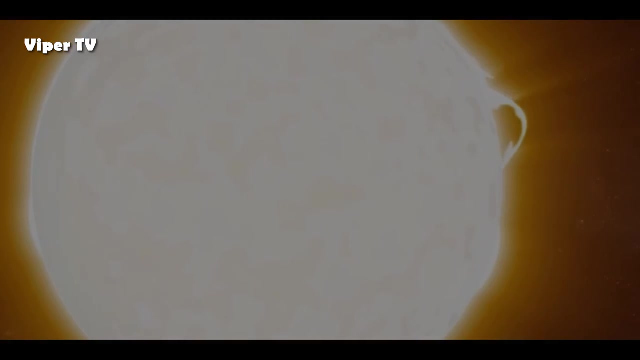 allowing us to make immensely detailed predictions about the characteristics of our sun in the past and in the future. Winding back the clock, the current consensus among astronomers is that four billion years ago, the faint young sun was at least 30% dimmer than it is today. 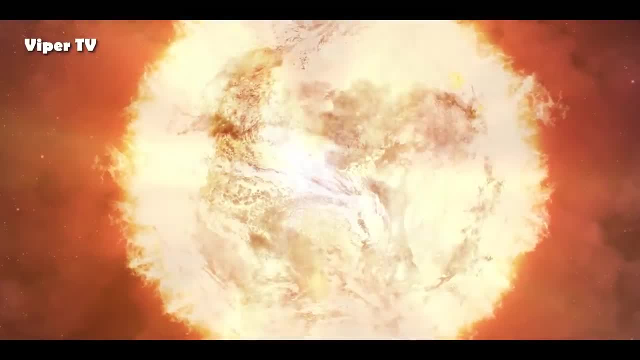 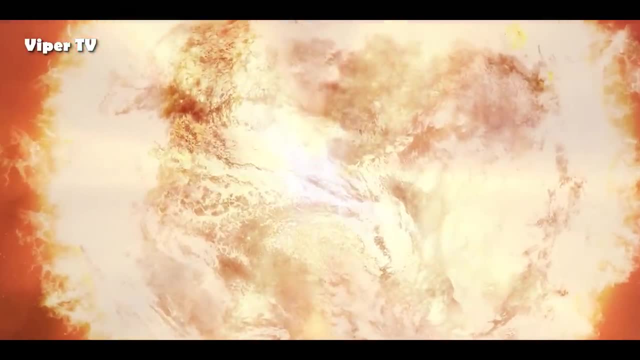 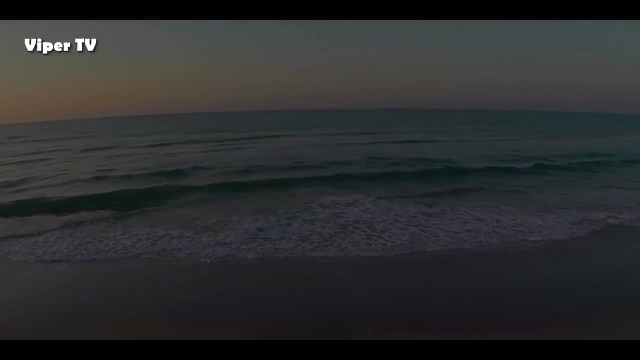 This cooler sun would have undoubtedly had a big impact on all of the terrestrial planets. Earth would have been much colder and, as it was receiving far less solar energy, it remains something of a mystery as to why our planet wasn't frozen solid Instead at this time on Earth, 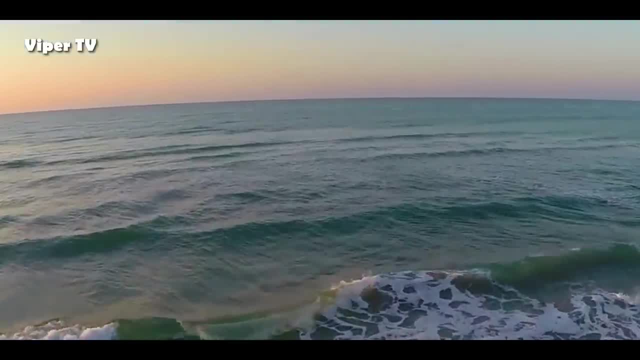 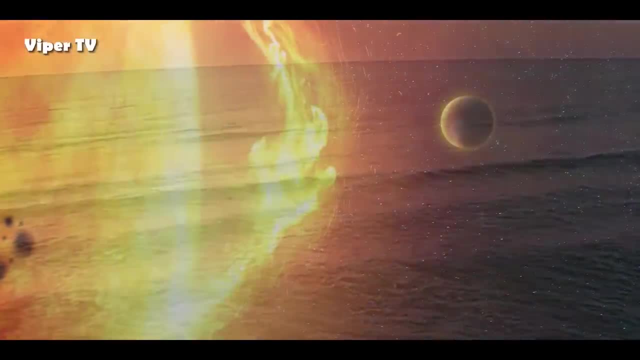 first life was just beginning in the liquid water that we are pretty certain covered its surface. At the same time, 3.5 to 4 billion years ago, the young sun would have bathed Venus in a warmer glow. This ocean world found itself in its very own sweet spot. 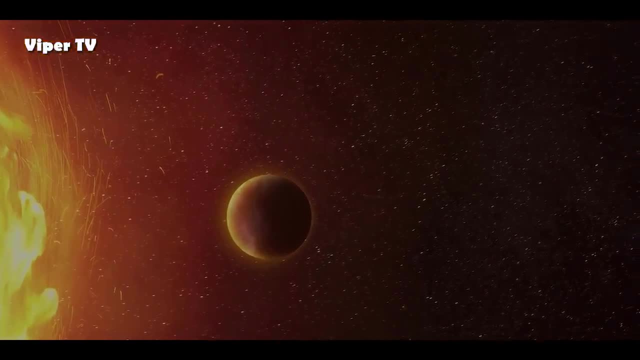 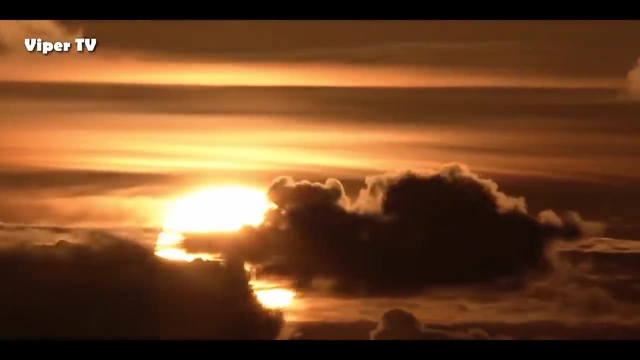 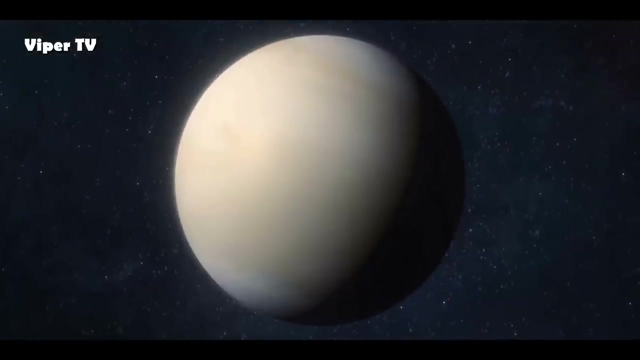 a world held in a delicate balance. With the sun weakened and restrained, the Earth-like atmosphere of Venus could act as a gentle blanket, keeping the surface temperate and covered in an abundance of liquid water. But even with this additional solar energy, we think Venus would still have been much cooler than the Earth is today. 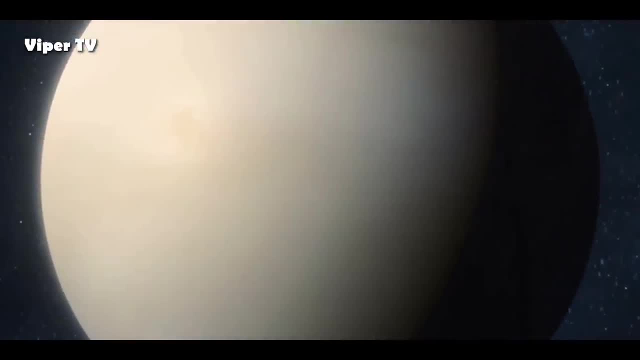 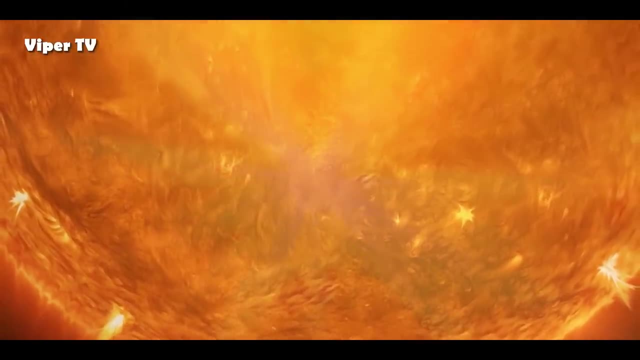 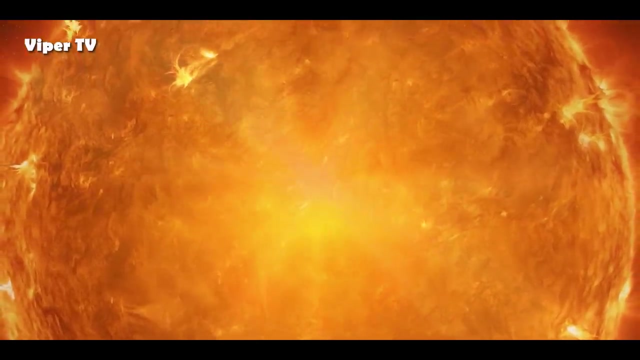 In fact, we believe temperatures at that time would have been like a pleasant spring day here on Earth. It wasn't to last. Slowly, the young sun grew brighter, its increased energy output causing temperatures to gradually rise, which in turn began to lift more and more water vapour into the air. 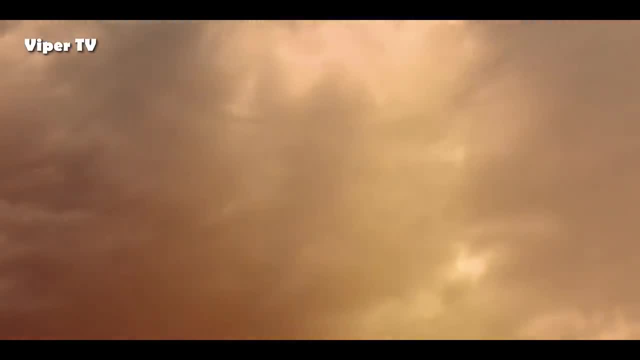 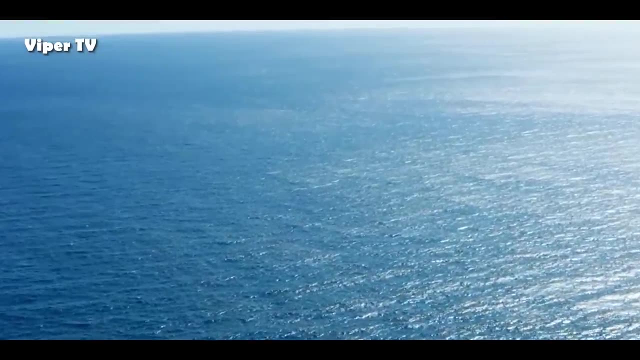 thickening the atmosphere and sealing the planet. The Earth was a planet that was in a state of unhappiness. It was a planet that was in a state of unhappiness, and it was a planet that was in a state of unhappiness because it was not aware of its fate. 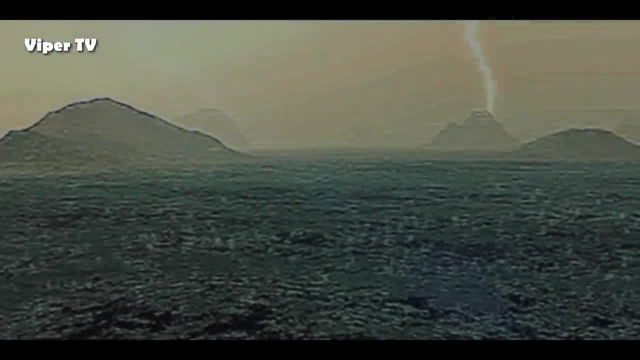 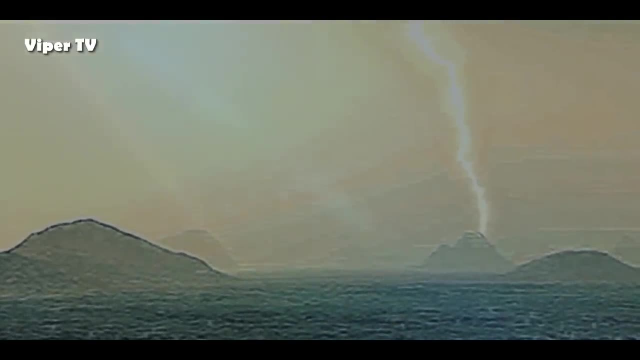 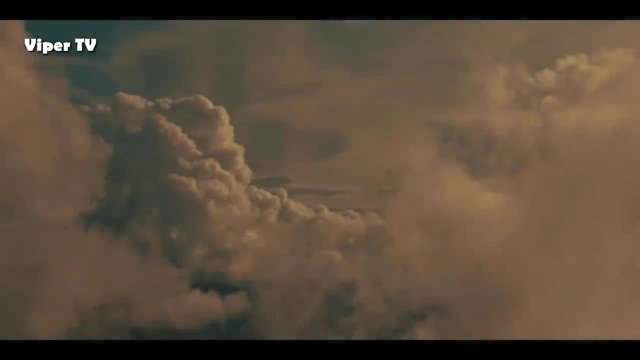 Although the oceans of Venus may have persisted for billions of years, as the surface warmed and the atmosphere thickened, the destiny of this planet was already set, driven by an unstoppable process we have recently become very familiar with here on Earth. The greenhouse effect is a process that has the power. 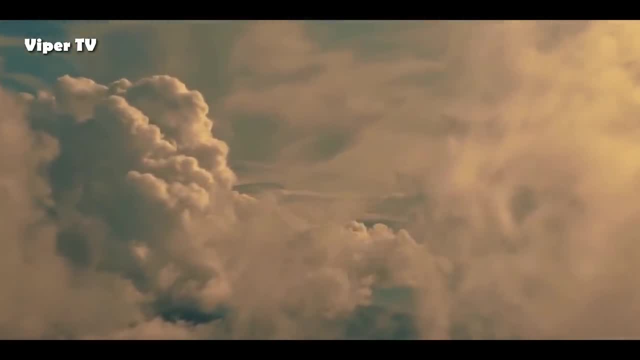 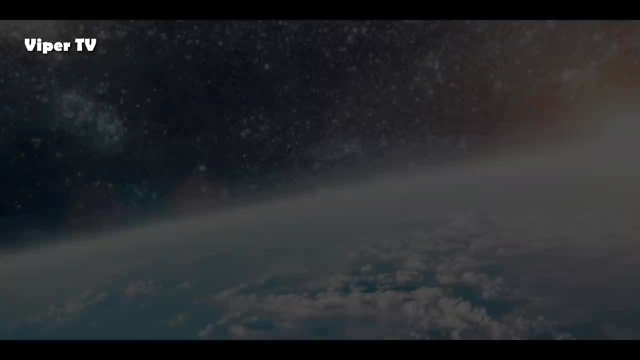 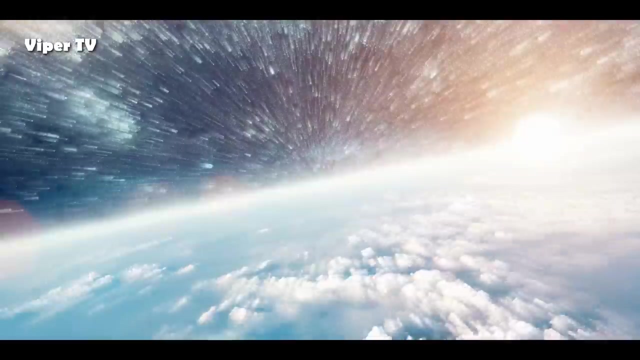 to change the atmosphere. It actually boils down to some pretty simple physics. It's all about how sunlight, solar radiation, interacts with the constituent parts of an atmosphere. In the case of the Earth, as solar radiation hits our atmosphere, some of it is reflected straight back out into space. 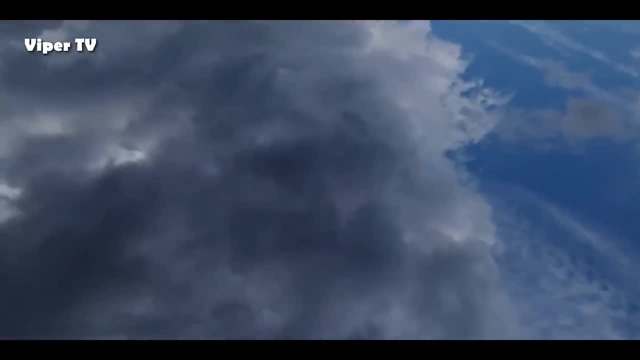 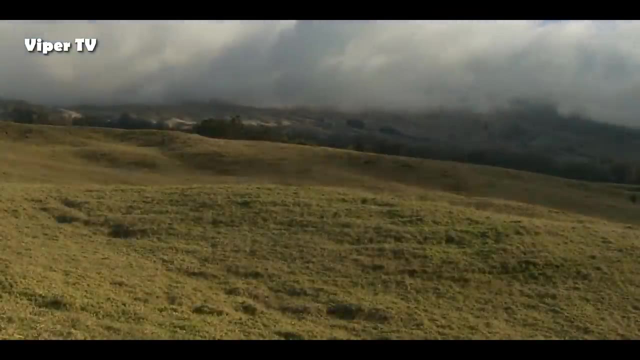 some is absorbed by the atmosphere and clouds, but most of the sunlight- about 48%- passes straight through the atmosphere and is absorbed by the Earth's surface, which is what makes it visible, The reason so much solar radiation makes it to the surface. 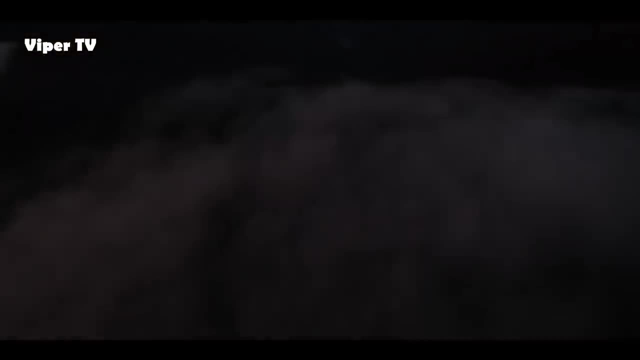 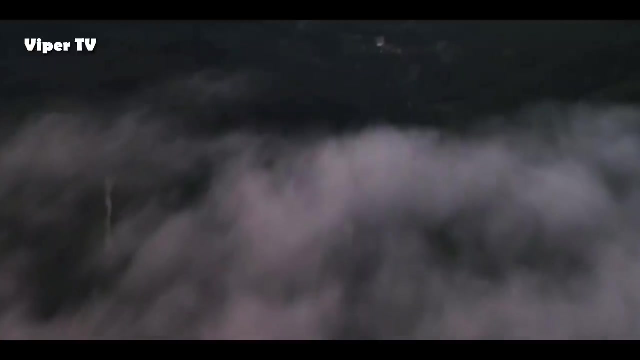 is because the gases in our atmosphere, like water, vapour and carbon dioxide, are transparent to light in the visible spectrum. When you think about it, that's pretty obvious, because there's a source of visible light in the sky- the Sun- and we can all see it. 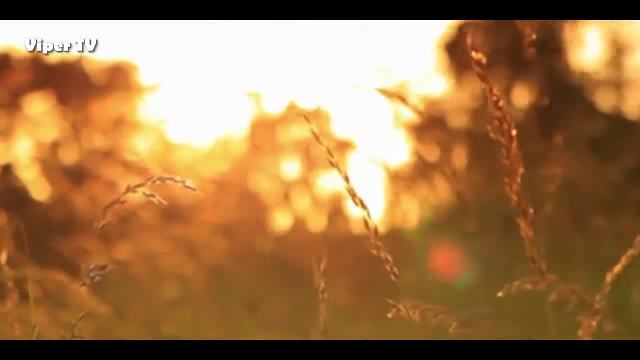 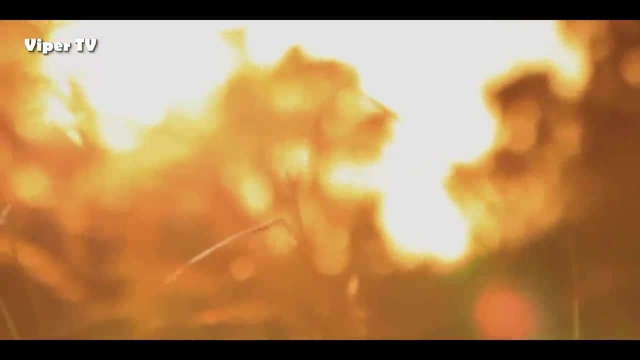 But it's a different story when that sunlight heats the surface of the Earth and re-radiates back out not as visible light but as the longer wave infrared light, the thermal radiation. We can't see this light, but as it radiates back out from the Earth's surface. 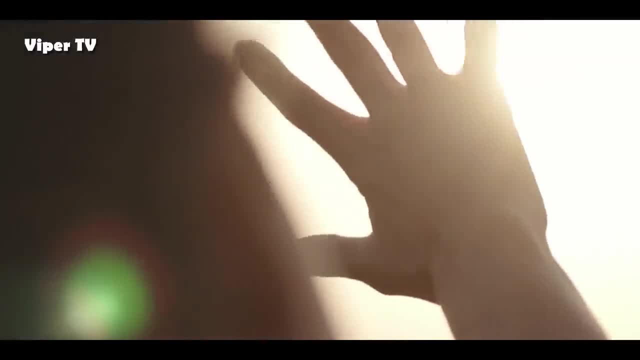 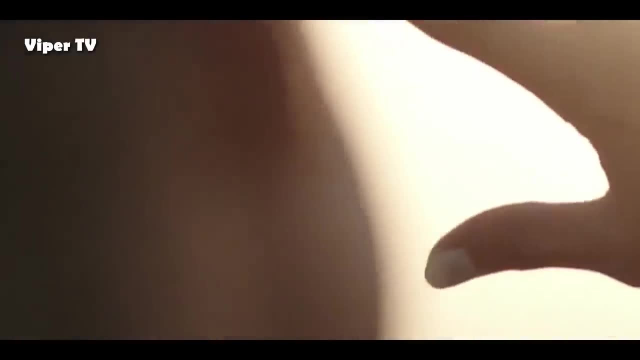 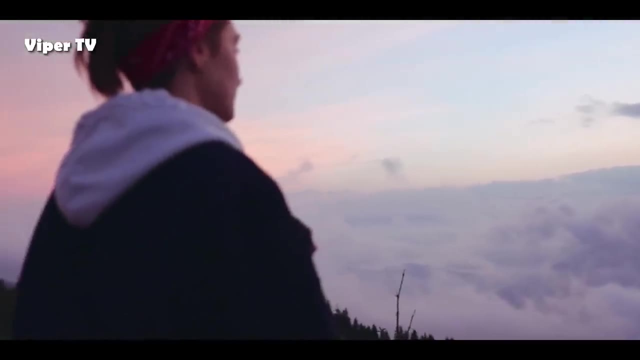 carbon dioxide and water vapour absorb the infrared, trapping that energy, and so the planet maintains a higher temperature. that is intimately linked to the constituent parts of the atmosphere, The higher its level of gases like water vapour, carbon dioxide, methane and ozone. 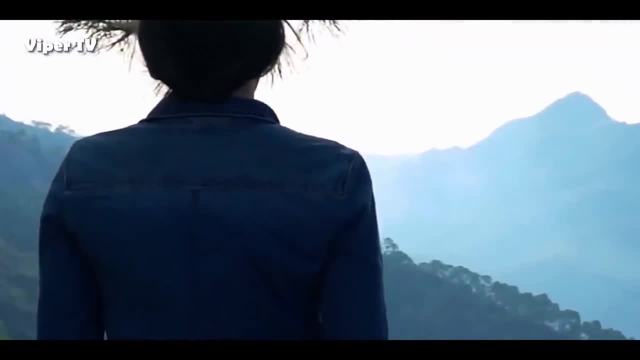 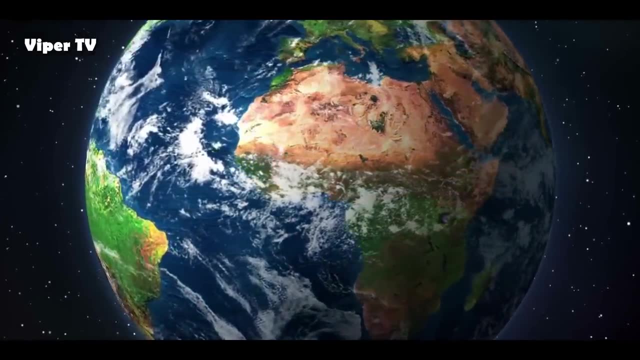 the greater the greenhouse effect and the bigger the uplift in temperature. Despite the very real threat that this now poses to the future of our planet, the greenhouse effect on its own is not necessarily a bad thing. The Earth would be at an average temperature. 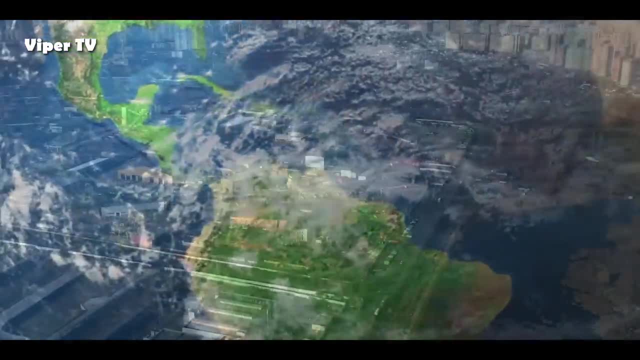 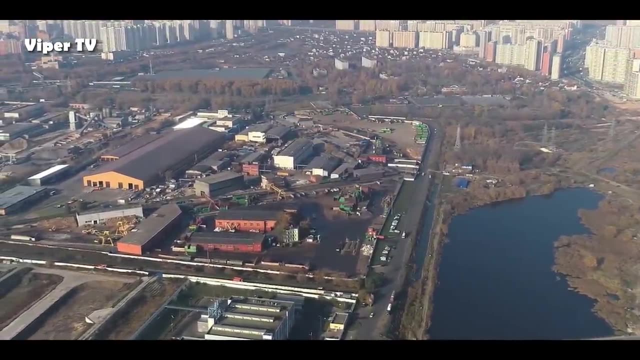 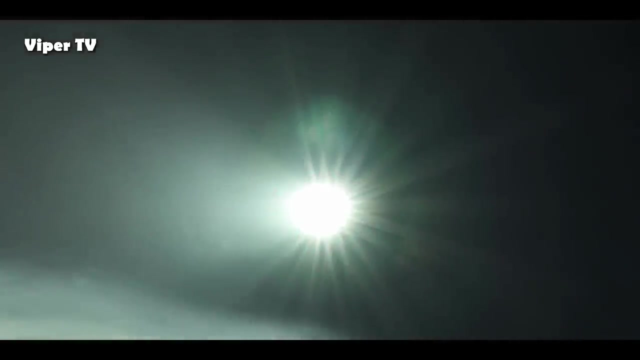 of around minus 18 degrees Celsius without it. But, as we are currently witnessing here on Earth, shift the balance of those gases and things can change very quickly At some point in Venus's past, the levels of water vapour lifted into the atmosphere by the warming Sun. 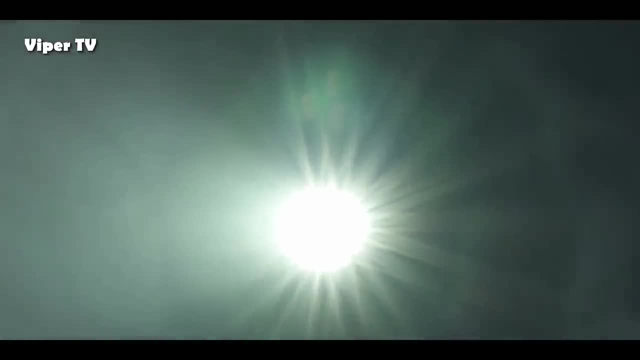 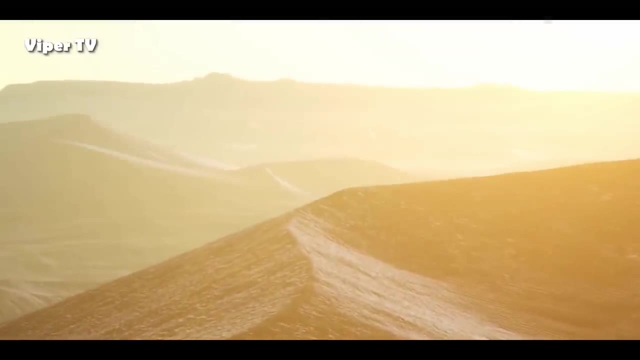 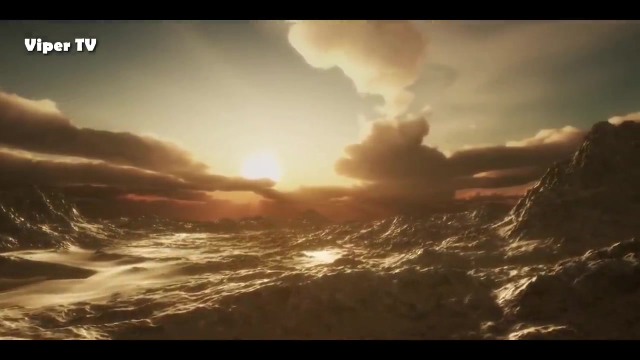 pushed the greenhouse effect to become precariously more intense. With less and less of the Sun's energy escaping, the ambient, temperatures began to rise exponentially until the day came when the last raindrops fell onto the surface of the planet, the heat evaporating the rains long before they could reach the ground. 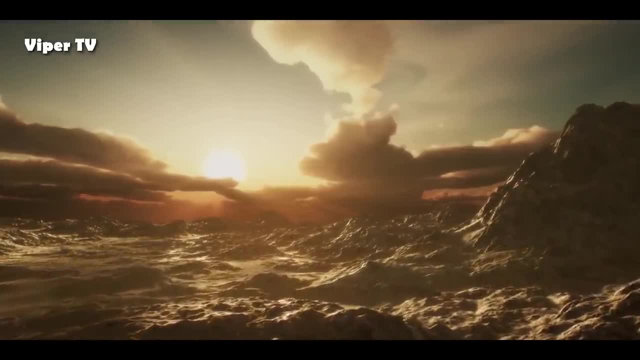 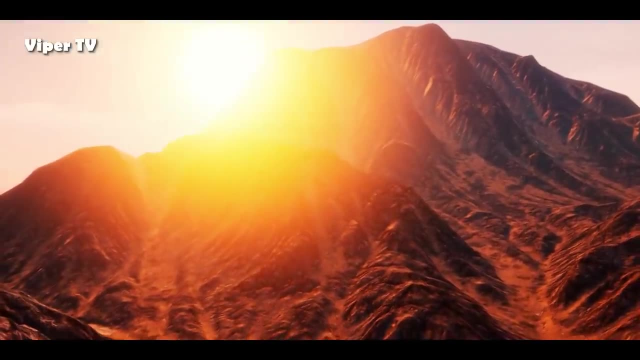 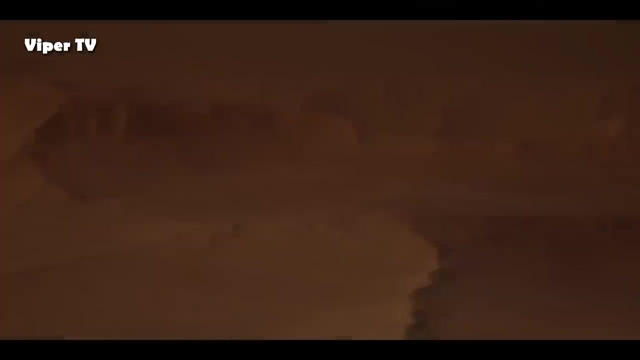 Venus had reached a tipping point. With the increasing temperatures feeding more and more water vapour into the atmosphere, a runaway greenhouse effect took hold, driving away the oceans. This led to the surface of the planet getting so hot that carbon trapped in rocks was released into the atmosphere. 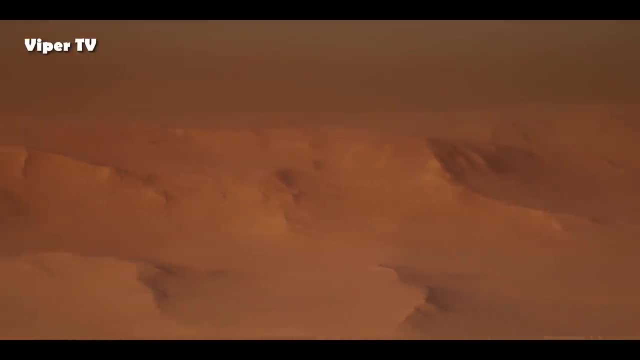 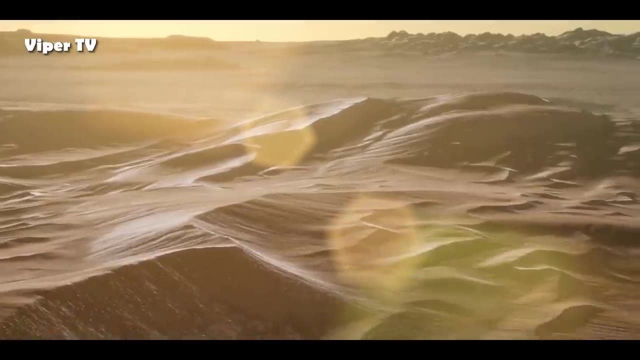 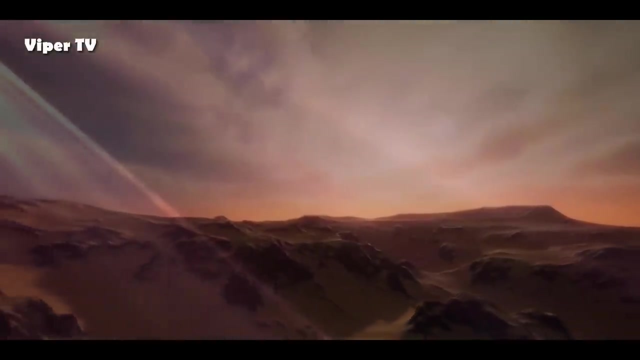 mixing with oxygen to form increasing amounts of another greenhouse gas, carbon dioxide, With no water left on the surface and no other means to remove it. carbon dioxide built up in the atmosphere, setting the planet on a course that would result in the scorched body that we see today. 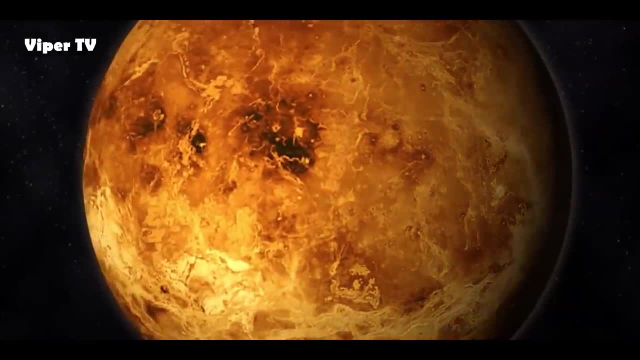 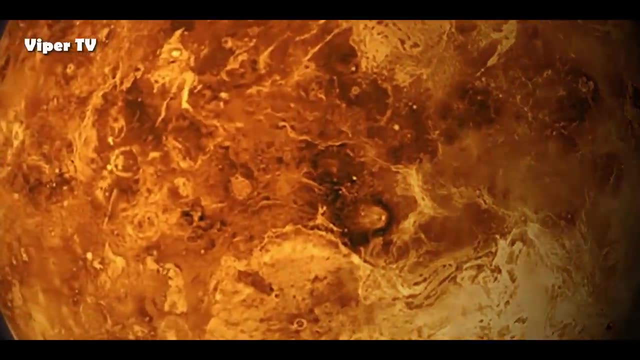 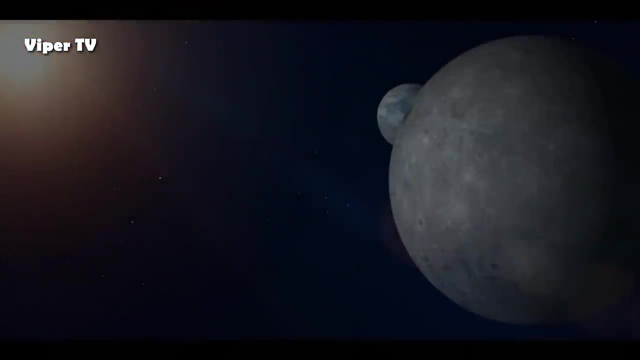 And so Venus's moment in the Sun came to an end. Earthlings, take note: When it comes to the greenhouse effect, there is a precariously thin line between keeping a planet warm and frying it. Of the four rocky worlds, only one has managed to navigate through the instability. 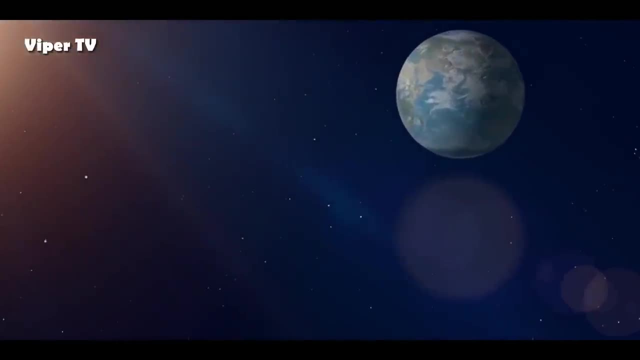 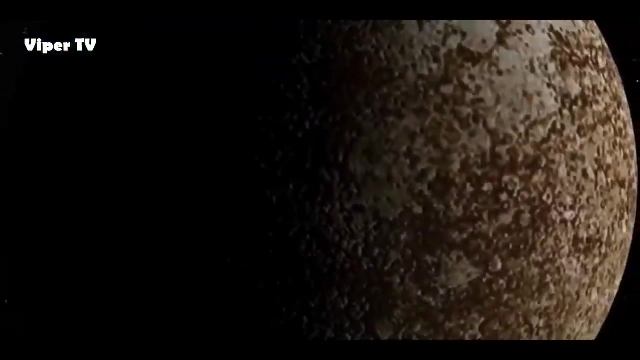 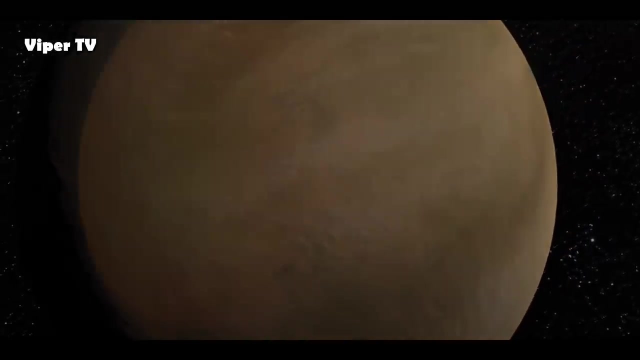 and constant change of our solar system over the last four billion years and maintain the characteristics needed to support life. Mercury lost its fight early, as it was flung inwards towards the Sun. Venus flourished at first, before slowly coming to the boil, and Mars, the runt of the litter. 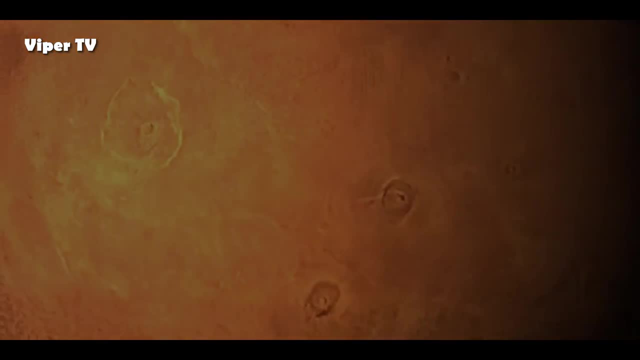 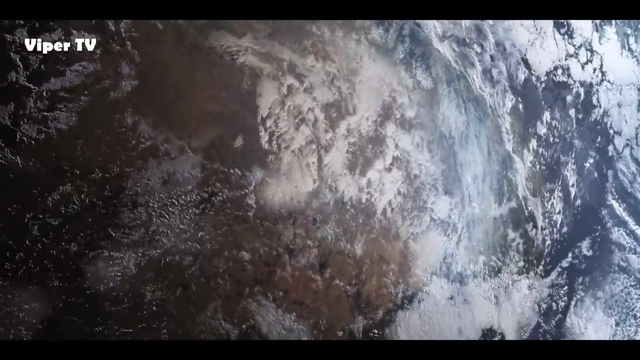 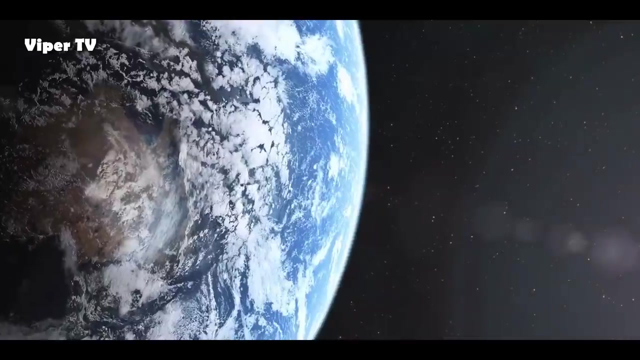 became a frozen wasteland long ago. Only Earth, uniquely among the planets, has persisted with an adequate stability over the last four billion years to allow liquid water to remain on its surface and an atmosphere just thick enough to keep its climate calm, not too hot and not too cold. 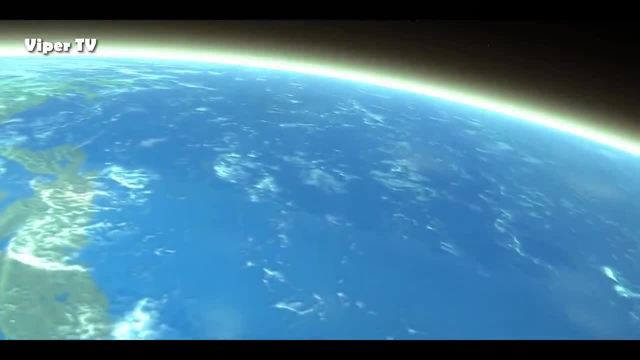 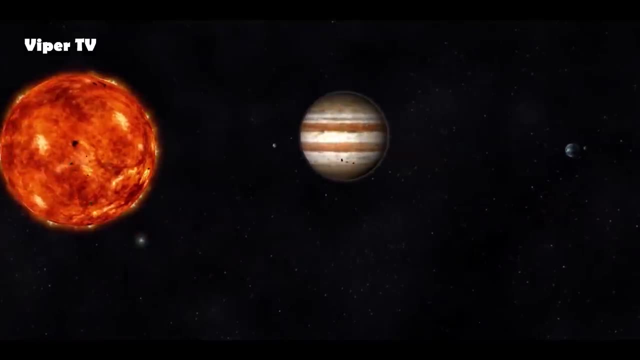 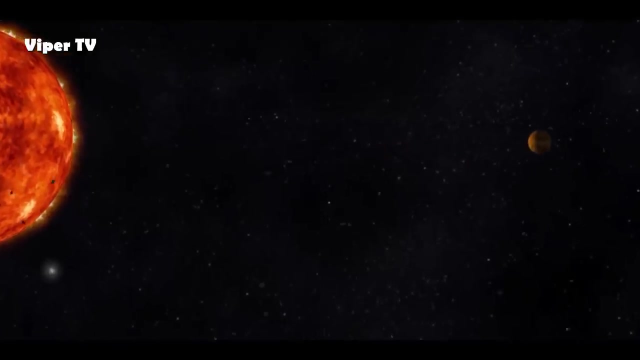 Events have rocked us, and extremes of temperature have waxed and waned, but never outside of the parameters needed to harbour life In a chaotic solar system filled with planetary might-have-beens, Earth is a shining example of stability, And the evidence for this is to be found in every nook and cranny of the planet. 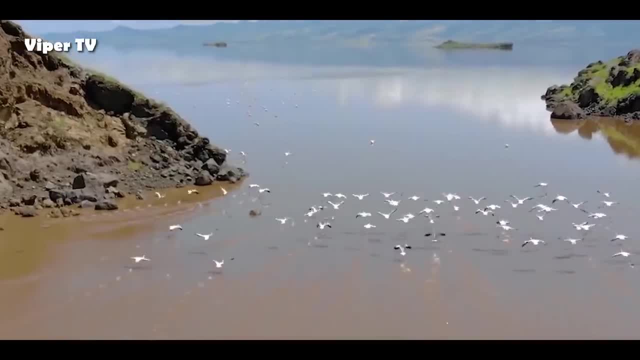 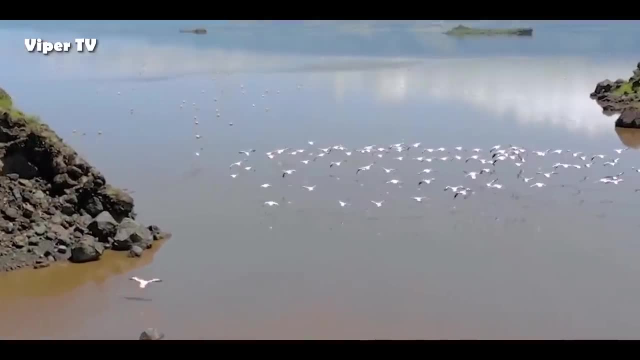 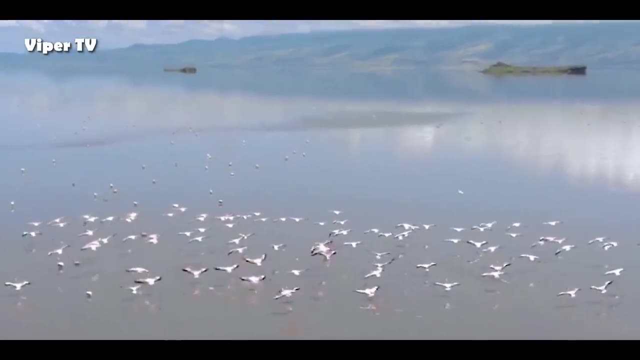 Today, Earth is dominated by life. The land and seas are teeming with millions upon millions of species, with thousands of new life forms discovered each year. Somehow, even when disaster threatened, the Earth has remained a living world, While endless species have come and gone. 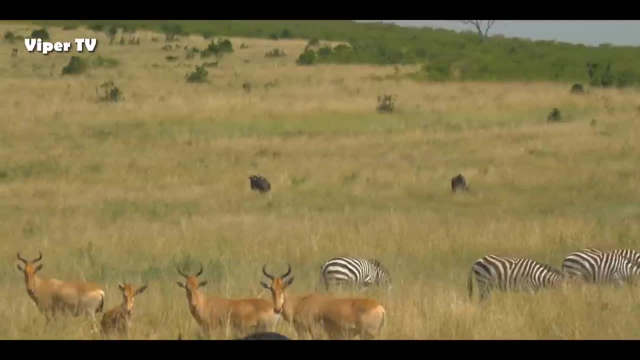 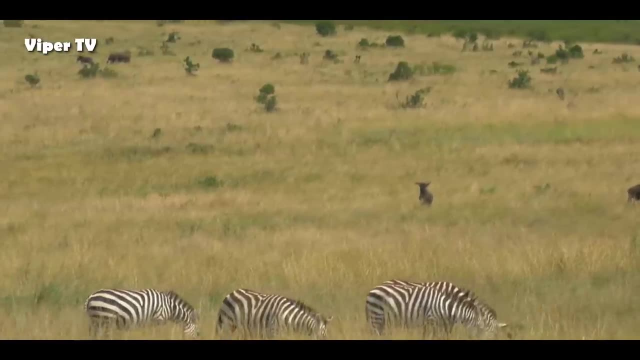 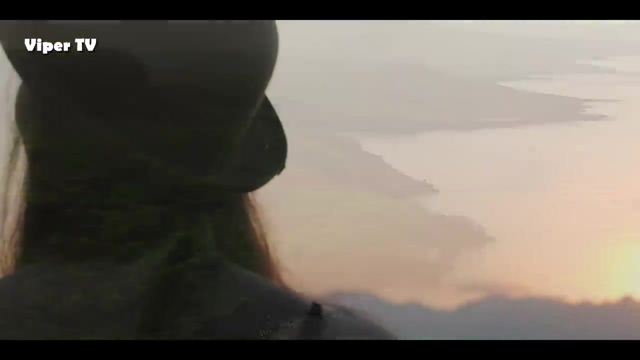 life has always persisted. It's woven into the fabric of the planet, an integral part of every continent and every ocean. Life plays a crucial role in maintaining the balance of the atmosphere that keeps our planet temperate, But we know for certain it cannot last. 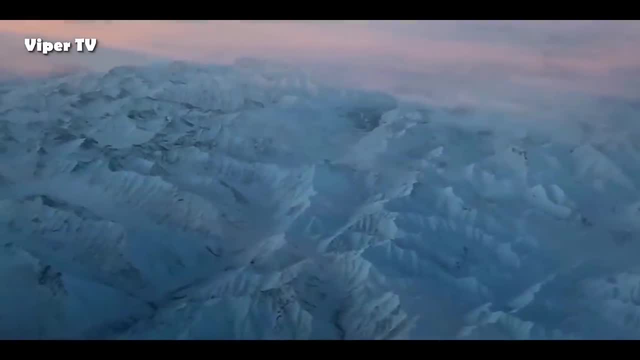 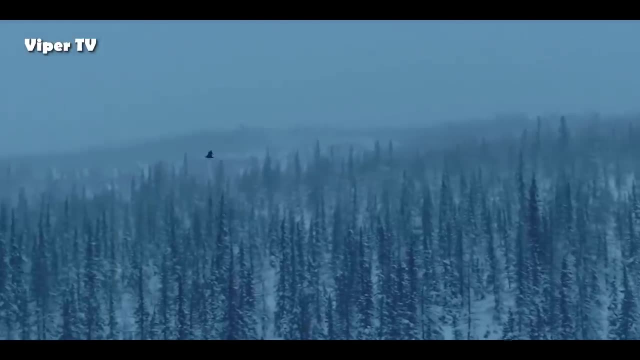 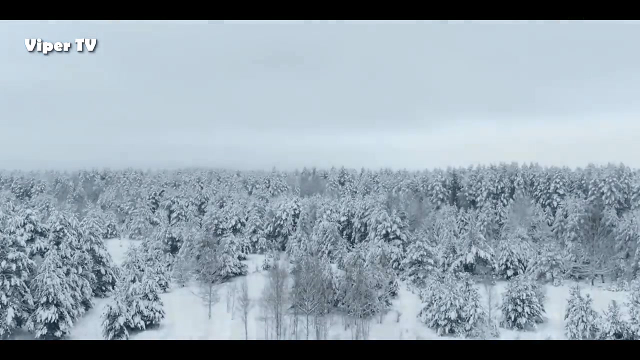 The Kamchatka Peninsula in eastern Siberia is one of the most inhospitable places on Earth, A volcanic wasteland peppered with thousands of hot springs. it's here that we find some of the toughest living things. Extremophiles survive here. 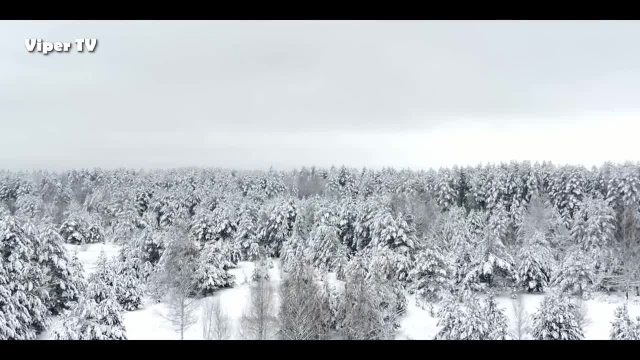 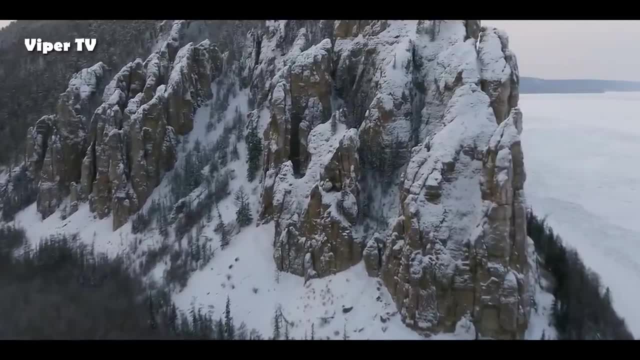 that are able to withstand temperatures and pH levels higher than any other land-based life forms we have ever discovered. Kamchatka is part of the Pacific Ring of Fire and, despite its remoteness, biologists have long been enticed here to explore its toxic bubbling cauldrons. 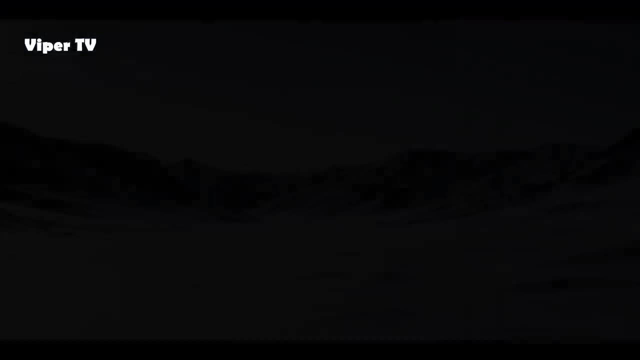 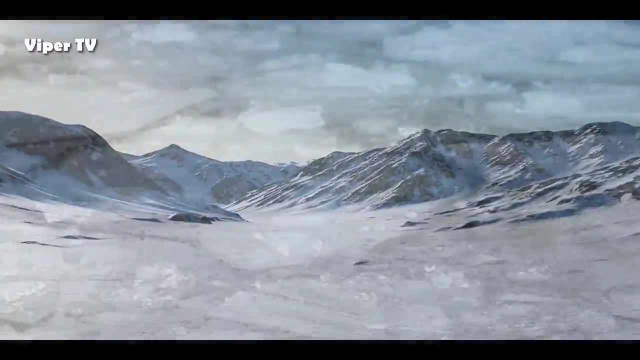 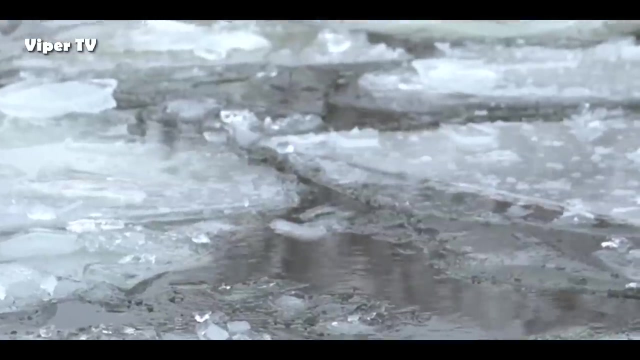 for signs of life. Complex life, animals and plants struggle to survive in temperatures above 50 degrees Celsius. So searching for life here is all about searching for single-celled life forms, bacteria and archaea- ancient microorganisms that are somehow able to endure in this hostile environment. 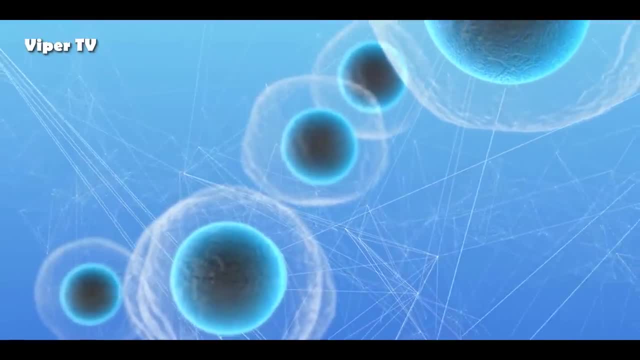 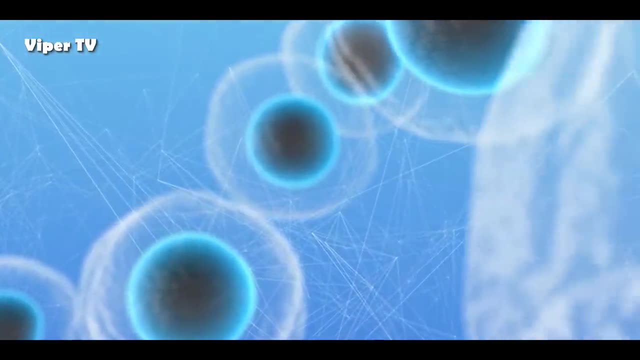 Life forms like Acidilobus aceticus, an archaea that can be found in a hot spring where the water is so acidic it reaches a pH of 2, and where temperatures rise to 92 degrees Celsius In other parts of the hydrothermal field. 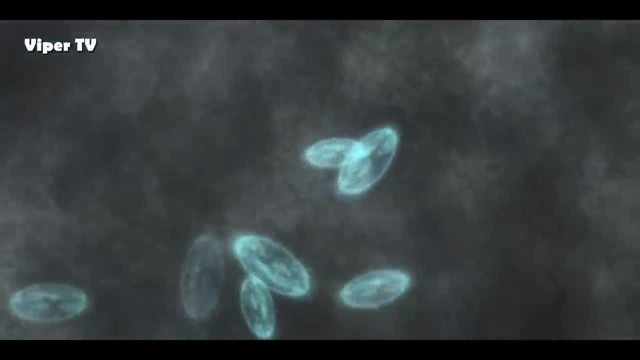 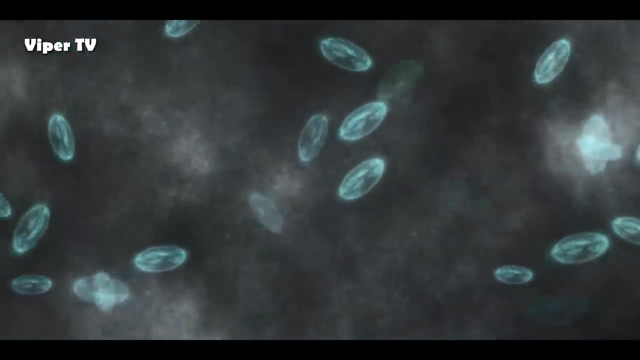 bacteria like Desulfurella acetivorans have been discovered, which happily live in pools that are touching 60 degrees Celsius, but it's these that are the real hotheads. In one of the biggest and hottest pools investigated by scientists, a large number of microbes have been found. 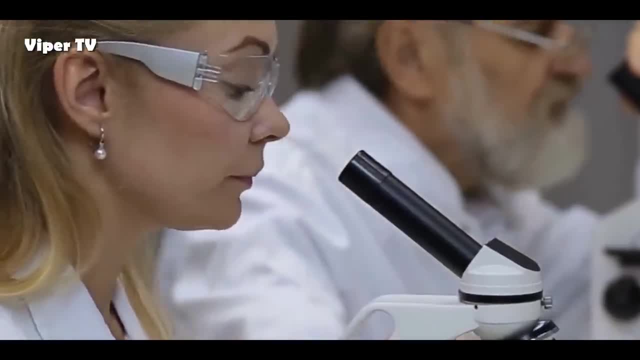 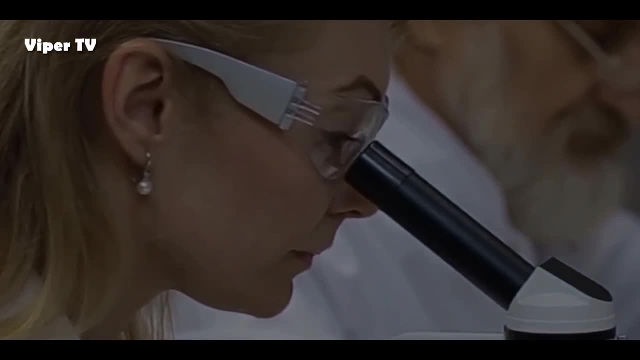 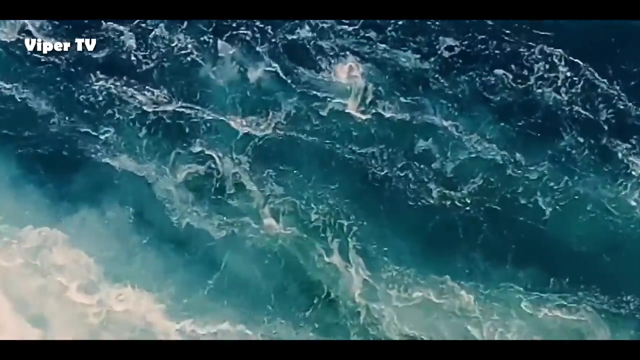 living in temperatures approaching 97 degrees, making it one of the most dangerous, if not the hottest environment ever studied for signs of life on land. But to find the greatest hotheads on planet Earth you need to look not on land but deep beneath the sea. 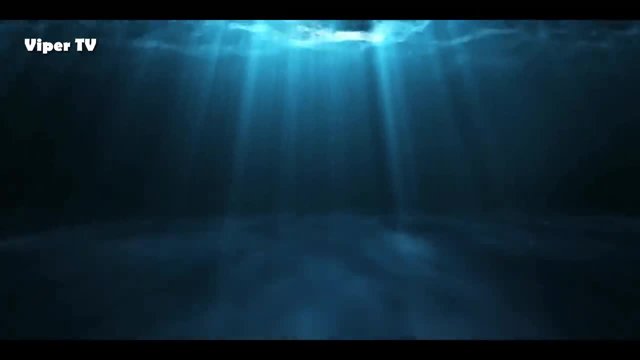 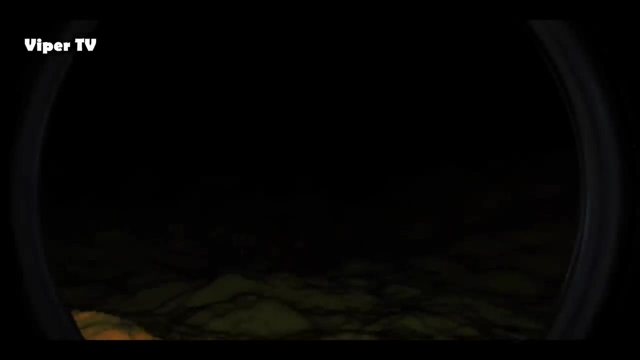 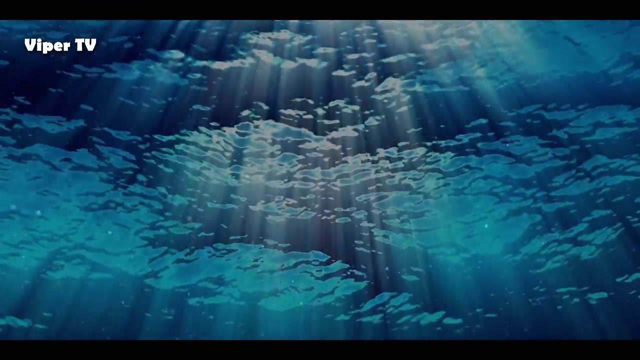 In the furthest depths of the Atlantic, around the black smoker hydrothermal vents blurting out of the ocean floor, we found strains of archaea that can survive temperatures of 122 degrees Celsius and perhaps even higher. These rare life forms live at the very edges of biology. Unique adaptations to their cellular chemistry enable the proteins and nucleic acids that create the structure of the microorganism to function, while the membranes that are protecting the cells utilize different fatty acids and lipids to keep the cells stable at the higher temperatures. Perhaps there are even tougher life forms that we are yet to discover. 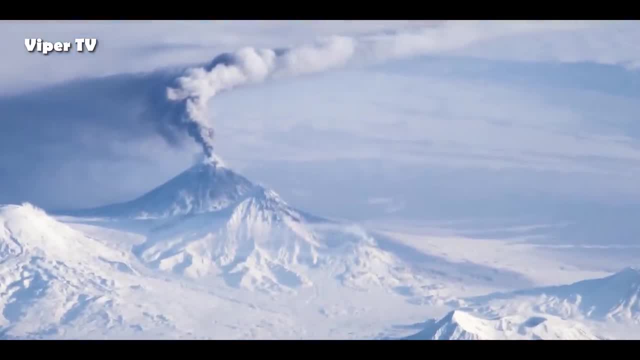 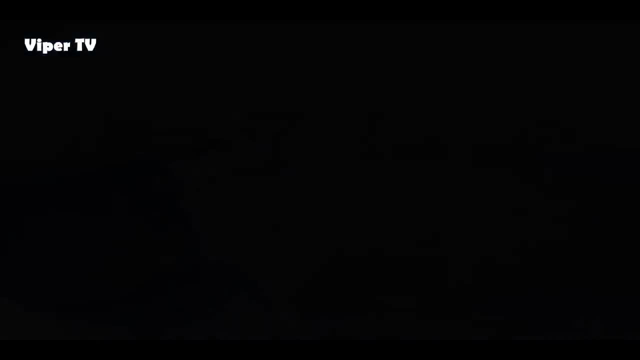 but the thermophilic microorganisms that we have so far identified and investigated in places like Kamchatka all point to the fact that life has its limits. Evolution by natural selection can only adapt so much, and even though it's impossible to imagine what life on Earth 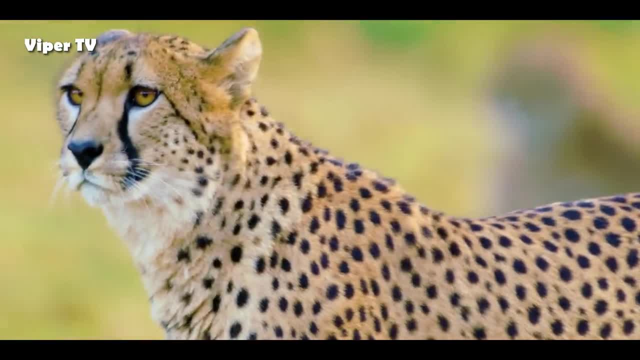 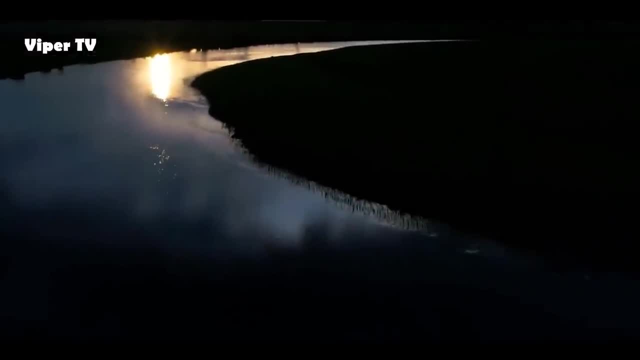 will look like in a few hundred million or even a few billion years' time. we know that biology is constrained by thermodynamics, And so we can say with some certainty that there will come a time when the Earth is too hot for any living things to exist. 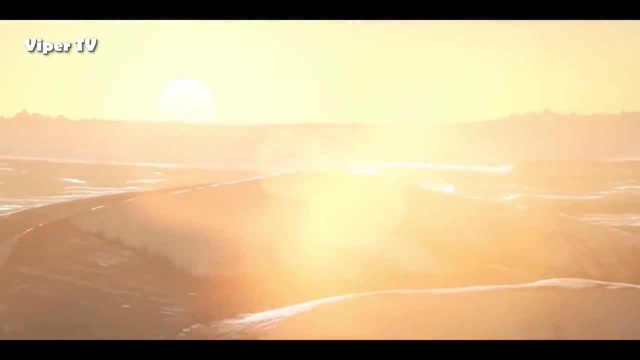 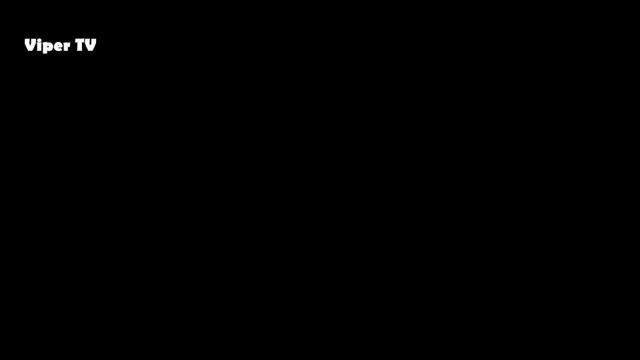 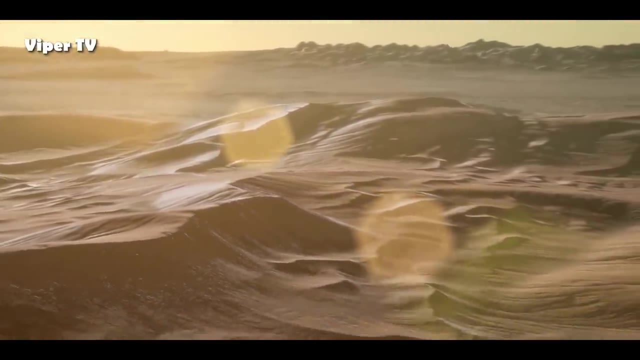 Natural selection will eventually run out of options as the laws of physics outplay it, and all life will come to an end. When this will happen, no-one can be certain, But as the Sun ages and grows, hotter, temperatures on Earth will rapidly rise. 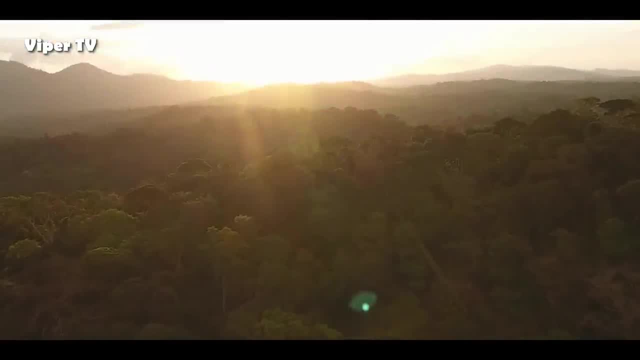 Today, the average surface temperature on the planet is 14.9 degrees Celsius, But with just a 10% rise in the Sun's luminosity, the average temperature will rise to 47 degrees, And that's the average temperature on Earth. The increased temperatures will raise great storms across the planet. The rains will remove carbon dioxide from the atmosphere and it will be locked away as newly formed sedimentary rock Trees and plants will struggle as they are robbed of the gas that sustains them. 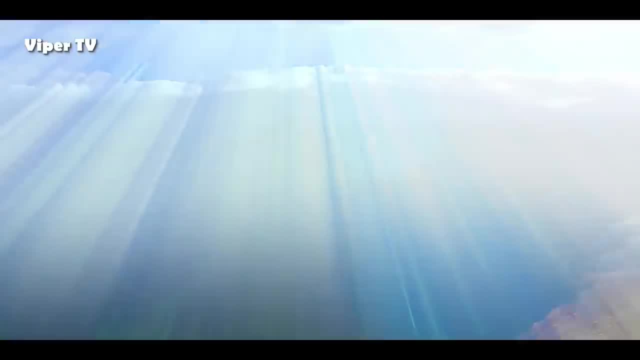 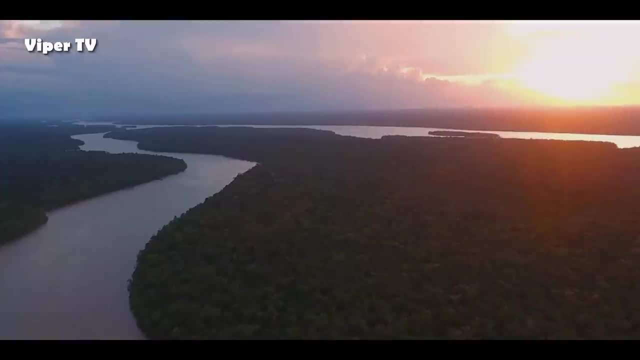 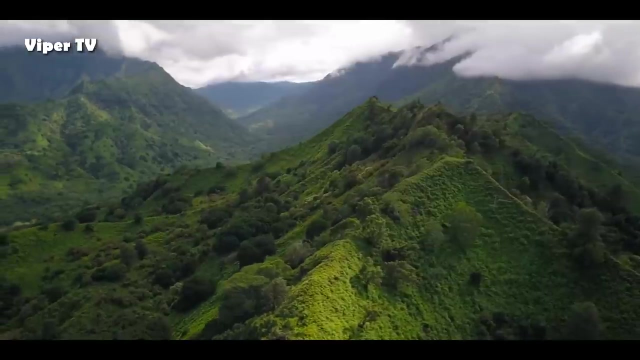 until eventually, photosynthesis will cease, The lungs of our planet will fail and the precious oxygen that green plants and algae produce will dwindle. With the primary food source gone, the food chain will collapse and the age of complex life on Earth will draw to a close. 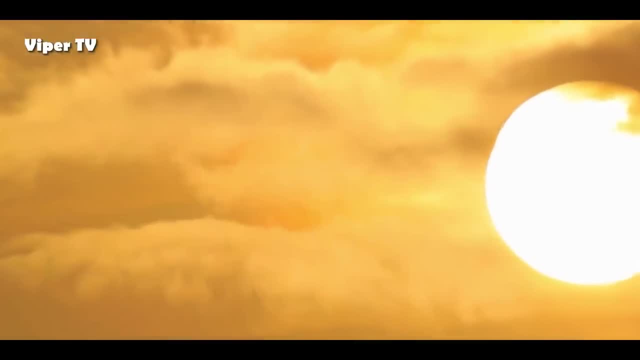 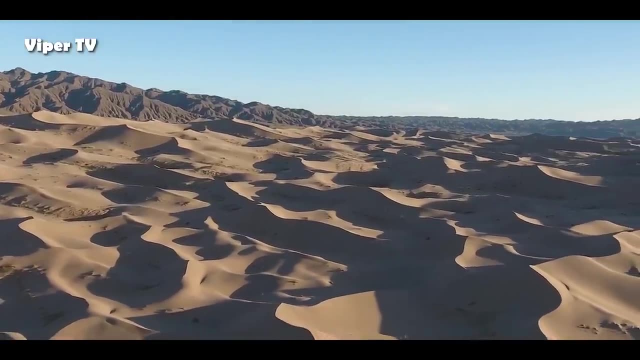 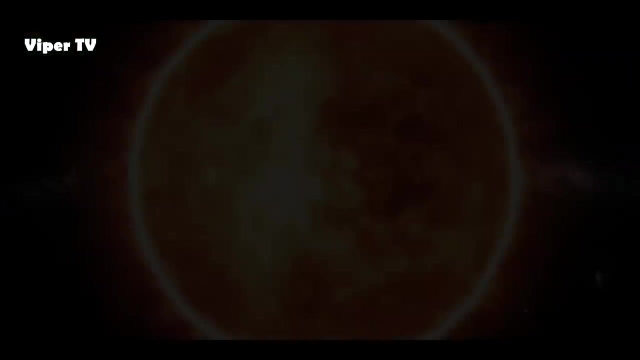 Heat-loving extremophiles may flourish for millions of years more, but eventually nuclear physics will have its way And, as average temperatures race above 100 degrees Celsius, the last pockets of life will be extinguished from the Earth. We can say with confidence: this is going to happen. 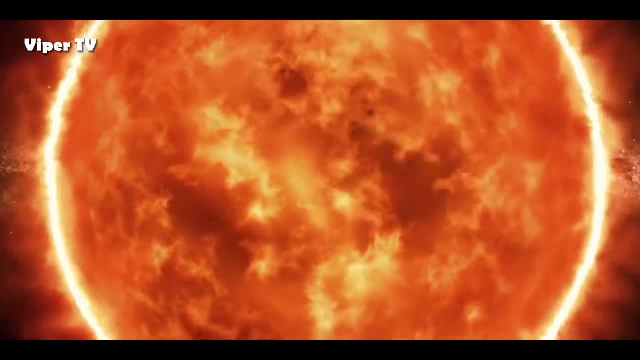 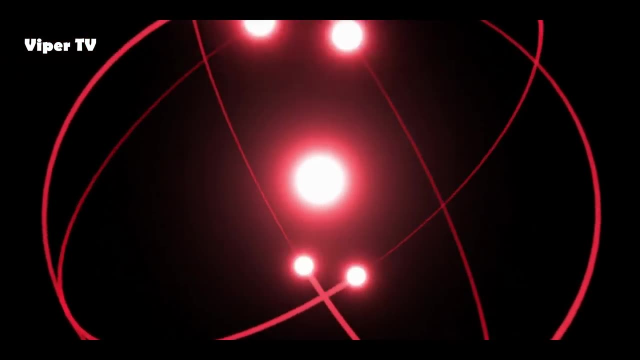 because we can plot the future. We can plot the future of our sun far more precisely than the future of the Earth. Our understanding of nuclear physics allows us to predict what happens inside the cores of stars, and thus we can see the past, present and future of stars like ours. 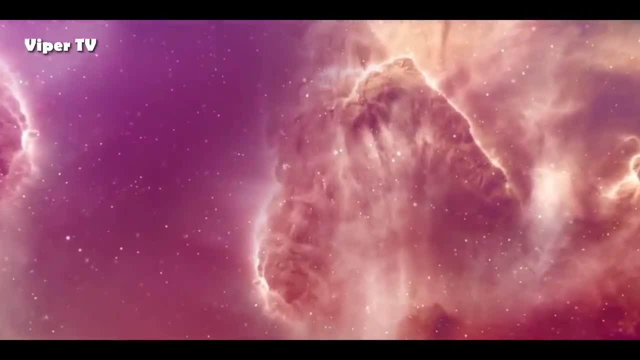 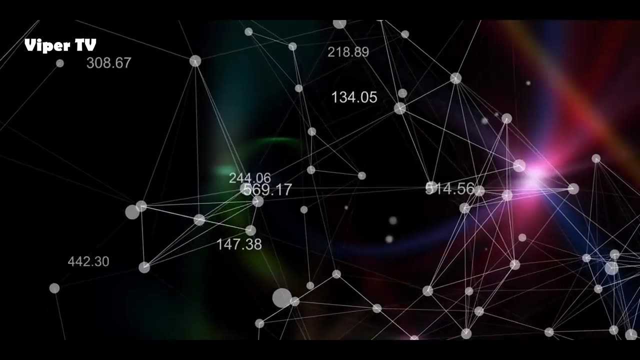 written. across the night sky. The heavens are filled with shining examples of stars that give us a glimpse into the future of our sun. Arcturus, for example, in the constellation Boötes, is one of the brightest stars in the Northern Hemisphere. 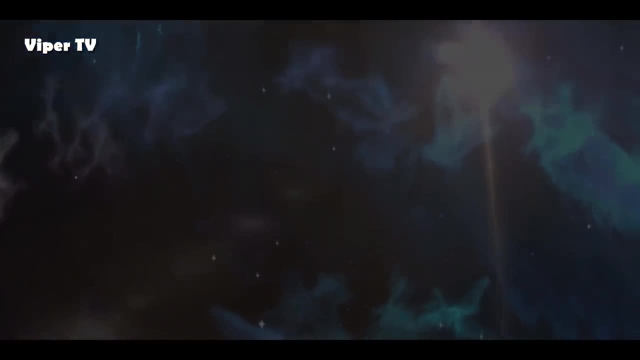 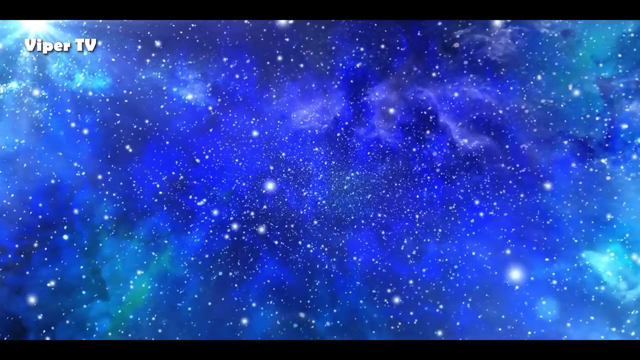 It's around the mass of the sun, perhaps a little bit heavier, and so, in the distant past, would have had remarkably similar characteristics to our own star. Today, though, Arcturus is 6 to 8 billion years old, potentially 3 billion years older than the sun. 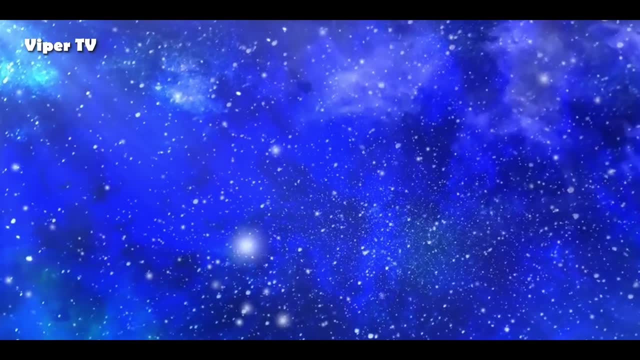 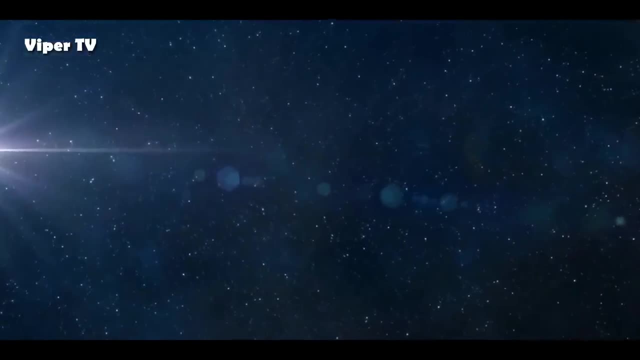 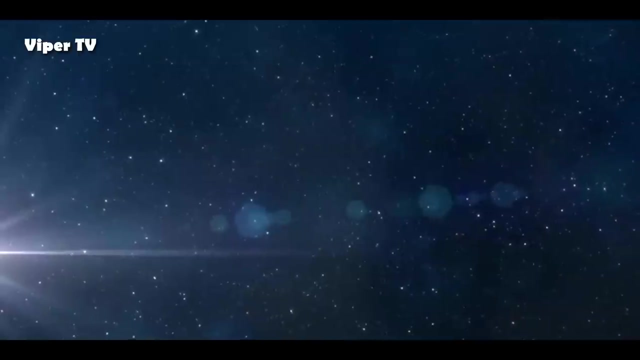 and, as it is no longer a main-sequence star, it is now in the red giant phase. It's fuel-exhausted. it has swollen up to 25 times its original diameter and is around 170 times as luminous, Despite the fact that, as its core slowly burns out, it is cooling. 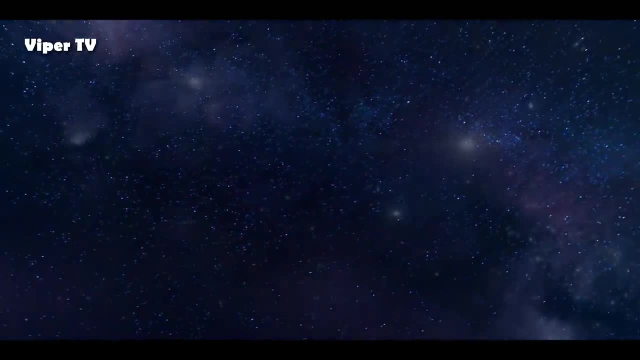 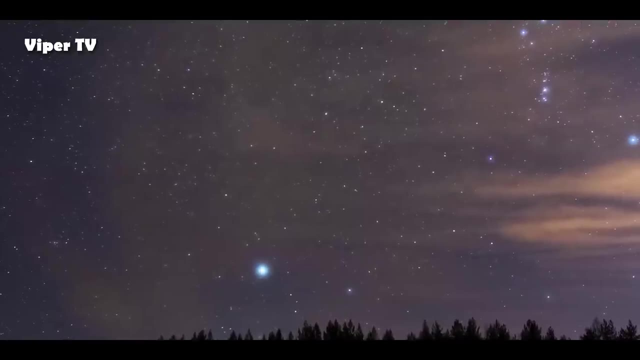 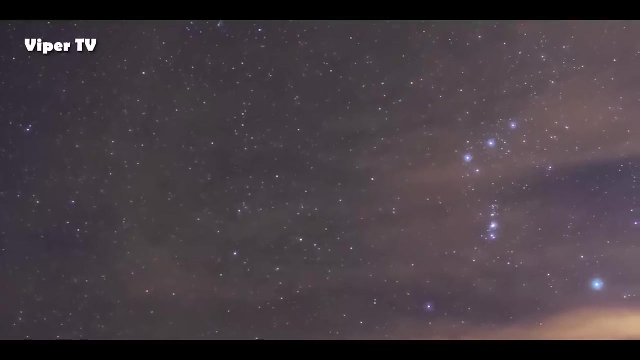 To see even further into the future, we need to look towards the brightest star in the northern sky, Sirius. The Dog Star, as it's commonly known, is twice the mass of the sun and still fully in the main sequence, But obscured by the glare of Sirius A, is a faint companion. Sirius B 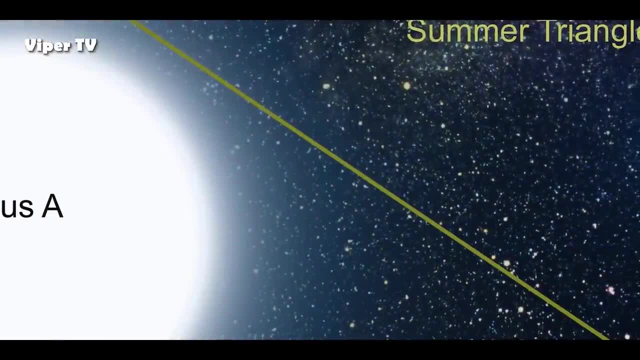 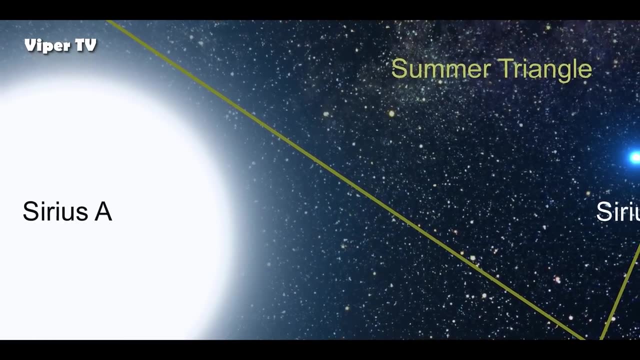 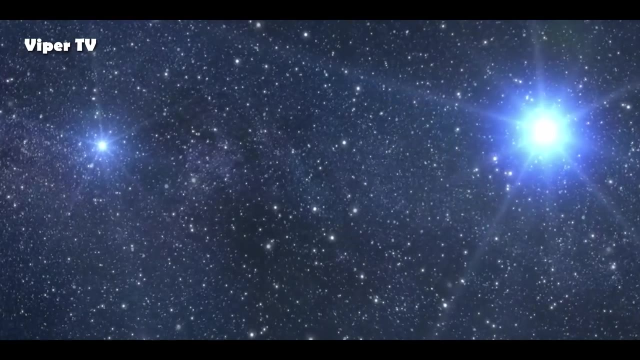 This is a star that has already burnt through its fuel, swollen into a red giant and the outer layers have drifted off into space, leaving the fading core of the star about the size of the Earth, known as a white dwarf. These stars are just two examples amongst many. 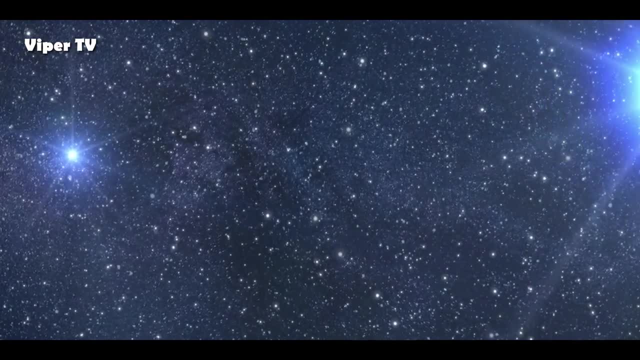 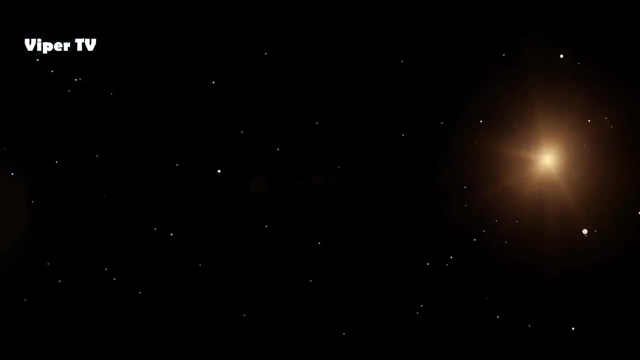 that point us towards the ultimate fate of our sun, a fate that we believe will play out over the next 5 billion years or so. Just like Arcturus, as the sun exhausts its hydrogen fuel, its outer edge will inflate and it will enter a red giant phase. 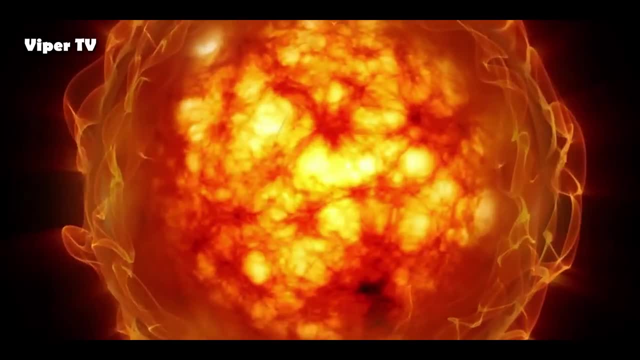 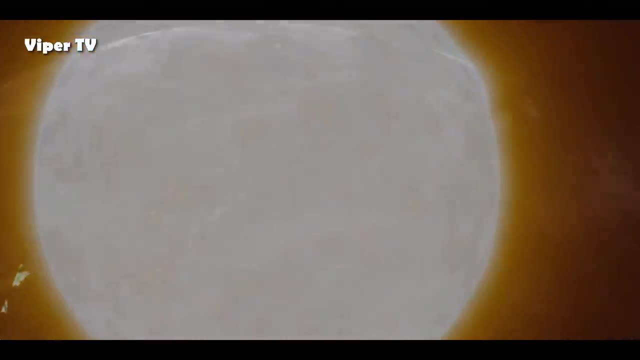 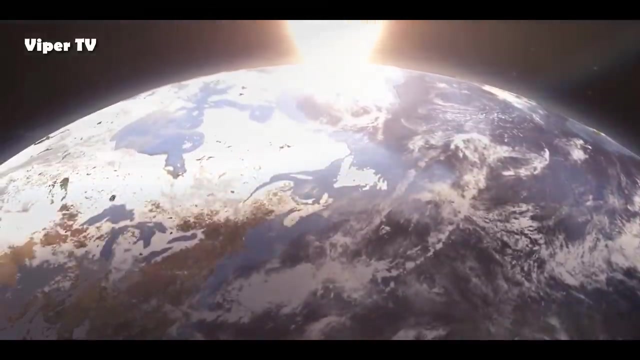 Expanding millions of kilometers out into space. it will engulf Mercury first. Venus's fate will be sealed next, as the sun expands further. Some models predict that Earth may just escape the fiery end of its neighbors, heated to 1,000 degrees Celsius. 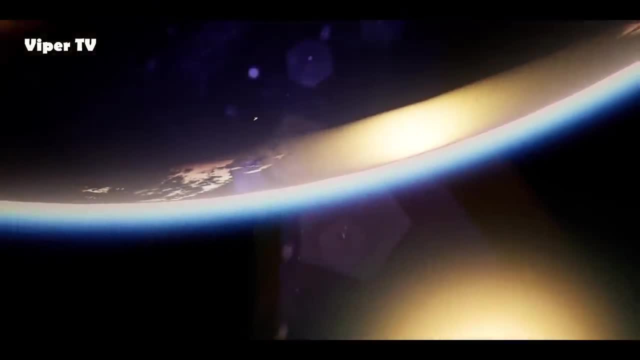 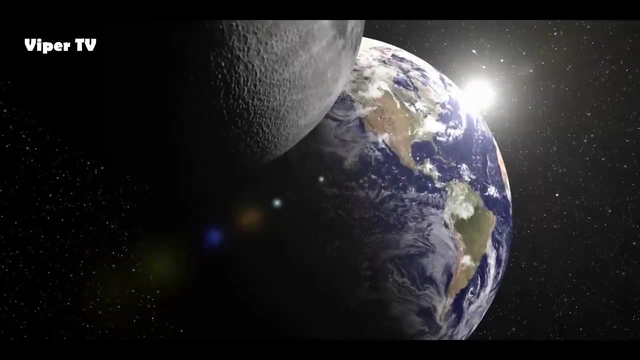 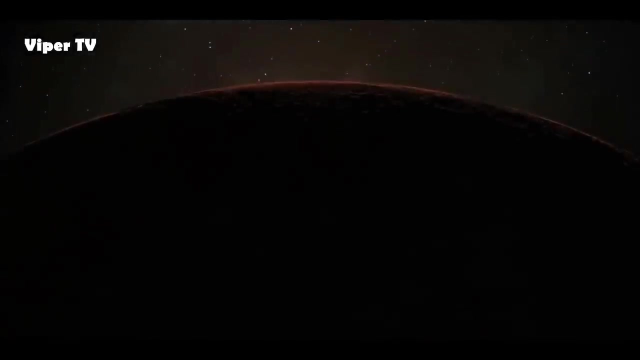 but hanging on beyond the edge of the dying star as its orbit extends out due to the lessening mass of the sun. Dead but not destroyed Earth and Mars will orbit as burned-out relics of their former selves. The era of the four rocky inner planets will be over. 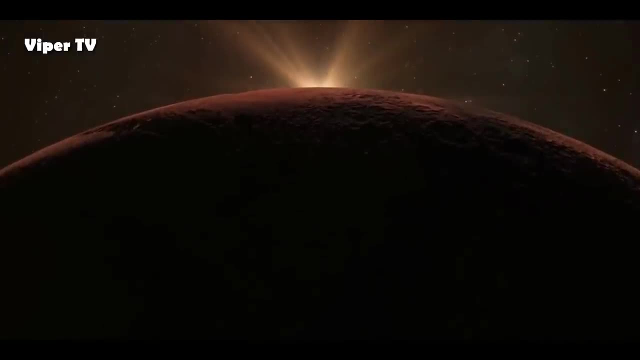 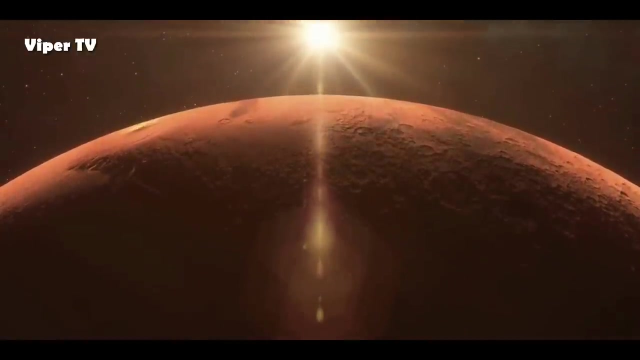 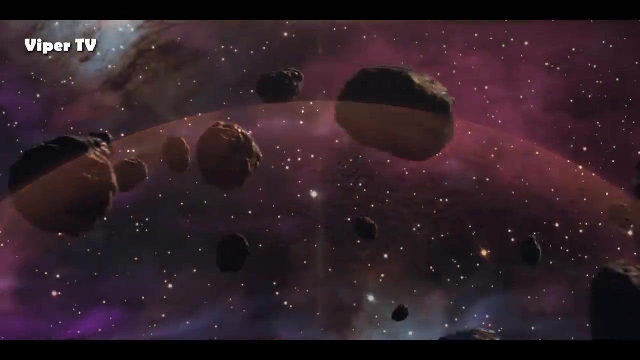 the billions of lives lived on the surface of one of them nothing but a distant memory. But within our solar system lies another family of rocky worlds whose moment in the sun may be to come Far beyond the asteroid belt, millions of miles away from the sun-drenched planets of the inner solar system. 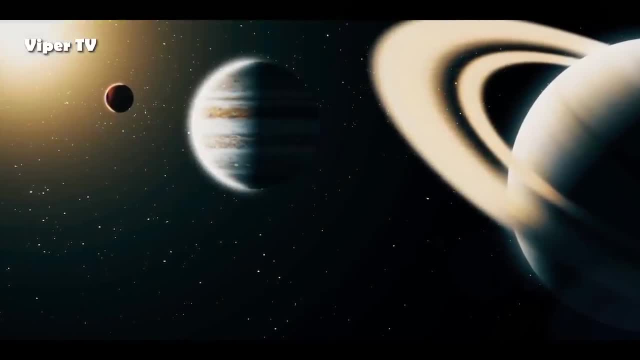 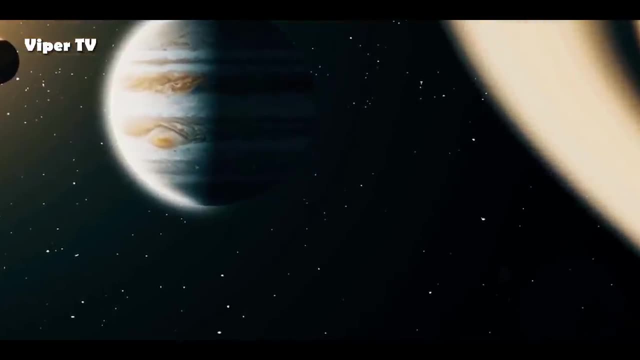 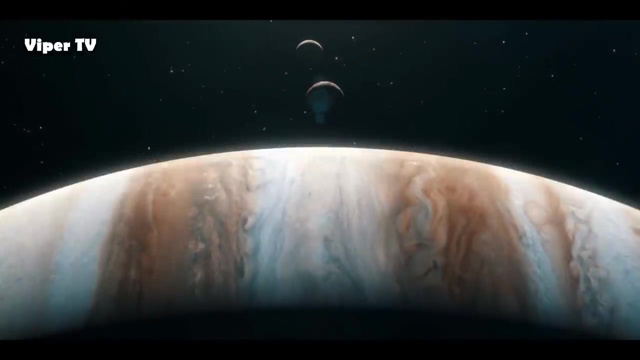 the gas giants of Jupiter and Saturn are home to another family of rocky worlds. Jupiter alone has 79 known moons orbiting it, a menagerie of satellites of multiple shapes and sizes. We've been peering at these moons since Galileo Galilei spotted four of them. 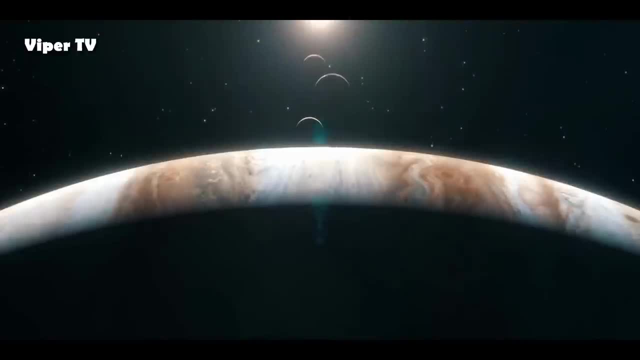 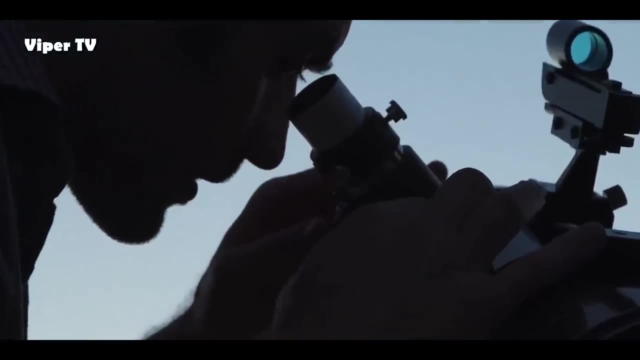 Io, Europa, Ganymede and Callisto, known as the Galilean moons, over 400 years ago, with his telescope, transforming our understanding of our place in the solar system. Today, we have explored the Galilean moons not just from afar. 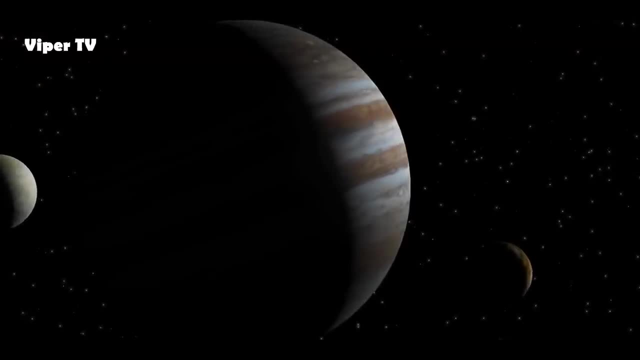 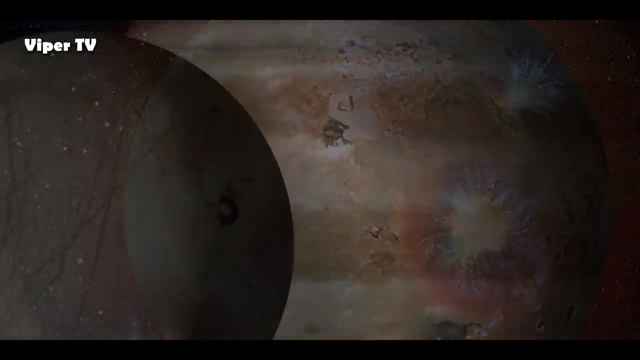 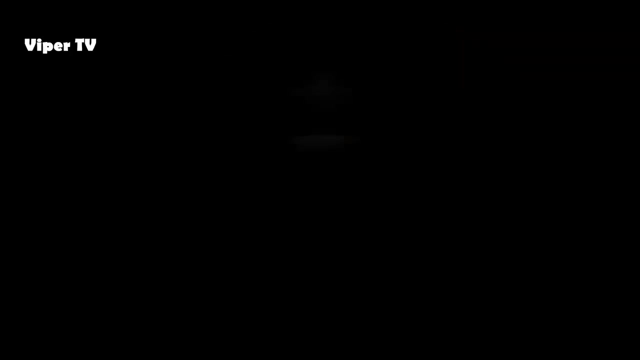 but close up and found them to be dynamic worlds. Io is fiercely volcanic and Europa. the ice moon shows tantalizing evidence on its surface pointing to a subsurface ocean sitting below its icy crust. Ganymede and Callisto make up the final two Galilean moons. 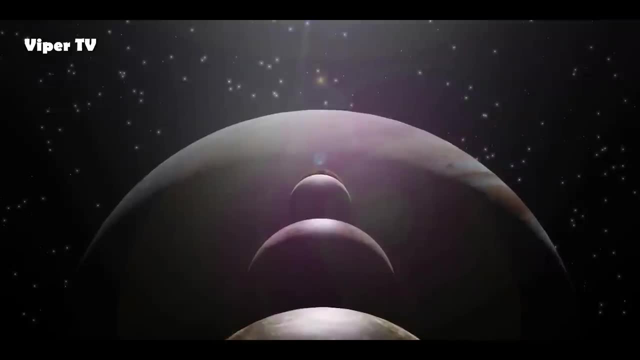 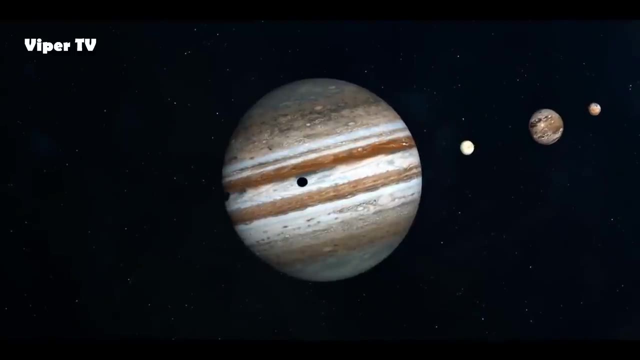 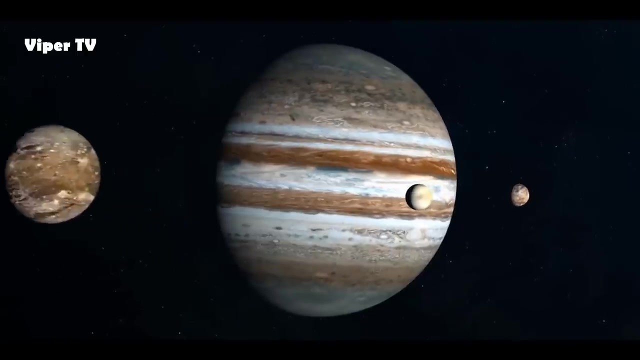 and just like Europa, they are rocky worlds with an abundance of water, ice on their surfaces and perhaps their own oceans lurking beneath. These three rocky, frozen worlds are all sitting in the cold outreaches of our solar system, touched by the distant sun but barely warmed. 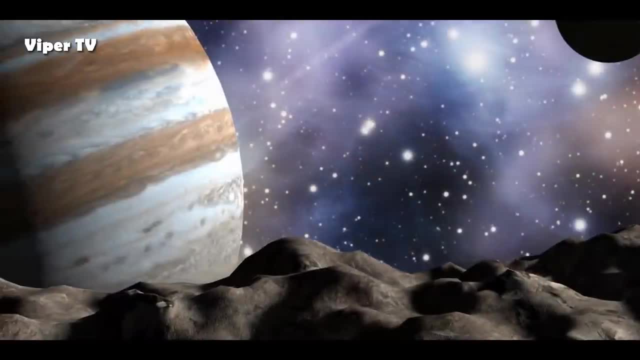 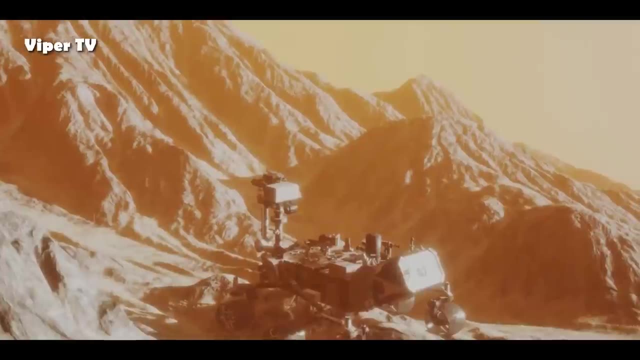 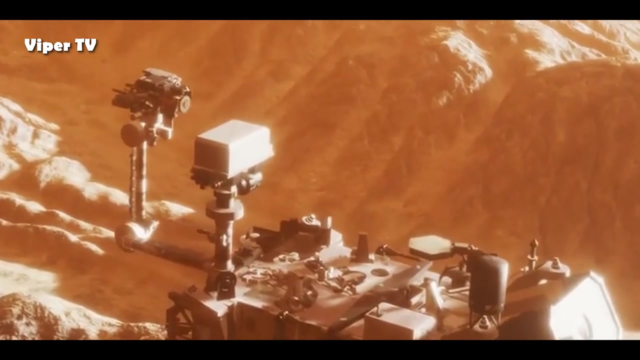 lying dormant until, perhaps one day, the aging sun will reach out and turn these bodies into ocean worlds For the very first time. In early October 2012,, Curiosity rolled to a halt at a place the geologists christened Rock Nest and scooped up a handful of Mars. 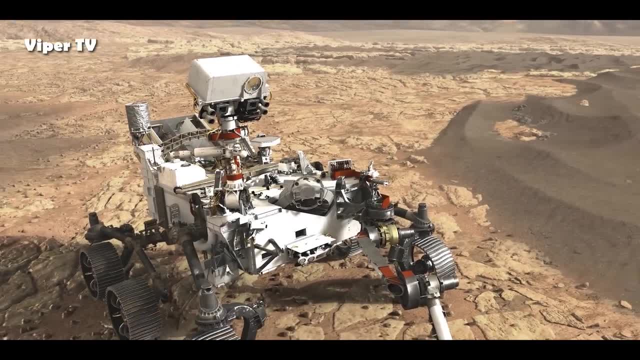 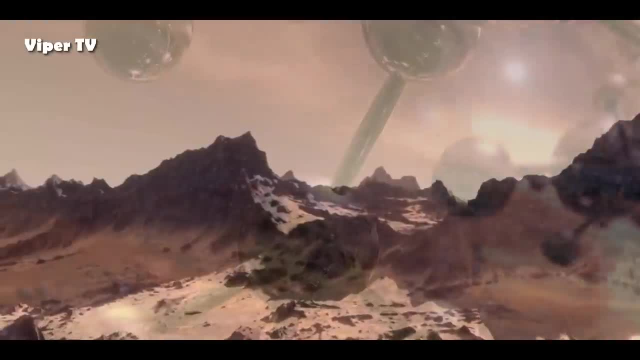 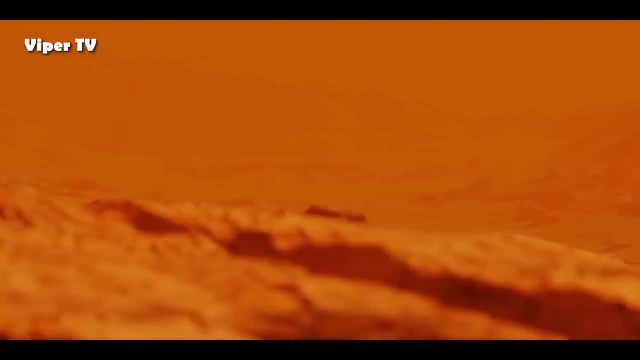 The sample of dust, dirt and finely grained soil was fed into the SAM and heated to 835 degrees Celsius. The baking process revealed the presence of significant amounts of carbon dioxide, oxygen and sulfur compounds. SAM's analysis also suggested the presence of carbonates. 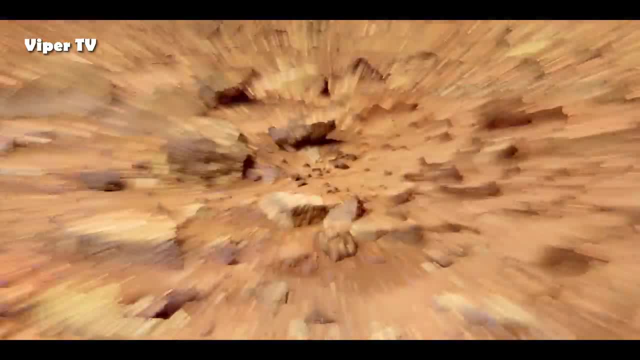 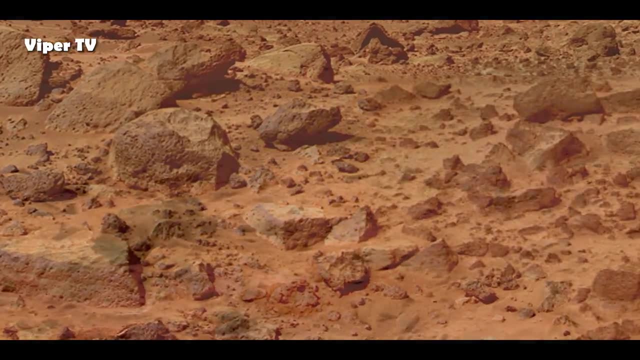 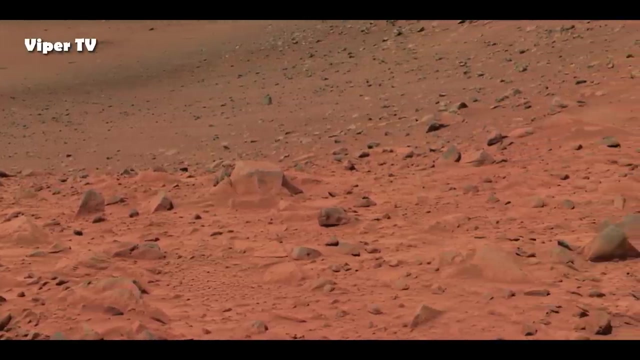 which form in the presence of water. Perhaps most surprising of all, the soil from Rock Nest didn't just provide circumstantial evidence for ancient water. Around 3% of the sample's mass was water suspended as small, ephemeral droplets of salty liquid. 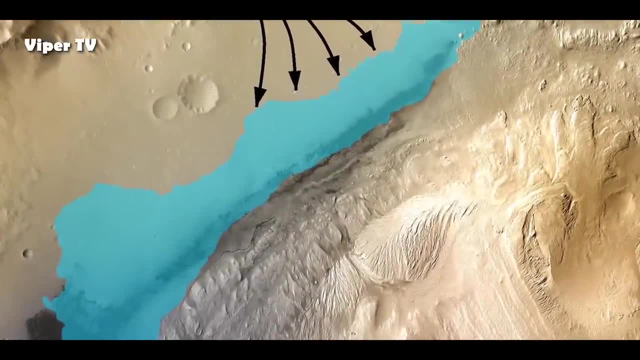 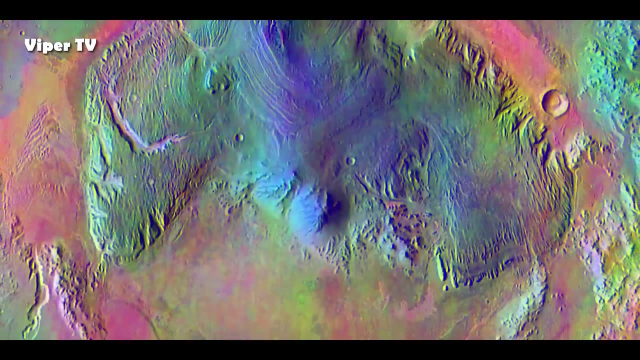 Curiosity, is sitting on the floor of a lost lake, a body of water that filled Gale at the Noachian-Hesperian boundary. The patterns of sedimentary deposits suggest the lake rose and fell in multiple cycles over tens of millions of years. 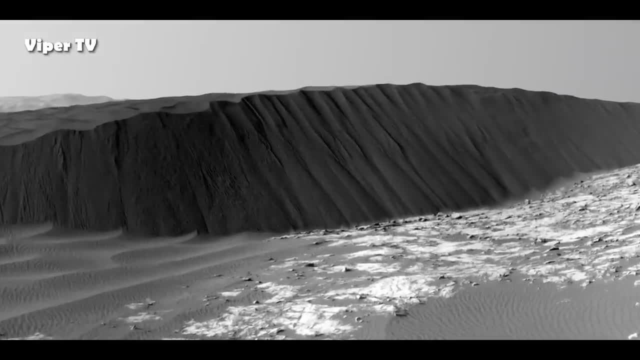 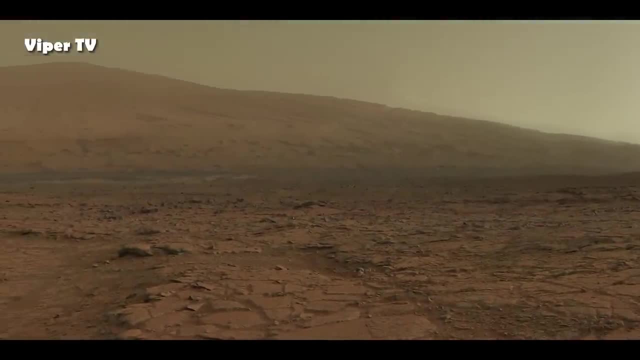 A transient landscape of ancient streams, deltas and ponds is bounded by the border of the crater When alighting on ancient riverbeds running down from the crater's rim. Curiosity has found sulfur, nitrogen, hydrogen oxygen, phosphorus and carbon. 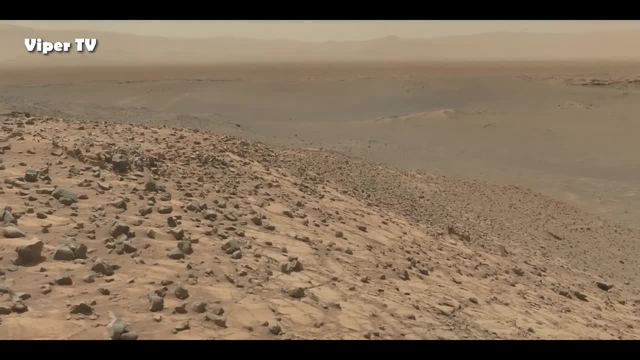 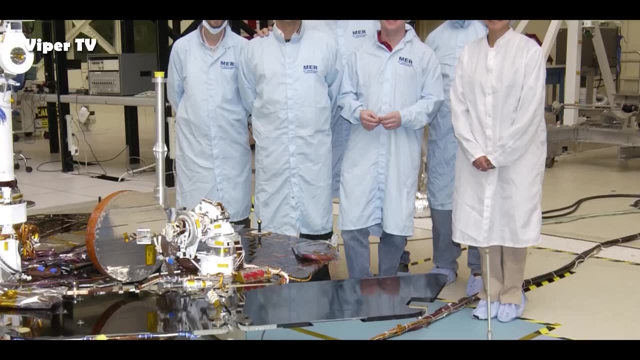 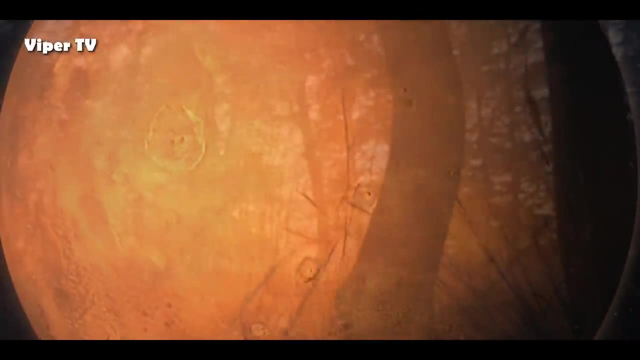 All the necessary building blocks for life. Summarising the results in August 2017, Michael Mayer, NASA's lead scientist for the Mars Exploration Programme, said A fundamental question for this mission is whether Mars could have supported a habitable environment. 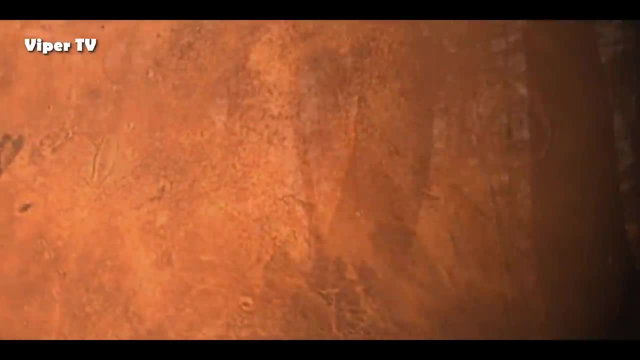 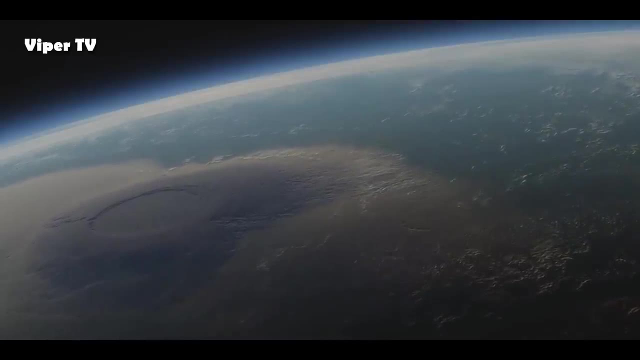 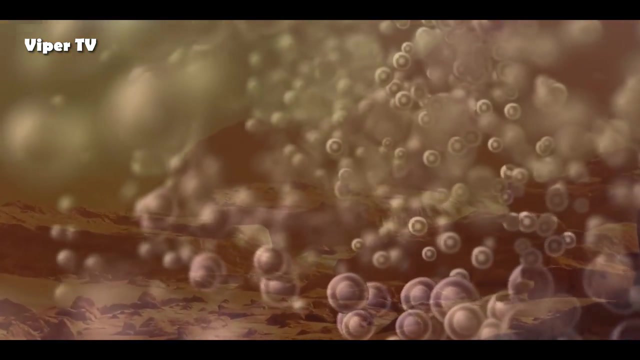 From what we know now, the answer is yes. In June 2018, two new discoveries strongly reinforced the idea that Mars was once a habitable world and maybe still is. Curiosity found complex organic molecules a few centimetres below the surface. 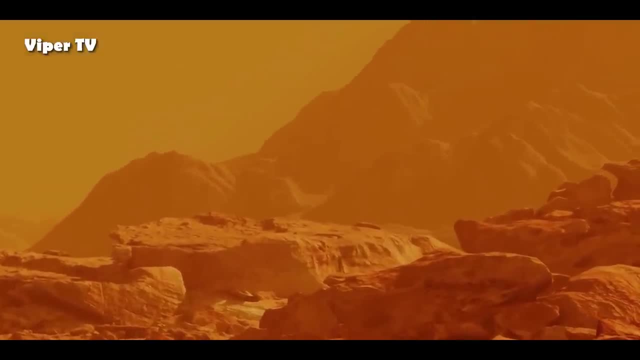 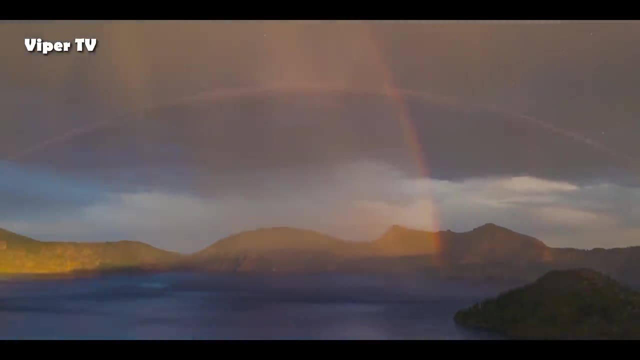 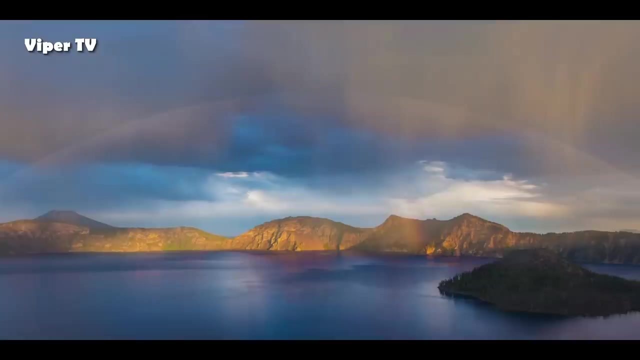 in rocks, known as mudstone, that formed from silt deposited on lake beds. This means that all the ingredients for life were present at the time when Gale Crater was filled with water. Detected molecules include benzene, toluene, propane and butane. 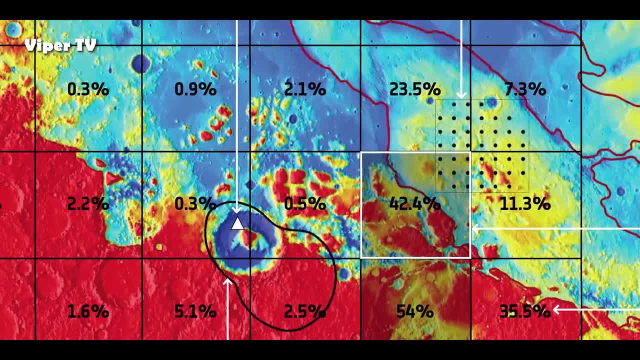 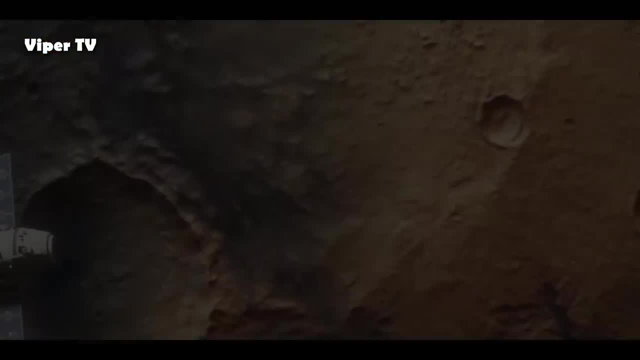 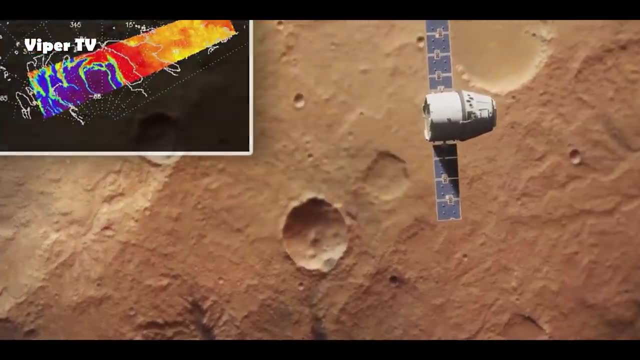 Even more tantalisingly, Curiosity also observed a strong seasonal variation in methane levels in the Martian atmosphere today, reaffirming and enhancing previous observations of methane spikes from orbit. The important additional information from Curiosity was that the methane peaked repeatedly in the warm summer months. 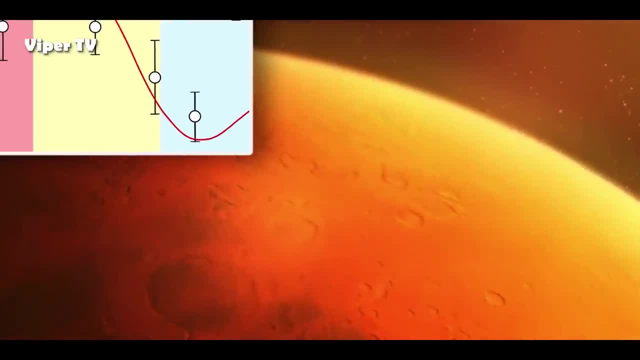 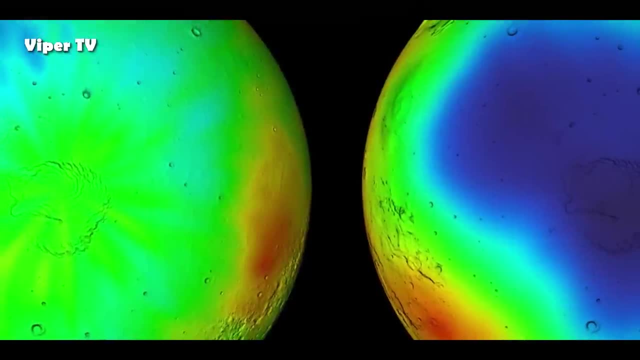 and declined in the cooler winter, which is what would be expected if the methane had a biological origin. This is not irrefutable evidence, but it is likely to be the basis of life on Mars today. by any means. It's thought that geological processes may be able to account. 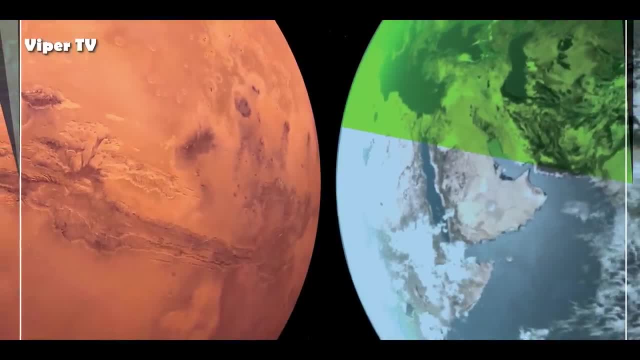 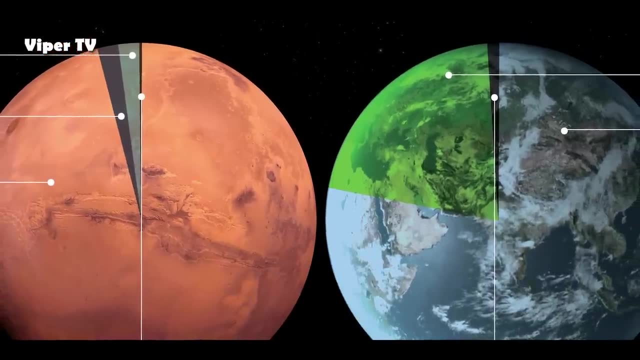 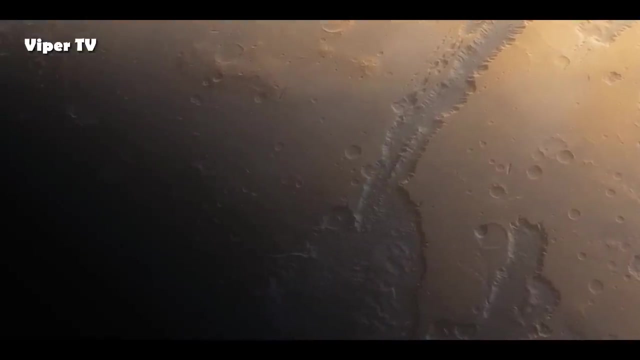 for such a seasonal variation, although, if this were Earth, a biological explanation would be favoured. The appropriately cautious Michael Mayer had this to say in June 2018.. Are there signs of life on Mars? We don't know, But these results tell us we are on the right track. 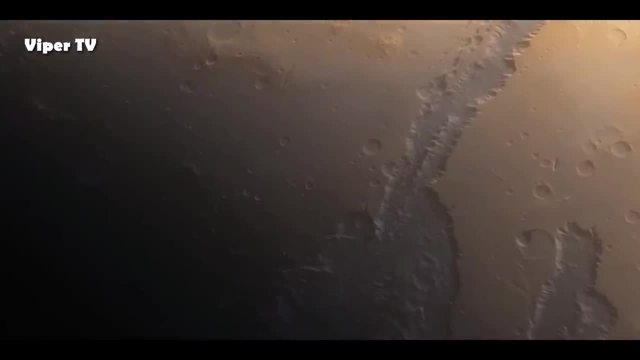 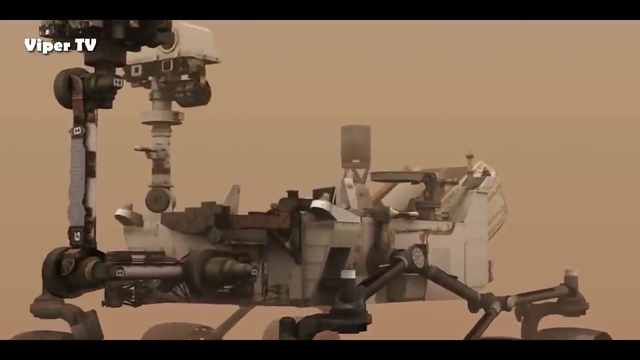 Science is a humble and cautious pursuit, and from the time of Viking we've known that Martian soil chemistry is notoriously complex and can easily catch out the unwary scientist. So we should leave it there. Curiosity continues its journey through Martian geological history, emboldened. 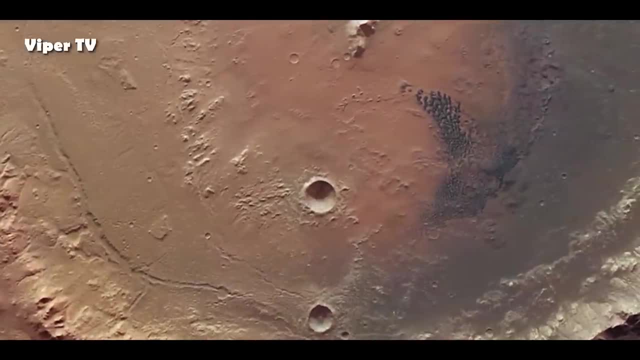 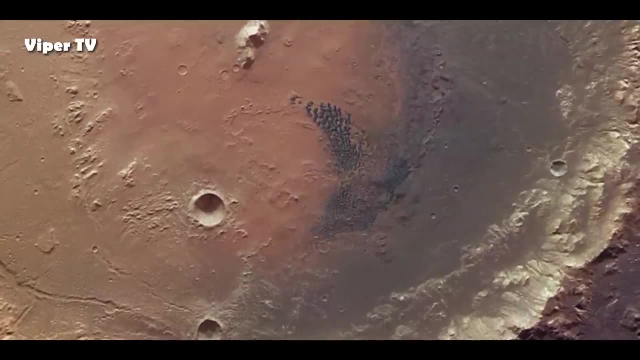 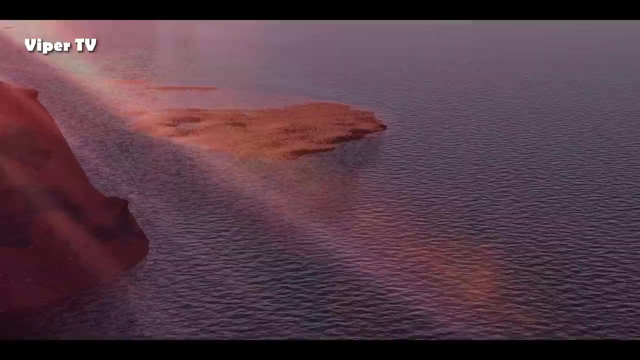 It is certainly driving across an ancient lake bed where, for a reasonably extended period, over three billion years ago- conditions were favourable and all the ingredients for life were present. While we shouldn't speculate or read too much into the results to date, we can let our imaginations wander for a moment. 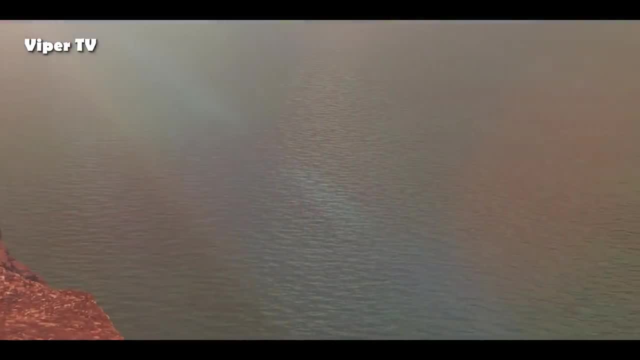 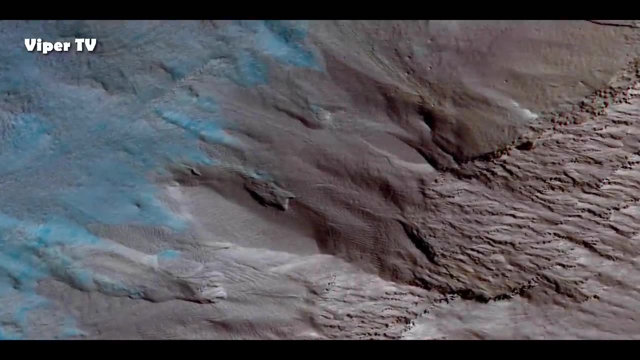 to picture what Gale Crater might have been like during the late Noachian, when life was gaining a foothold on her sister world. We stand on the shores of a lake partially filling Gale, fed by runoff from snowmelt on the far northern rim. 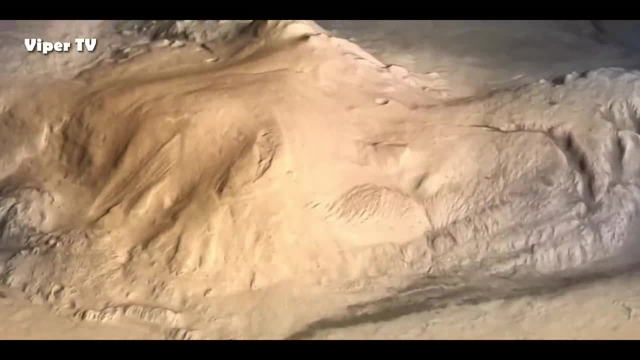 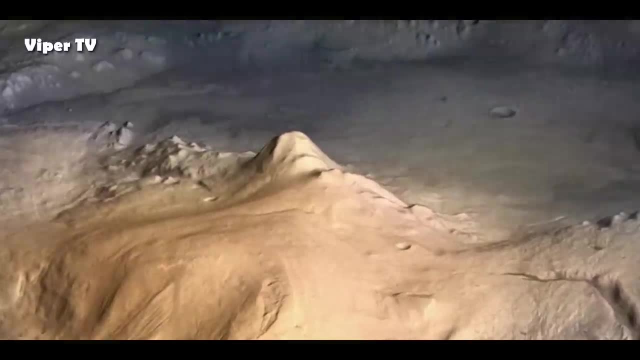 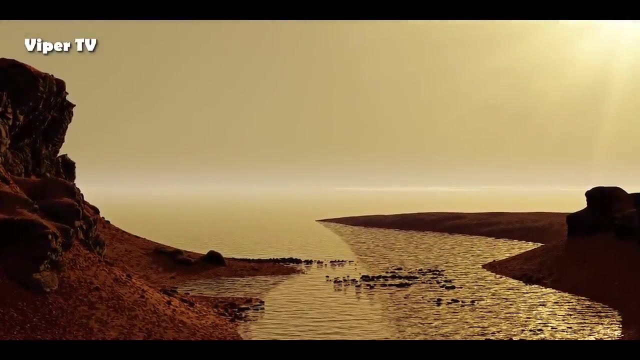 Where Mount Sharp now stands, a small island breaks the surface: blue, Not the mountain of today, but a small central peak left over from the impact, A place of grand beauty where each Martian evening the pale sun sets in the west, beyond the island. 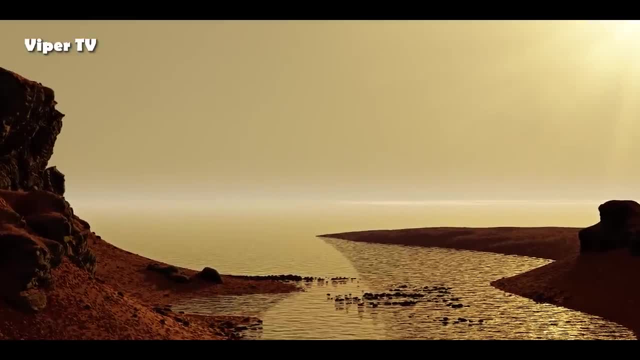 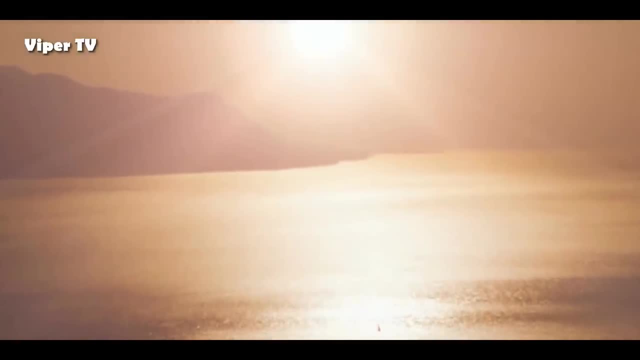 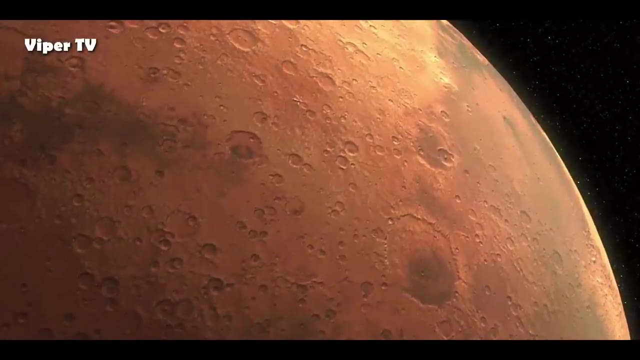 rays glinting dimly off the still waters, interrupted by the shadow of the peak out to the crater's edge, A sundial marking the passing of time on a lake populated by microbial Martians. Mars is a mirror for our dreams and nightmares. 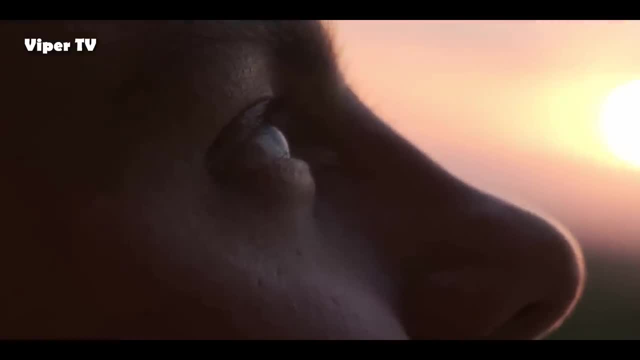 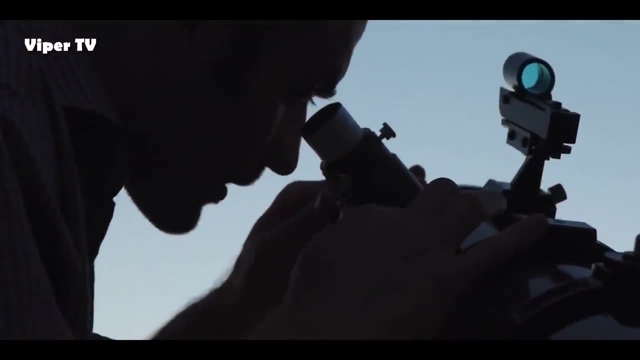 To the naked eye, the planet exhibits a reddish hue, blood-red in the imagination. god of war, star of judgment Through a small telescope. it is the most Earth-like of planets, with cinnabar deserts and white polar ice caps. 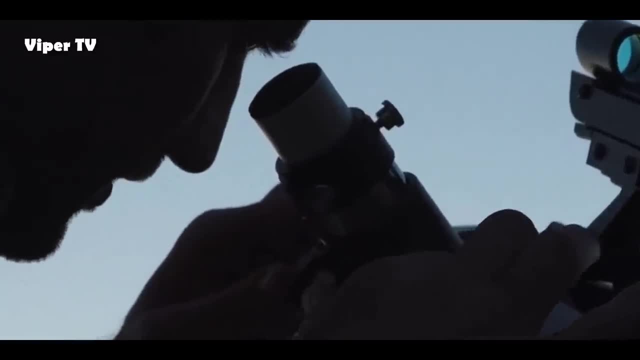 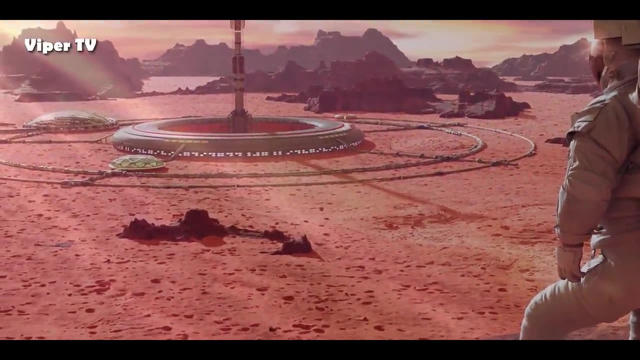 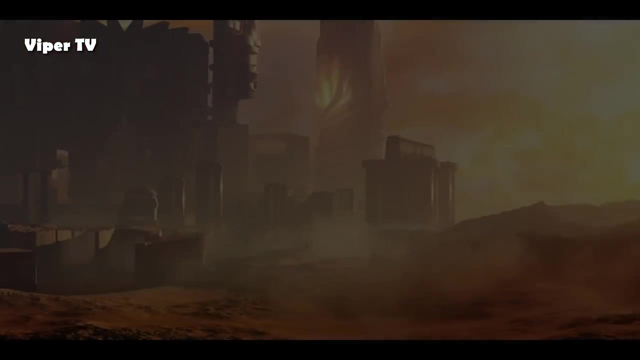 A world we could imagine visiting, perhaps even settling in. 19th-century astronomers convinced themselves. they saw plains and mountain ranges, and canals delivering meltwater from high latitudes to arid equatorial cities. Some thought the Martians a peaceful civilisation. 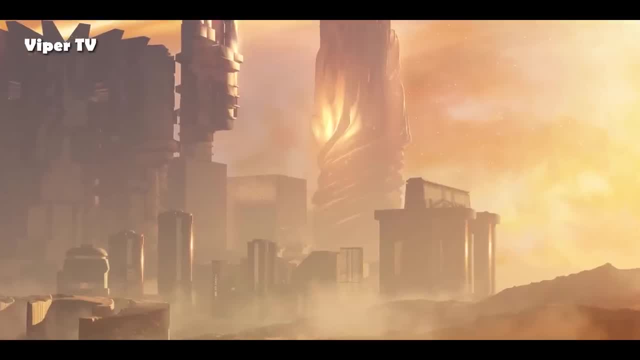 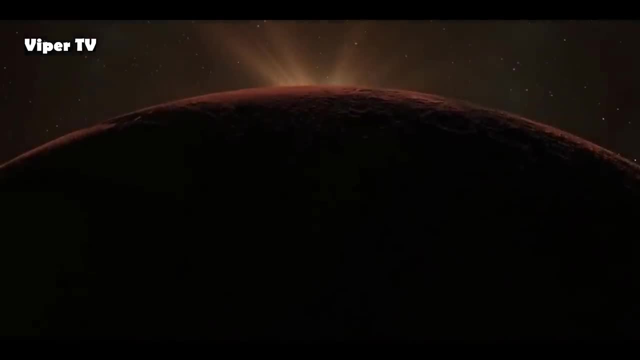 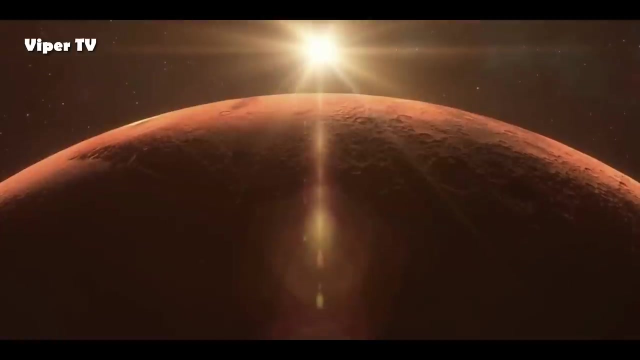 far in advance of our own. Others saw threat Across the gulf of space. minds that are to our minds as ours are to those of the beasts that perish. intellects, vast and cool and unsympathetic, regarded this Earth with envious eyes. 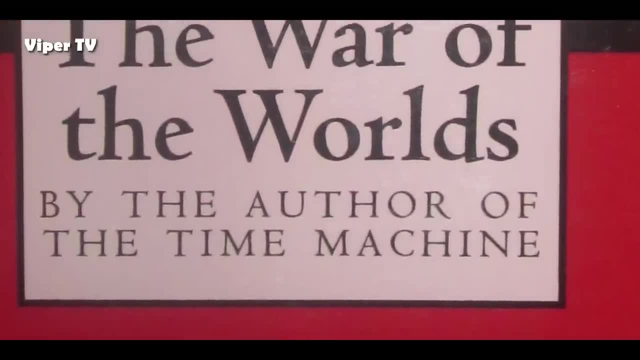 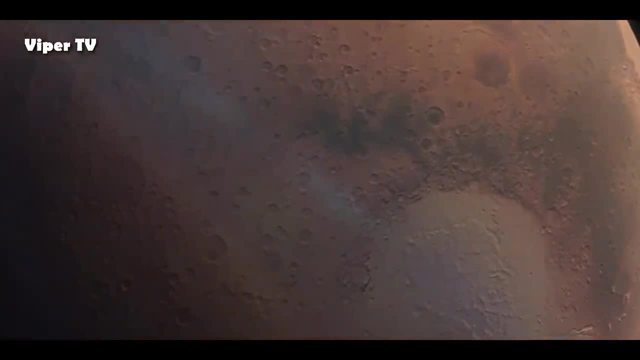 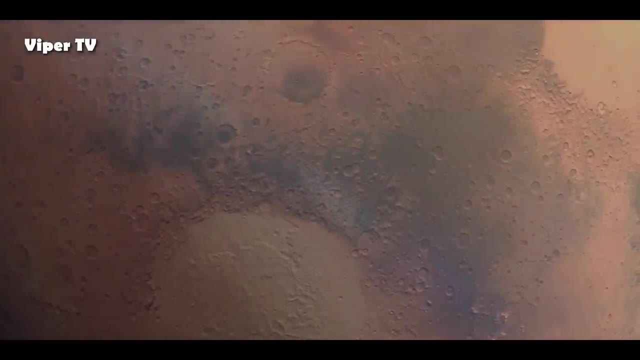 wrote HG Wells in his classic science fiction novel The War Of The Worlds in 1897.. The nature of Mars remained a mystery until well into the 20th century because the planet is small and far away and therefore difficult to view with ground-based telescopes. 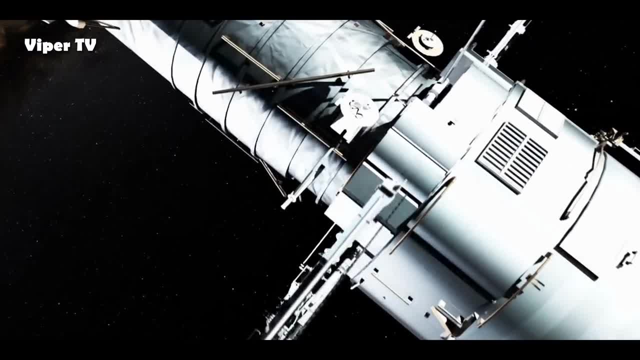 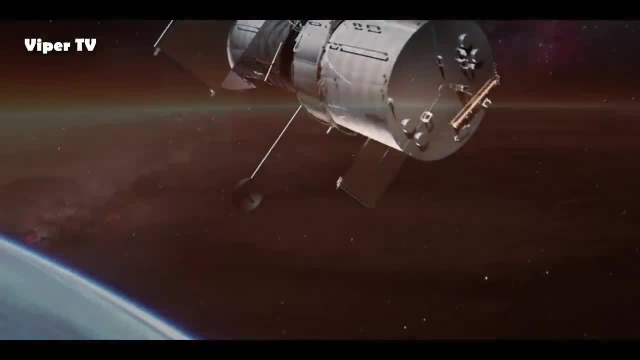 Even the Hubble Space Telescope, high above the distorting effects of Earth's atmosphere, produces images which would not, at first sight, have prevented Wells from publishing, With a little imagination, the ice caps, high clouds and dark regions circling the deserts. 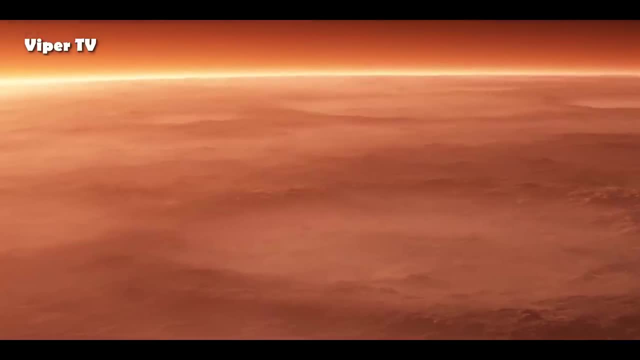 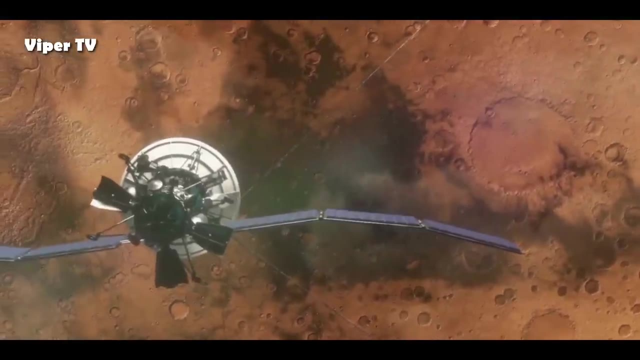 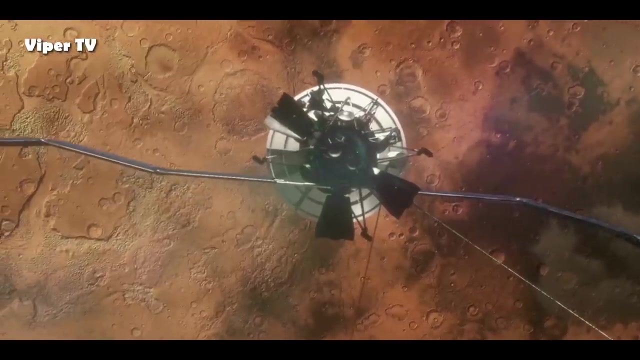 could be mistaken for evidence of a water cycle feeding the seasonal advance and retreat of vegetation. Photographs from the first flyby of Mars by NASA's Mariner 4 spacecraft on 15 July 1965 abruptly laid to rest the romantic notion of Mars as Earth's habitable twin or potential foe. 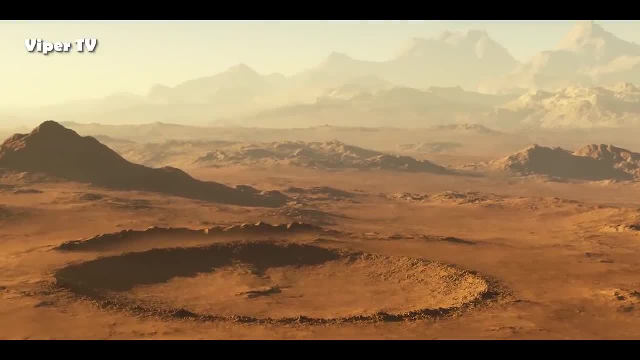 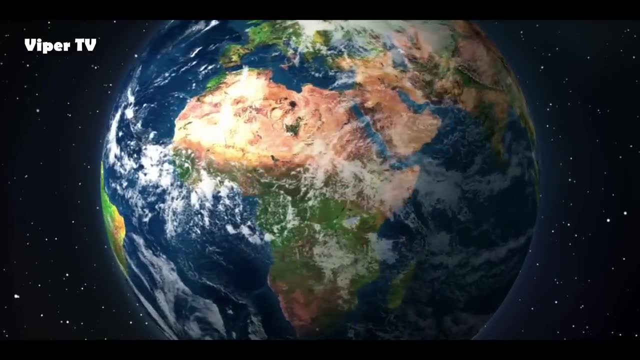 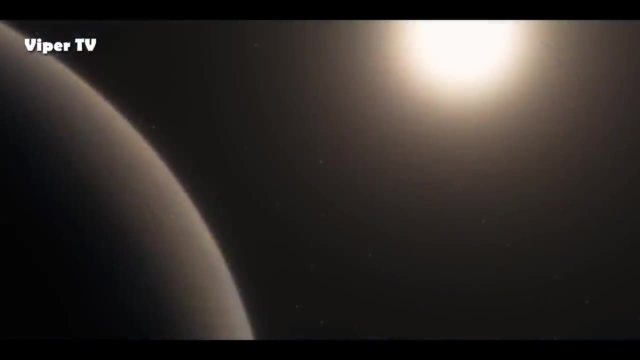 These images revealed an arid surface reminiscent not of our blue planet, but of our desiccated moon. Overnight, we discovered for certain that Earth is the only planet in the solar system capable of supporting complex life And contemporary accounts of the impact of the Mariner 4 flyby. 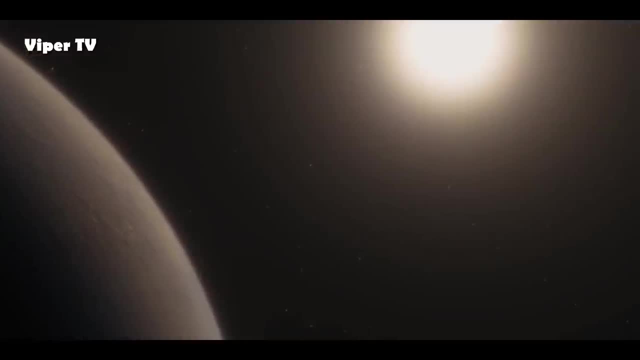 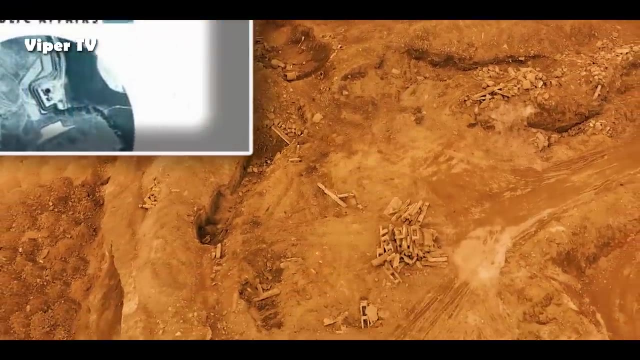 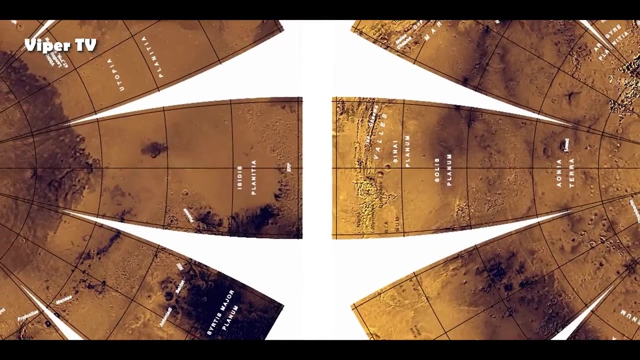 suggest that this was a powerful realisation. In November 1965, the Bulletin of the Atomic Scientists carried an article entitled The Message from Mariner 4, and the message was bleak. The shock of Mariner's photographic and radiometric reports is caused not only by their denial of the terrestrial image of Mars. 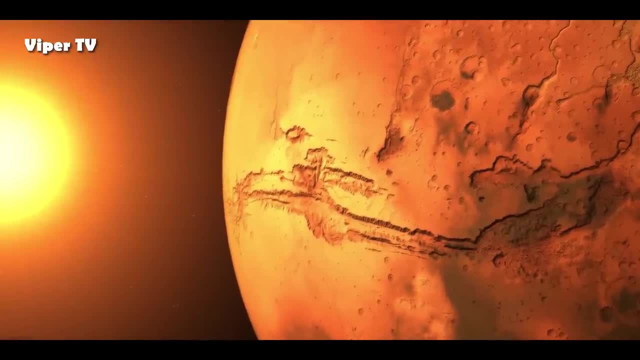 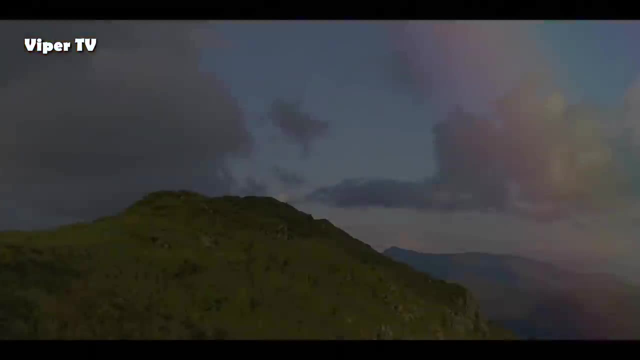 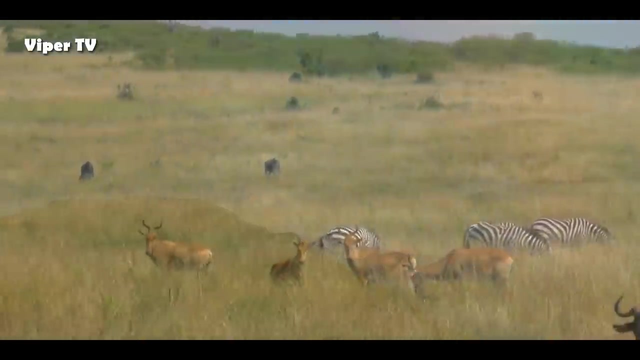 but by the revelation that there is no second chance, at least not in the solar system. President Lyndon B Johnson was reported as commenting: It may be, it may just be, that life as we know it, with its humanity, is more unique than many have thought. 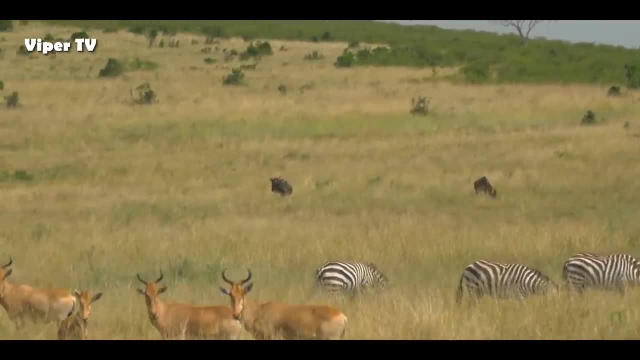 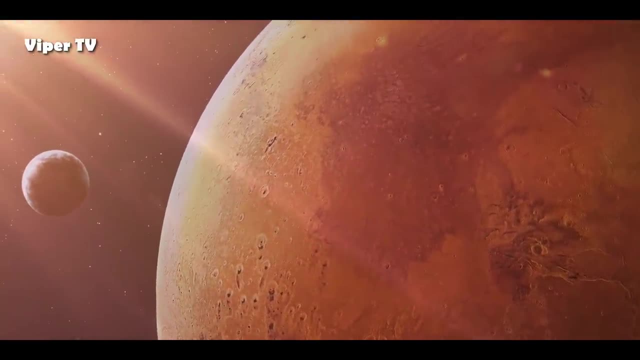 The hesitation in the first few words is revealing. Here is Mars as a symbol of our cosmic isolation. It is as though deep, or perhaps not so deep, in the subconscious, The 1960s power brokers, all the way up to the president. 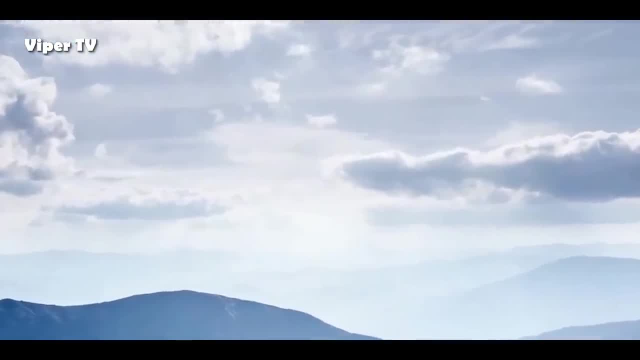 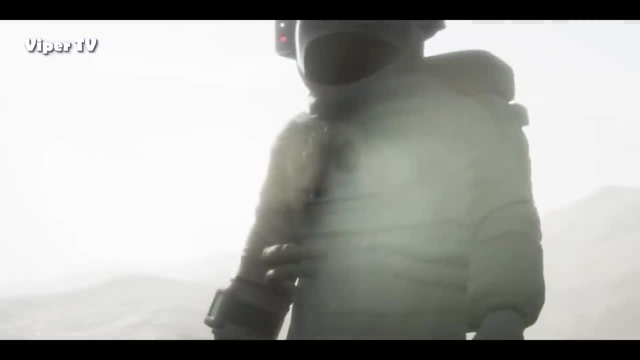 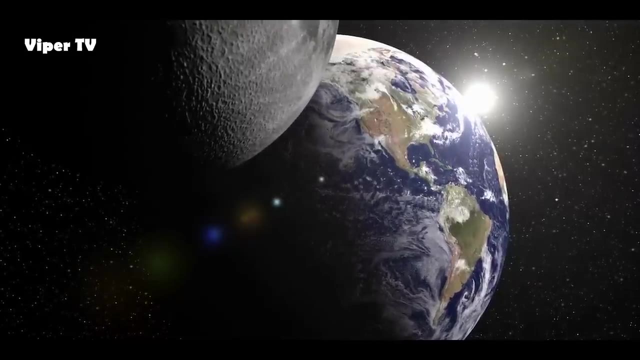 suddenly understood that the Earth is far more fragile and precious than a dispassionate analysis of their Cold War brinkmanship might suggest. Or perhaps the perspective delivered by exploration is always shocking. Apollo 8's Earthrise- the photograph that delivered such a positive end. 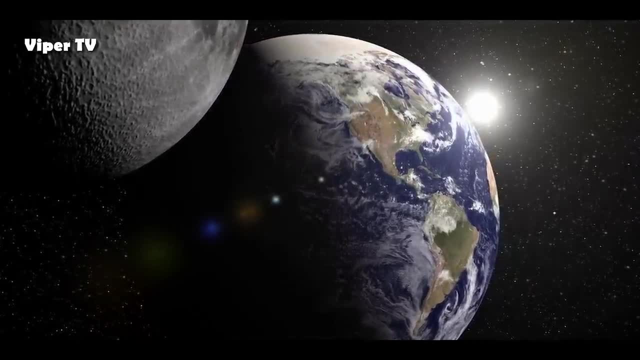 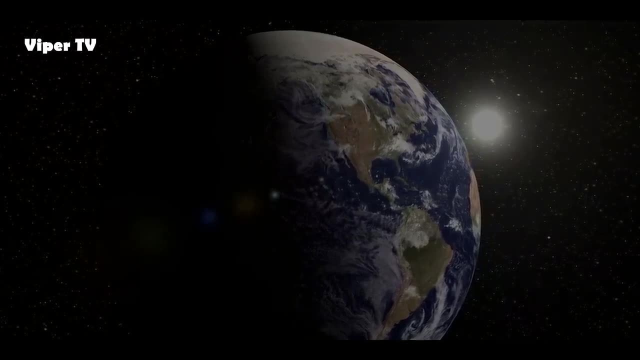 to a troubled 1968 by setting the blue Earth against the grey Moon was three years away, But red Mars provided a foretaste. In response, Carl Sagan co-authored a paper suggesting, somewhat playfully, that all was not lost. 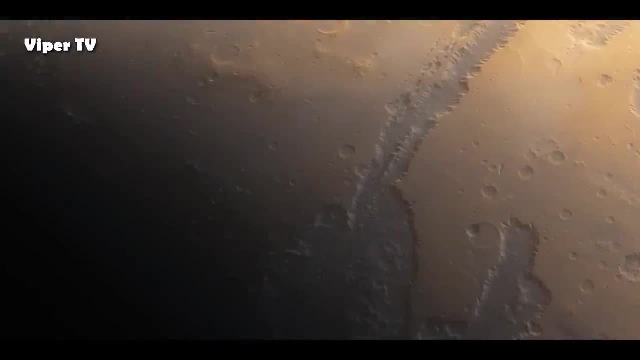 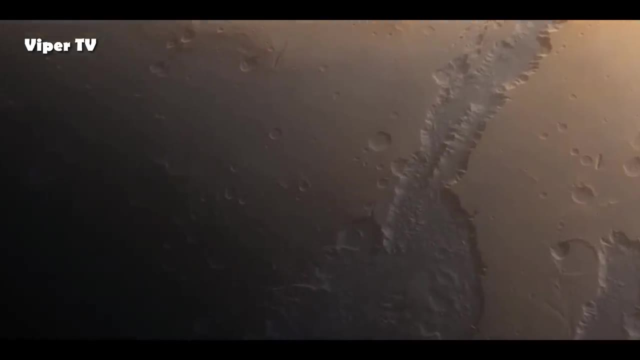 Mariner 4 took only 22 photographs with a resolution of over a kilometre in a strip crossing the region in which the astronomer Percival Lowell had sketched canals from his observatory in Flagstaff, Arizona, at the turn of the 20th century. 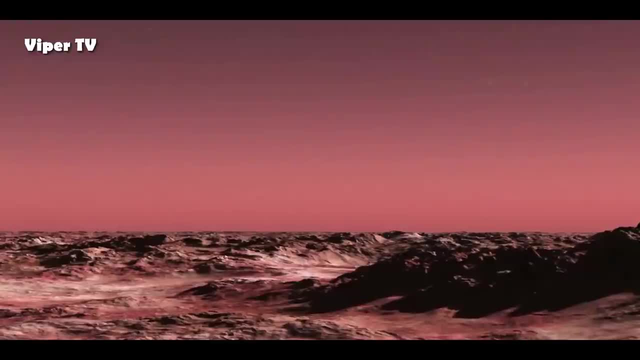 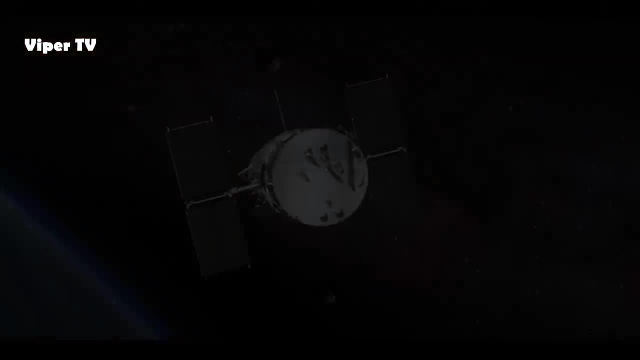 From the warmth of the Arizona desert. Lowell wrote that Mars was chilly, but no more so than the south of England, which certainly supported a civilisation of sorts. Using several thousand photographs- photographs of a similar resolution- taken by meteorological satellites in Earth's orbit. 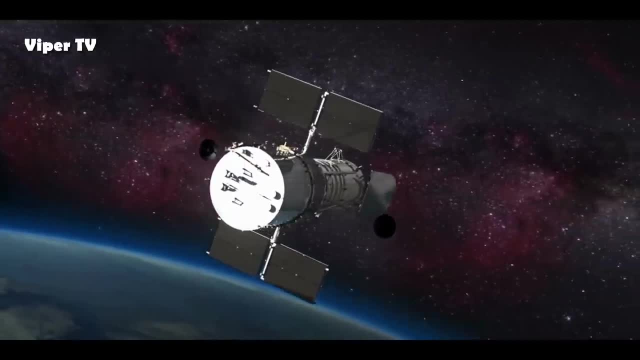 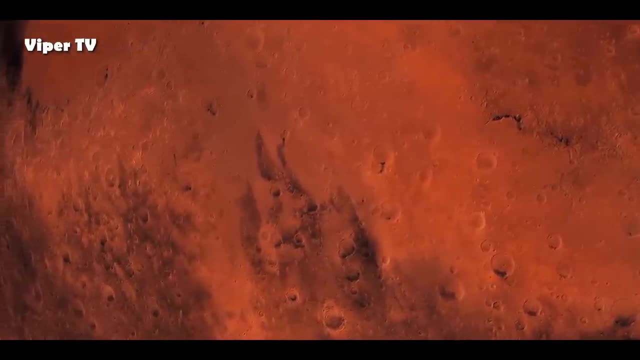 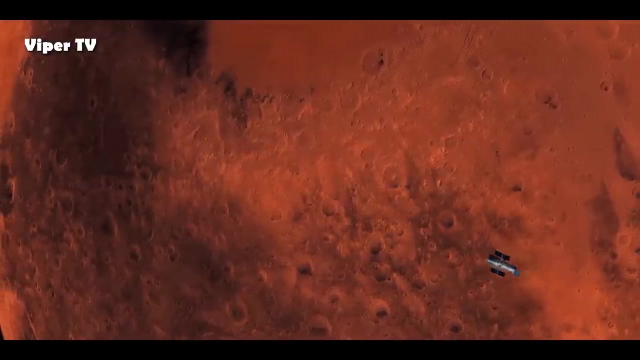 Sagan and his co-authors found only a single feature that unambiguously indicated the presence of a civilisation: Interstate Highway 40 in Tennessee. They concluded that Mariner 4 would not have detected human civilisation had it flown by Earth. 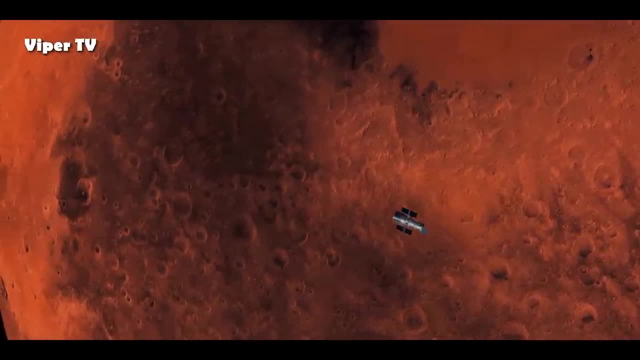 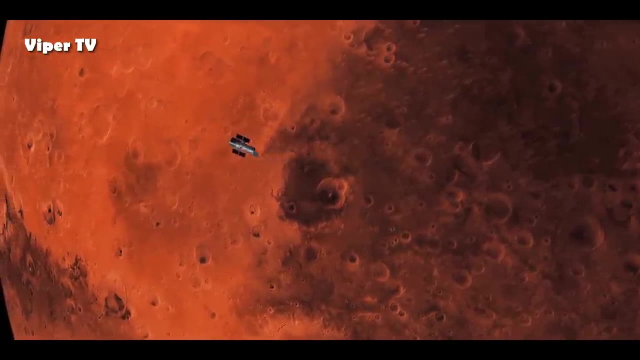 We do not expect intelligent life on Mars. but if there were intelligent life on Mars comparable to that of Earth, a photographic system considerably more sophisticated than Mariner 4 would be required to detect it. The non-existence of an extant Martian civilisation. 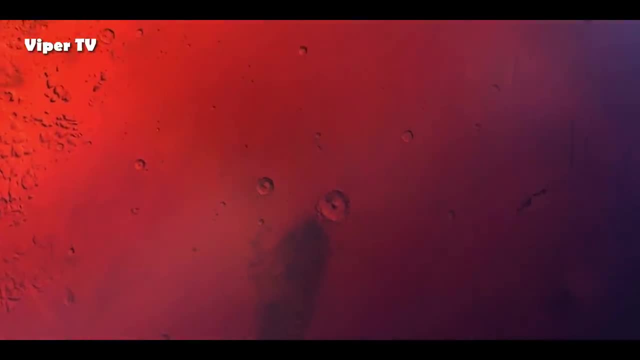 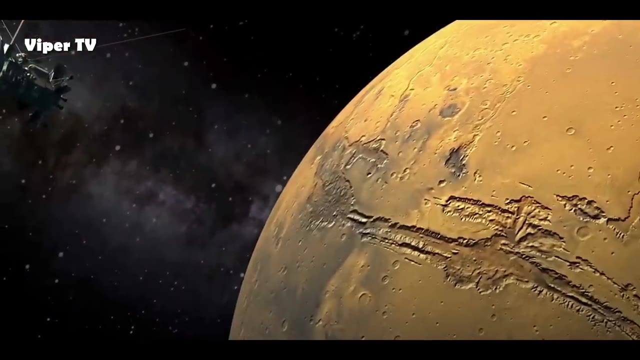 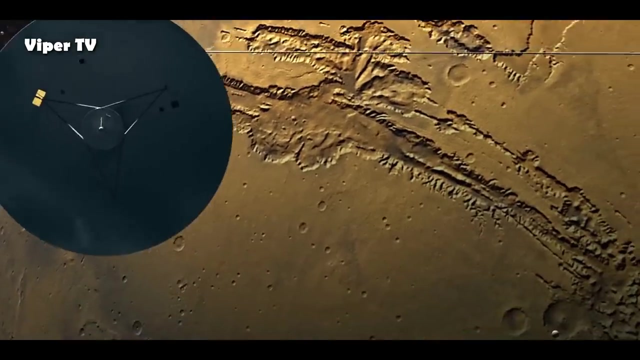 was confirmed by the Mariner 9 mission in November 1971, the first spacecraft to orbit another planet. Mariner 9 achieved a photographic resolution of 100 metres per pixel and no sign of intelligent life, past or present, was detected. 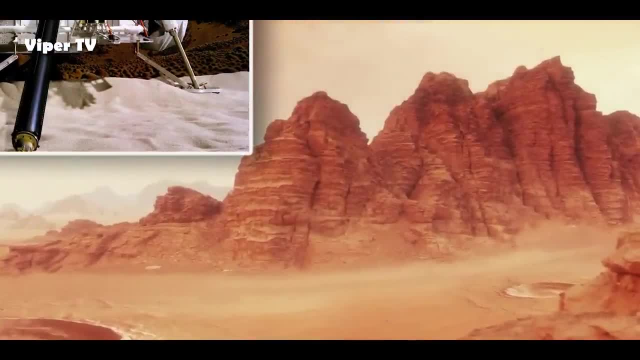 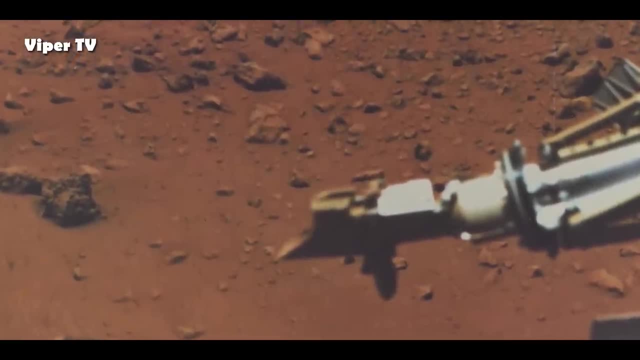 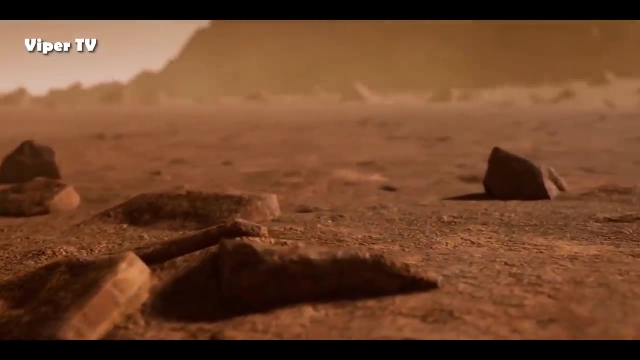 The twin Viking landers in 1976, failed to detect even microbial life, although the combined results of the suite of microbiology experiments carried by the spacecraft are not considered to be unequivocal, because Martian soil chemistry is to coin a phrase from the official NASA report. 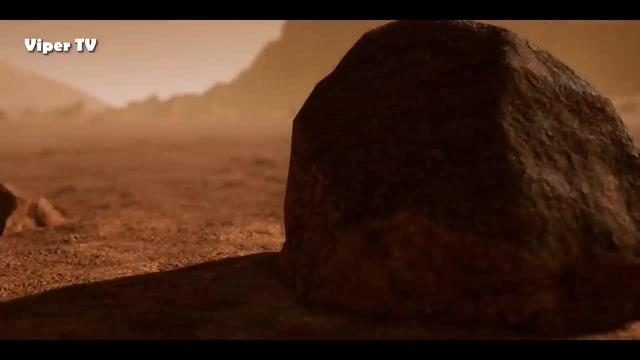 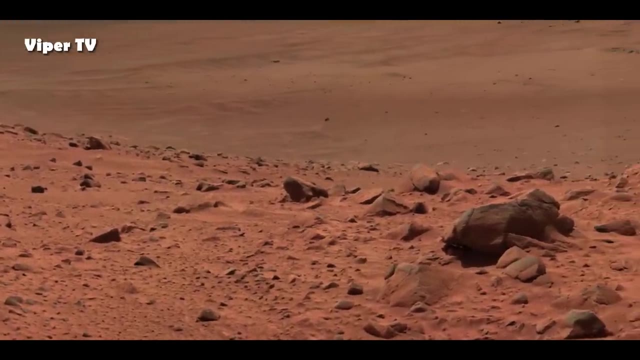 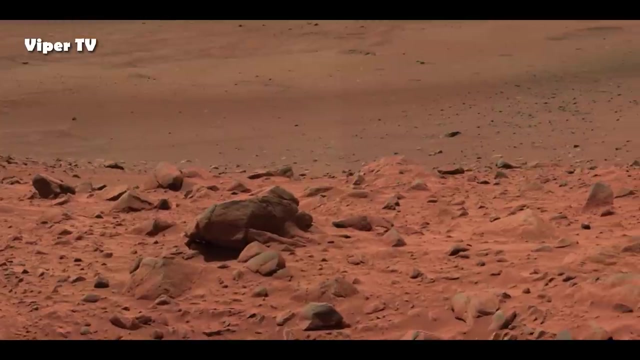 enigmatic and could conceivably have masked any biological activity. In hindsight, the fact that Mars is not teeming with life today is not so surprising. Mars orbits 50 million miles further from the Sun than Earth and receives less than half the solar energy. 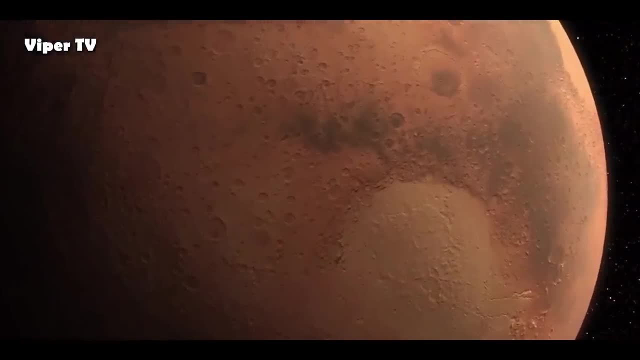 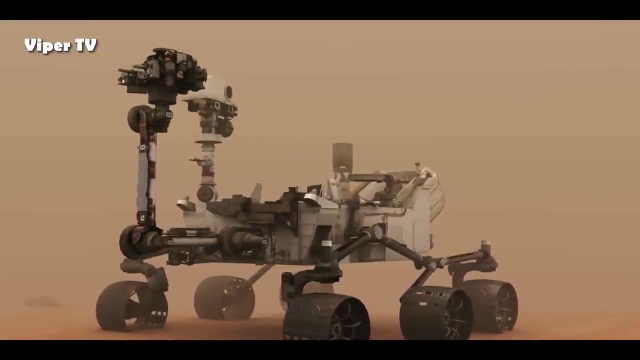 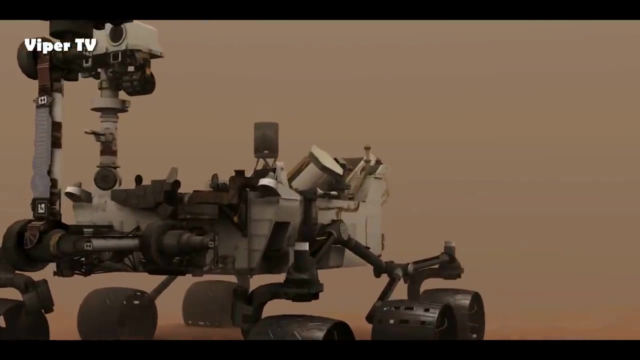 It is a small world with a tenuous atmosphere that provides little insulation or greenhouse warming. NASA's Curiosity rover in the Gale crater has measured midday temperatures above 20 degrees Celsius, but in the early hours of the morning it has experienced minus 120. 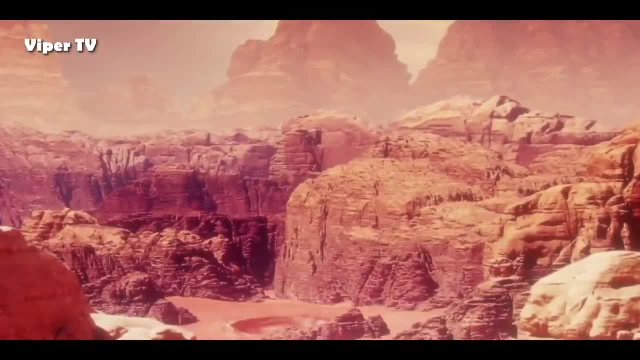 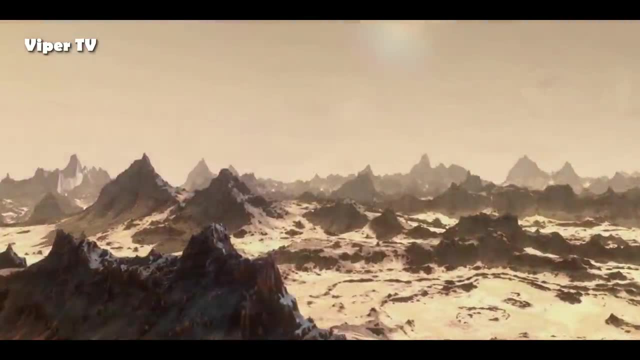 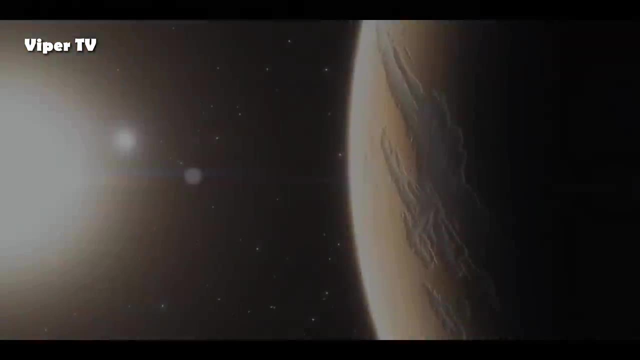 As Alfred Russell Wallace wrote in 1907, any attempt to transport water across the Martian surface today would be the work of madmen rather than of intelligent beings. There are no canals, no cities and no envious eyes. The planet is a frozen, hyper-arid desert. 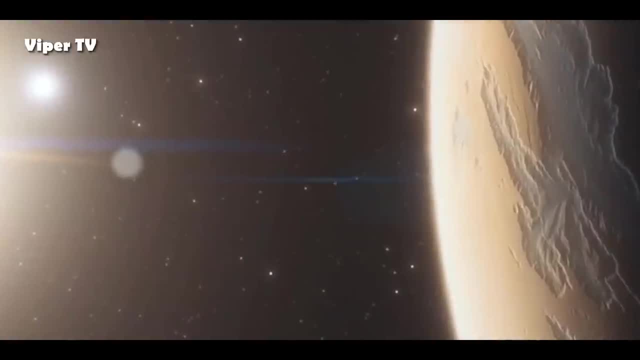 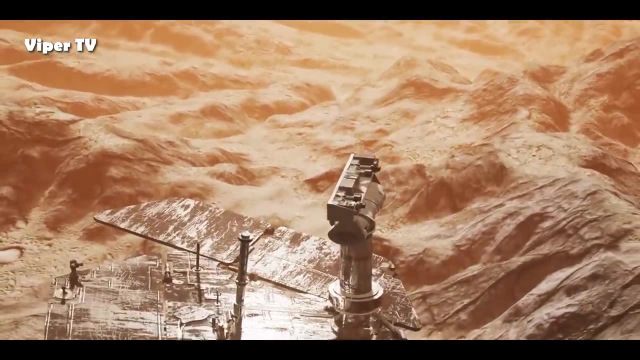 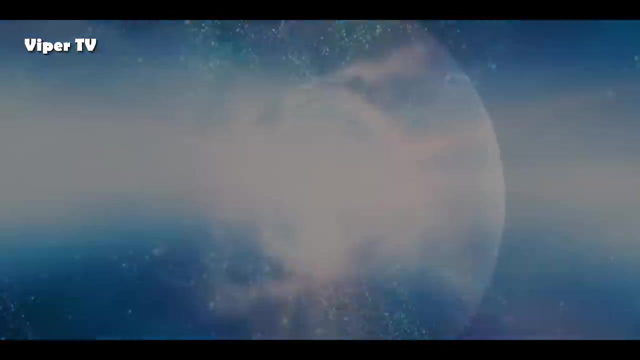 too far from the Sun to support complex life. Yet it hasn't always been this way. Observations from our fleet of orbiting spacecraft and landers have revealed a complex and varied past. Once upon a time, the red planet was glistening blue. 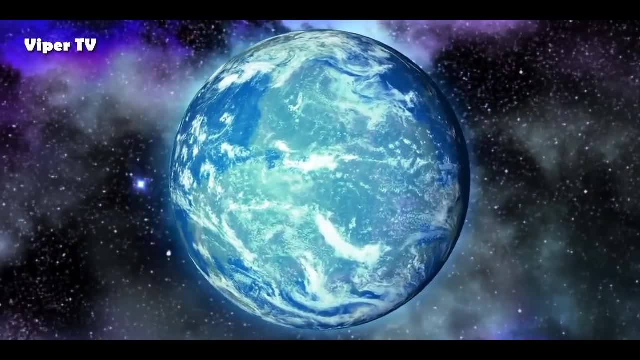 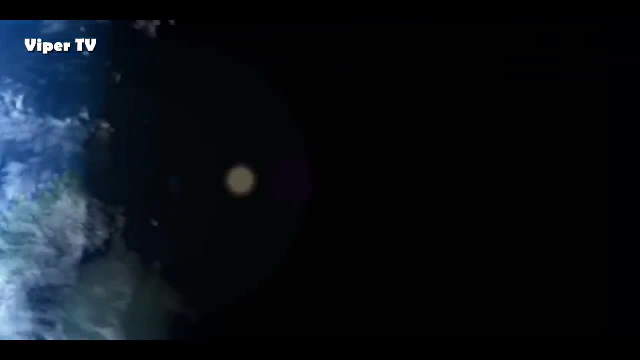 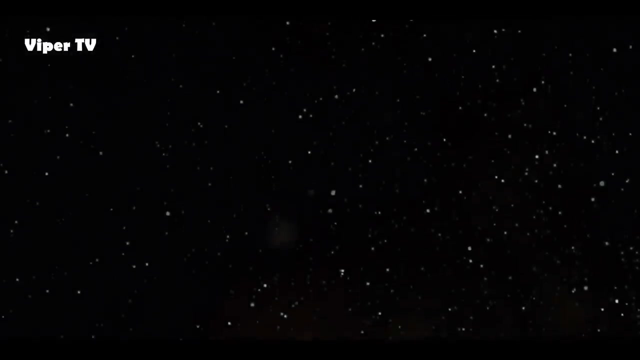 Streams ran down hillsides and rivers wound their way through valleys carved by a water cycle from land to sky and down again from mountains and highlands to the sea. This presents a great challenge for planetary scientists. Put simply, nobody would have been surprised. 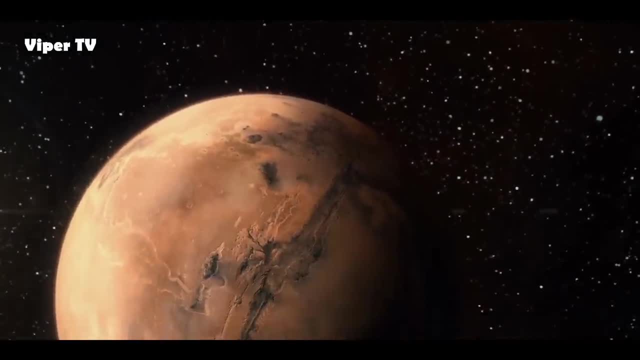 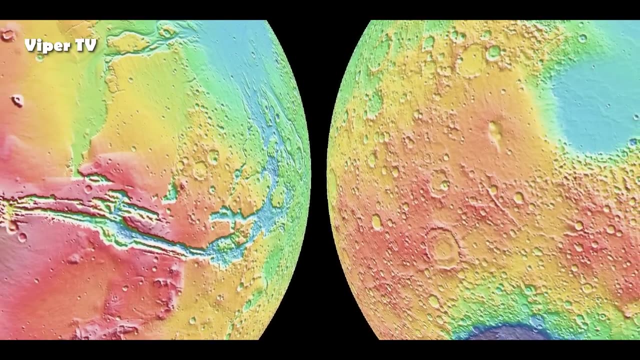 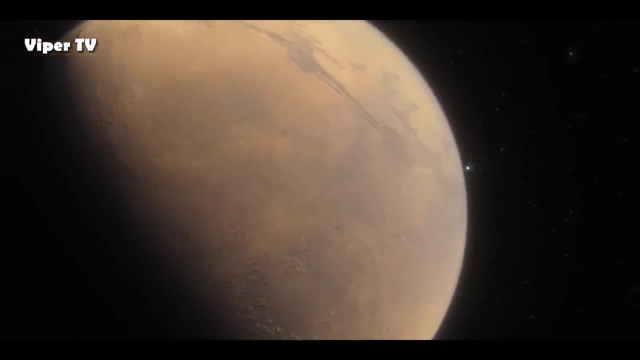 if Mars had always been an inert rock, because it is a small planet Far from its star. But the geological evidence is unequivocal. The surface tells a different story. Mars, then, remains an enigma. As a wandering red star, it stirred the imagination of the ancients. 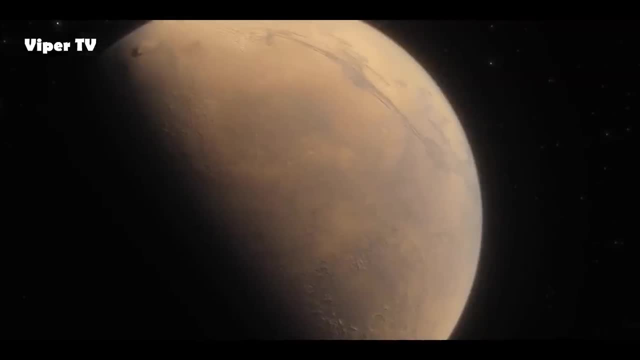 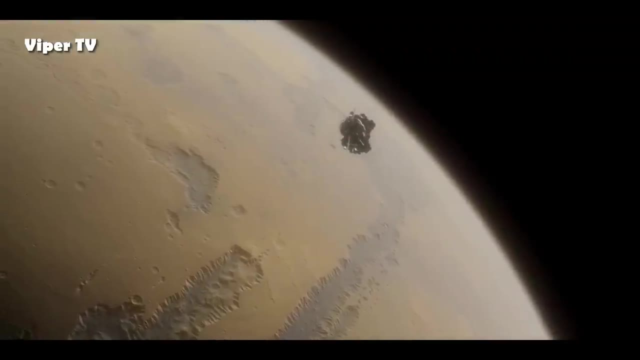 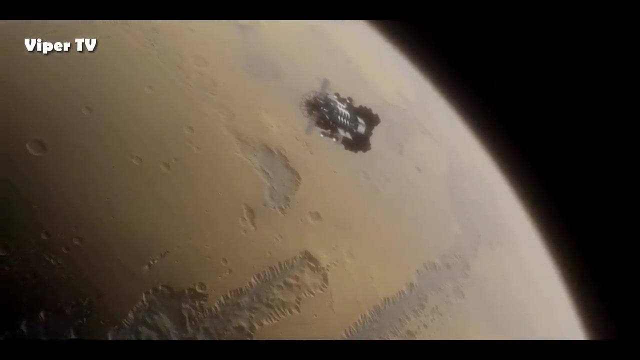 As a telescopic image, too small and shifting for visual or intellectual clarity. it became our twin When spacecraft flew by. it shocked us into considering our cosmic isolation. The red planet was relegated in our collective consciousness to the status of just one more rock. 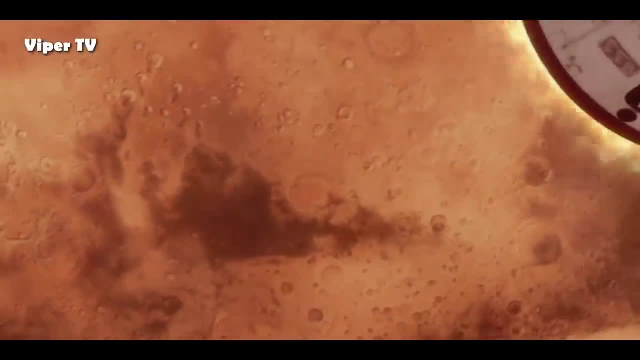 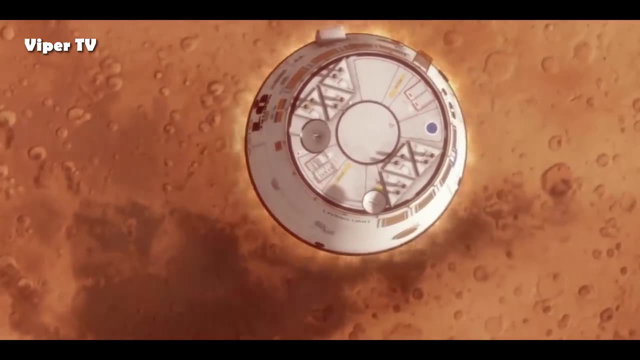 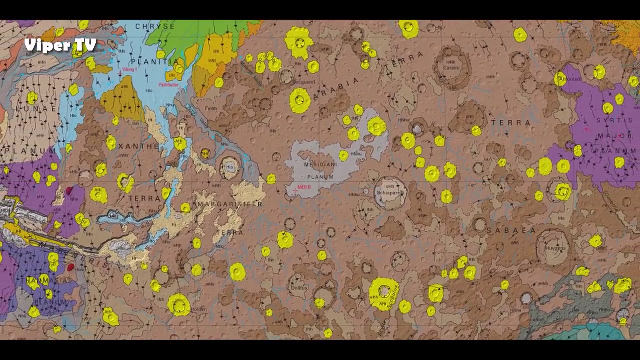 glistening in the night. Then we landed and discovered a world that was once habitable and could be again. A map of Mars can be read like a history book, Unlike Earth, where constant weathering, tectonic activity and volcanism have erased the deep geological past. 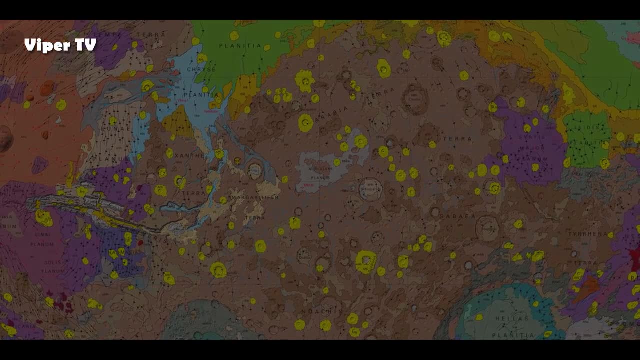 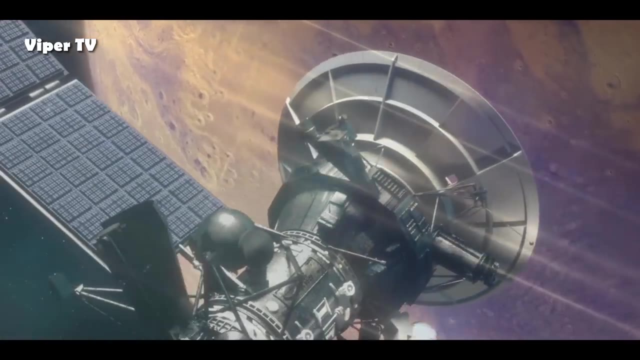 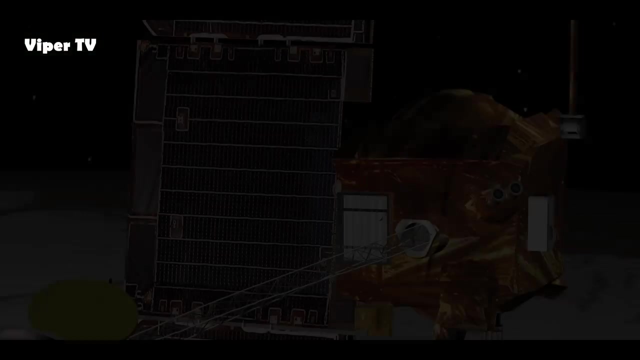 Mars has been relatively quiescent for most of its life. The scars of collisions from the first turbulent billion years after the formation of the solar system can still be seen from orbit. Ancient cataclysms documented below a thin film of dust. NASA's Mars Global Surveyor spacecraft. spent four and a half years mapping Mars in the late 1990s and provided detailed maps with colours corresponding to differences in altitude. Just as on Earth, there is significant variation, but the geological features on our smaller sister world are much bigger and bolder. 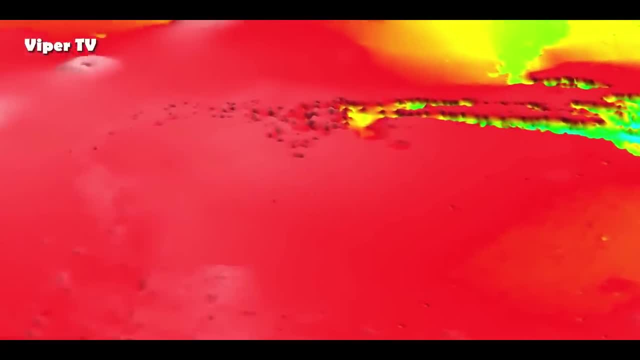 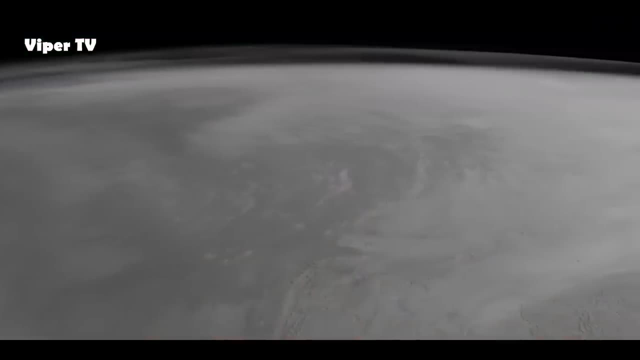 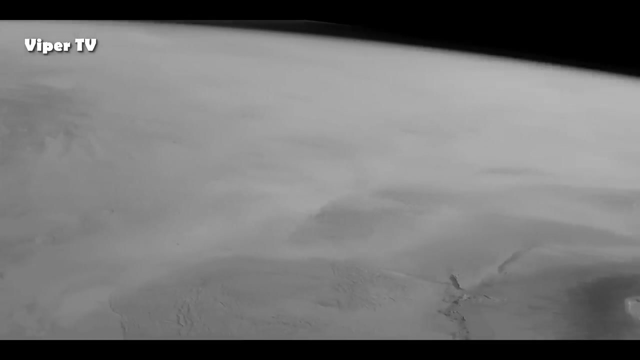 The highest elevations on Mars are found on the Tharsis Rise, a great volcanic plateau and home to the largest volcano in the solar system, Olympus Mons. At over twice the height of Everest, Olympus Mons towered over the Earth and it towers 25km above the lowlands. 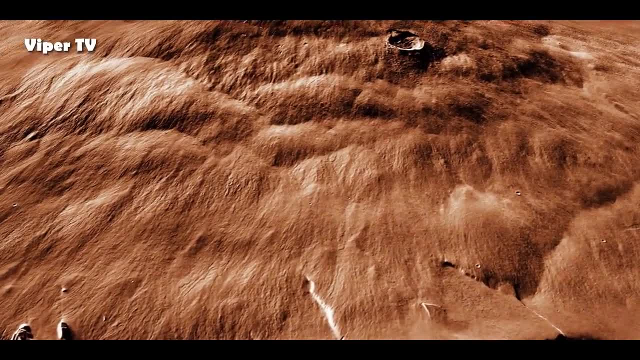 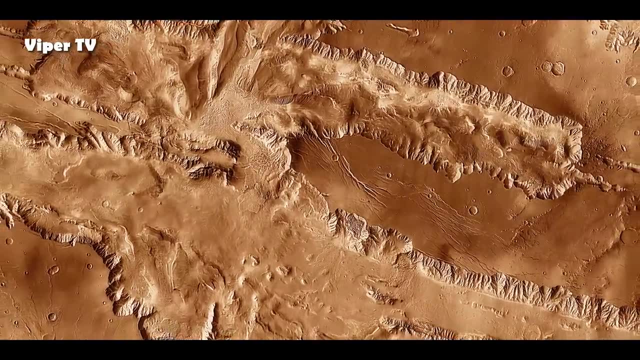 of Amazonis Planitia to the west, and its base would fit inside France, just about Cutting a deep scar across Tharsis. to the south-east of Olympus Mons is Valles Marineris, named after the Mariner 9 spacecraft that discovered it. 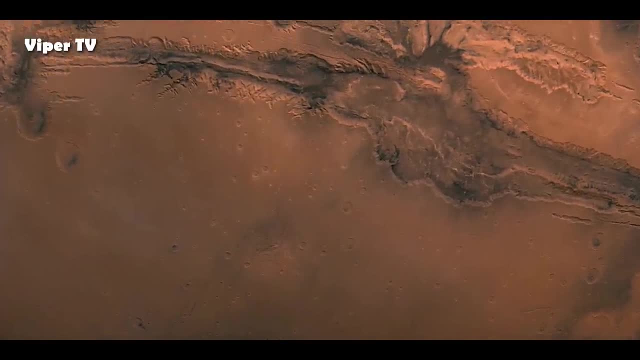 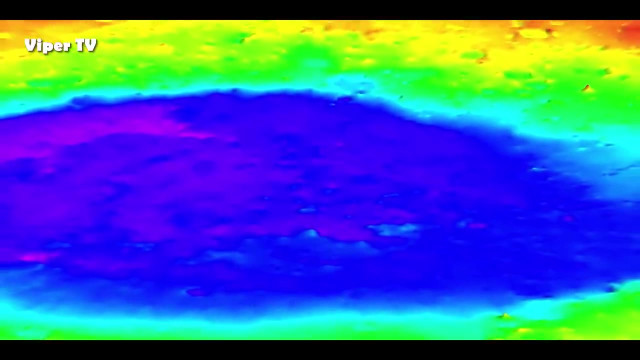 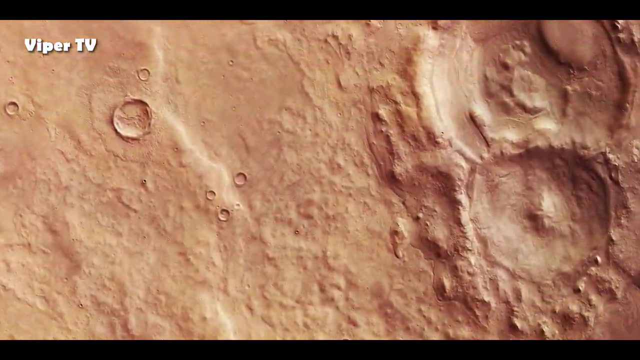 a canyon that dwarfs anything on Earth. The Grand Canyon would fit into one of its side channels. The lowest points on Mars are found in the Hellas Impact Basin, the largest clearly visible impact crater in the solar system, From the highest points on the crater rim to the floor. 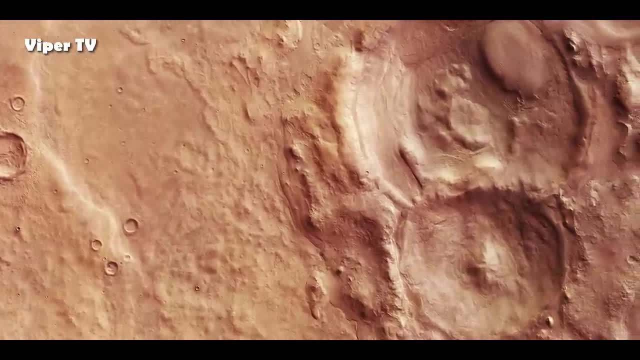 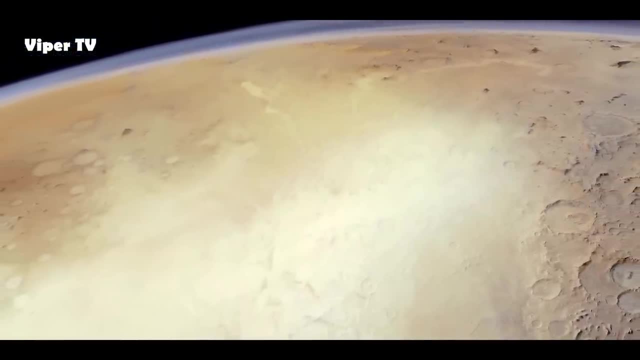 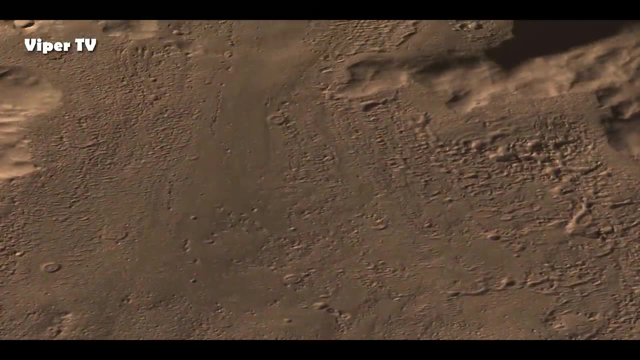 Hellas is over 9km deep. It could contain Mount Everest. The atmospheric pressure at the floor is twice that at the rim, high enough for liquid water to exist on the surface in a narrow range of temperatures. These are extreme altitude differences for a small world. Over 30km from the summit of Olympus Mons to the floor of Hellas, On much larger Earth. for comparison, there is only 20km difference between the summit of Everest and the Challenger, Deep in the depths of the Mariana Trench. 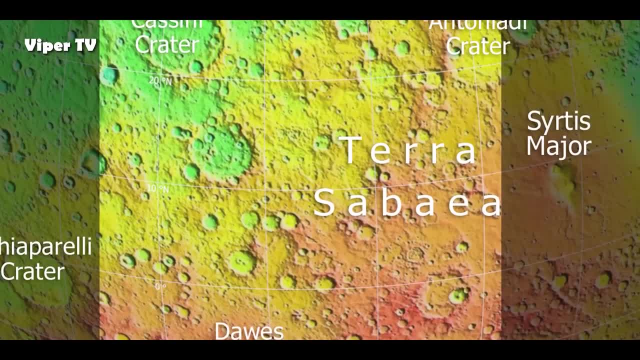 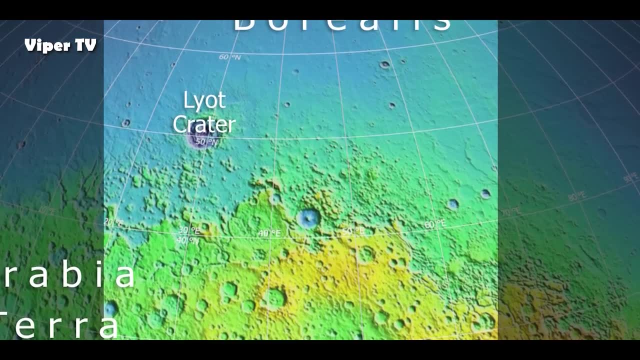 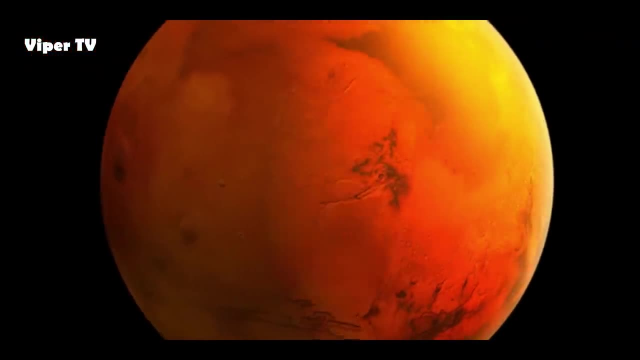 The most striking and ancient elevation difference on Mars is that between the northern and southern hemispheres of the planet, known as the Global Dichotomy. Mars is an asymmetric world. The northern hemisphere is, on average, 5.5km lower in altitude than the southern. There is no consensus as to how the dichotomy formed, other than that it was early in the planet's history and before the large impacts which created the Utopia and Crisee basins around 4 billion years ago. At some later time. 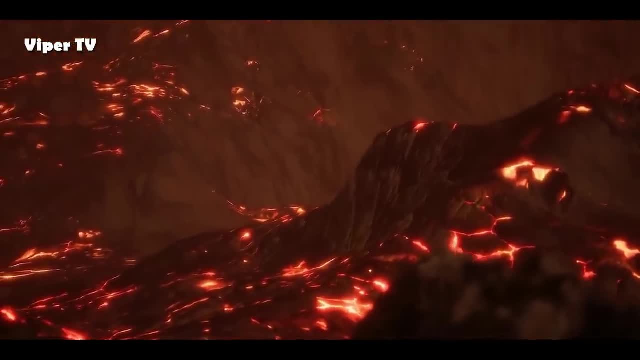 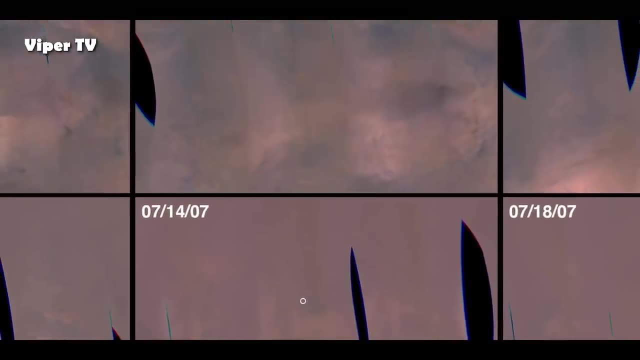 the northern lowlands were resurfaced by volcanic activity in a similar fashion to the smooth lunar seas, which accounts for their lack of cratering relative to Earth. This is due to the much more ancient terrain to the south, The oldest terrain on Mars. 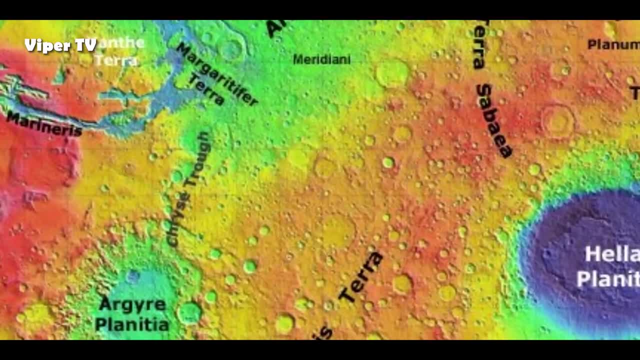 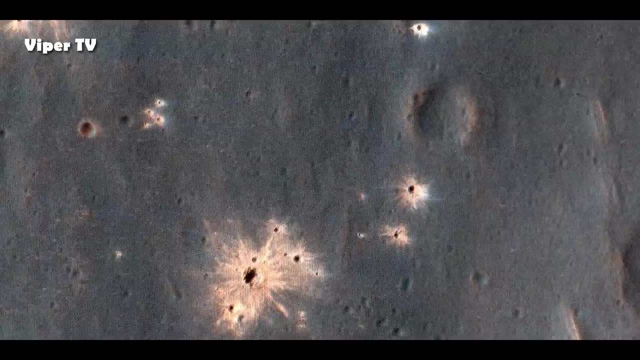 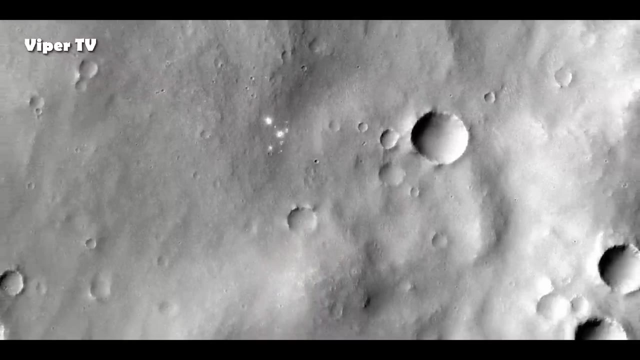 is found in the Noachis Terra region of the southern highlands. It is characterised by heavy cratering reminiscent of the far side of the Moon. Even small craters in the Noachian highlands are heavily eroded, which suggests the regular, if not persistent, presence of liquid water. 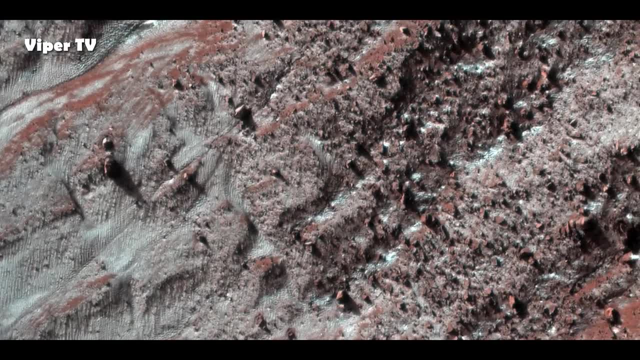 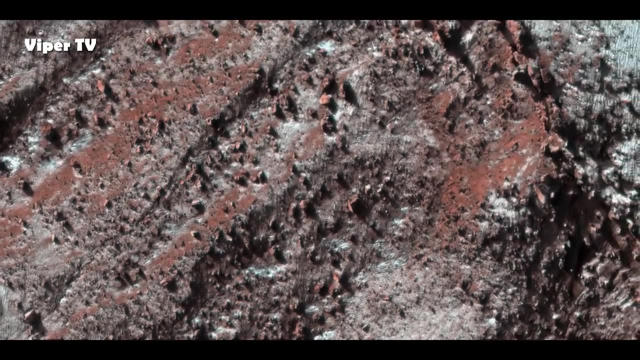 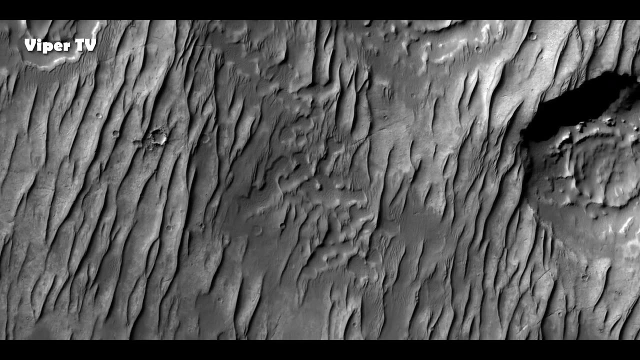 There are dry river valleys and deltas and evidence of water pooling in the craters and overflowing their walls, forming interconnected networks of lakes. This is how we know Mars was once a warmer and wetter world, at least occasionally. The evidence is written across the land of Noah. 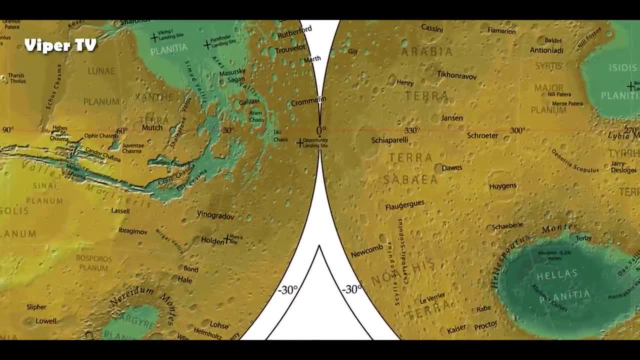 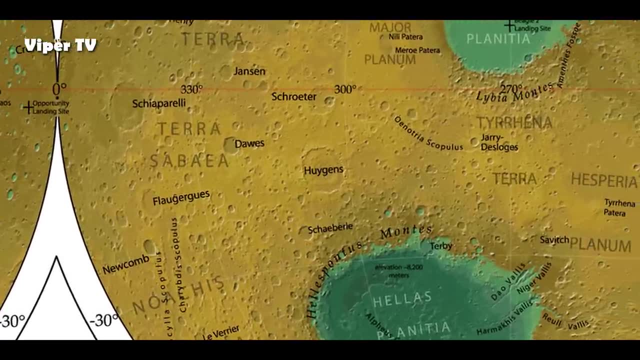 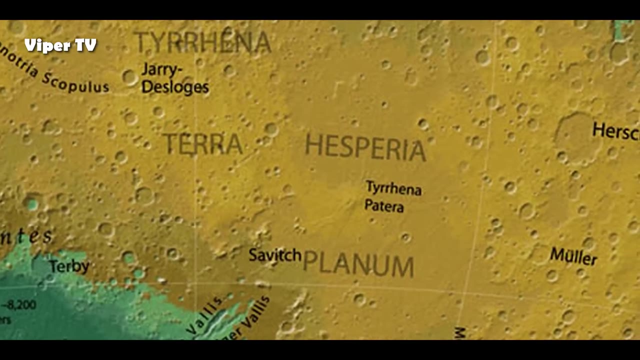 In contrast, the younger terrain of Hesperia Planum displays much less evidence of regular erosion by water, but bears the scars of occasional catastrophic floods that cut deep valleys over very short periods of time and may have formed temporary lakes. The Amazonas Planitia region shows little sign of flowing water. 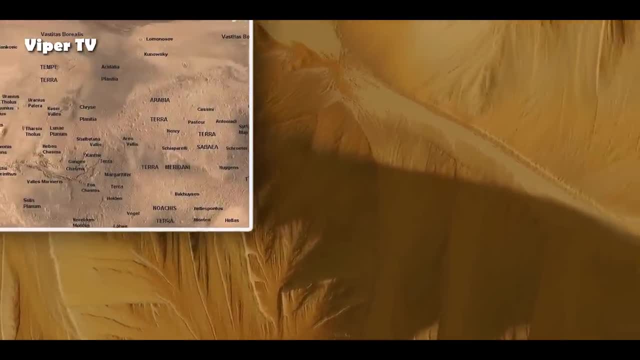 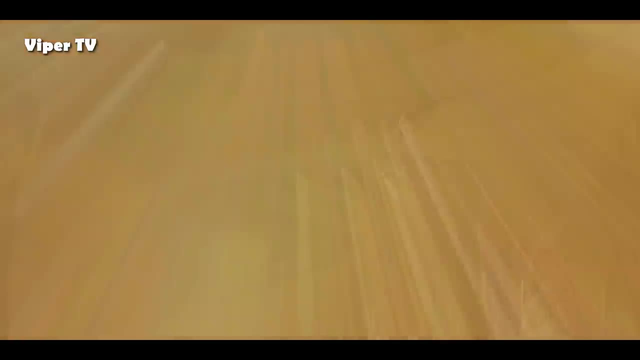 fewer impact craters and less evidence of active volcanism, suggesting it was formed more recently, when Mars was significantly less geologically active. The persistence of surface features over many billions of years in the Noachian, Hesperian and Amazonian regions. 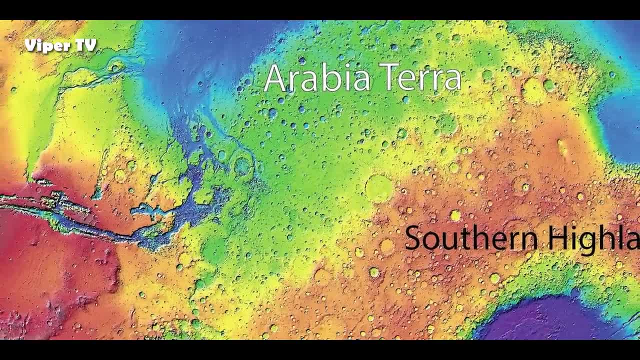 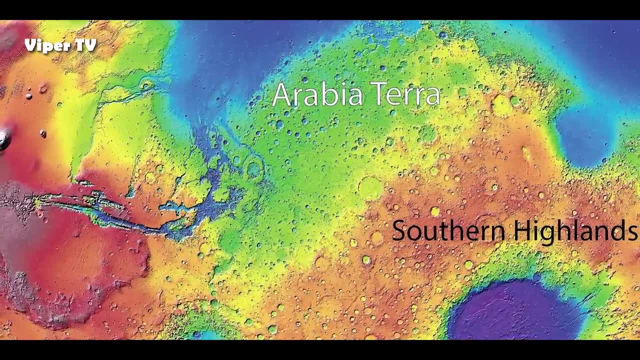 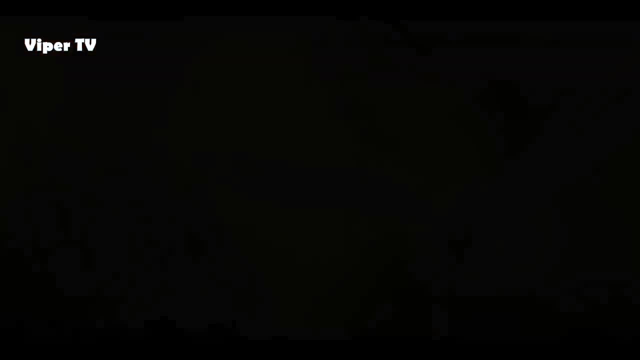 has led to the historical epochs of Mars being named after the distinctive terrains that still bear the characteristic marks of the climate and geological activity that formed and sculpted them. The Noachian period was the earliest and wettest, and coincided with the origin of life on Earth. 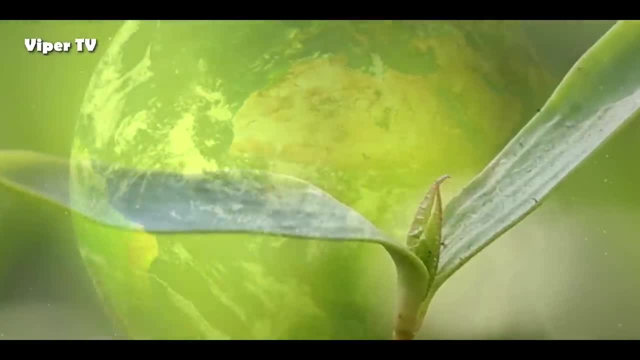 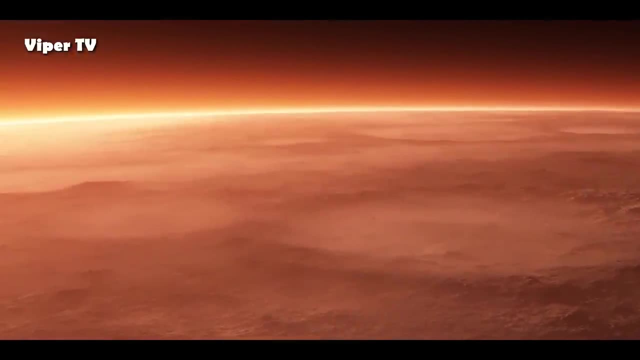 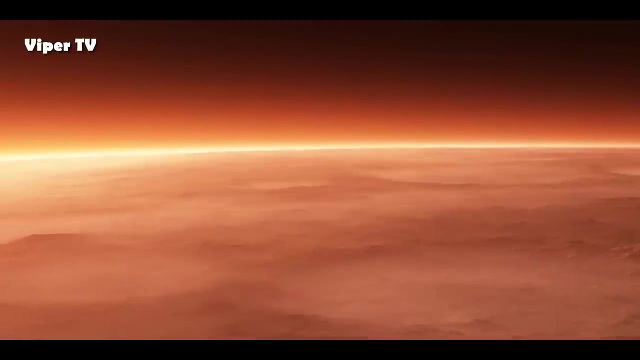 around four billion years ago, when conditions on both worlds appear to have been very similar. The Martian atmosphere may have been denser than Earth's and dominated by carbon dioxide, but significant questions remain about how such an atmosphere could have warmed Mars sufficiently to deliver the warm, wet climate. 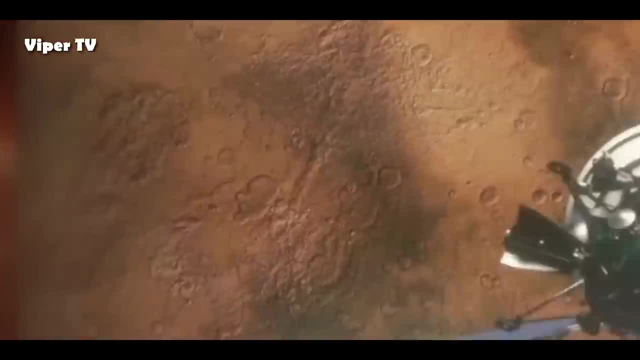 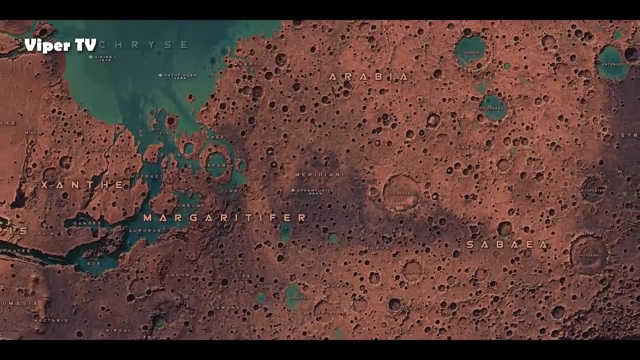 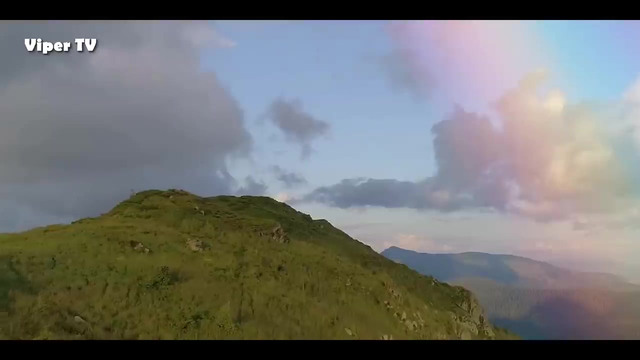 and how that atmosphere was lost? The MAVEN spacecraft currently in orbit around Mars aims to answer this question. The Noachian period ended as Mars became increasingly cold and arid around 3.5 billion years ago, just as life was gaining a foothold on Earth. 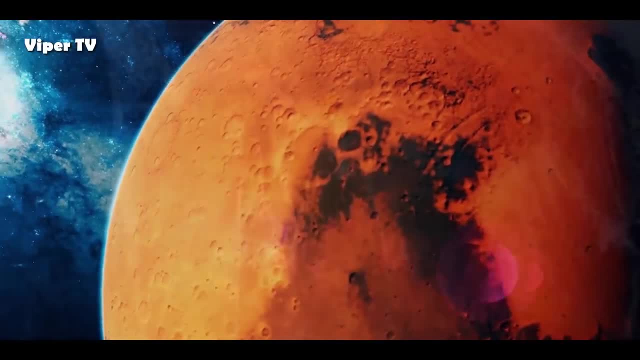 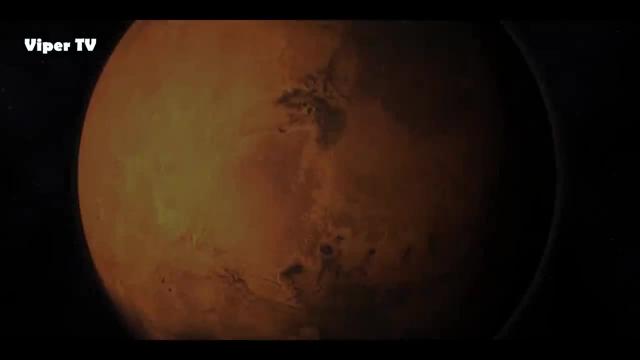 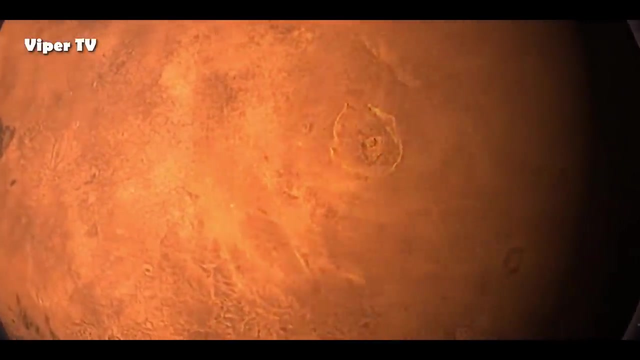 The Hesperian period. the time of catastrophic floods ran from the end of the Noachian to around 3 billion years ago, when Mars entered its current frozen, arid phase, punctuated by occasional volcanic activity and the large-scale movement of ice. 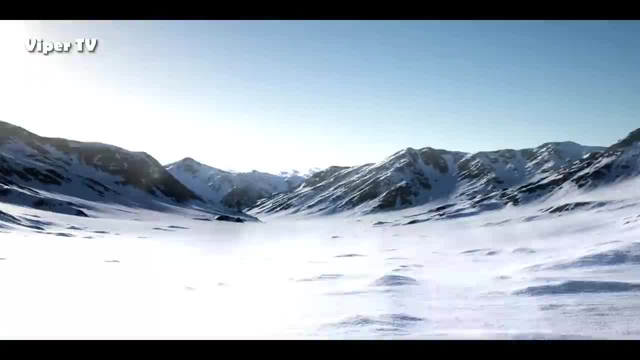 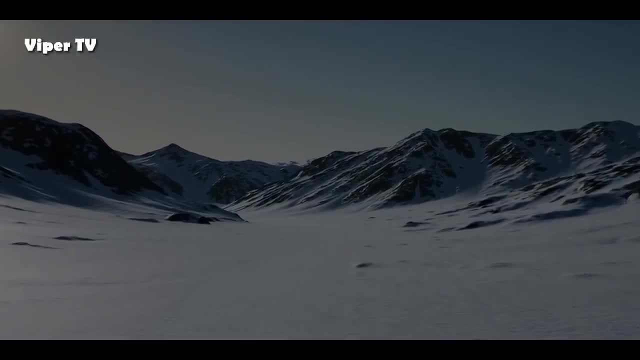 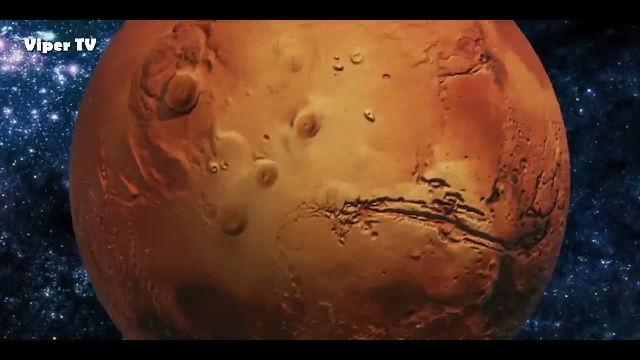 but with very little evidence of flowing water. The long, three-billion-year freeze from the end of the Hesperian to the present day is known as the Amazonian. This is a summary of what we know about Mars. The whys pose a significant challenge to planetary scientists. 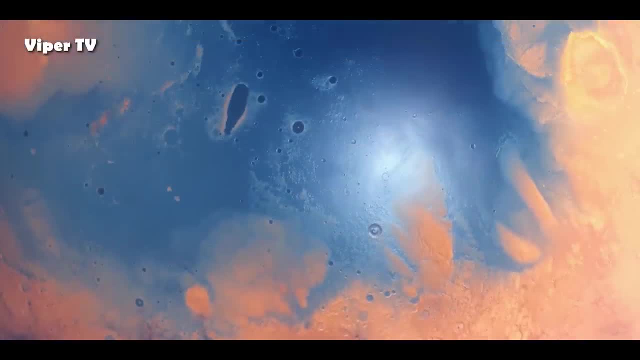 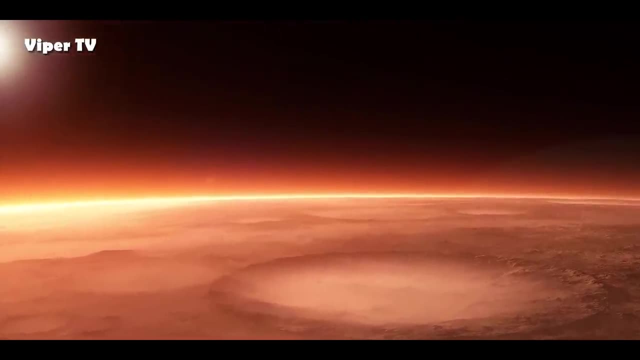 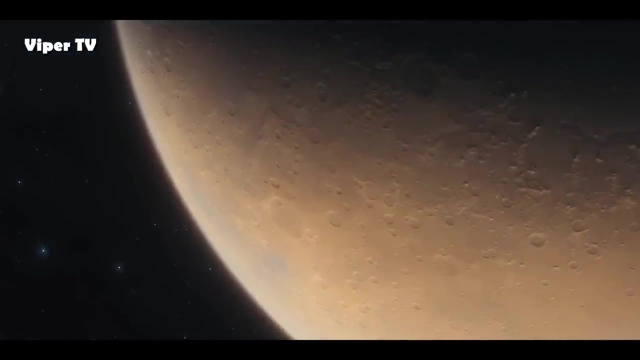 Given a warm, wet and seemingly stable world early in its history, what triggered the loss of atmosphere and descent into modern-day aridity? What happened to the water on Mars? Was it lost to space or does it persist today as surface ice? 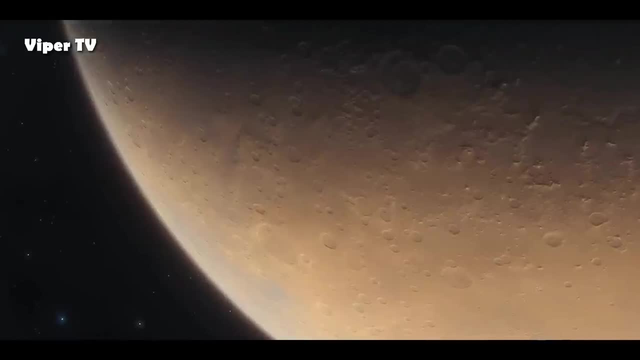 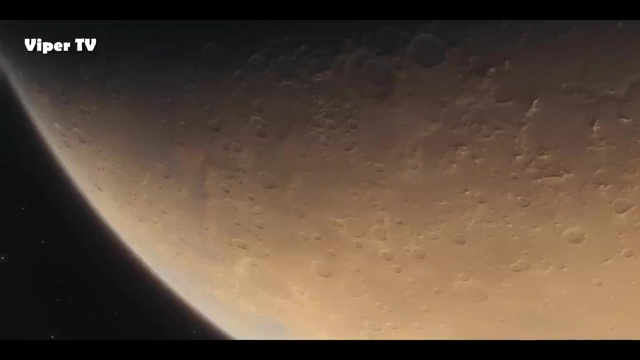 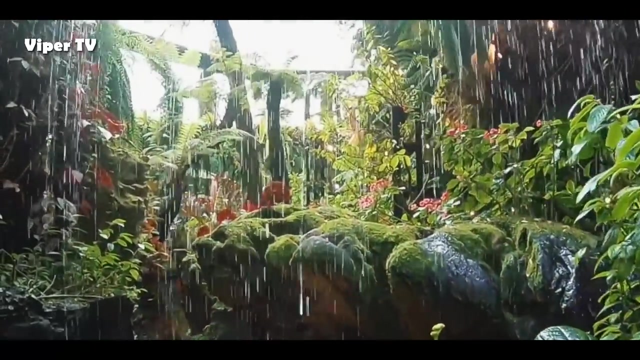 or in subsurface rocks or reservoirs? If so, how much water is still accessible? Could we exploit the ancient reservoirs of Mars to support a human colony? And, perhaps most significantly of all, did life arise on the planet during the Noachian period? 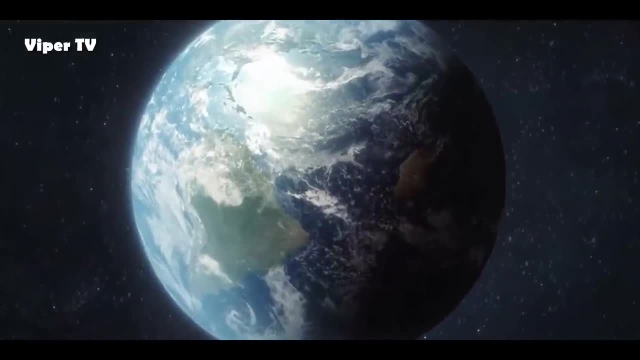 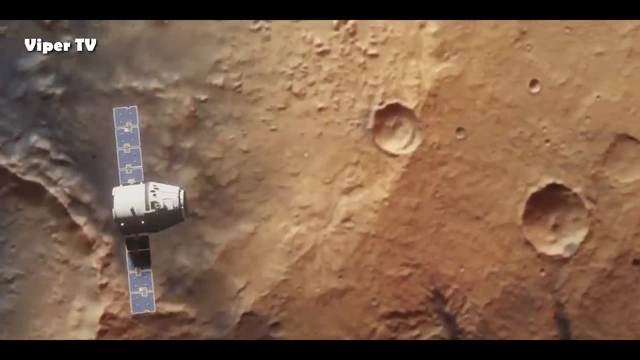 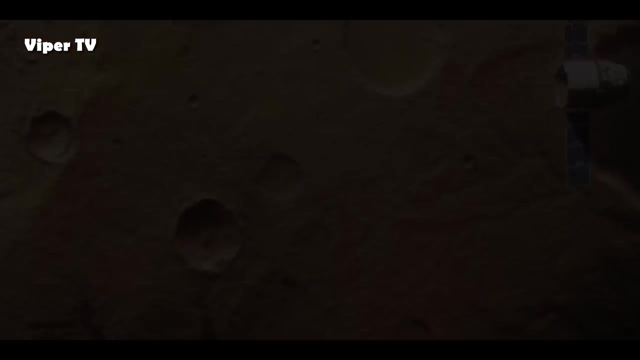 coincident with the origin of life on Earth, And could that life still be present on Mars today? The current fleet of spacecraft in orbit around Mars and roving across its surface has been designed to answer these questions. Mars today is a planet buzzing with activity. 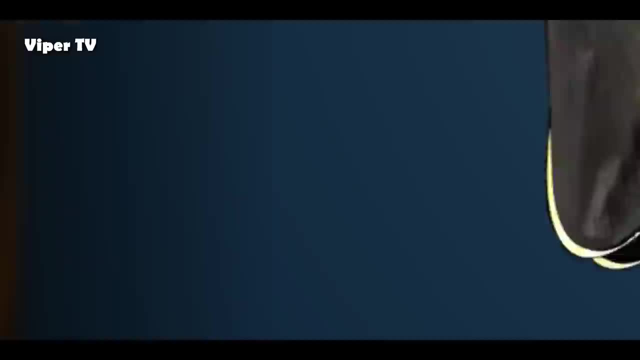 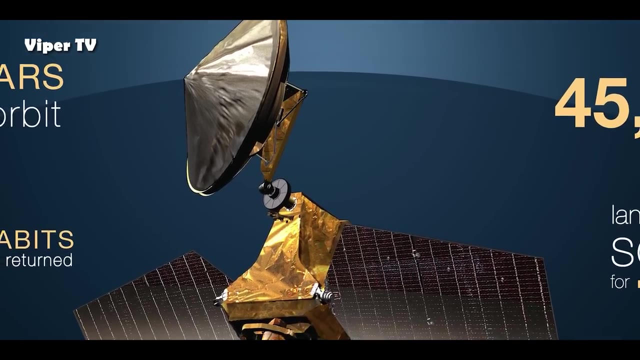 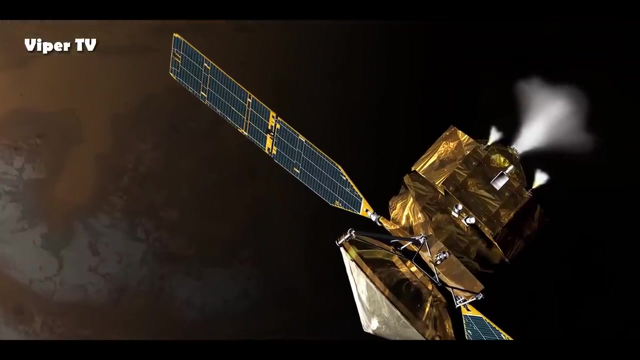 Communications to Earth and the Martian internet are managed by the Mars Reconnaissance Orbiter, MRO, an orbiting bridge between worlds. MRO carries the HiRISE instrument, a camera with resolution high enough to see basketball-sized features on the Martian surface. 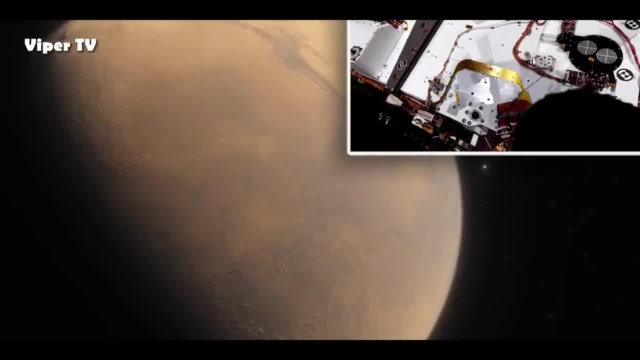 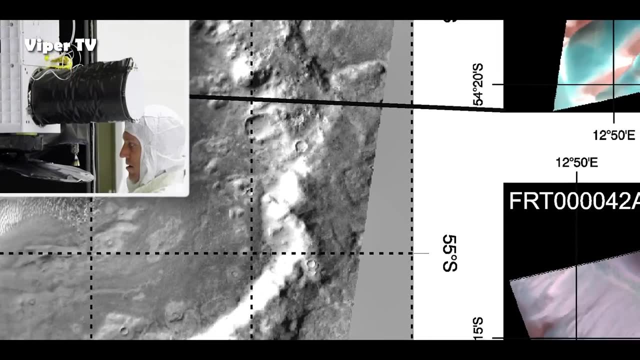 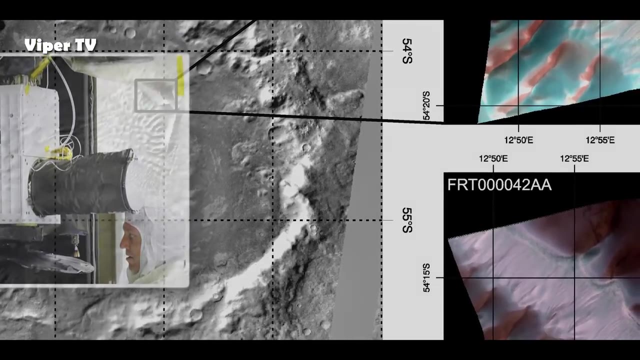 The Mars Colour Imager Marky camera monitors Martian weather and the Compact Reconnaissance Imaging Spectrometer for Mars, CRISM, identifies mineral deposits, particularly those formed in the presence of surface water. Orbiting with the MRO is the Mars Atmosphere and Volatile Evolution Mission MAVEN. 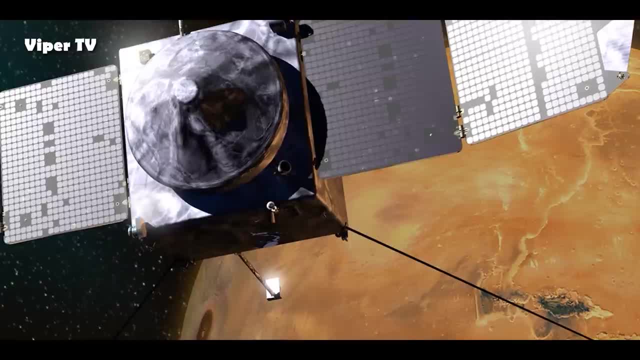 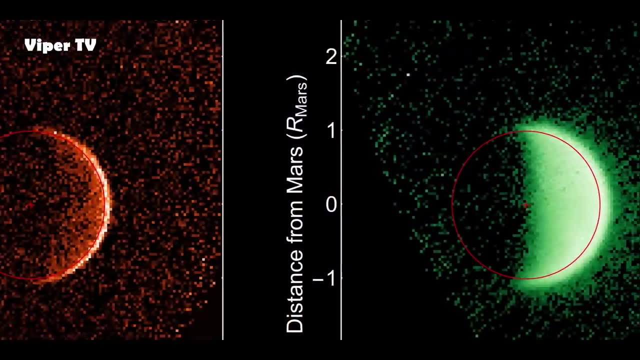 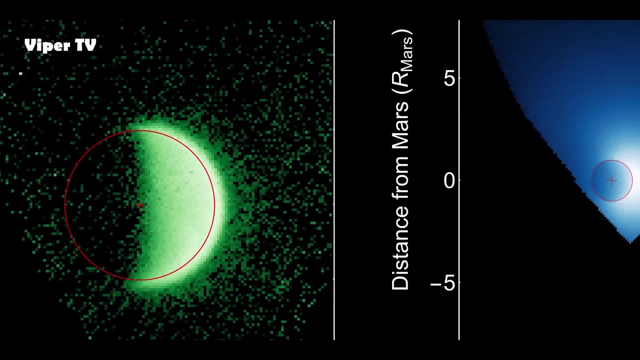 This camera-less spacecraft operates between 150km and 6,000km above the Martian surface, Measuring the composition of the atmosphere at different altitudes and observing how the tenuous gases are stripped from the planet by the solar wind. Mars Odyssey is the veteran of the orbiting fleet. 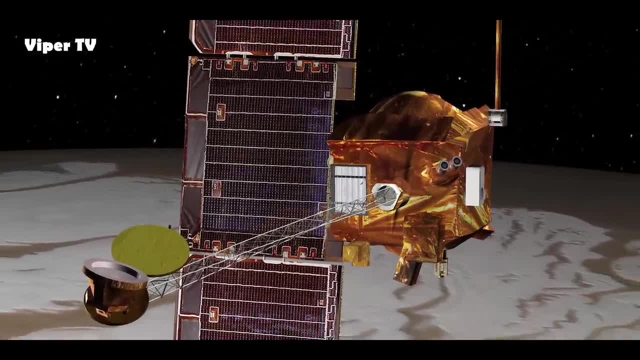 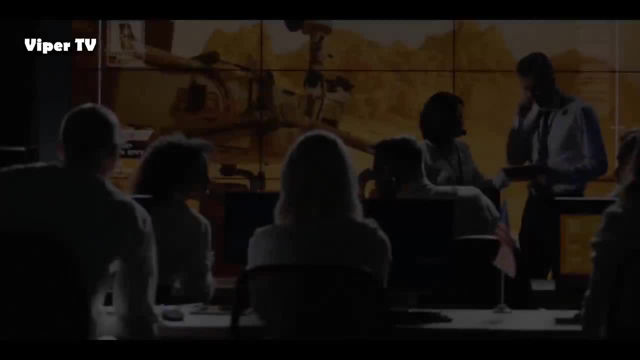 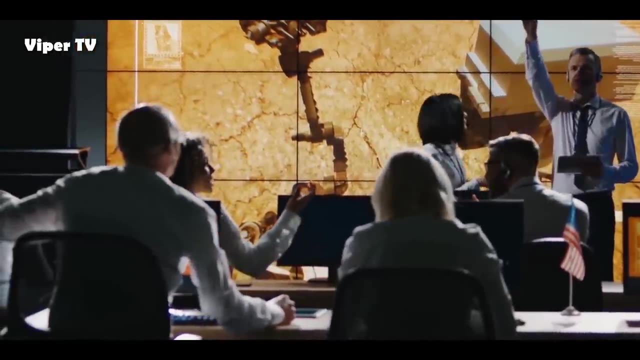 having arrived in 2001 and still being operational in a polar orbit, searching primarily for water ice on the surface. Mars Express is a European Space Agency mission that is delivering high-resolution photographs, mineralogy data, radar, investigation of the near subsurface. 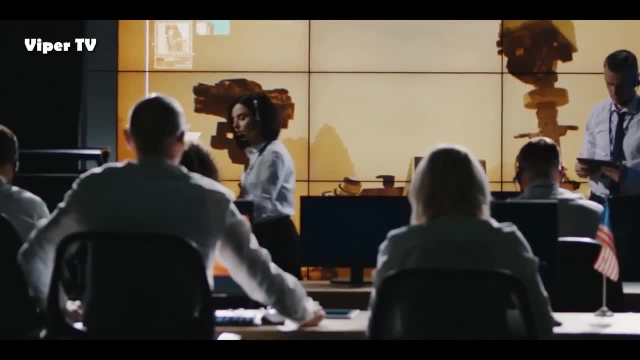 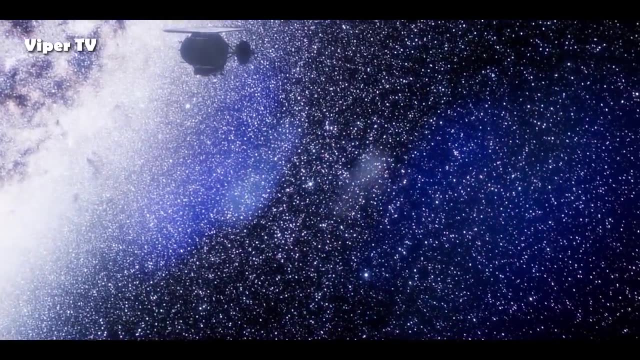 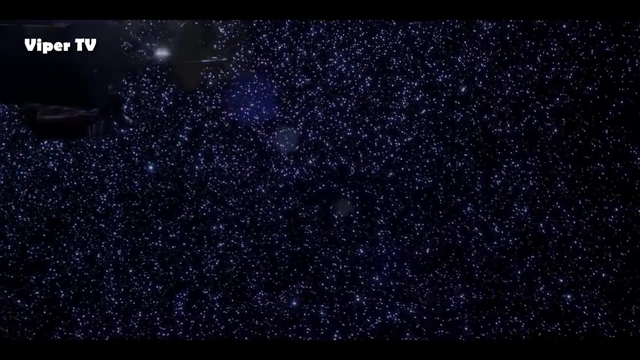 and atmospheric measurements, including the search for methane, a gas that on Earth is associated with biological activity. India's Mangalyaan space probe is primarily a technology demonstrator, but it carries a secondary scientific package capable of investigating atmospheric composition. The newest arrival at Mars. 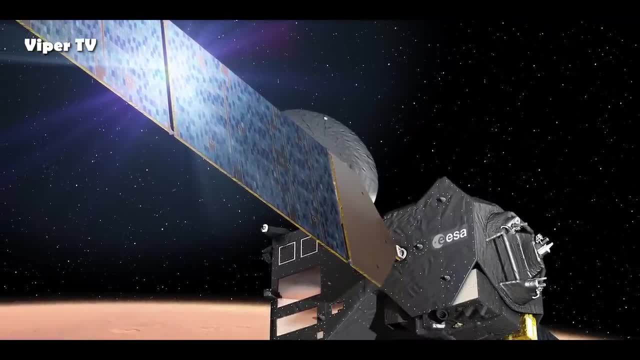 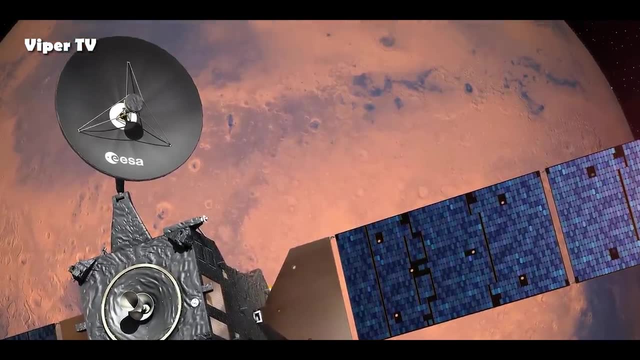 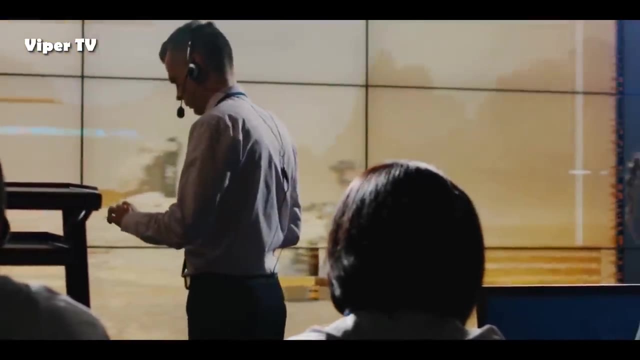 is the joint European Space Agency Russian ExoMars Trace Gas Orbiter, which will observe seasonal changes in the Martian atmosphere and search for subsurface water deposits. The spacecraft will form the communications bridge for ESA's ExoMars rover, due to land in 2021.. The two most recent explorers of Mars are the Opportunity and Curiosity rovers. The Opportunity rover landed on the Meridiani Planum close to the Martian equator, on 25 January 2004,, with a planned lifetime of 90 Earth years. 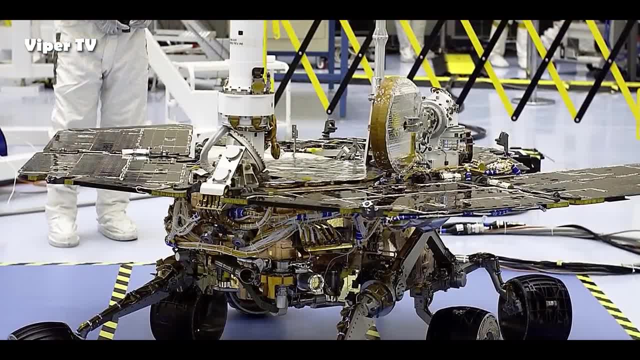 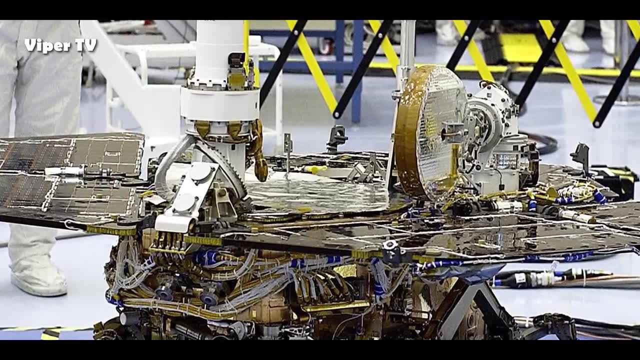 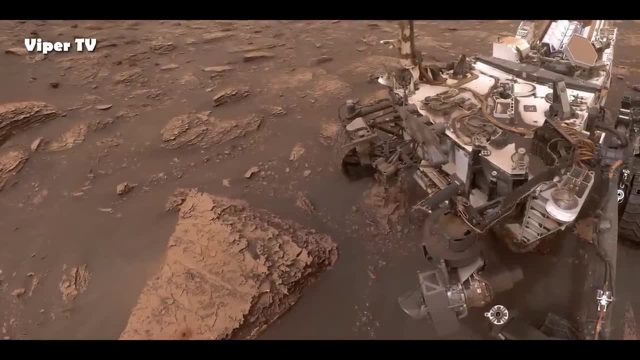 In a spectacular testament to the Jet Propulsion Laboratory's engineering excellence, Opportunity remained operational until a planet-wide dust storm covered its solar panels in June 2018, after over 14 years and a journey of 45 kilometres on the surface of Mars. 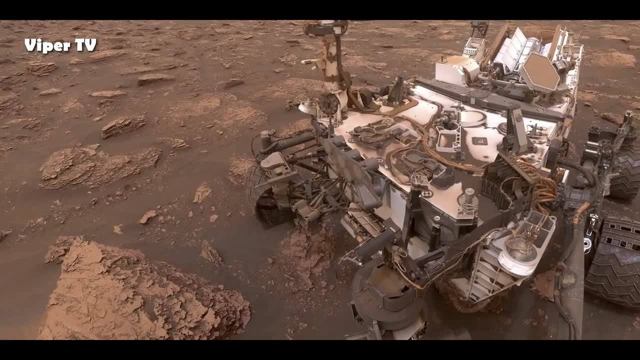 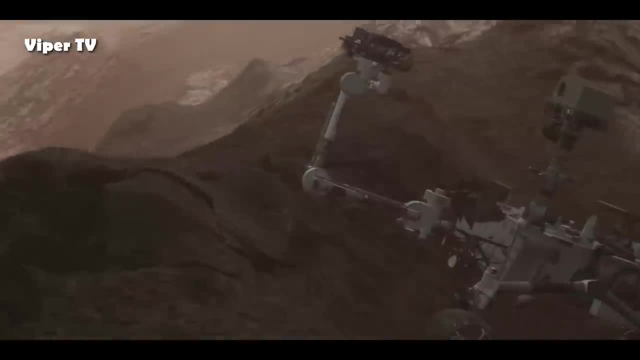 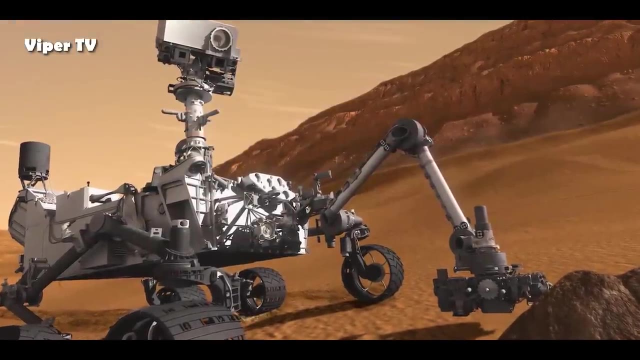 exploring the Endurance, Victoria and Endeavour craters. On 13 February 2019, Opportunity was finally declared. Opportunity's younger and far larger companion on Mars is Curiosity, the most massive and most capable spacecraft ever to touch down on a planet beyond Earth. 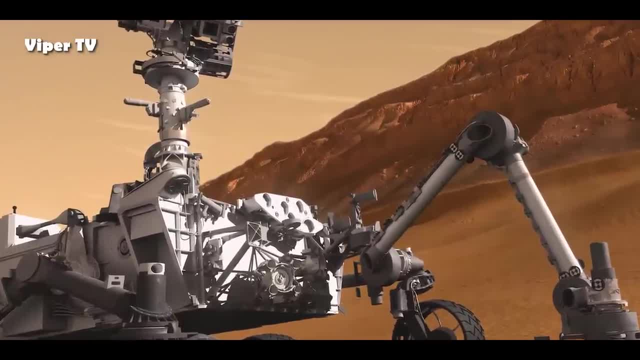 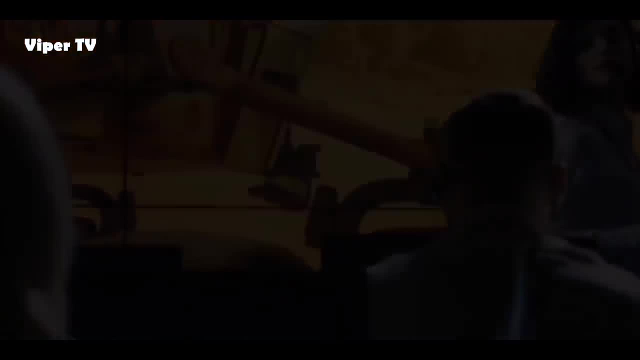 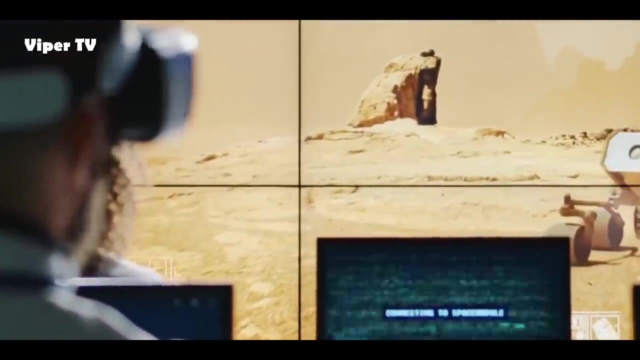 The landing itself was a tour de force of engineering ingenuity and audacity. The enormity of the mission is best described through the words of Alan Chen: operations lead at NASA for the Curiosity mission at 10.31 PDT, when he said: 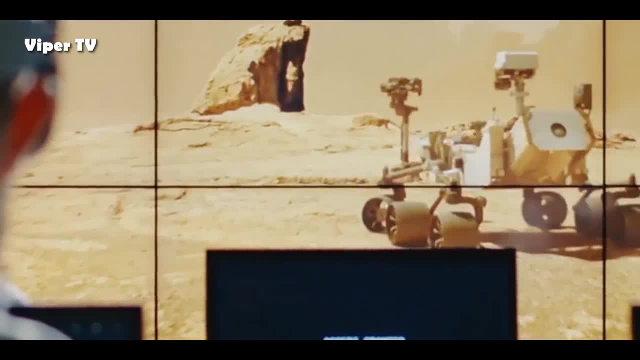 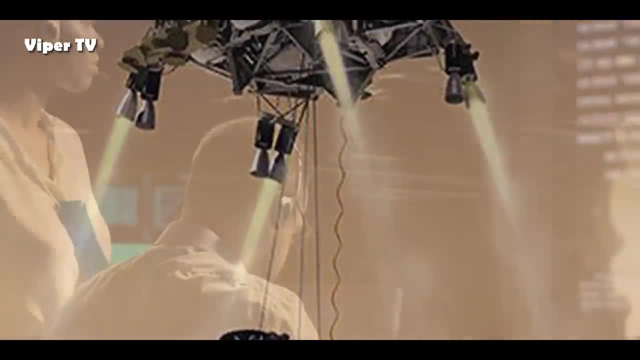 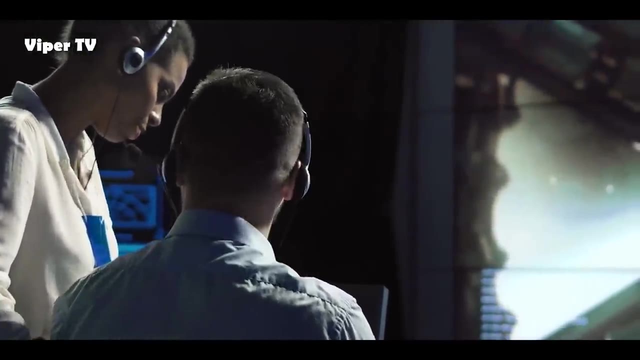 at 10.31 PDT on 5 August 2012,, watching the landing at the Jet Propulsion Laboratory alongside the team. The engineers described it as seven minutes of terror. seven minutes to manoeuvre a spacecraft that had taken eight years to design and build. 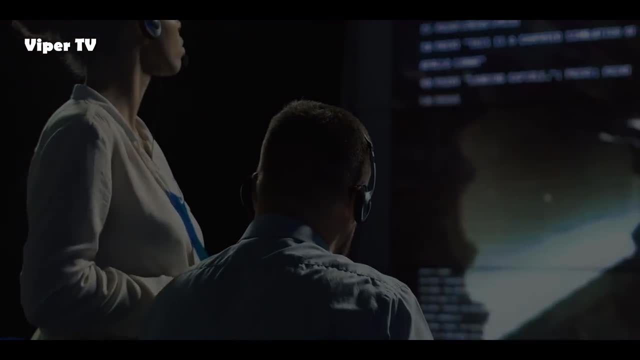 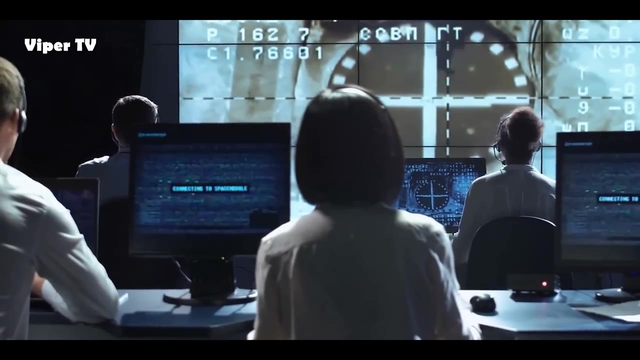 with a programme cost of more than $2.5 billion. from 13,000 miles per hour at the top of the Martian atmosphere to a soft landing on the surface of the planet. The tension reflected the high stakes. The Mars Science Laboratory mission. 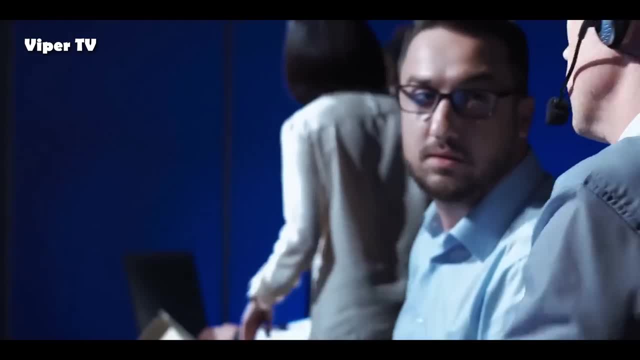 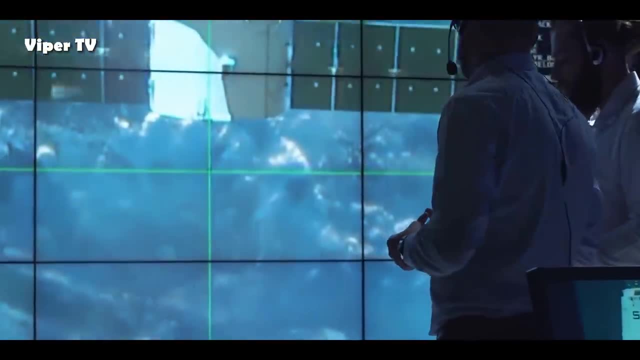 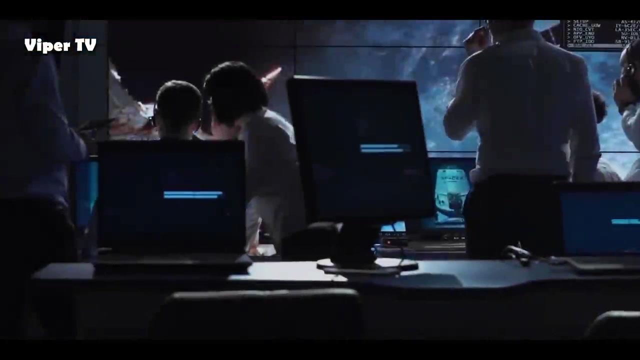 to give the lander and orbiter their full title, was a high-risk flagship science mission in the same category as Voyager, the Hubble Space Telescope, Viking and Cassini, and was beset by cost and schedule overruns and controversy. This is, in many ways, unsurprising. 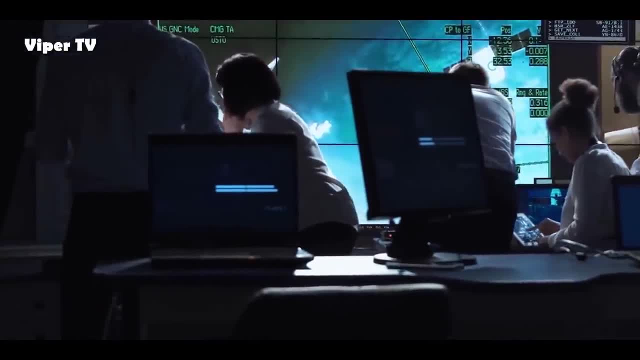 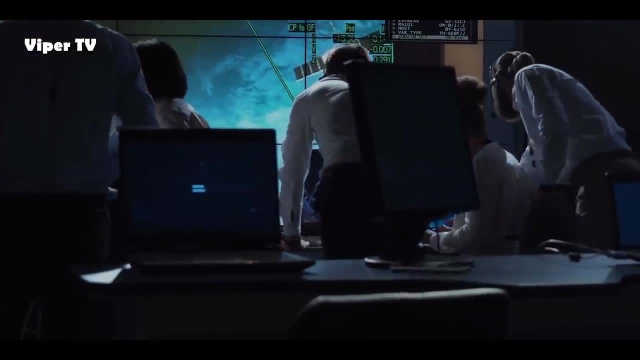 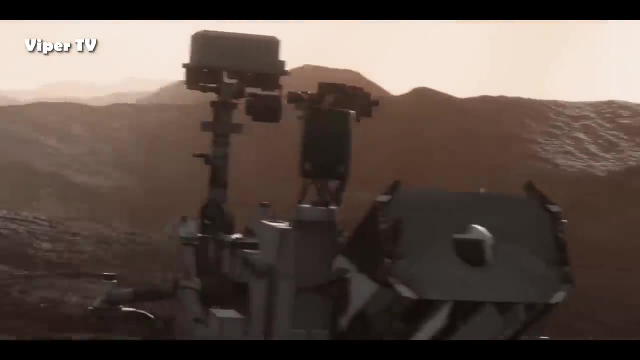 New technologies and ambitious scientific objectives are difficult to implement and achieve and, in part because of this, deliver great rewards. In hindsight, nobody would question the value of any of these missions, which have delivered some of the greatest insights and most inspiring images in the history of exploration. 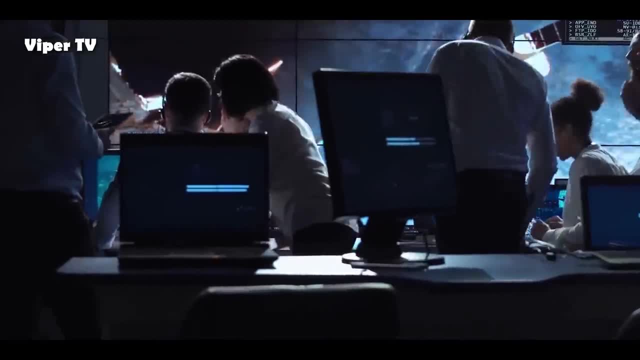 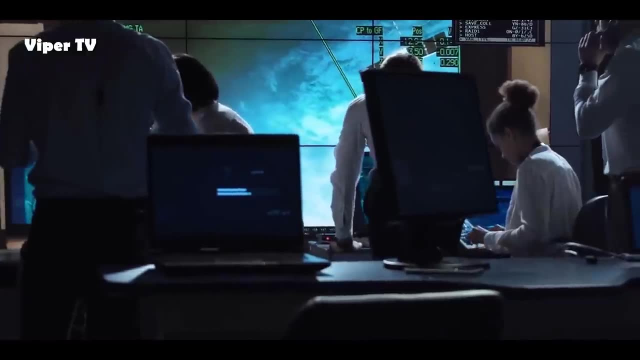 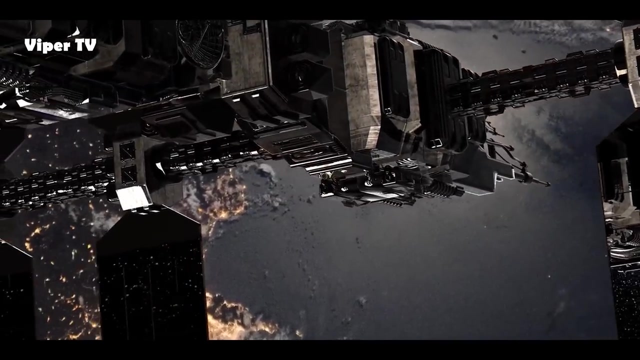 Yet this never prevents beam counters and rival scientists with agendas and, more charitably, budgetary challenges of their own whinging and even considering cancellation. This is naive. Funding for science is almost always grudging from a political class whose view of the acquisition of knowledge 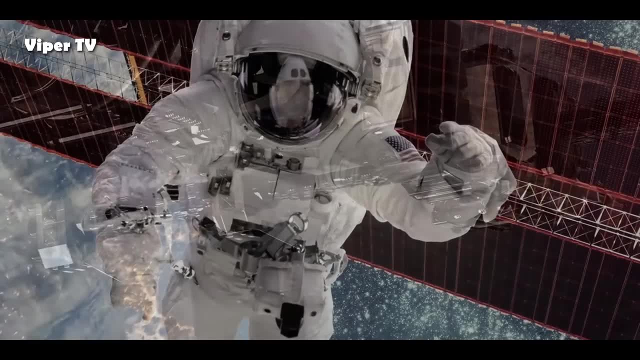 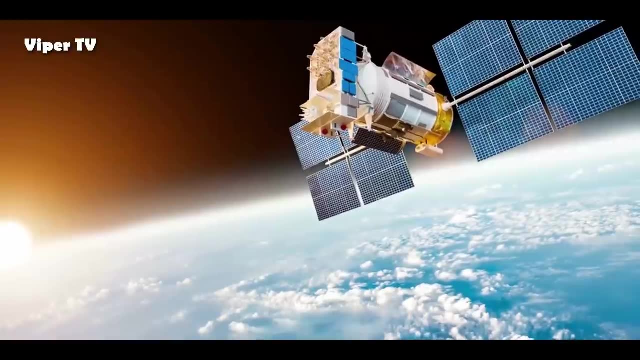 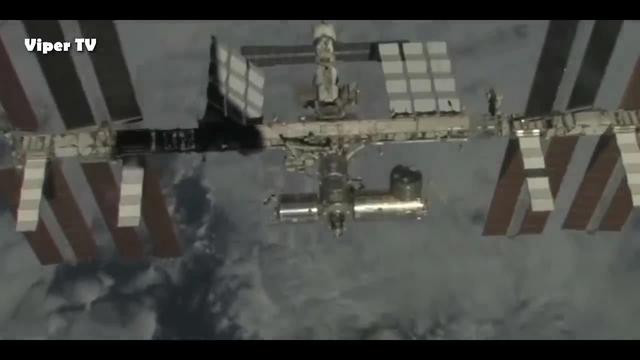 is utilitarian. The far deeper value of exploration as a critical part of the internal voyage of our species, bringing us into direct confrontation with the mystery of our existence, is lost on them, at least until occasional Johnsonian President, not Alexander Boris de Pfeffel moments. 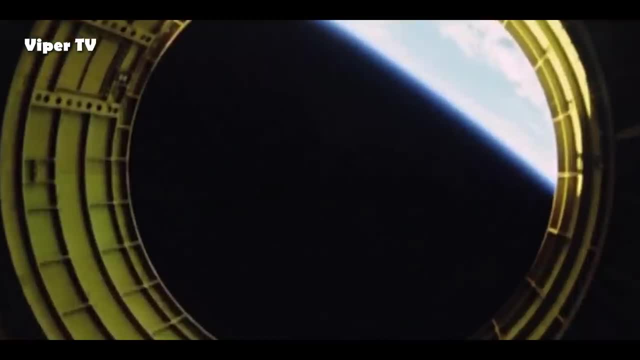 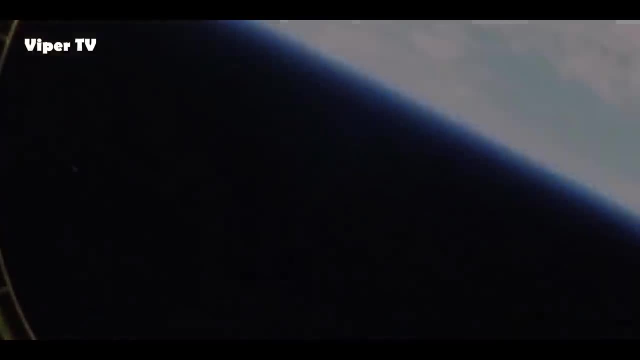 It may be. it may just be that life as we know it, with its humanity, is more unique than many have thought, and we must remember this, Which means that a cancellation of one project does not mean an uplift in funds for another. 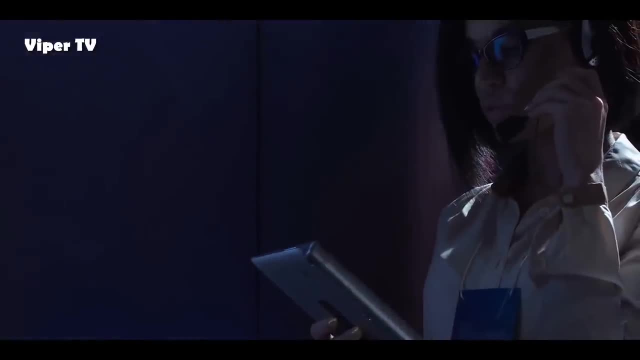 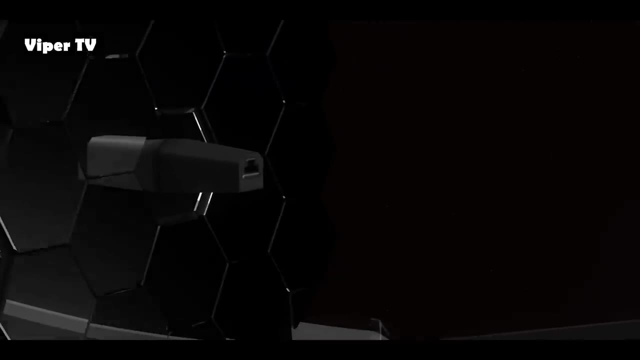 More likely, the budget will be lost to science. At the time of writing, the same issues plague another NASA flagship mission, the James Webb Space Telescope, As Robert D Baum wrote in an op-ed article for Space News in December 2008,. 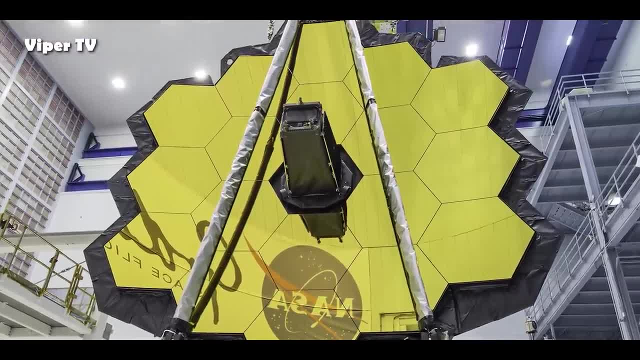 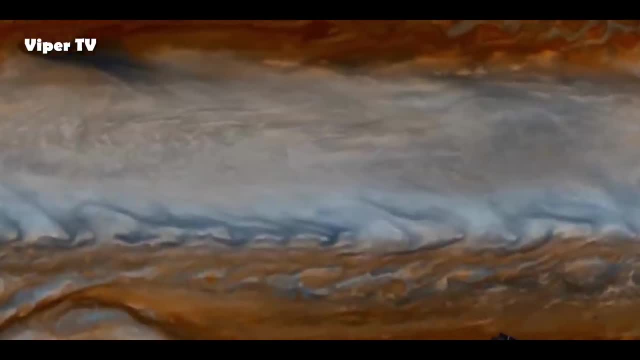 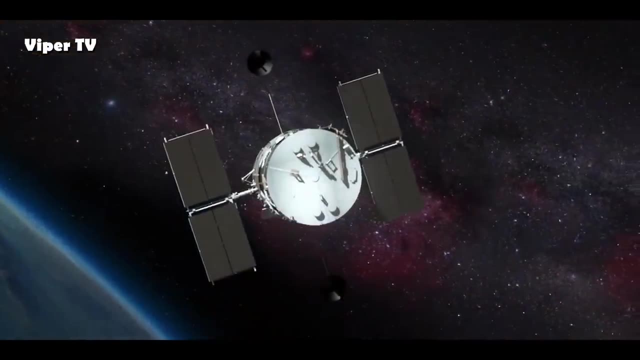 at the height of the Mars Science Laboratory controversy. when implementing flagship missions, cost and schedule overruns are not uncommon, But history shows that the mission return often eclipses the expenditure. The Hubble Space Telescope experienced a development cost overrun several times its approved project budget. 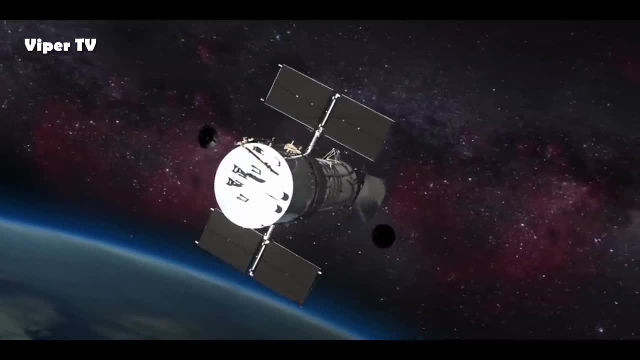 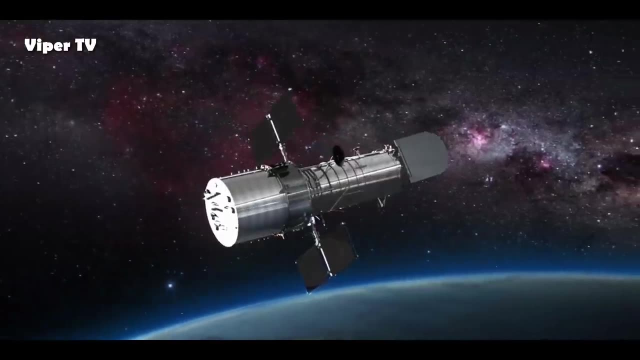 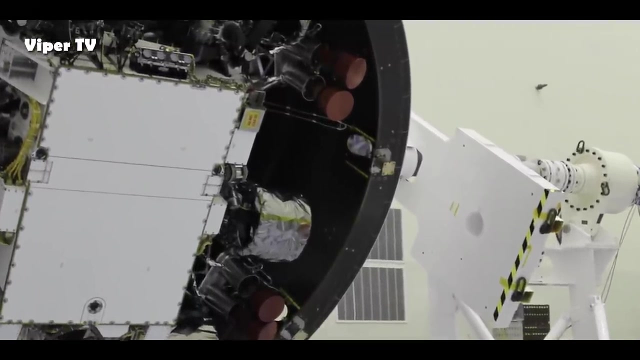 and was launched much later than originally planned. In hindsight, would any rational space scientist not concede that the return from Hubble was worth the investment, Given the fee bracket and the fragile atmosphere? however, no amount of philosophy or reason would mitigate the costs of failure. 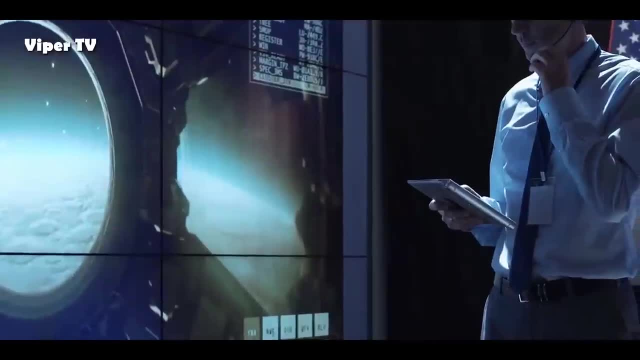 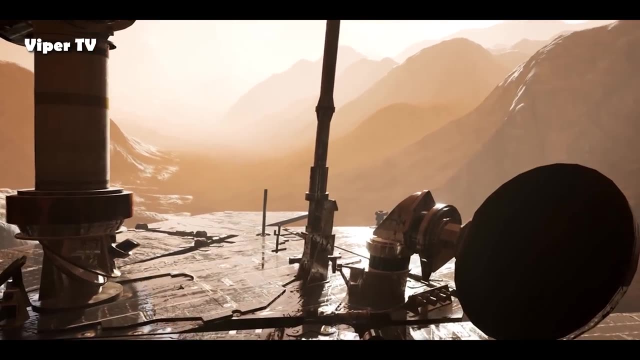 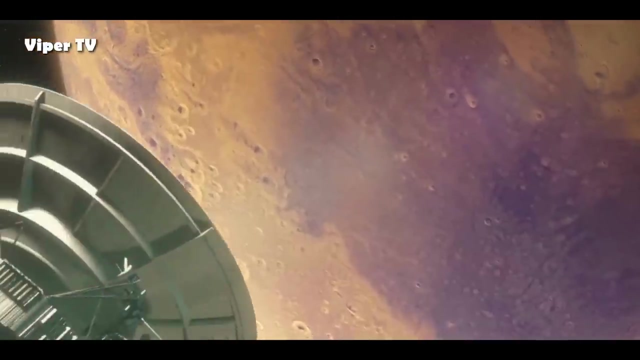 of the Mars Science Laboratory mission. A landing accident was both possible and unthinkable. Delivering almost a ton of fragile rover onto the surface of Mars with pinpoint accuracy is not trivial, which is perhaps why the chosen engineering solution seemed not to put too fine a point on it. daring. 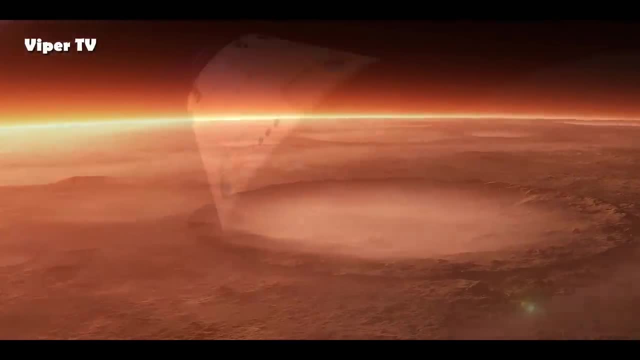 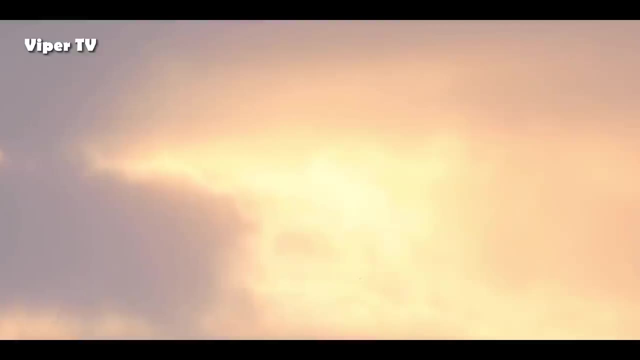 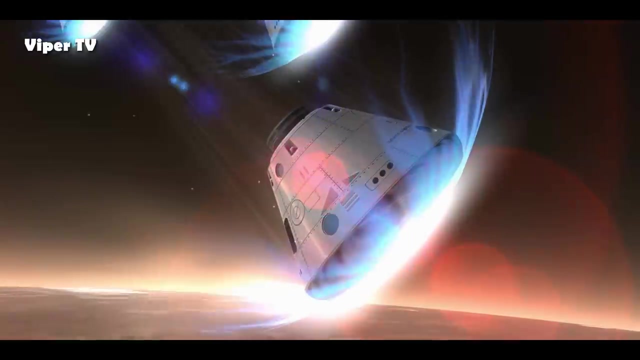 Mars has a thin atmosphere, so slowing down a spacecraft when it's travelling around ten times faster than a bullet is hard. And yet the atmosphere is thick enough to apply sufficient frictional heating to destroy a spacecraft without adequate protection, and turbulent enough to cause significant uncertainty. 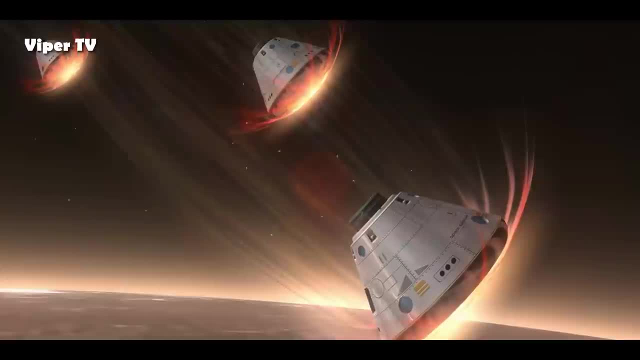 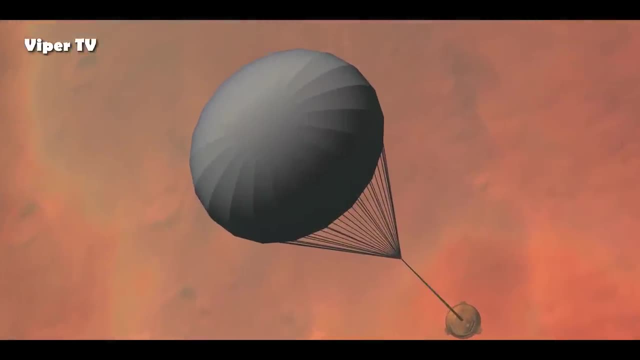 in the landing site of an unsteered vehicle. This renders the more obvious engineering solutions redundant. You can't simply deploy a parachute and float to the surface. The 1970s Viking landers used a combination of heat shields during aerobraking. 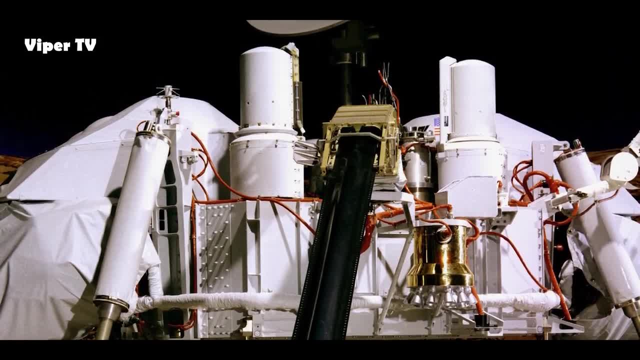 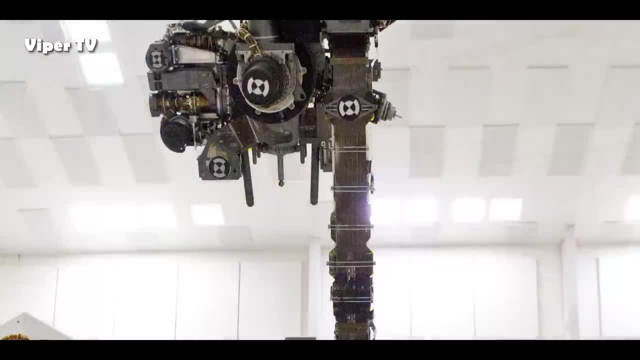 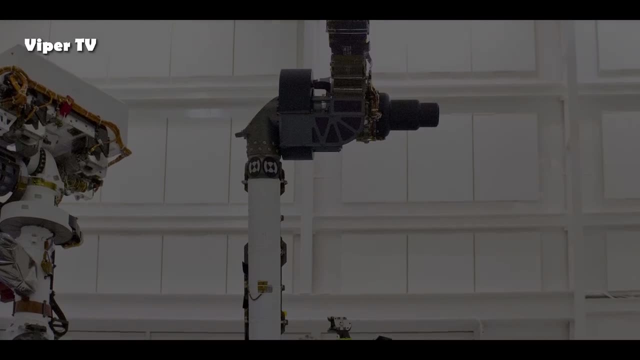 parachutes and retro rockets with success. But the Curiosity engineering team dismissed this tried and tested solution. It did not allow for high enough precision or for the gentle landing required for the pinpoint delivery of a large rover with delicate wheels. The Viking landers had legs built like tanks. The Viking landers also carried their heavy descent rocket systems with them to the ground, which didn't matter because they stayed put. Curiosity would have had to lug all this unnecessary mass around Mars for years. The Opportunity rover, her sister ship Spirit and the earlier Mars Pathfinder. 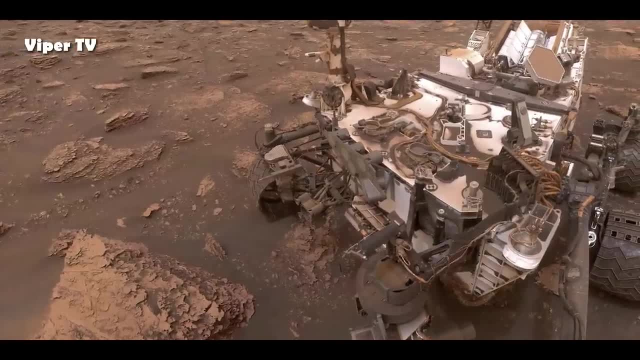 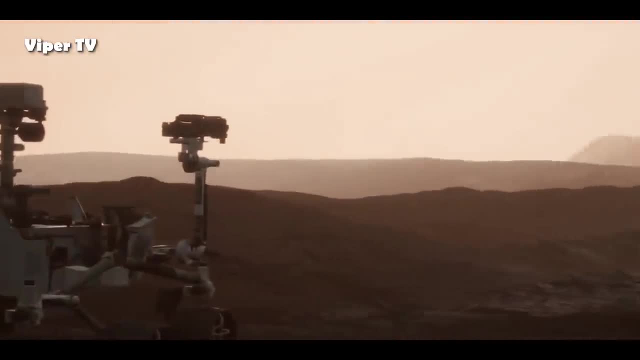 employed a combination of aerobraking parachutes, rockets and airbags to cushion the falling spacecraft. But these previous rovers were lightweight in comparison, at just over a fifth of the mass of the gargantuan Curiosity, A rover of this size and complexity. 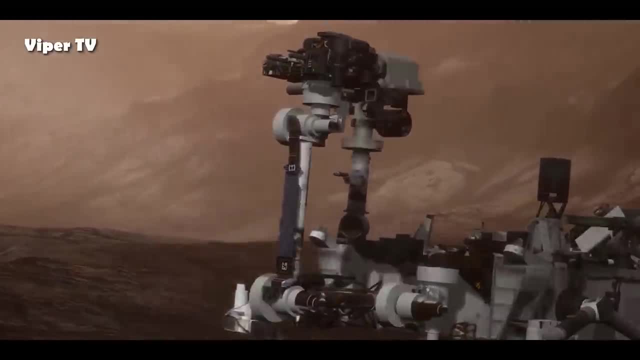 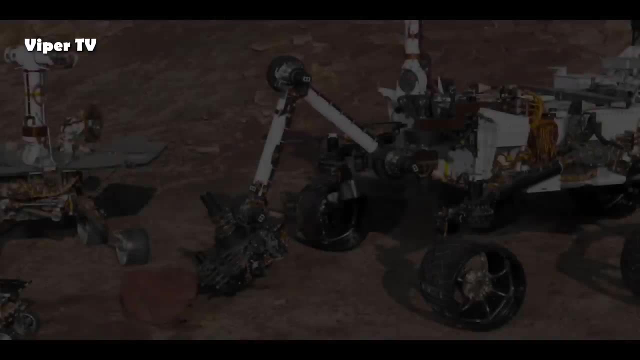 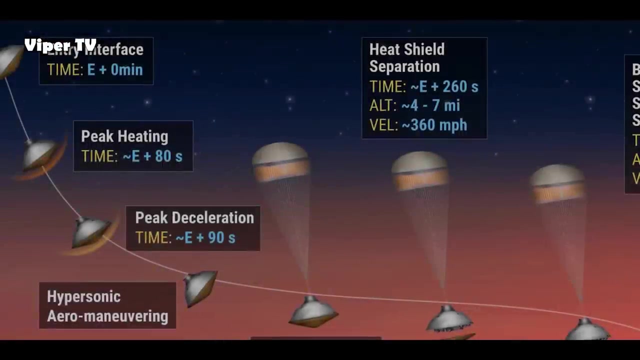 bouncing over the surface in an airbag cocoon was not considered feasible, primarily because of the sheer mass of the airbag system needed to cushion the impact. The lightweight Opportunity rover's landing system was almost twice the mass of the rover itself. The chosen entry, descent and landing procedure. 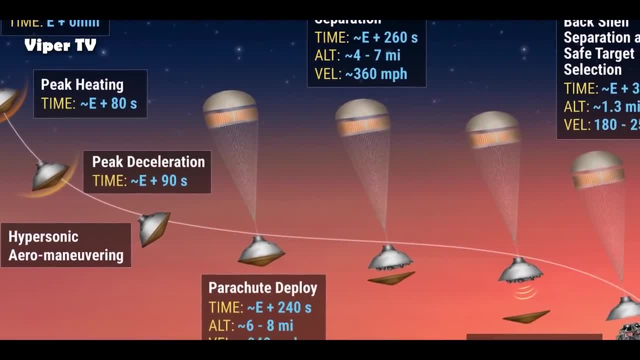 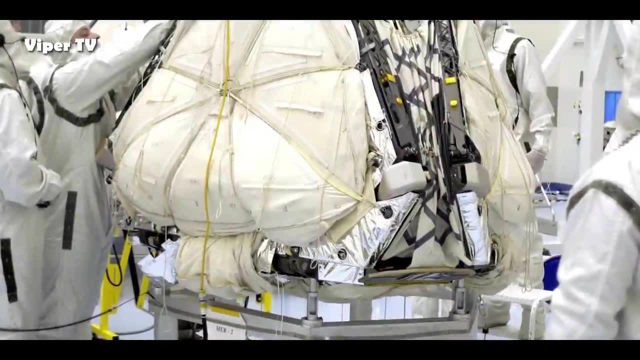 EDL for Curiosity was described by mission lead Adam Stelzner as the result of reasoned engineering thought. A beautiful example of the truism that reasoned engineering thought and common sense, at least of the sort possessed by the average golf club, bore. 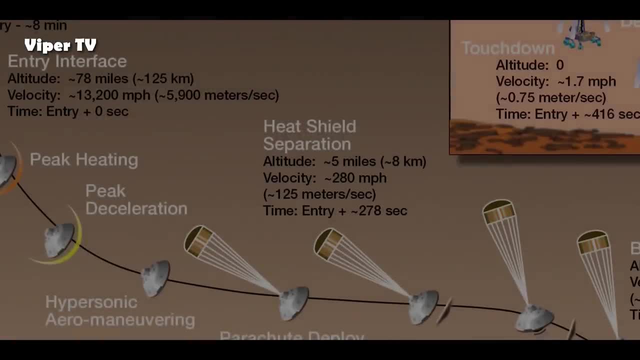 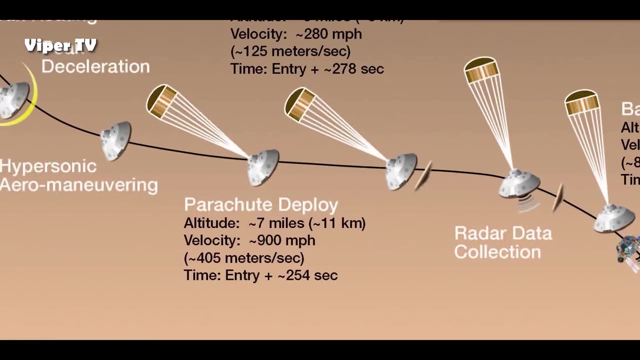 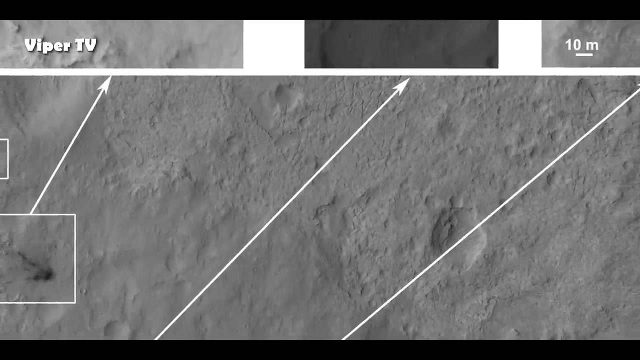 do not always match up. The Curiosity EDL appears to the untrained eye to be bonkers or maybe overcomplicated, but it wasn't and it worked. Tucked up inside a protective shell, Curiosity encountered the outer layers of the Martian atmosphere. 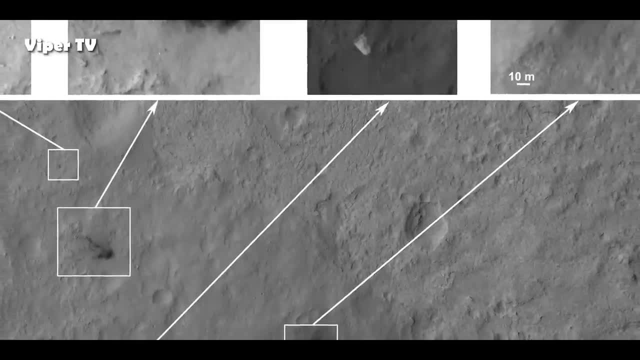 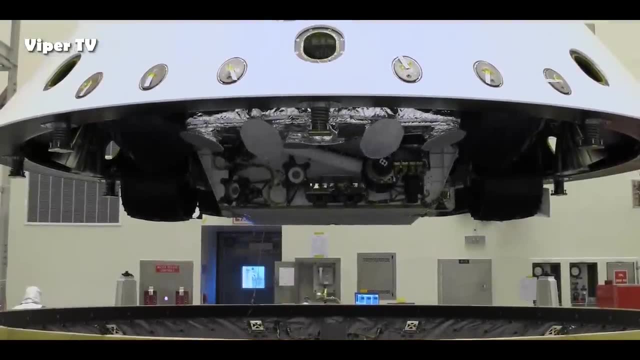 125km above the surface and travelling at around 20,000km per hour at 10.23pm Pacific Daylight Time on 5th August 2012.. The spacecraft at this stage cocooned inside a protective enclosure. 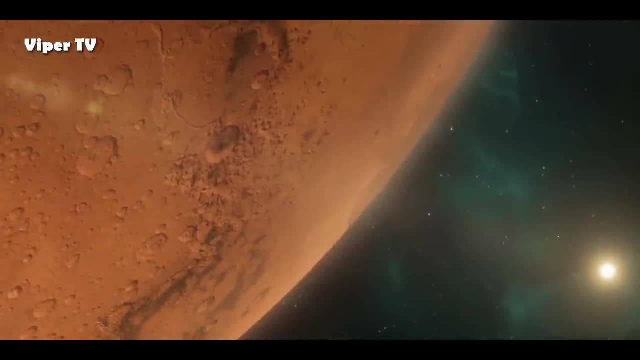 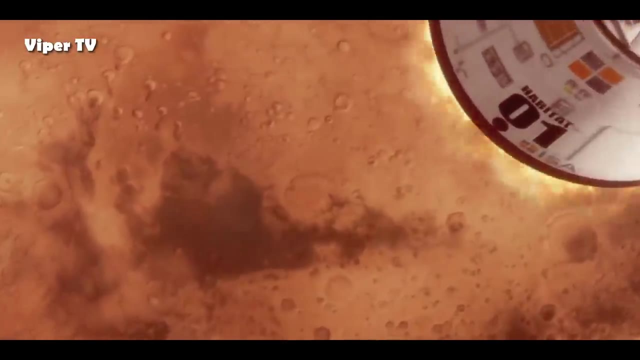 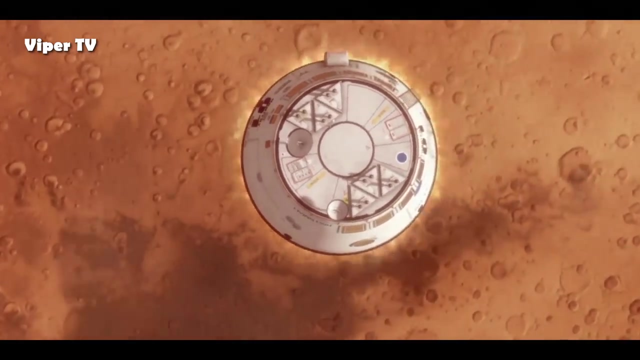 flew entirely under the control of its onboard computers, with no input from mission control on Earth. This was the first time an autonomous guided entry system was employed for an entry. It was the first time an interplanetary mission using a combination of thrusters and the ejection of balance masses. 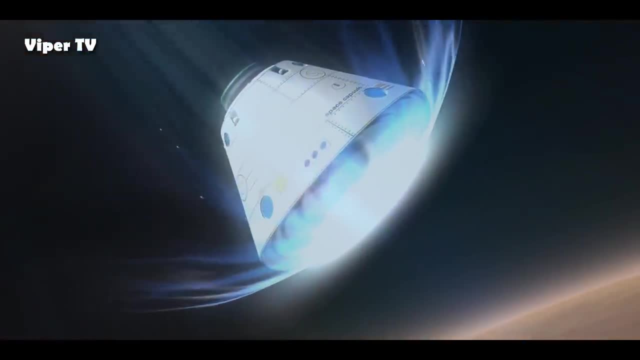 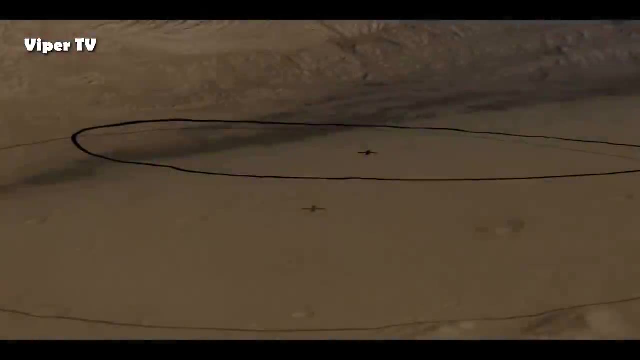 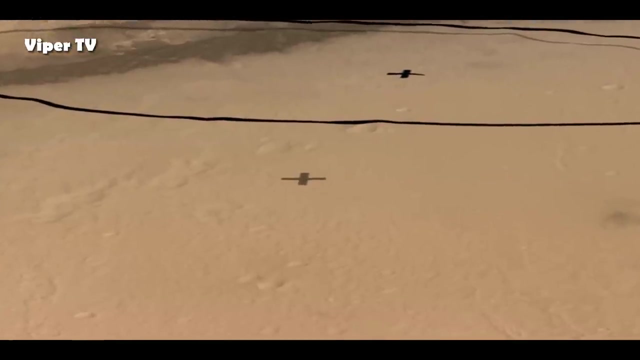 to shift the centre of mass and trajectory of the spaceship and guide it, with a design accuracy of around 10km, towards the chosen landing site. This guided, rather than ballistic, trajectory allowed for a much wider choice of landing sites for Curiosity than for the previous landers. 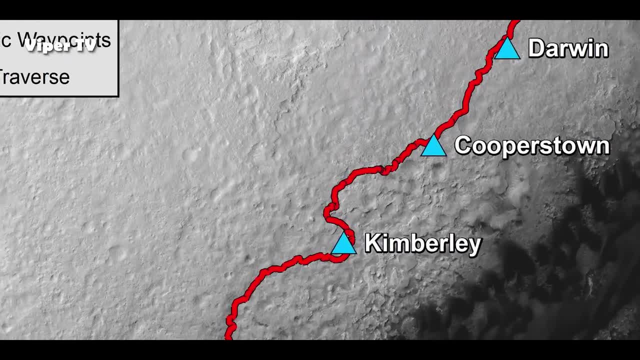 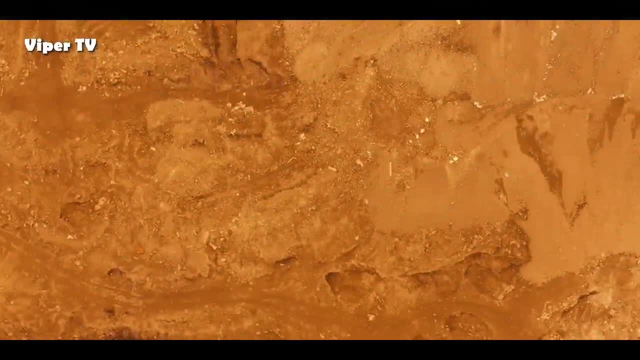 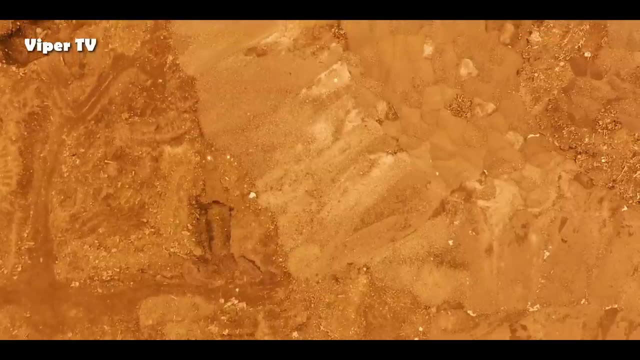 which required around 100km of flat, safe land at a nominal touchdown point, But it also required the rover to fly itself. The round-trip travel time for a radio signal to Mars was over 13 minutes when Curiosity landed, making control from the Jet Propulsion Laboratory in California impossible. 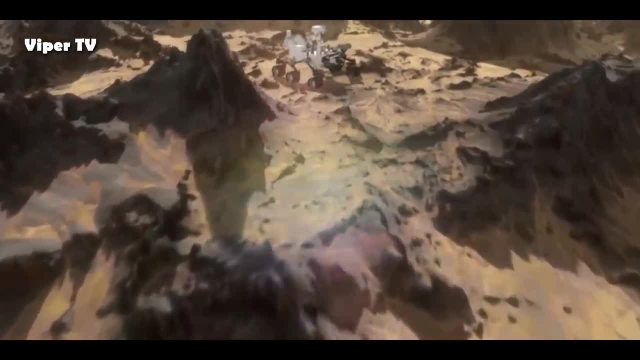 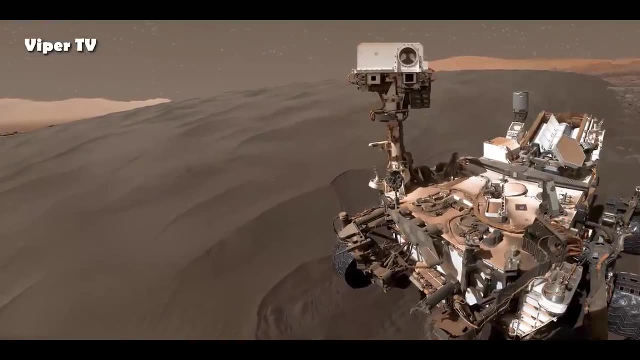 During the first stage of descent. a heat shield constructed from a unique material known as PICA, Phenolic Impregnated Carbon Ablator, protected Curiosity from peak temperatures of around 2,000 degrees Celsius generated by friction in the thickening Martian atmosphere. 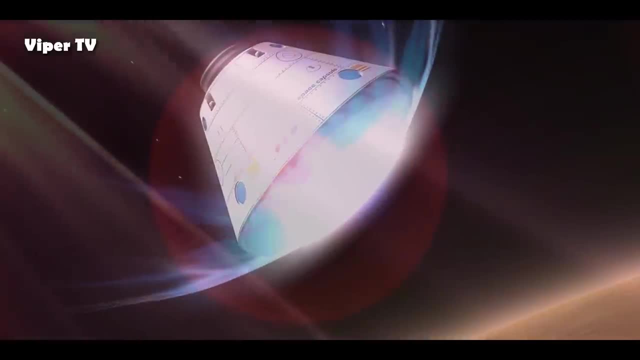 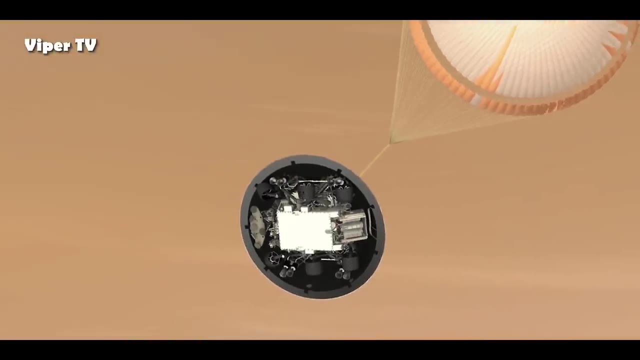 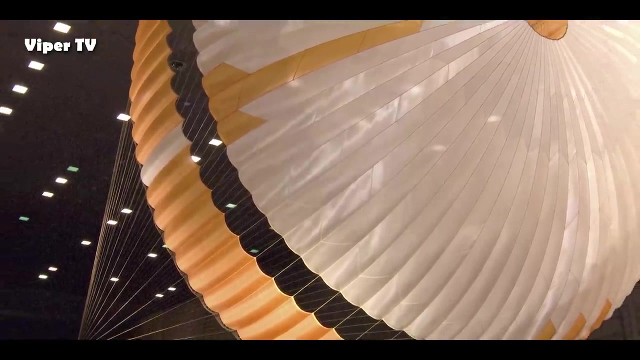 Four minutes after beginning the entry phase, slowed to just under 3,000km per hour. Curiosity's parachute deployed at an altitude of 11km above the surface. The supersonic parachute is a vast and complex structure: 80 suspension lines over 50m long. 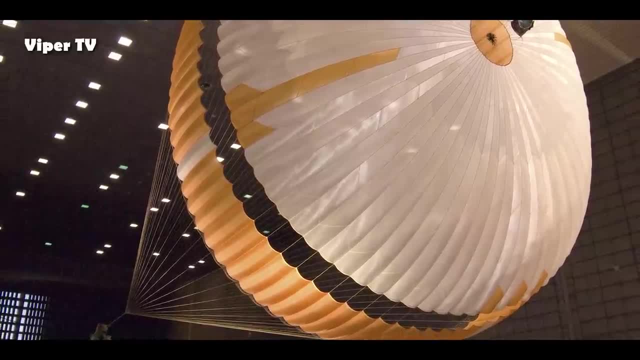 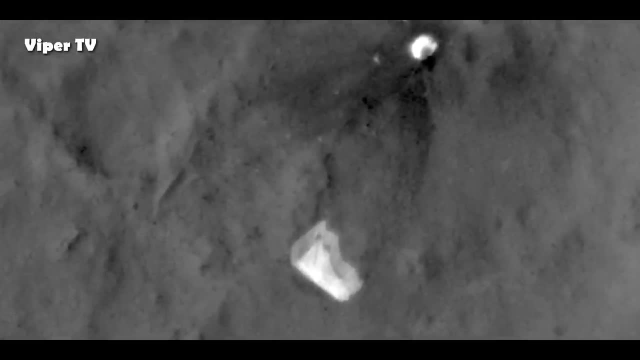 attached to a 16m canopy. Having slowed to a velocity of 700km per hour with the help of the parachute, the heat shield was jettisoned at an altitude of 8km, allowing the onboard radar to get a view of the ground. 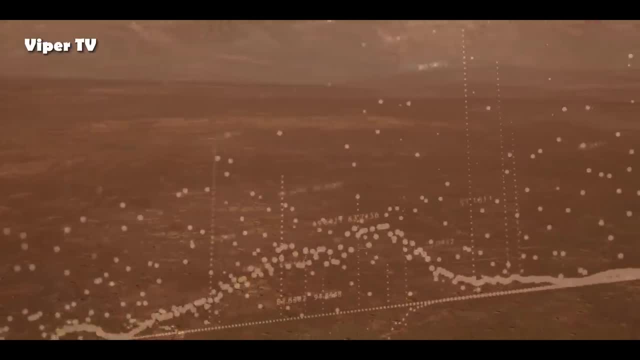 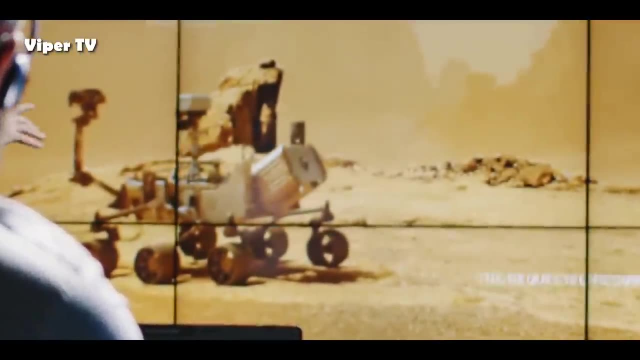 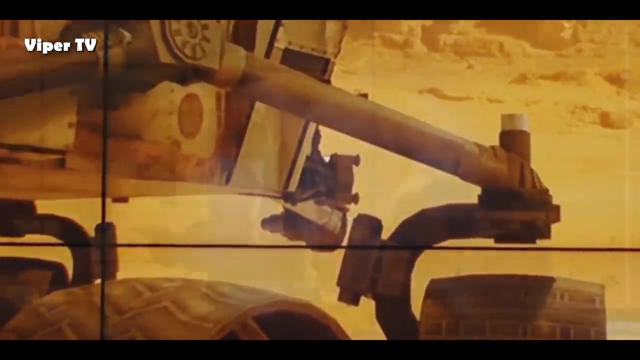 and deliver high-precision altitude and velocity measurements. With the parachute fully unfolded in relatively dense low-level Martian atmosphere, Curiosity drifted in the Martian sky for 80 seconds, descending ever more slowly At an altitude of 1.8km. 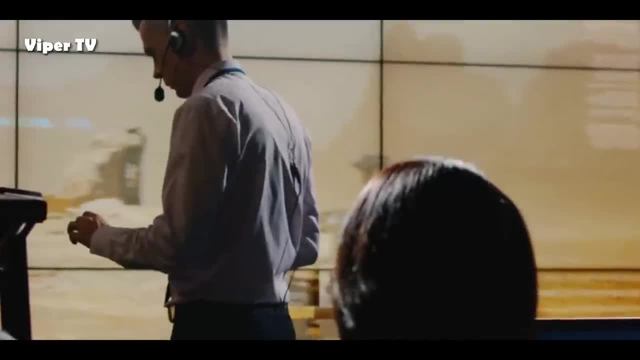 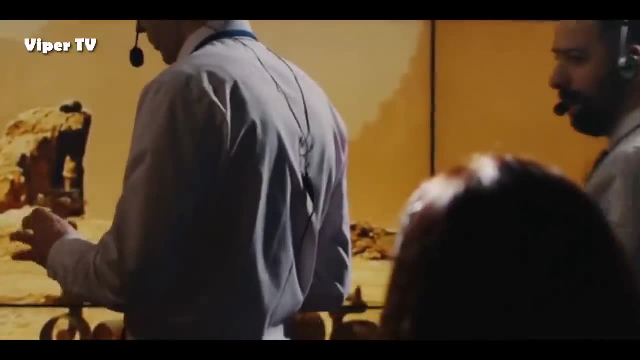 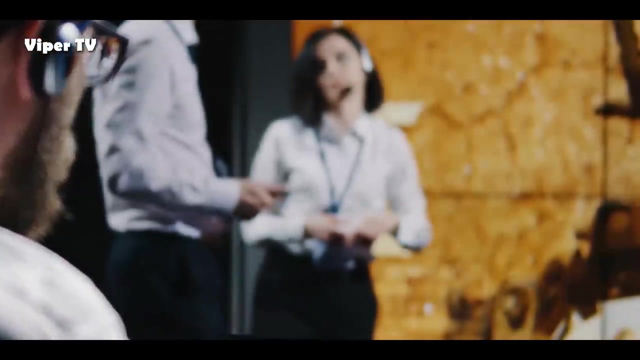 travelling at a sedate 280km per hour. the NASA timeline calls for a deep breath as Curiosity separated from the parachute system and dropped in freefall towards Mars. For engineers, says the NASA website, it's like jumping out of a plane for the first time. 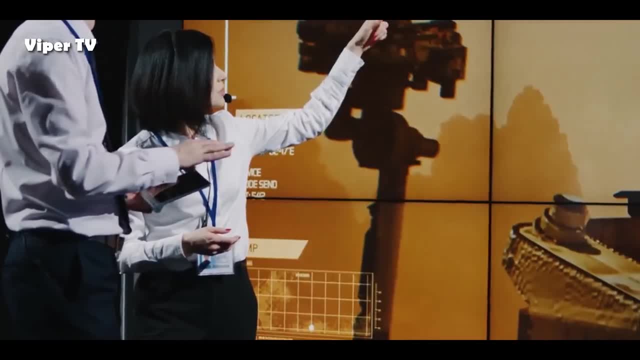 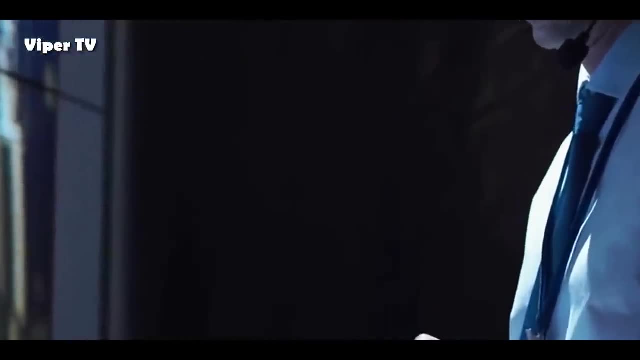 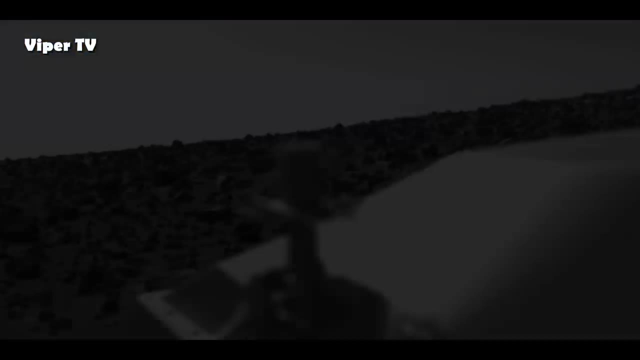 The freefall drop was designed to allow Curiosity to separate far enough from the parachute system so that it wouldn't accelerate back into it when, 300m further down, its retro rockets fired and the powered descent phase of the landing began. For the Viking landers, this was the final phase. 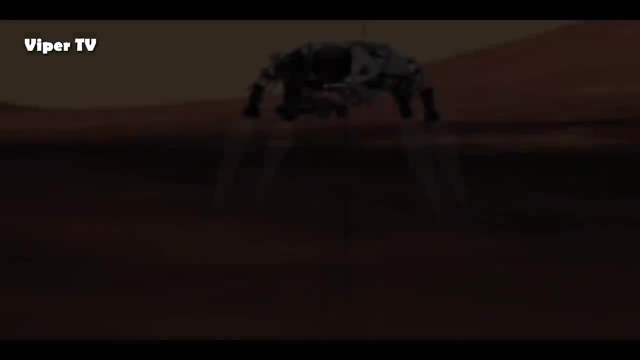 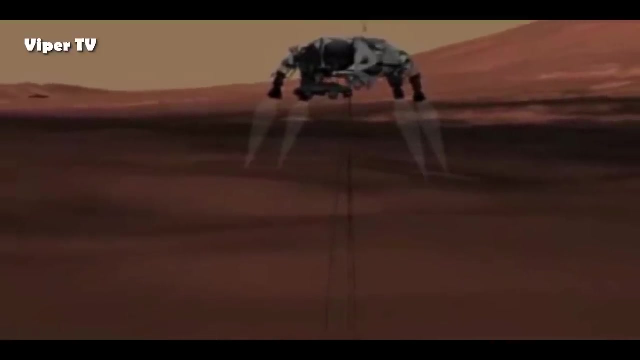 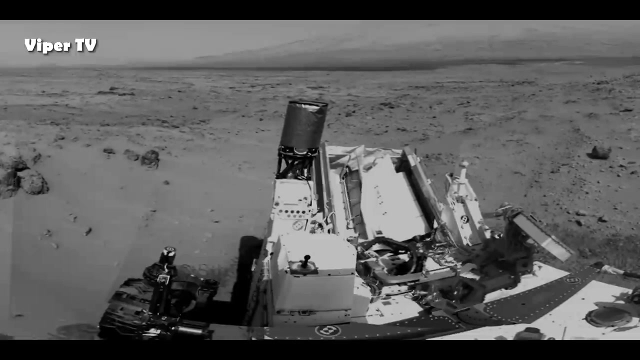 But for Curiosity, after the rockets had delivered the rover to an altitude of just 20m with a descent velocity of less than 1m per second- almost a hover- the audacious final phase of the landing protocol kicked into action The sky crane. 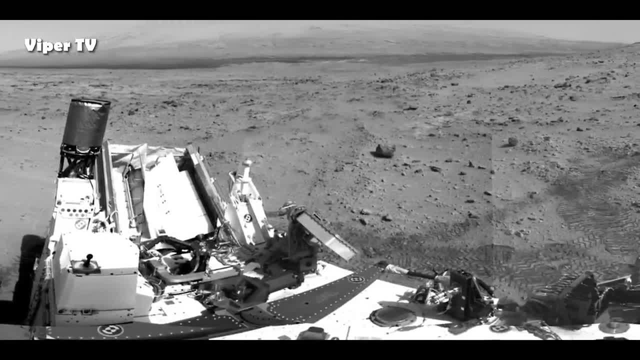 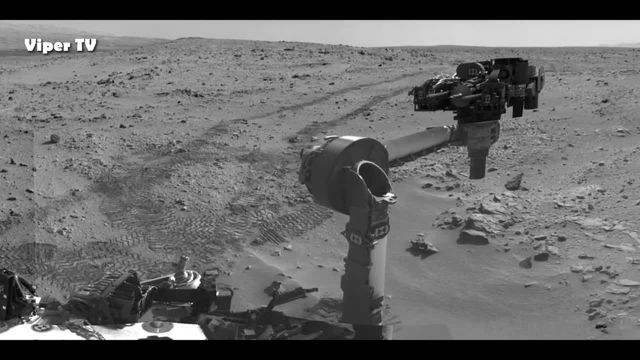 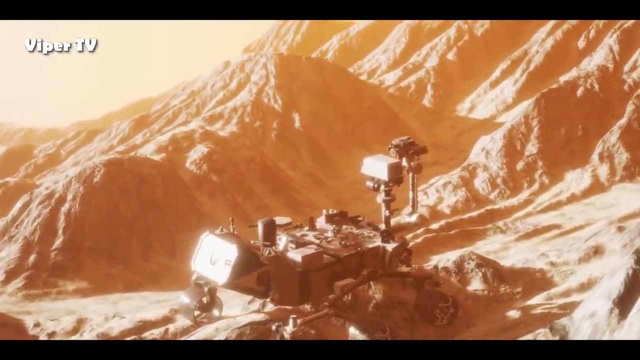 The rover slowly departed. the rocket cradle, attached by three nylon wires and an umbilical cord of electrical connections, 7.5m in length. Four of the rockets angled away from the vertical so as not to damage the rover, continued to fire. 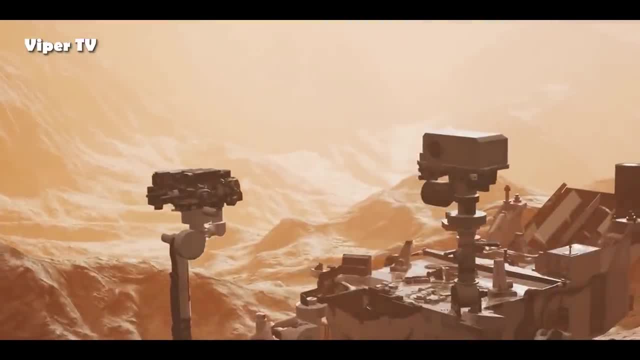 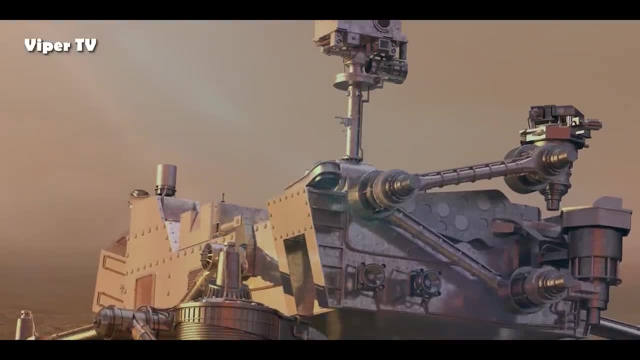 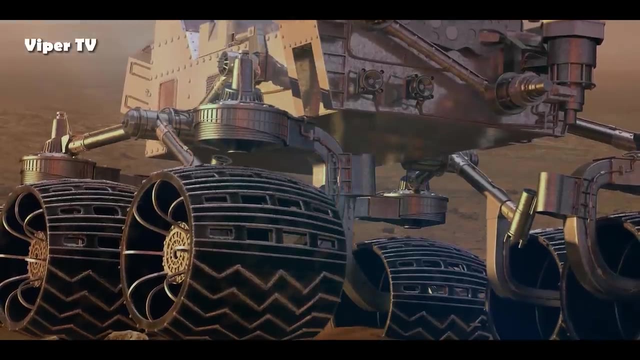 allowing the whole delicate system to approach the surface at walking pace. At 5m from the surface, Curiosity unfurled its wheels stowed for the eight-month journey from Earth. At 10.32pm the rover confirmed its wheels were in contact. 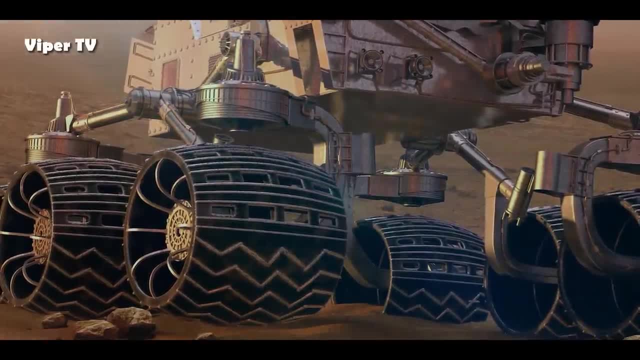 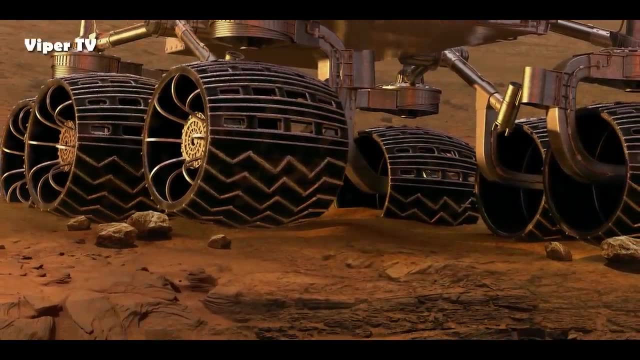 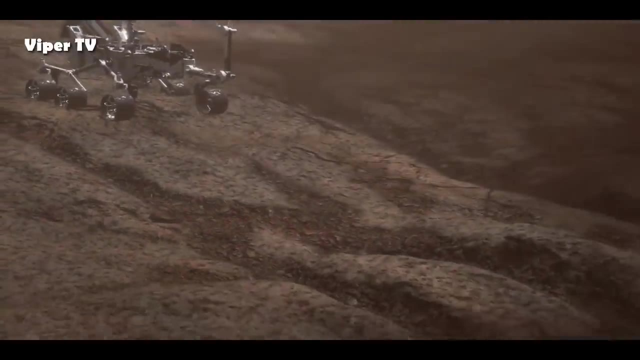 with the Martian surface and issued one last command through the electrical umbilical up to the sky. crane, I'm down, cut the cables and fly away. After a half-a-billion-kilometre journey, Curiosity was delivered safely to Mars. 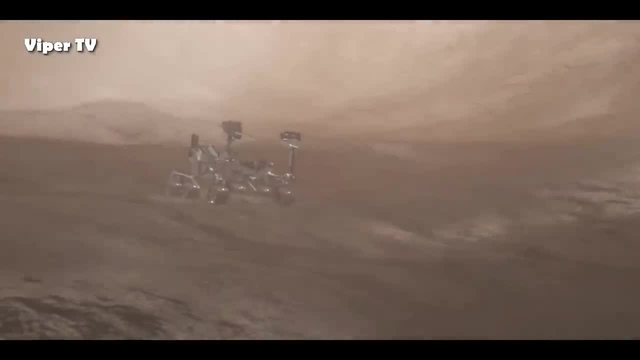 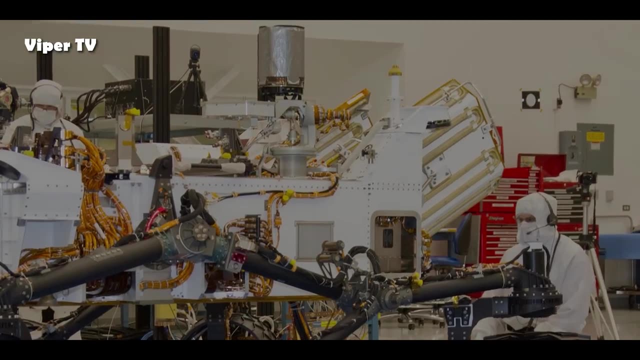 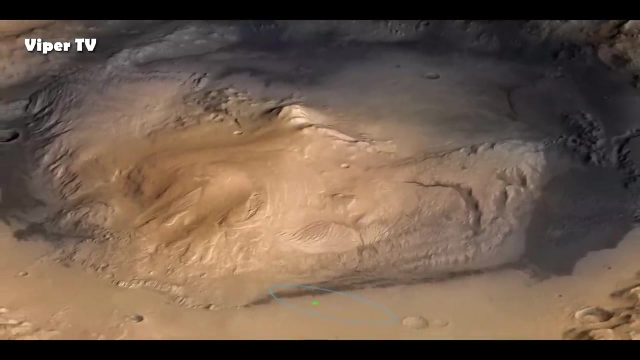 just 2.4km from its nominal landing point. A triumph of engineering ingenuity and brilliance, Curiosity was sent to Mars to explore Gale Crater, a 150-kilometre-wide impact crater formed during the late Noachian or early Hesperian period. 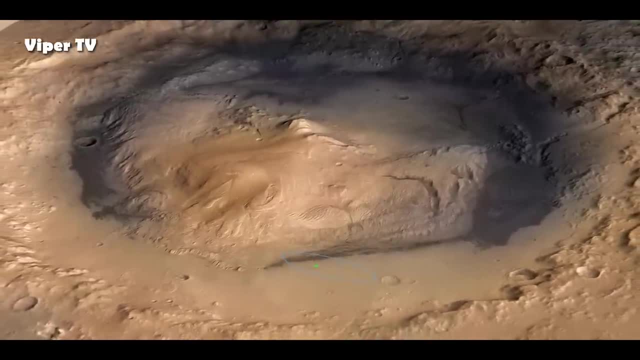 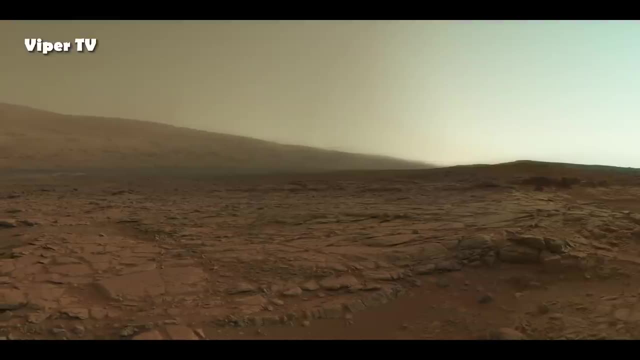 when liquid water would have been present, at least occasionally, on the surface. In the great tradition of astronomy, the crater is known as the Gale Crater. The crater is named after the Australian amateur astronomer, planetary observer, comet hunter and occasional banker. 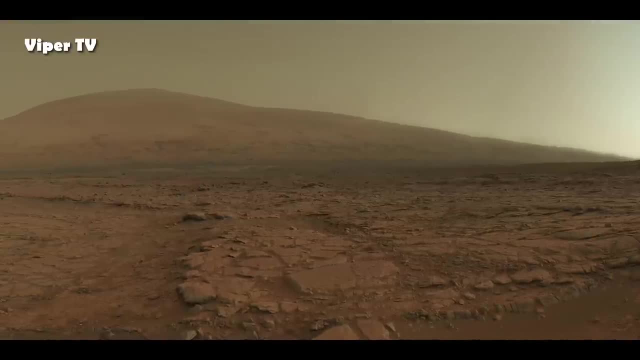 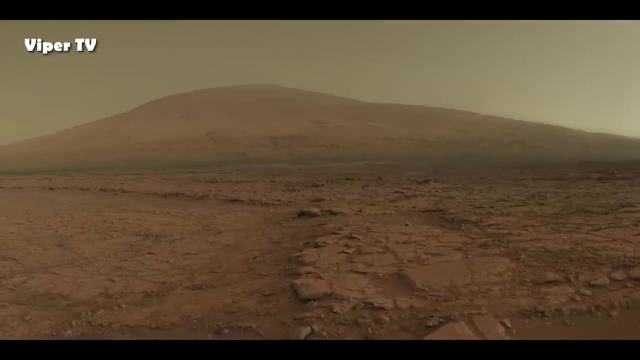 Walter Frederick Gale, who discovered a host of comets, as well as a number of geological features on Mars at the turn of the 20th century using self-built telescopes in his backyard. The primary reason for choosing Gale Crater was the unusual central structure, Mount Sharp. 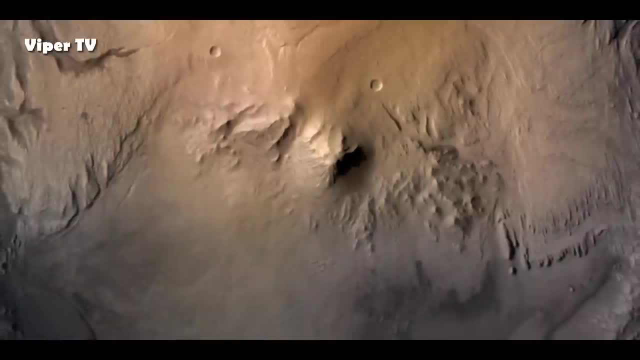 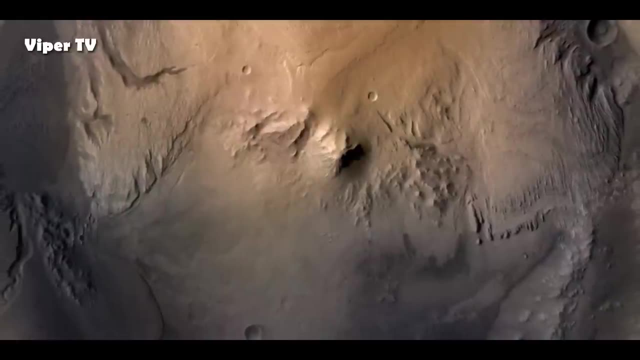 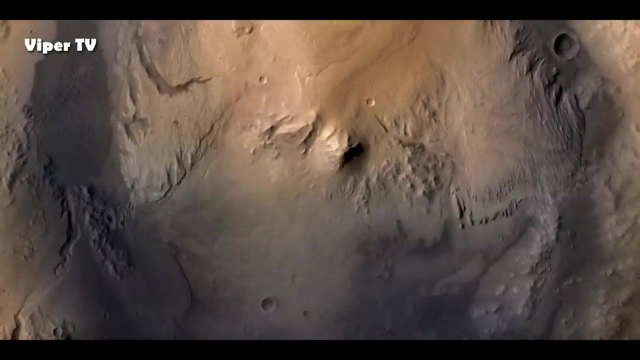 or Aeolus Mons, which rises over 5km above the crater floor. There is still debate about precisely how Mount Sharp formed, but the layers visible from orbit along its flanks suggest that it is the weathered remains of sedimentary rocks which once filled the crater. 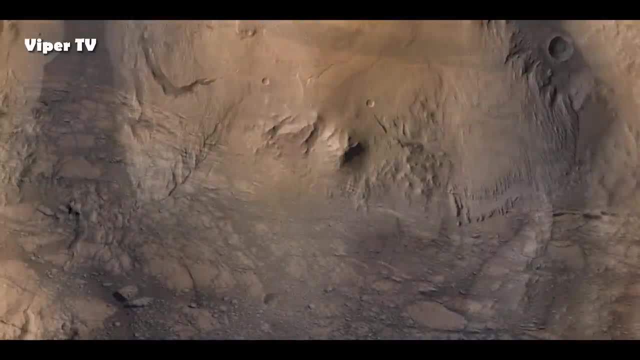 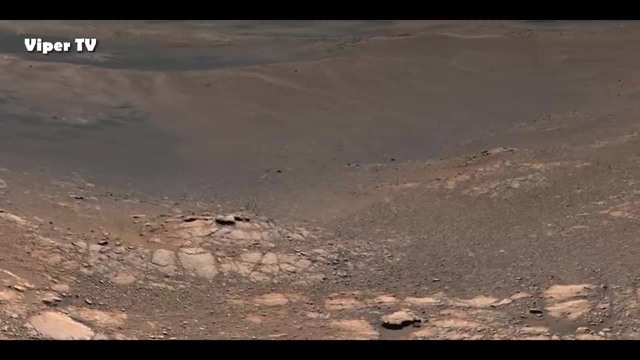 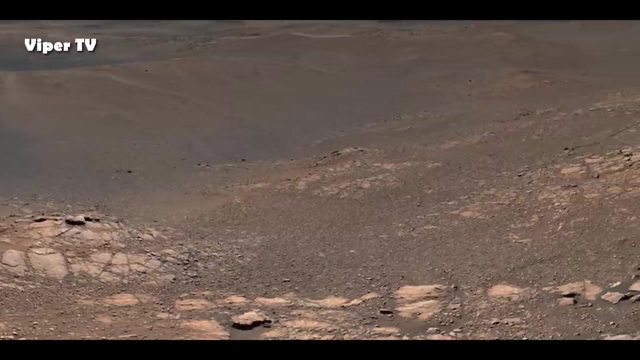 and were laid down over time. after the impact, Subsequent erosion by the relentless Martian winds removed much of the surrounding rock to reveal the ancient crater floor once more, while leaving the towering central structure intact. Deep exposed sedimentary layers are extremely enticing to geologists. 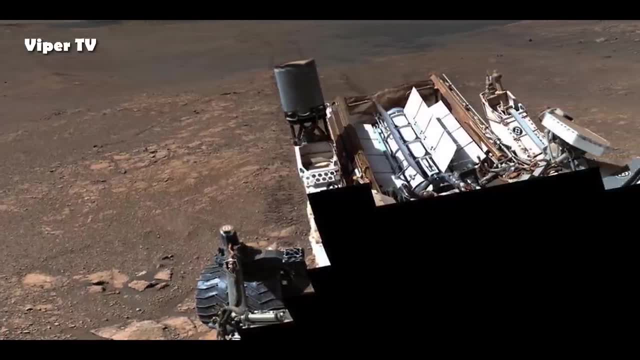 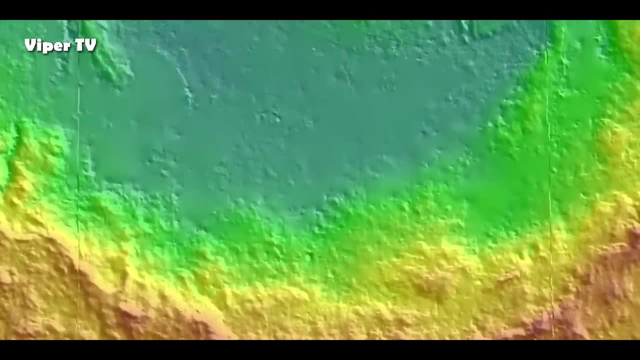 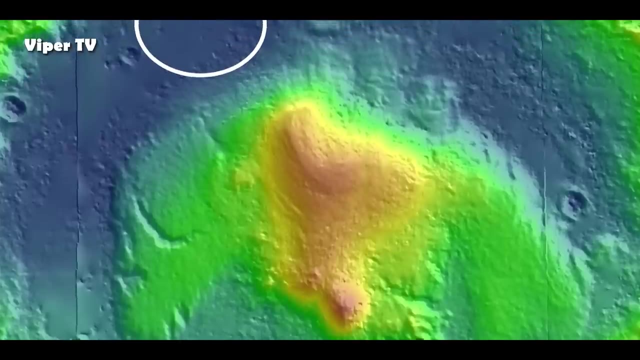 because a cross-section through rock is a cross-section through time. As surface and atmospheric conditions change, different sorts of rock are laid down and chemically modified. As Curiosity ascends the slopes of Mount Sharp, it climbs forwards through Martian time, and scientists are close behind. 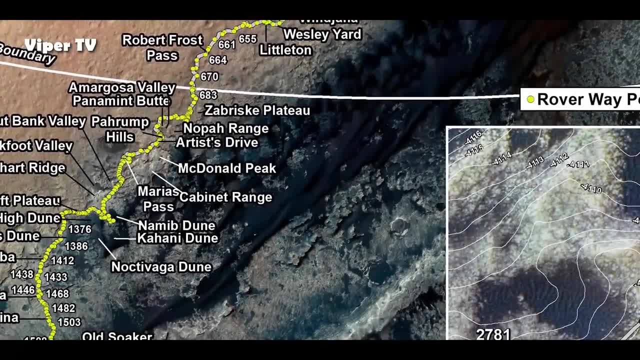 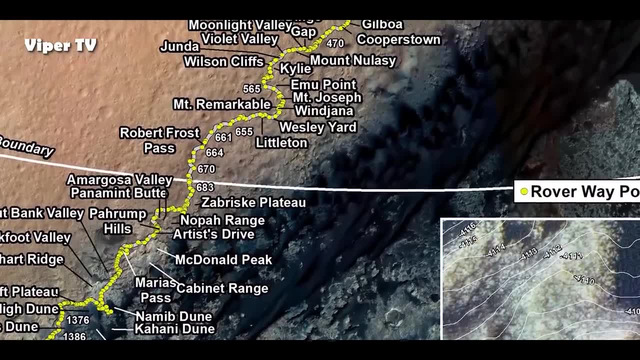 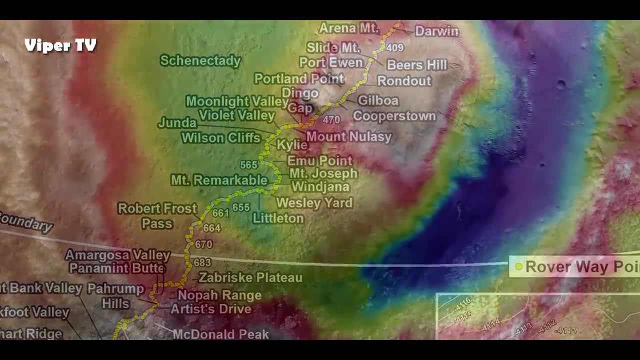 Joy Crisp, the deputy project scientist from NASA's Jet Propulsion Laboratory, explained the choice of landing site in the weeks before launch. Mount Sharp may be one of the thickest exposed sections of layered sedimentary rocks in the solar system. The rock record preserved in those layers 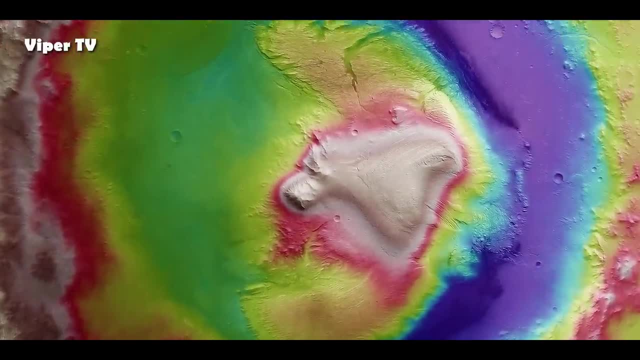 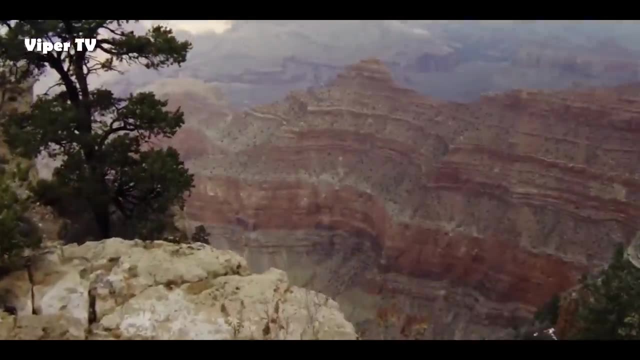 holds stories that are billions of years old, stories about whether, when and for how long Mars might have been habitable. Just as the layers of exposed rock in the Grand Canyon on Earth reveal the story of our planet, the exposed sedimentary layers of Mount Sharp. 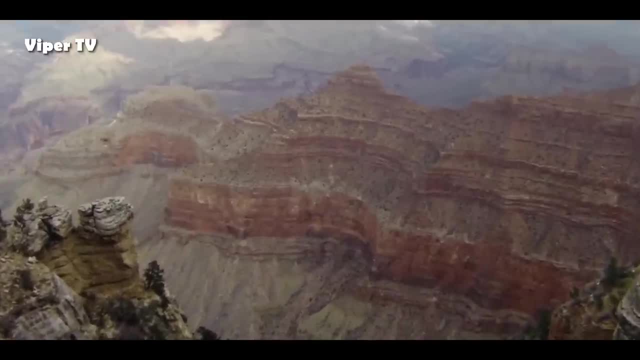 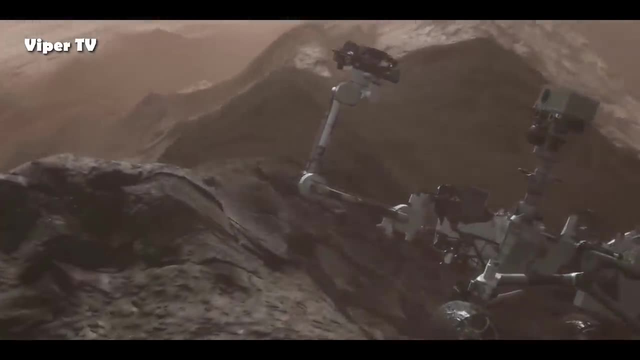 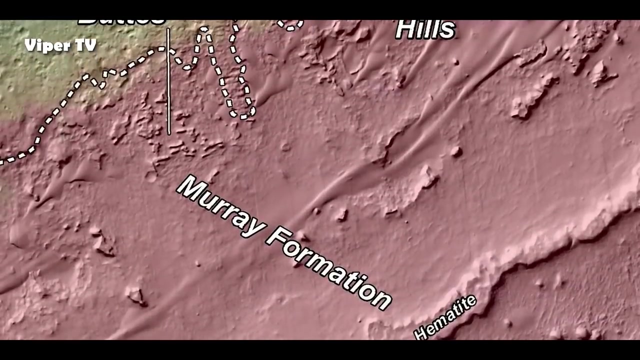 are a storybook that the winds of Mars have opened, ready for Curiosity to read. At the time of writing, Curiosity has travelled almost 19 kilometres from its landing site on the flat plains to the lower slopes of Mount Sharp, stopping along the way at each interesting site. 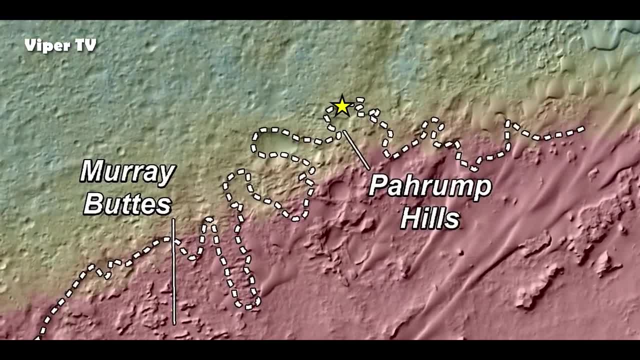 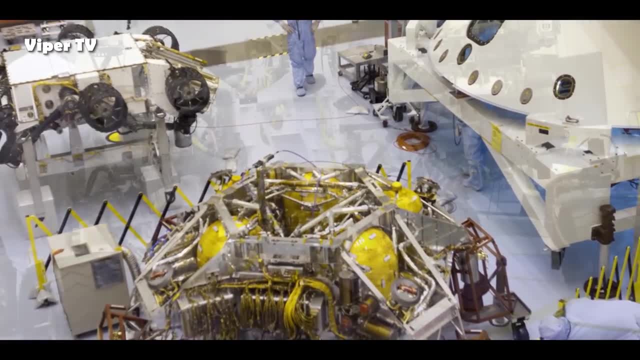 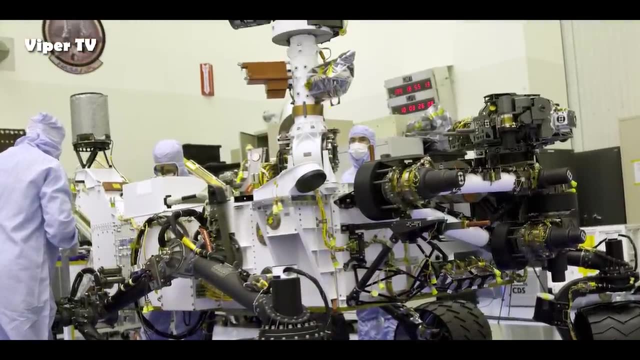 to characterise the geological environment. Curiosity's suite of scientific instruments is the most sophisticated ever installed on a spacecraft. The rover is a mobile geological laboratory capable of analysis of the Martian surface and the layers just beneath. NASA loves acronyms. 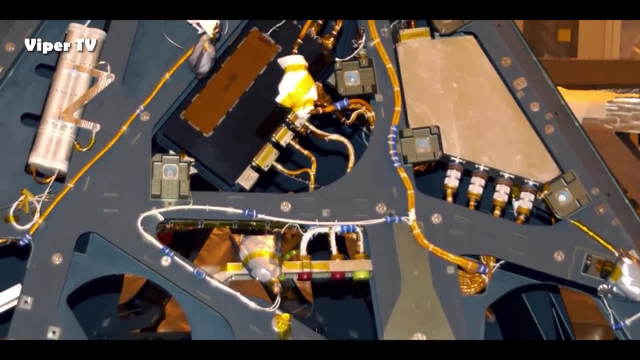 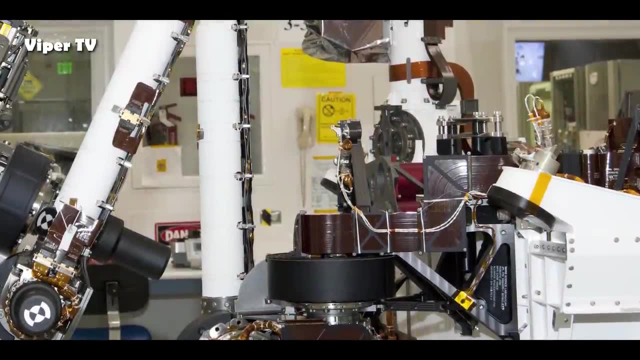 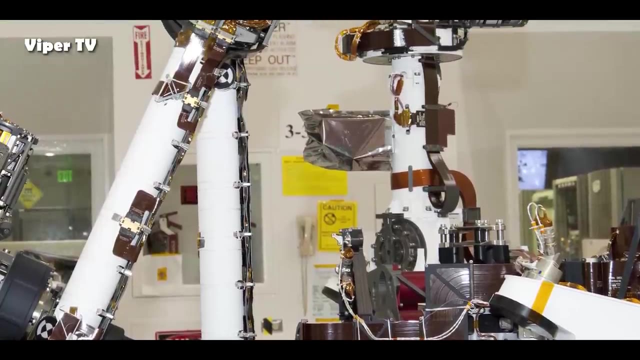 Curiosity acquires samples using the SSS, the Surface Sampling and Science System. It is made up of three parts: the SASPA Sample Acquisition, Processing and Handling Subsystem. SAM Sample Analysis at Mars Instrument. and CHEMIN Chemistry and Mineralogy Instrument. 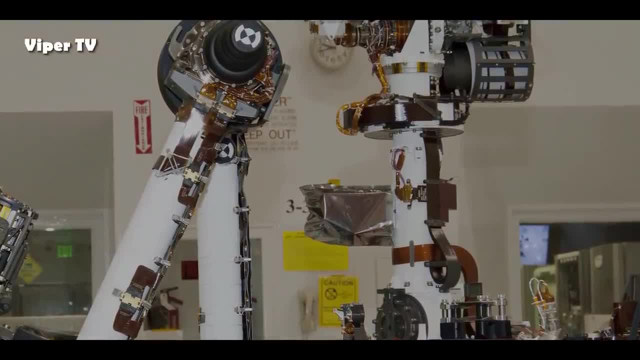 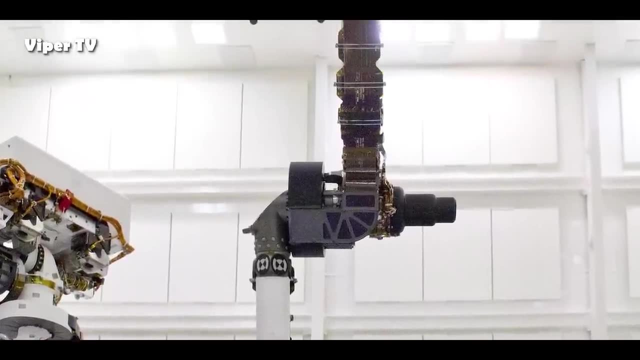 The main components of SASPA, which is mounted at the end of Curiosity's robot arm, are an Integrated Scoop and Sample Processing System, CHIMERA, and a drill for acquiring surface and subsurface samples. The Scoop and Sample Processing System. 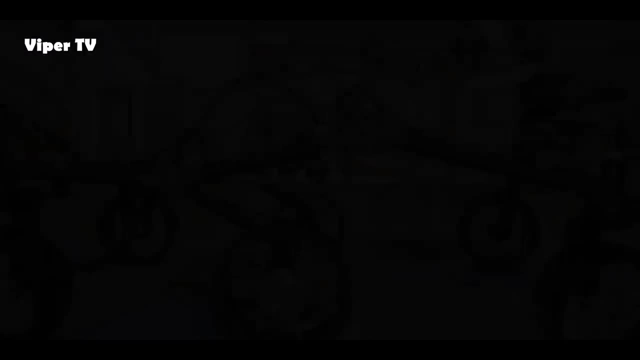 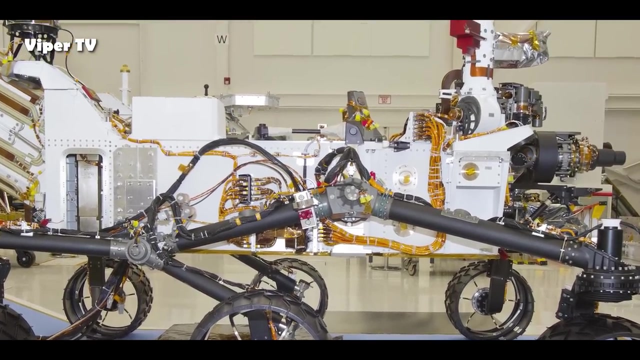 surely has one of the most inventive of all NASA acronyms, CHIMRA, pronounced CHIMERA, after the multi-headed creature of Greek mythology which stands for the Collection and Handling for In-Situ Martian Rock Analysis Tool. Someone deserves an award for that.